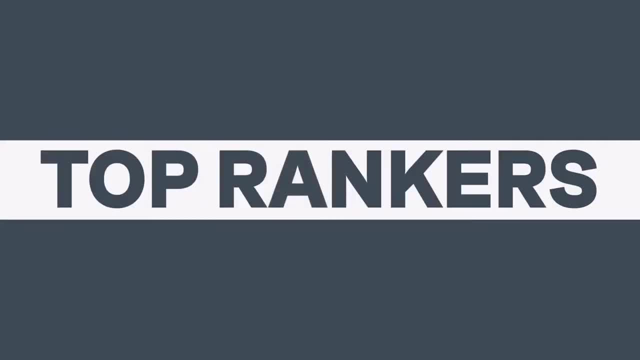 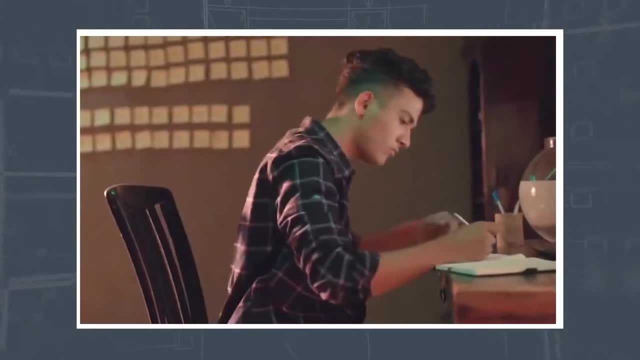 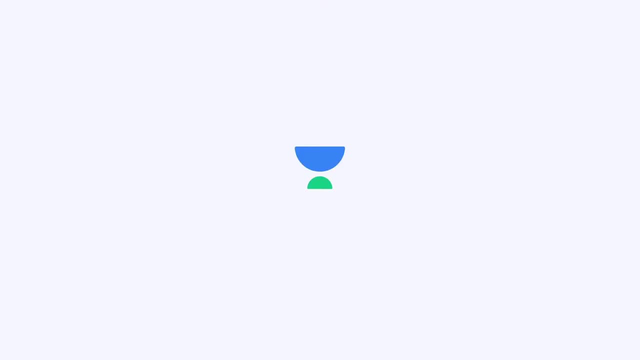 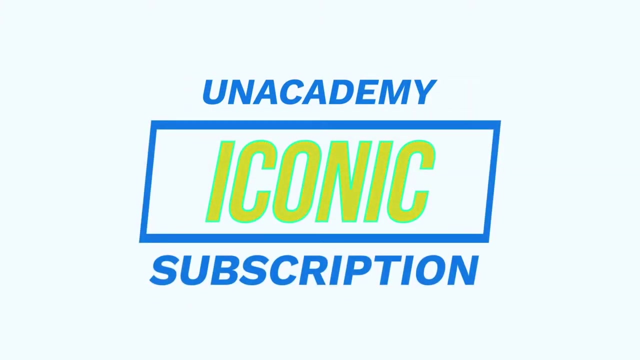 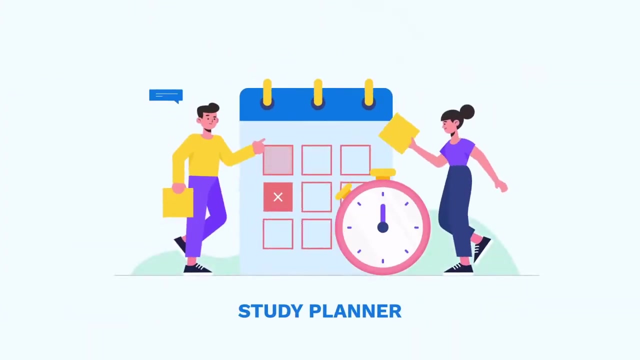 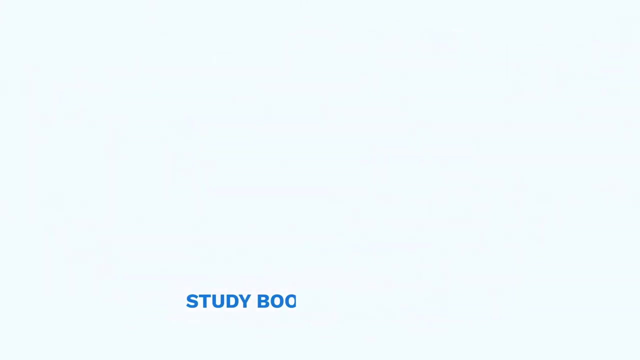 Live ranking after every question. Big rewards for top rankers. Your passion to crack GATE deserves this. Your hard work towards your dream deserves this. Fuel your inner fire for the ultimate GATE challenge. Unacademy Combat Register, now Untitled with our call: Mako heiksen. 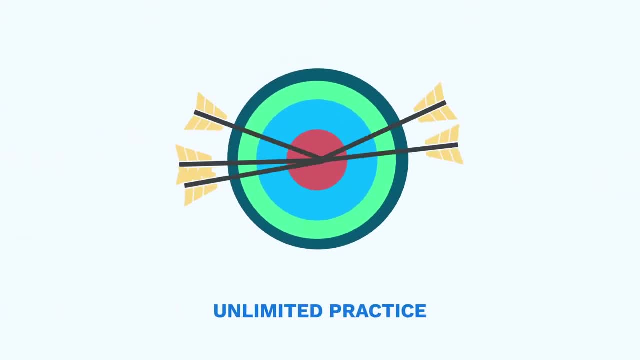 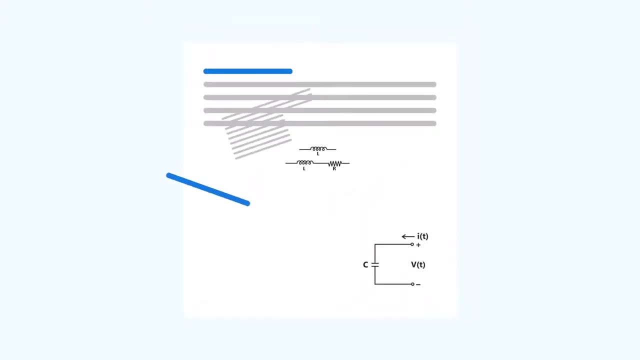 From all of us who work in GATE by carry on with the gauge. Thanks to my colleagues in HDK, With the passion and patience And full instructions you will get, Make sure you win on the Dream building Archives Day. Run and train as much as you can. 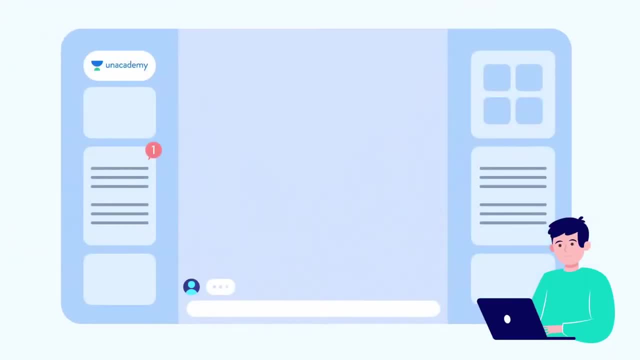 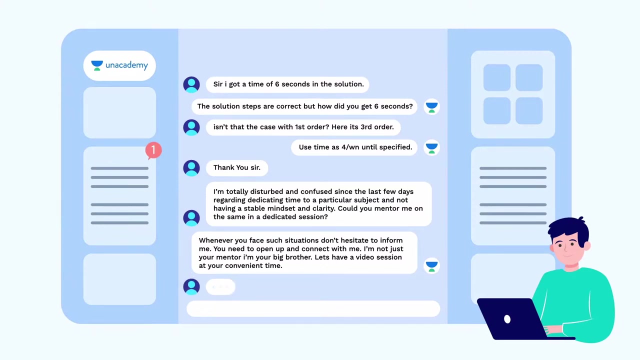 IT's so much fun. Enjoy the best of your GATE experience And don't forget: If you want to win your GATE Champions Muslims Championship, You will want to go through a total sievert test, Nice, to meet you. I'll see you next time. 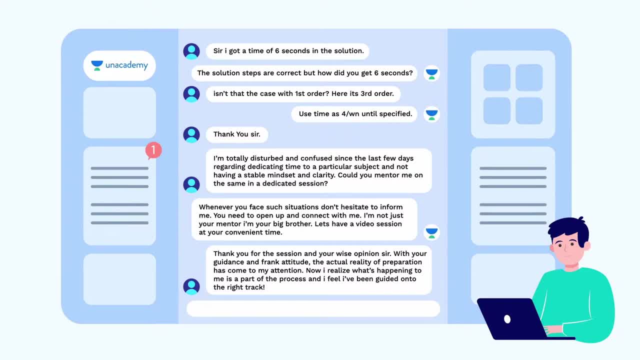 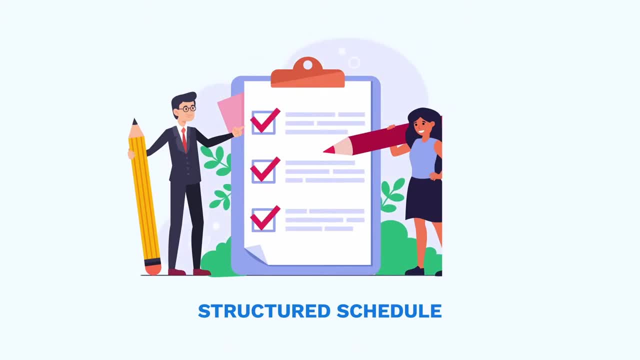 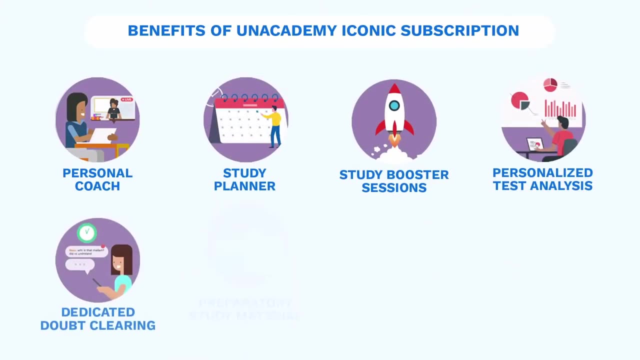 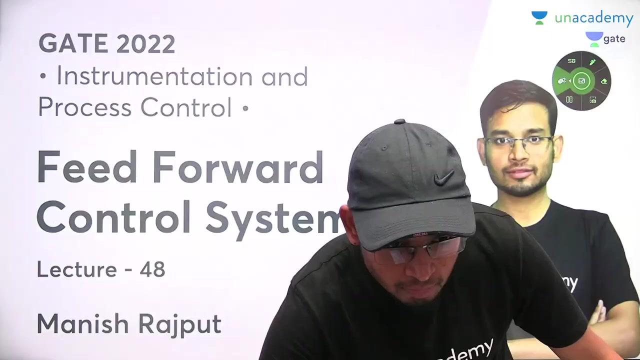 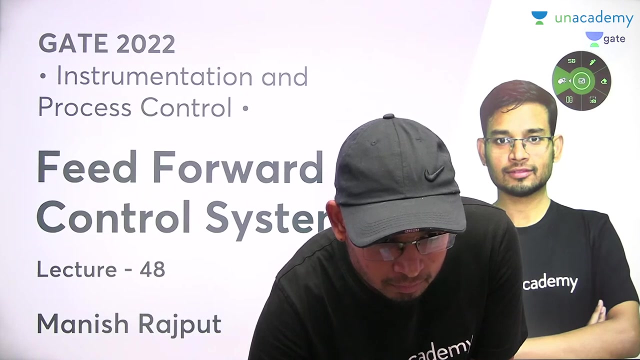 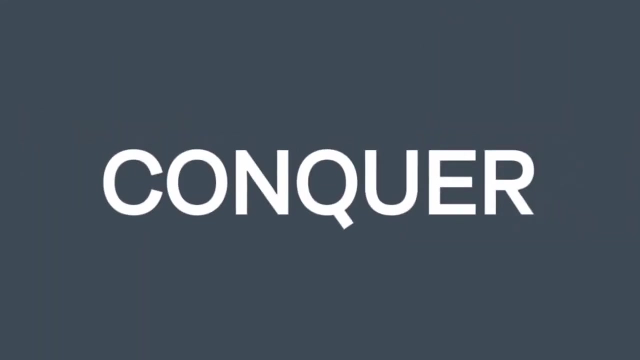 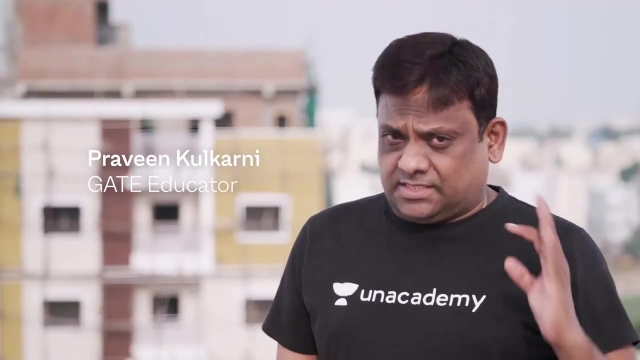 Bye-bye. It's time to experience something glorious: Unacademy Combat, Compete, Crack Conquer. A challenging gate contest engineered to give you an experience like none other, Where you put your knowledge to test And battle it out with the best. 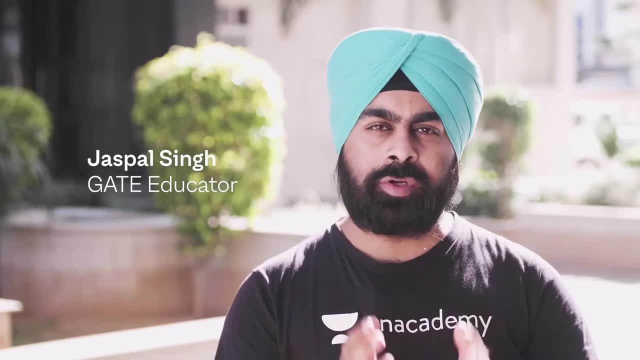 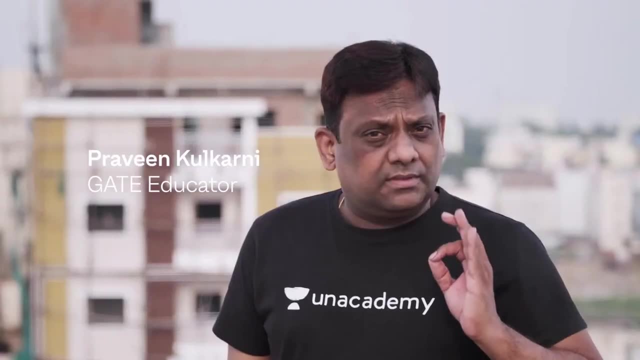 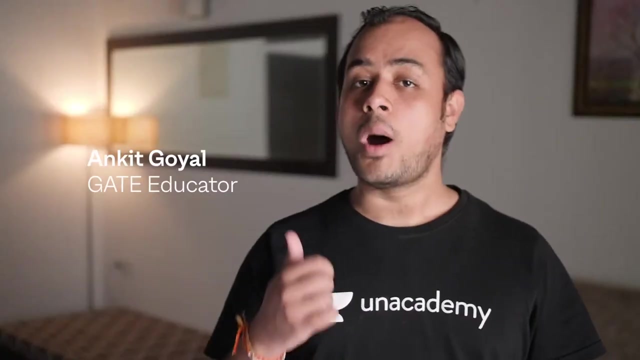 To bring out the best in you. Unacademy Combat is the most competitive gamified contest for the gate till date, With the best of the questions by best educators, With detailed videos, Solutions from top educators Right after each contest. Combat live with peers. 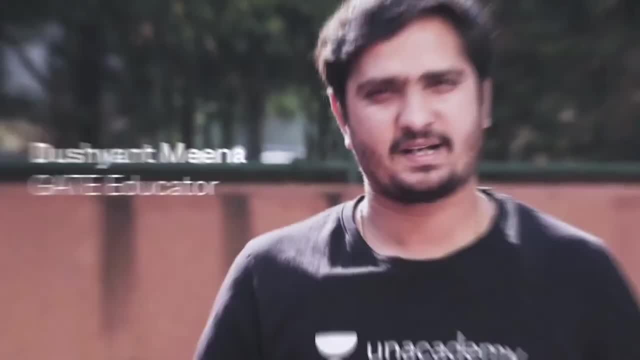 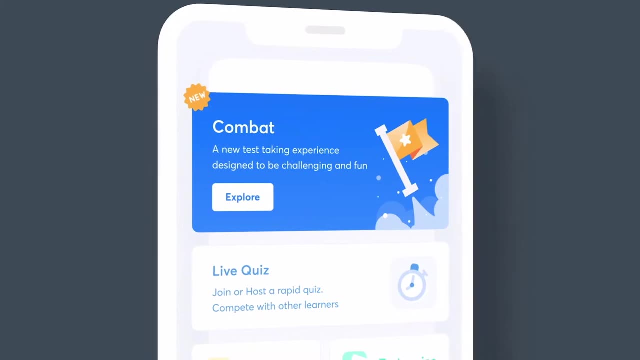 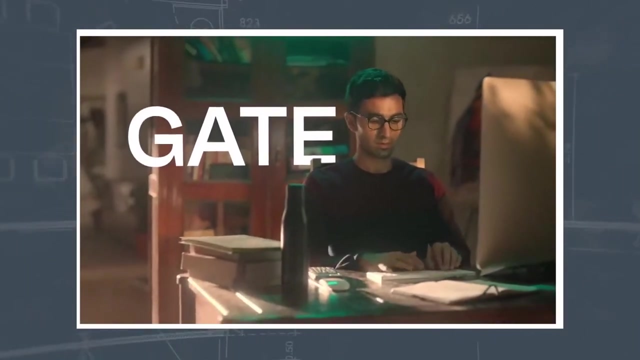 to get real-time rankings and win big. Participate in every contest to improve your ratings. Challenging contests every fortnight or alternate Sunday. Live ranking after every question. Big rewards for top rankers. Your passion to crack gate deserves this. 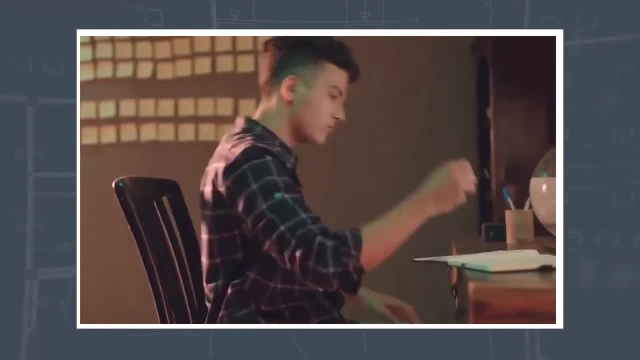 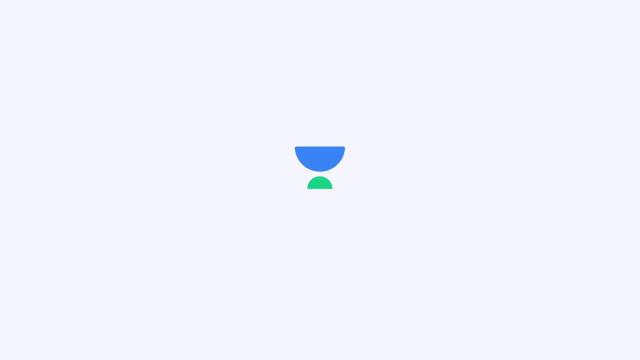 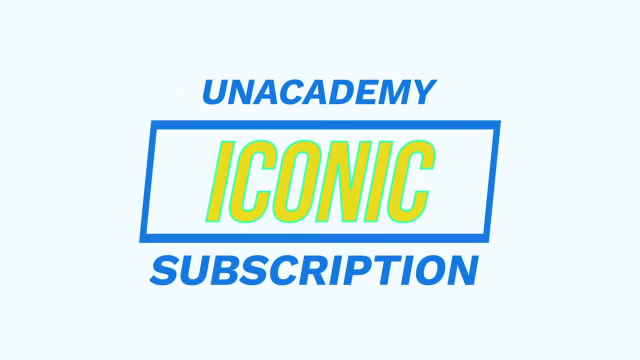 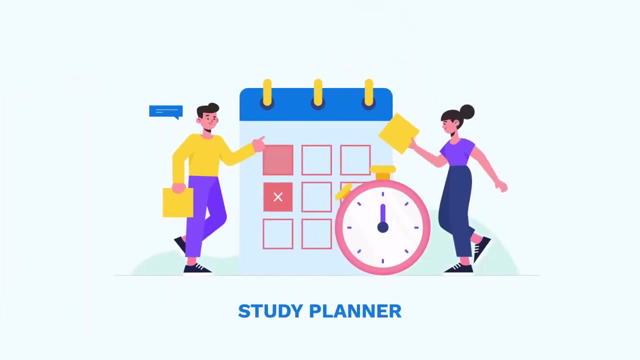 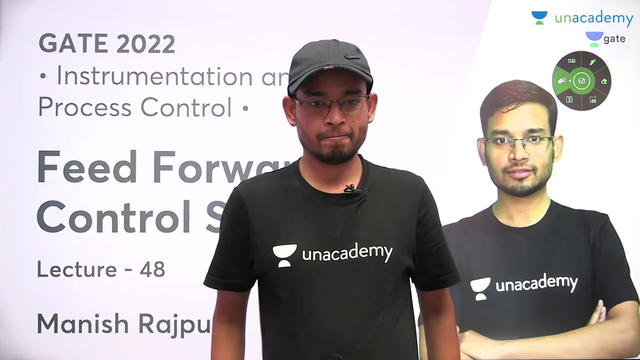 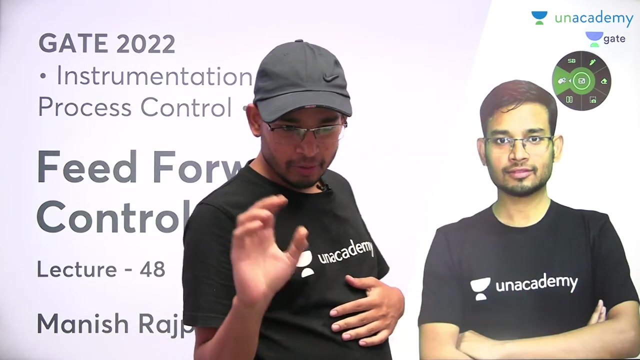 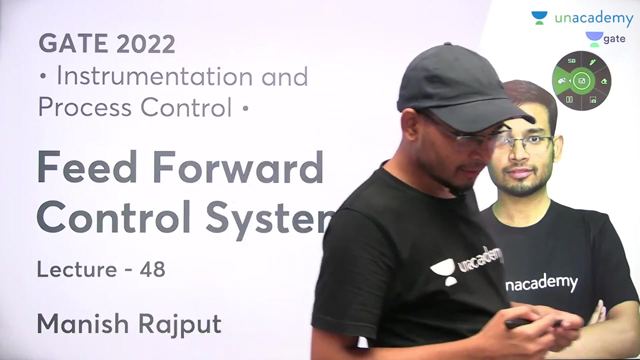 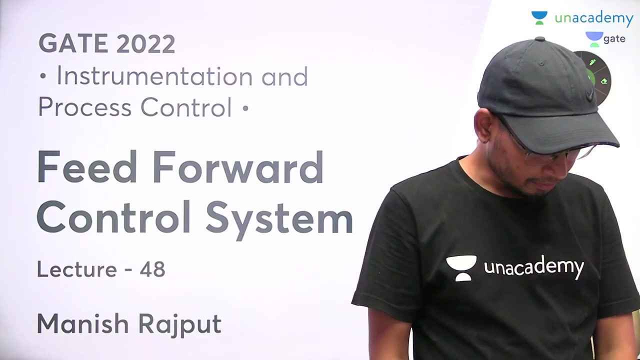 Your hard work towards your dream deserves this. Fuel your inner fire For the ultimate gate challenge. Unacademy Combat Register now. Now I can promise you that you won the first round. saharan lapsism: back up to your uh. 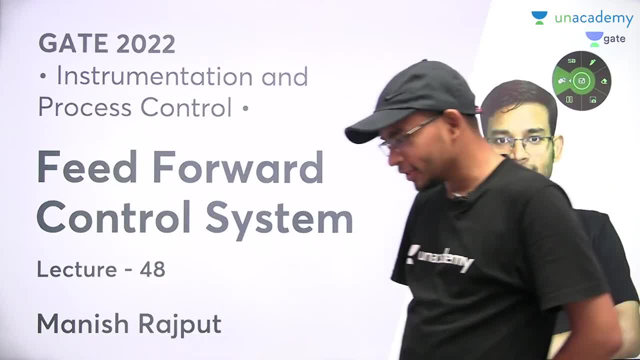 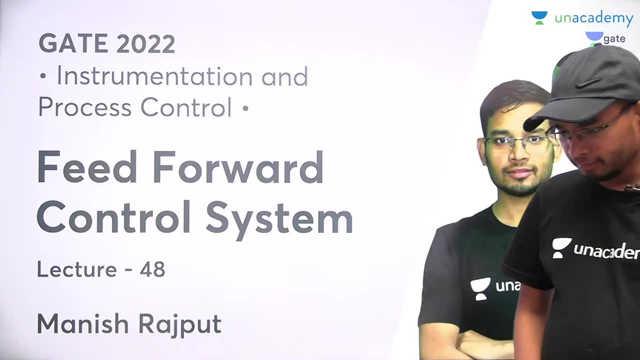 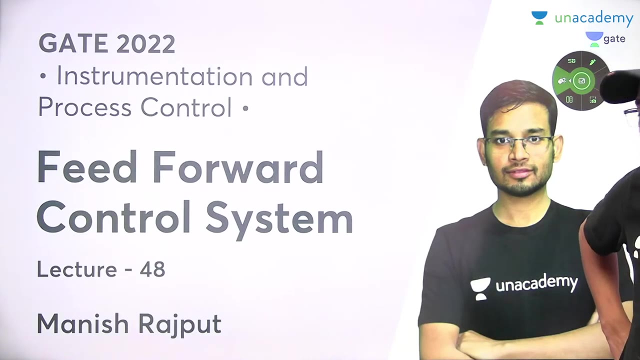 Yes, Are just a look. We will inform everyone so that everyone will join the session. We will inform everyone so that the maximum number of people at least reaches us. So we are going to talk about the advanced control strategy, in which we will talk about part A. 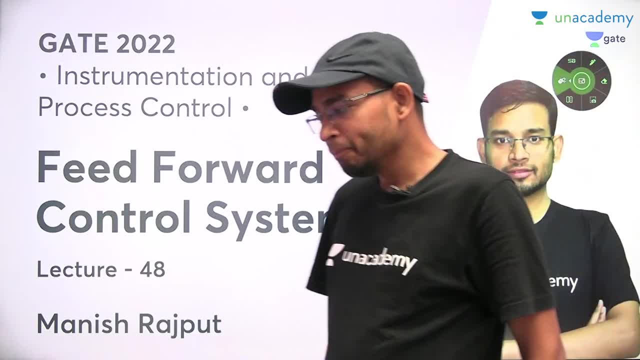 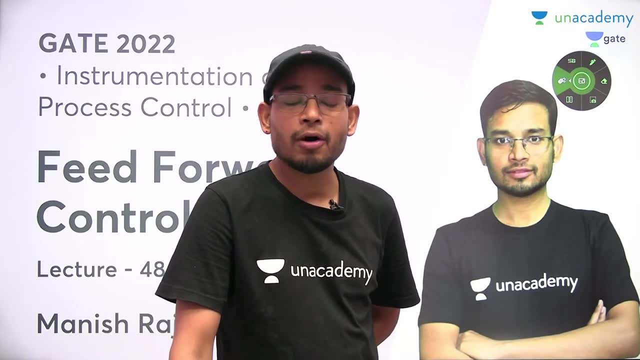 Feed forward controller. till now, you have talked about tuning. You had talked about tuning, you had talked about Jigal and Nicholas in tuning. The second method you had studied was cone and cone. The third one you had studied was body stability criteria. So with these three methods, you had tuned the controller. 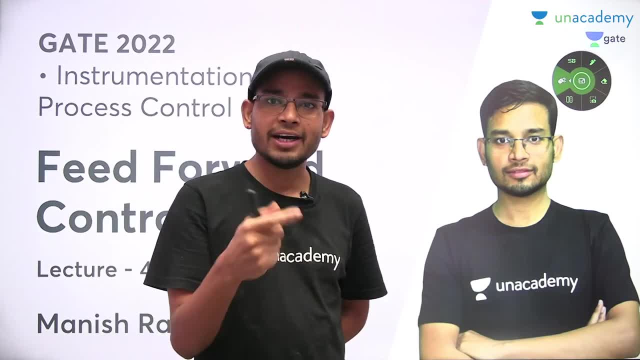 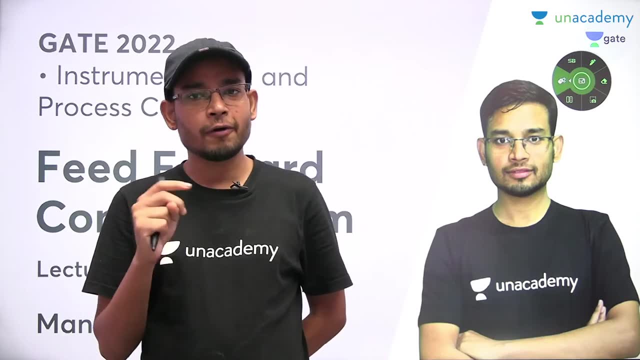 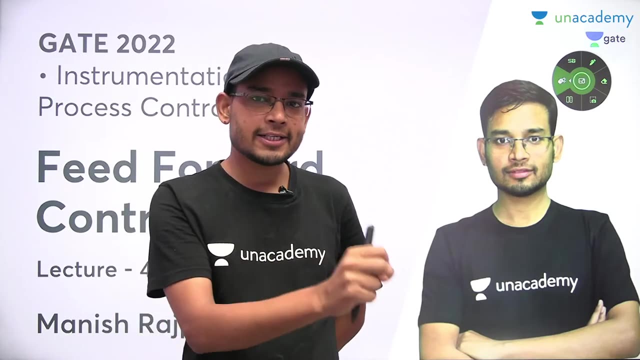 Now we will talk about how to make the controller more advanced. So we will talk about the advanced control strategy, in which you will study two strategies: First, feed forward control strategy one. The second one you will study on Monday, That is the cascading. Cascading will be the last part of the advanced and IPC. 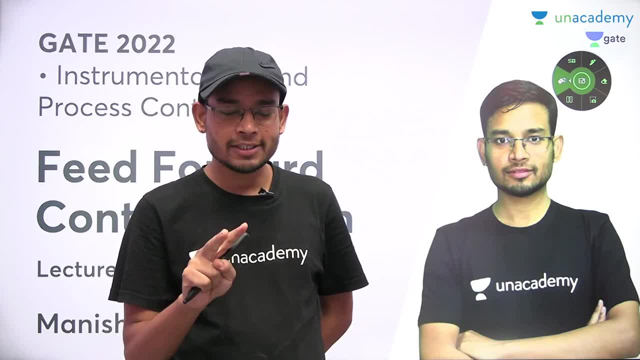 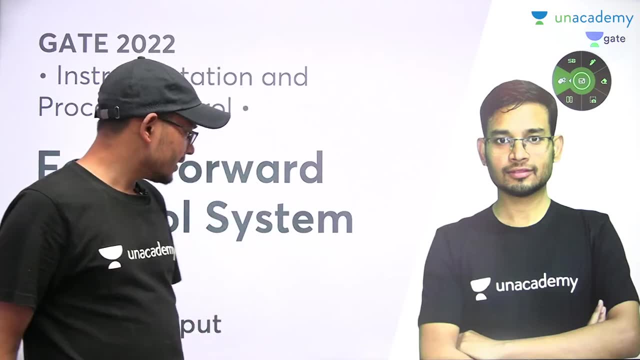 Okay, So your session will be over on Monday. Only two advanced techniques are left Today. we will complete feed forward And we will cover cascading on Monday. Okay, So I will just start the session from here. So, for those who are new students, I will tell you a little about myself. 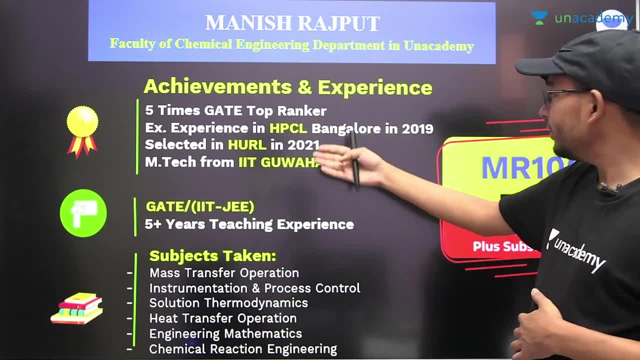 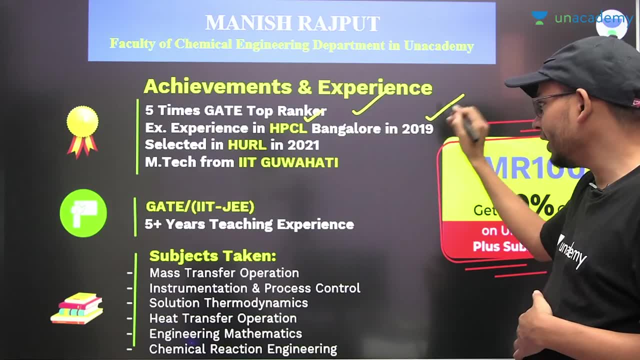 So I am Manish Rajput and this is my experience and achievement, as you can see here. Okay, you can see- And five times get qualified X experience in the HPCL Bangalore in 2019. Selected in the HURL in 2021. I am a tech friend. 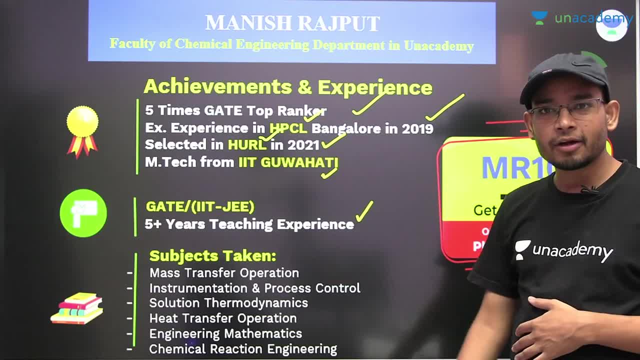 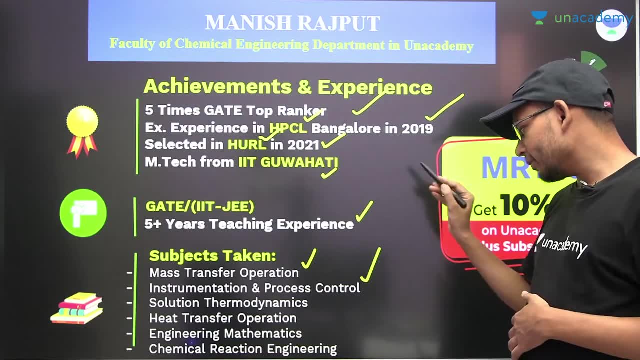 From IIT Guwahati And 5 plus this teaching experience, If we will talk about the my subject. So you must be seeing the subject. like all the people will be almost aware of the mass transfer operation. Okay, All the people are also aware of instrumentation and process control. 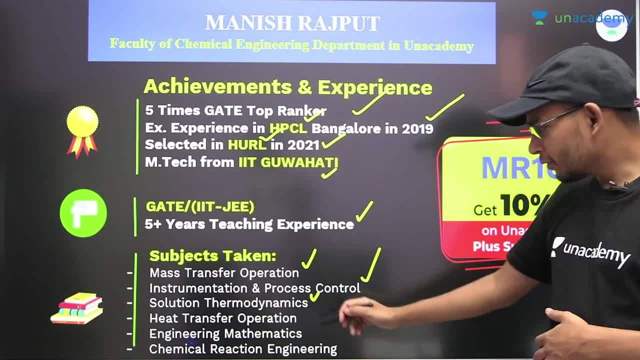 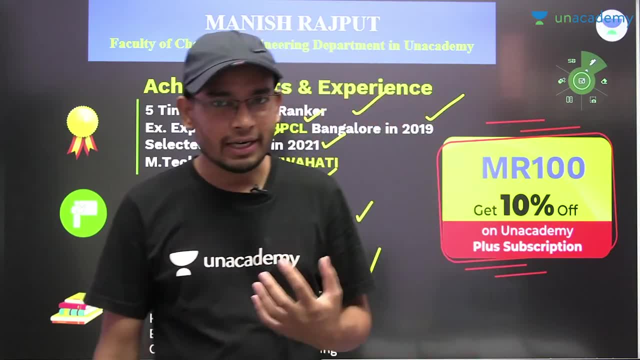 Many people will be aware of solution thermodynamics. Some people are not aware, So we will talk about them: Heat transfer engineering, mathematics and chemical reaction engineering. You can get to see this subject in the next session or in the coming time, And this is the my code. 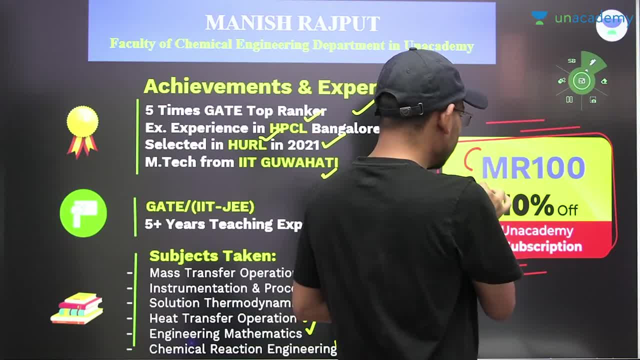 You can use this code: duration of the joining the plus course or iconic course. Okay, You can use this code duration of the joining the plus course or iconic course. You can use this code: duration of the joining the plus course or iconic course. You can use this code: duration of the joining the plus course or iconic course. 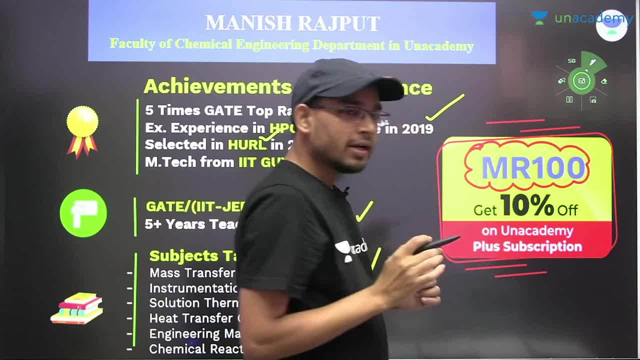 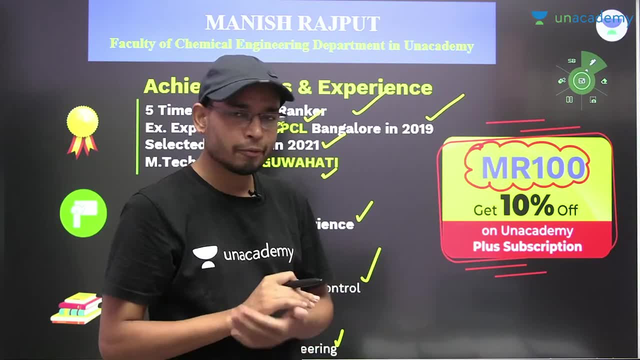 You. you can use this code. duration of the joining the plus course or iconic course. Okay, This is my code. OK, MR100, You can move from here properly. And the offer which is going on in the current. I will tell you the last date of the offer. 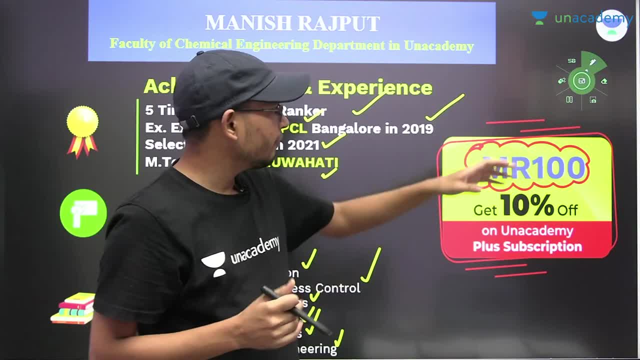 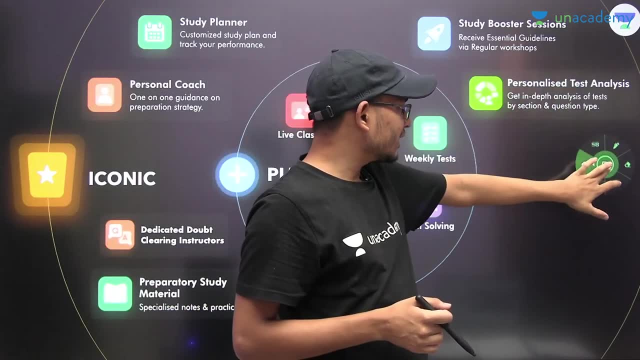 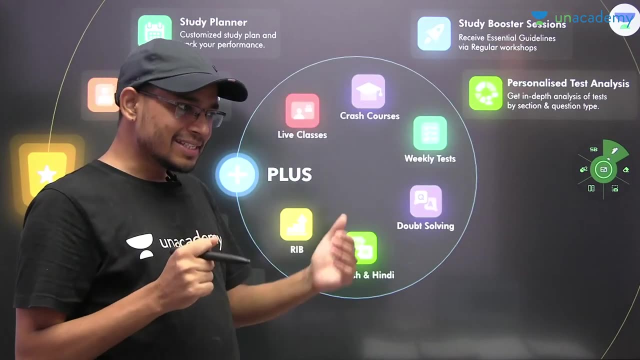 Ok. So whenever you need, You can move with a proper faculty code. You can enjoy the journey of plus properly from here. Come on, Incase you join plus. Whatever the whole story of the plus, I tell you And what will you get in the plus. So incase you join plus. 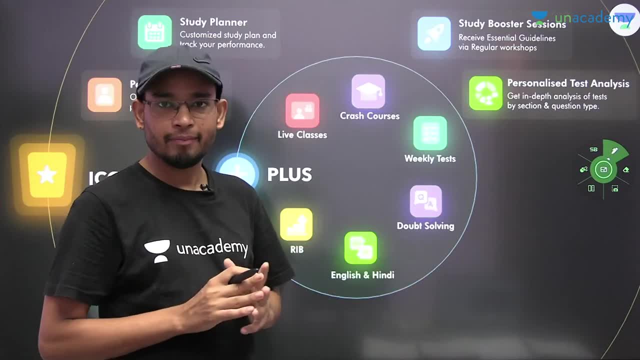 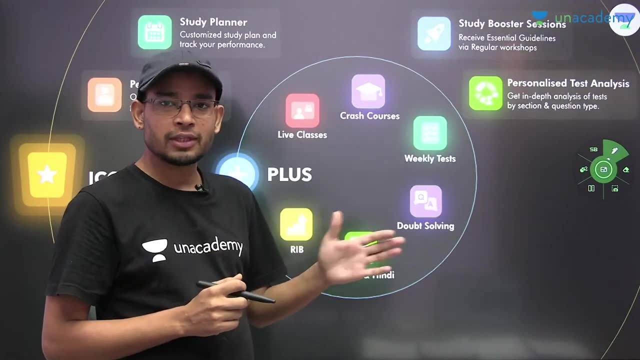 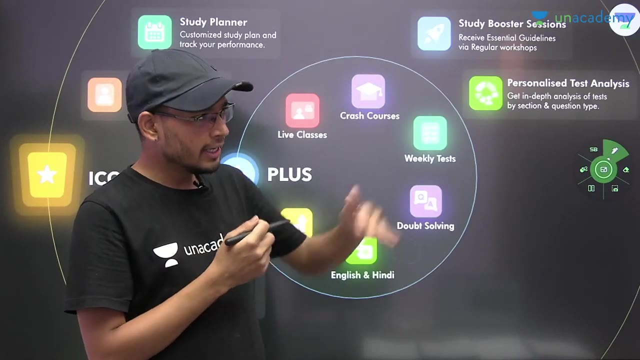 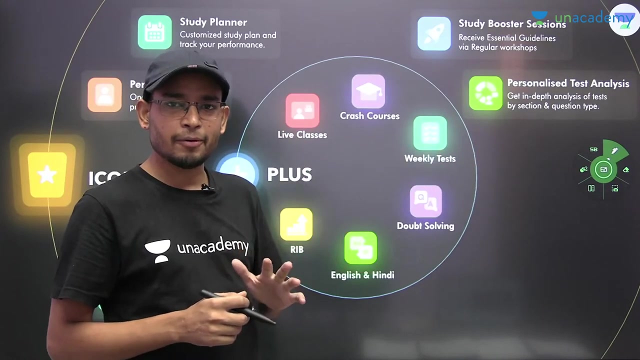 First of all, you will get things in a proper manner in which your regular classes are given, regular assignments are given. every Sunday. you have a test. this Sunday is the test of the mass transfer, as your mass transfer is going on. so you see, we organize your test on this Sunday. this will be the test on this date. this will be the subject on this date. this will be the topic on this date. doubt clearing session will be at this time. so it is predefined in a proper way. it is not that the next topic is coming. 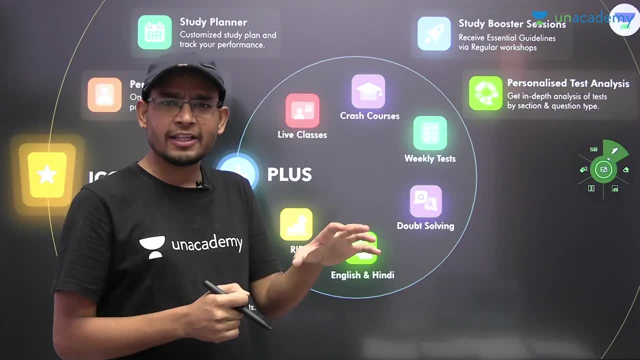 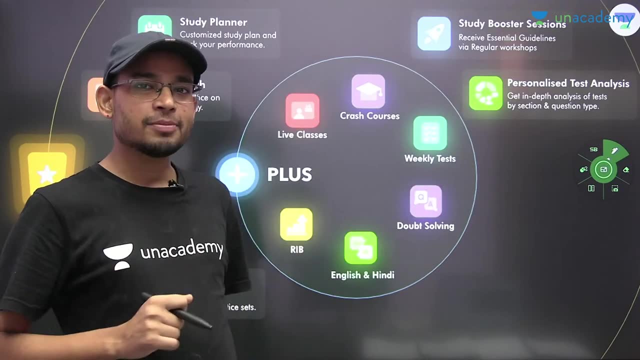 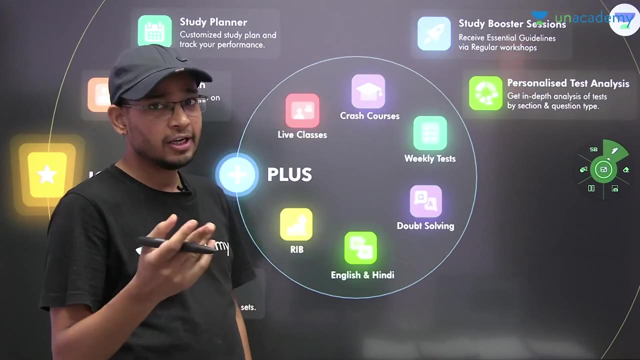 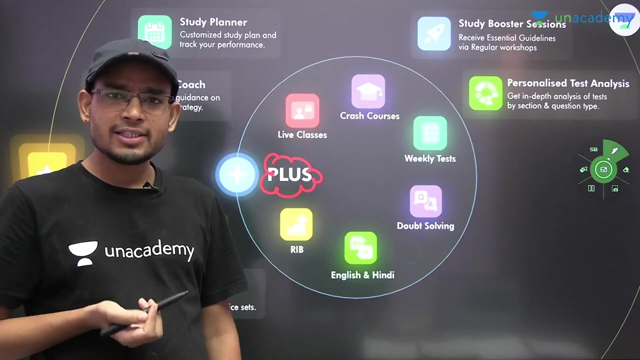 so the topic is properly defined, the timing is defined, each and everything is defined. the timing of the test paper is different. the whole session of the mass transfer. you will see I will take four to five tests in the whole mass transfer and I will take it separately. those who will sit down and do their preparation in the way of exam. you will get a test in that way. so there are many advantages of plus which I have told you. so you should not have any doubt that in case you have to start the journey in a proper way, seriously, then move with plus. 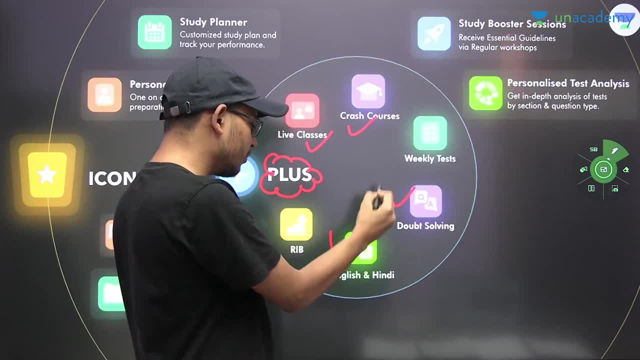 okay, at this time there are lots of live classes doing tracks, test weekly, you will get out-solving sessions and now our team is providing you with Hindi in Hindi, and just I will talk about Iconic. yes, iconic, in case. 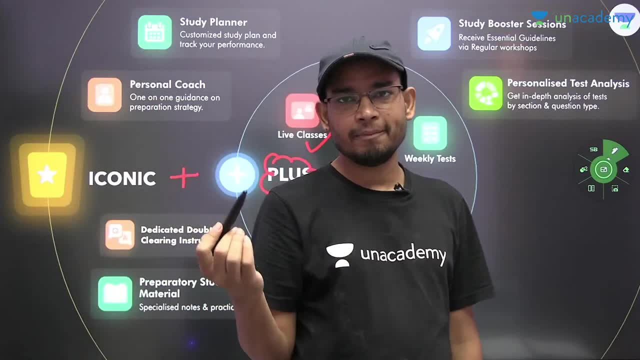 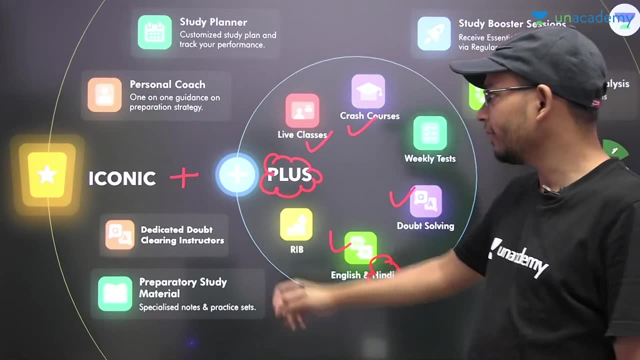 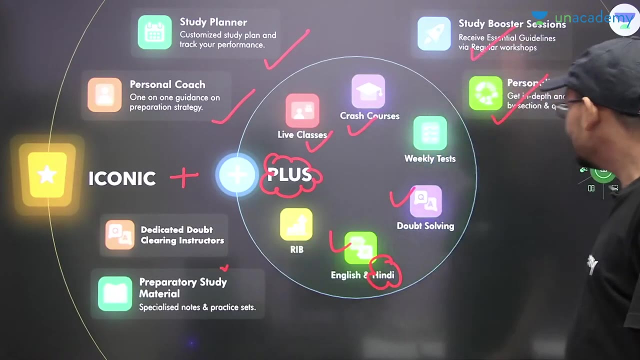 you are able to afford. the cost is a bit high. you think that there is no problem? I can use iconic. If there is a matter of study, we will not compromise in any way. so here you will get personal coach and study plan, study booster session and personal test, and here you will also get material. okay, let's talk after this. after this Moza, you are going ACTABAT. yes, then after that. trabal Kunjar is also related. ok, Udh �cyl cá idea کی. 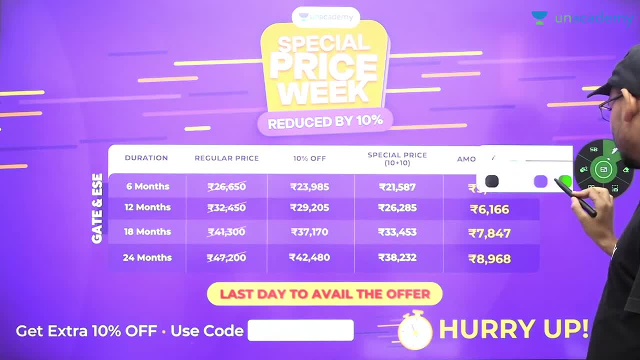 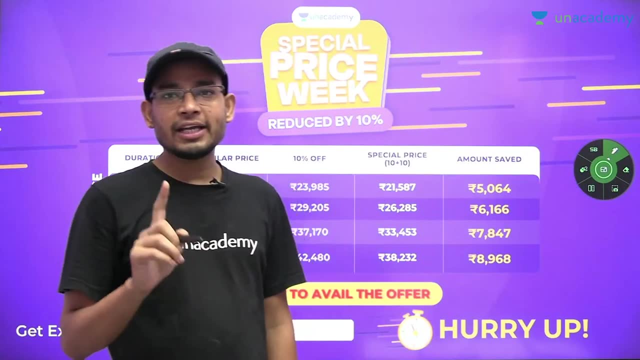 Now I will tell you that now this offer is coming, all of them can take advantage of it. So those who are especially third year, second year students or final year students, they think that the thing is not being made from YouTube. I need to take plus. 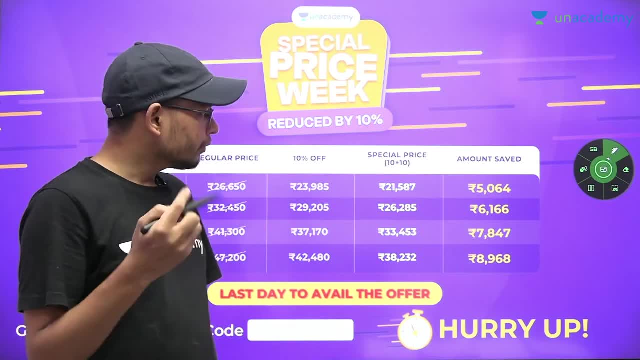 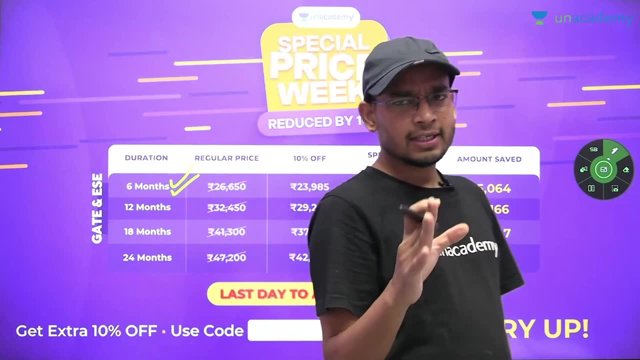 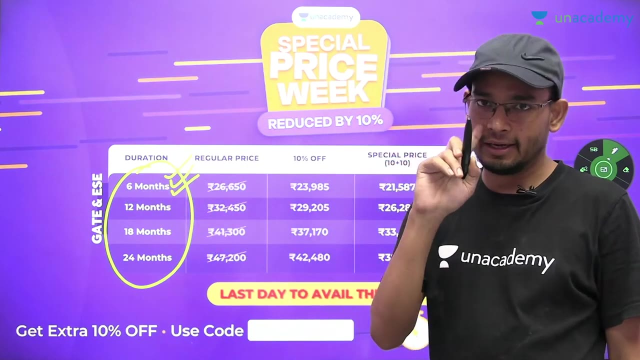 we will do investment once you will get the return of it live. so you think that you will get the benefit by joining plus once. then you can definitely join. Yes, what are the chances of the offer you have here? see, till now it was not included for 6 months. now it has been included for 6 months. 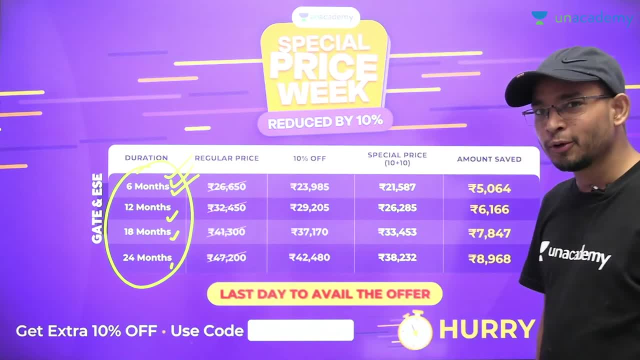 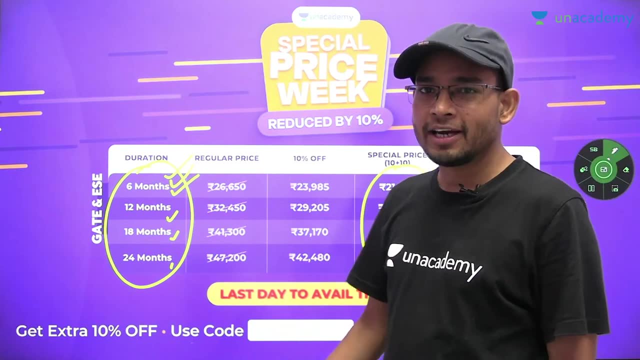 12 months, 18 months, 24 months, and I will tell you literally, I will give you an honest review. so the fees you are getting now, the offline matter will go on. so see, in offline, you will get the fees three times. 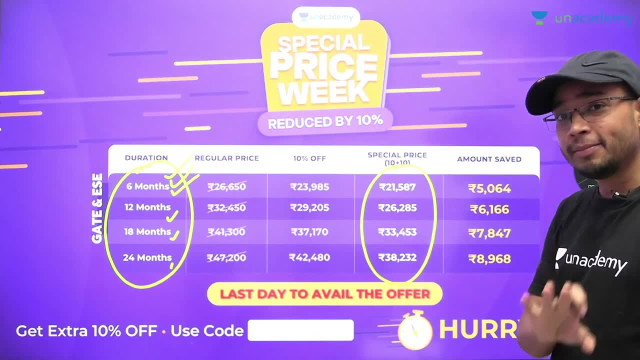 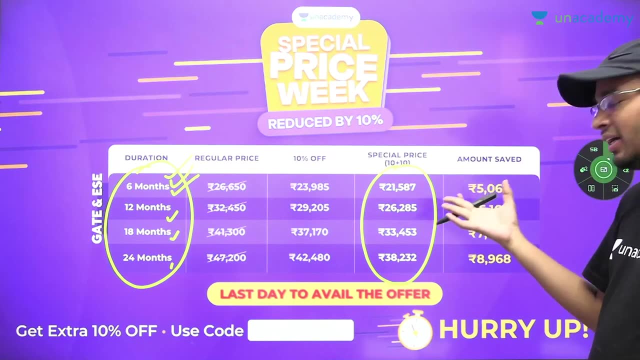 Okay, offline, offline, and you will also give it by going to ask your seniors when the offline matter was going on, then online Unacademy, which is providing you with the things. it is in a very reasonable price. Okay, I will tell you. 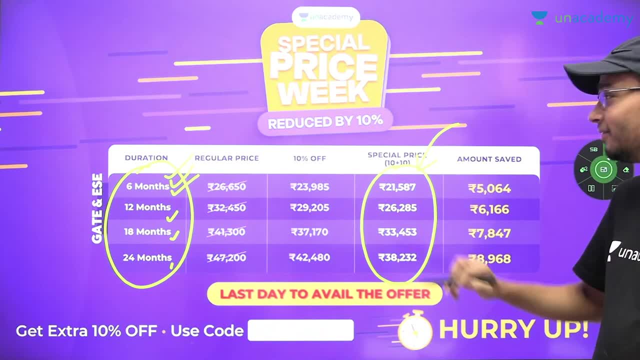 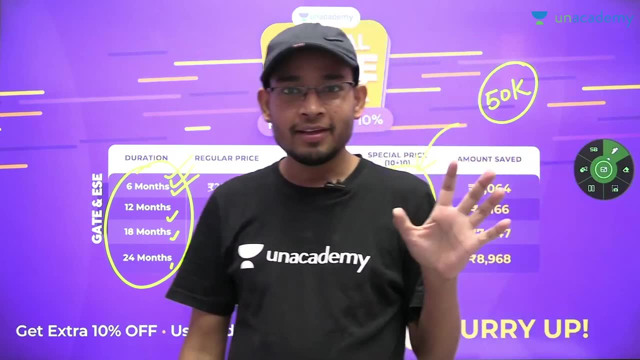 if you stay outside, the cost of the hostel will come to Rs 50,000 per year. Okay, for 50,. you will only get the cost of staying in the hostel. the fees of the institute will be different. Okay, if you have done the preparation of BTech. 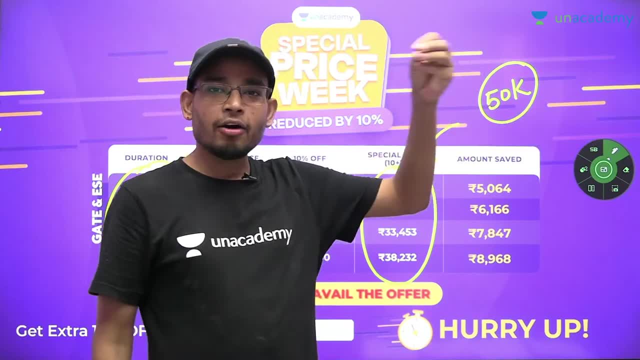 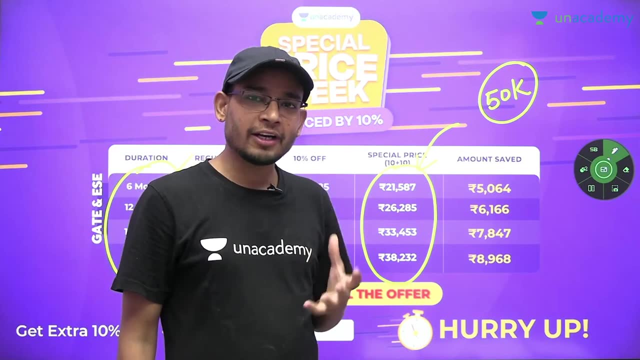 then the cost of living in it will come, and the cost of living will come, and that too, the body will lose weight in it. Okay, our age is young, we are also young, you are also young, so there is no difference. 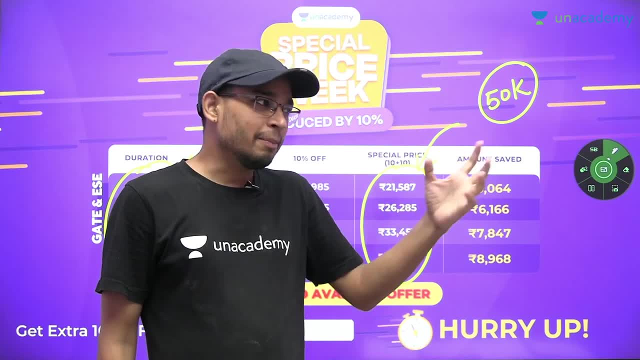 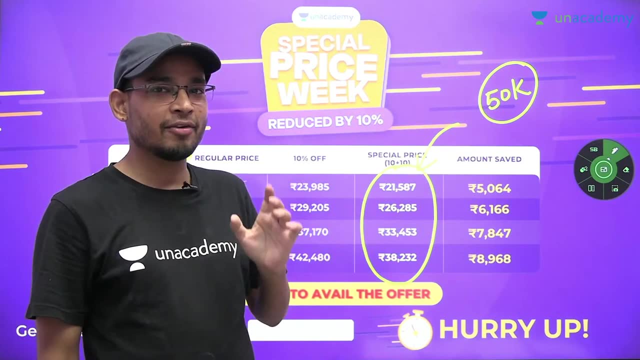 because whatever food you get, sometimes you are working with samosas, sometimes you have eaten food once, then also the work is going on. Okay, so it is different. ask the people who live outside. the biggest problem comes to eat, because I have been living outside for 11-12 years. 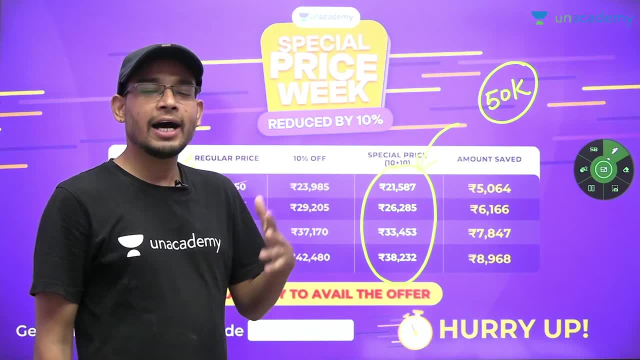 okay, I have removed the whole student life outside. okay, stayed in the hostel for a few days after going to IIT. yes, I got some good food, there is no doubt in that. but before going to IIT, I have done a lot of work. 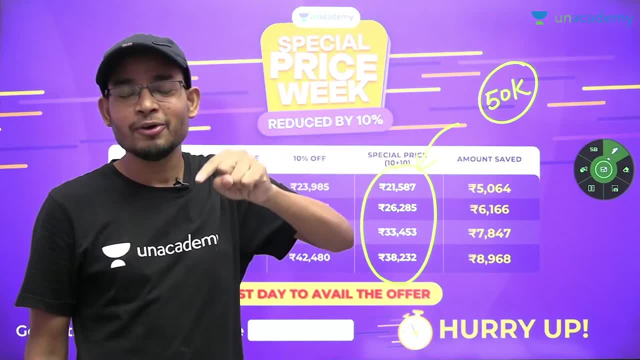 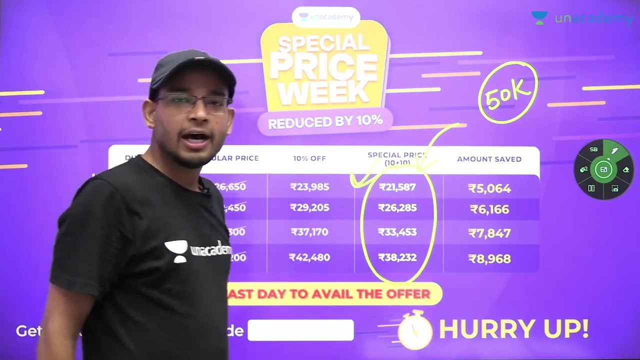 okay. so the biggest problem comes to eat. so let me tell you, sit at home and study. if you have a bus course, then invest this much. this much investment can be done properly. you will get a cost of around 21,000,. 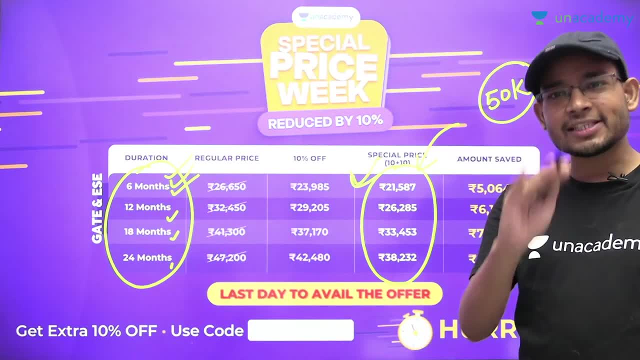 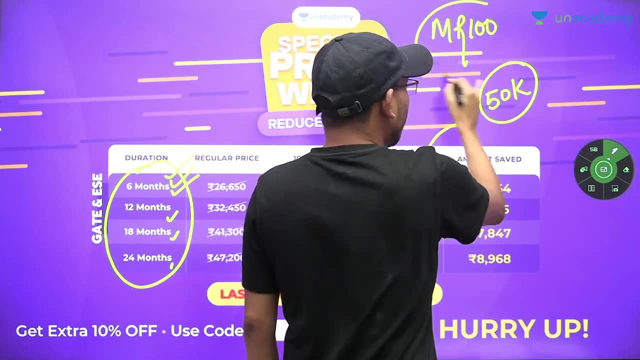 you can move properly with 6 months. you think that you have to work with us, okay. so you remember the code MR100, from here, you will get the current discount. you will get 10% from here. okay, along with this. 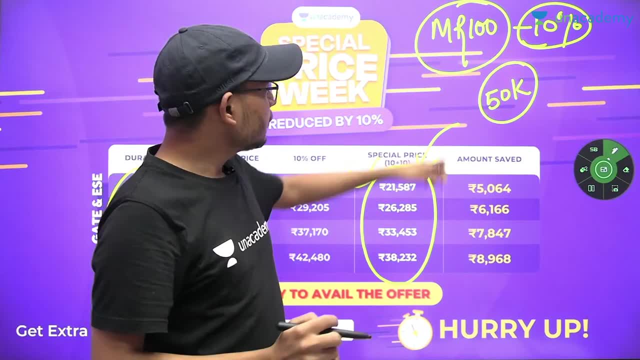 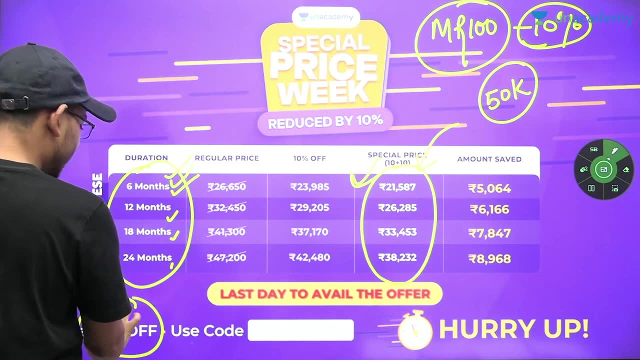 the personal bonding and relationship will be of a different level. so you can move from here with this code, okay, and yes, you will get 10% more off. okay, we will use the extra code of Unacademy and this Unacademy of 10% is providing you. 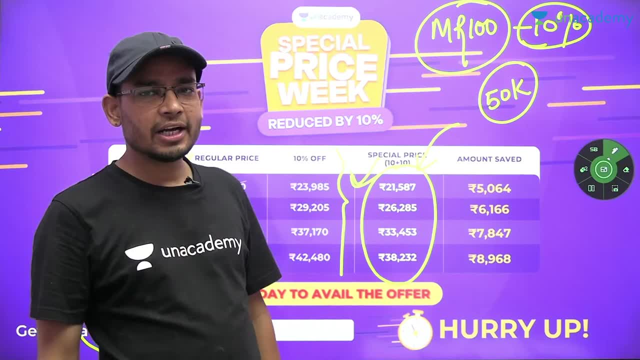 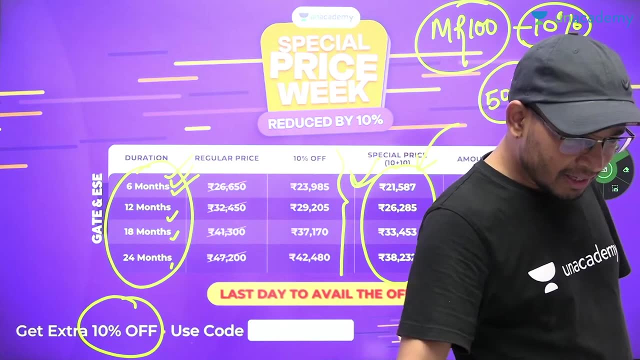 okay. so you will see, you will get a 10% discount in this, so it means that it is at a reasonable price so you can start the journey properly. there is no problem, sir. I have been outside and seen. 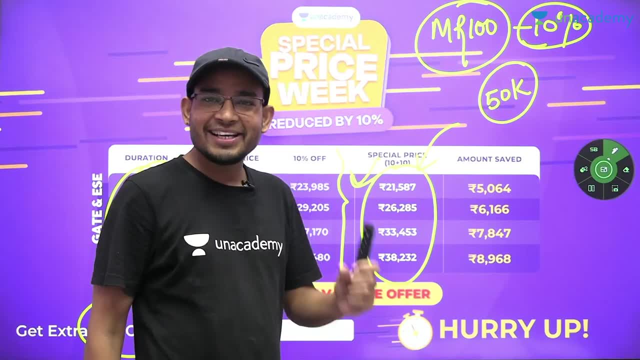 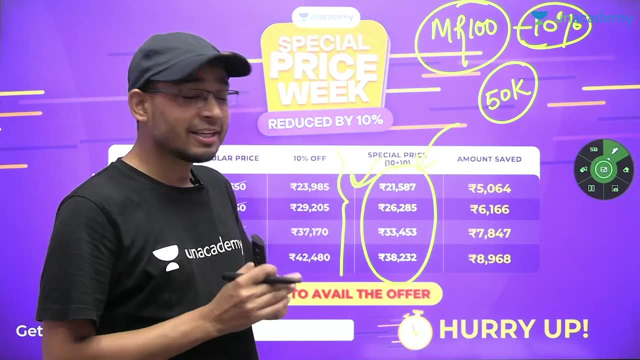 yes, Jay Prakash has been outside means he has eaten chickpeas from every street. okay, so Jay Prakash has an idea. so those who have seen it outside ask them how much problem there is means things. the biggest problem is food. 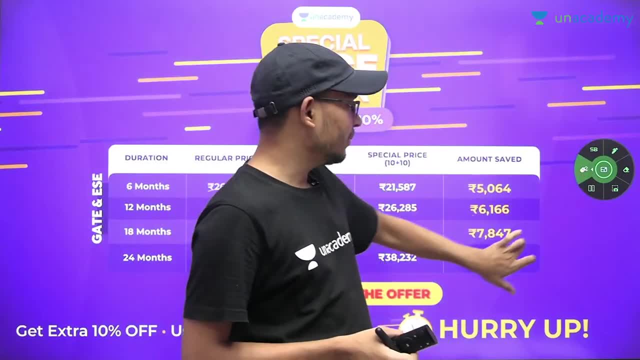 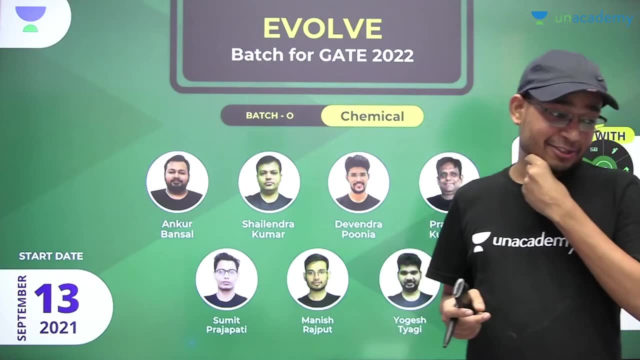 everything else is fine. everything else is fine. food is not good. no matter how good the place is, it cannot be maintained. yes, those who are living outside ask them how much is spent in a year. so at this time you can take its benefit. 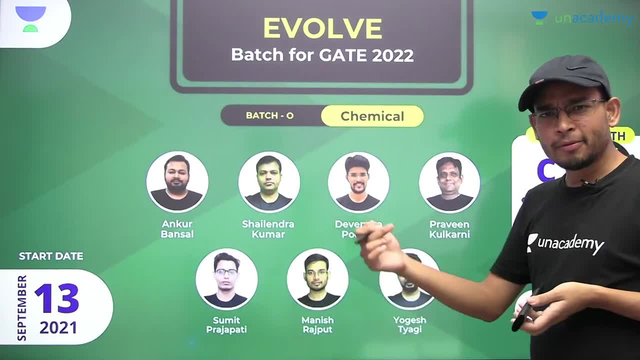 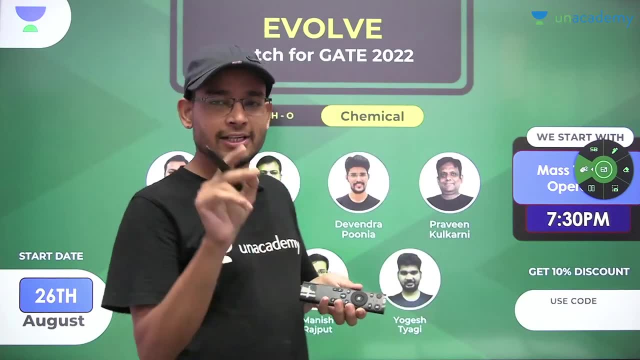 see, this chemical reaction engineering silencer has just started, so you can move with it properly. and after this, another subject is going on, that is the mass transfer operation from tomorrow. the distillation has started. okay, your distillation has started from tomorrow. 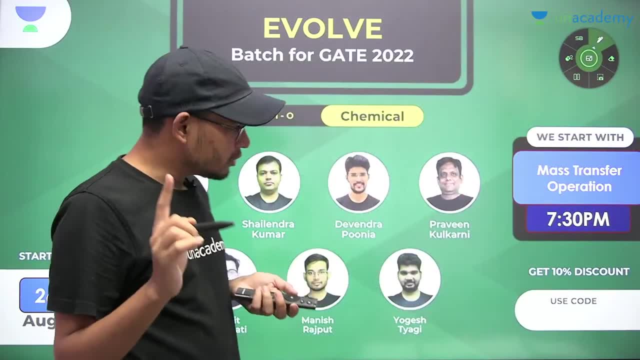 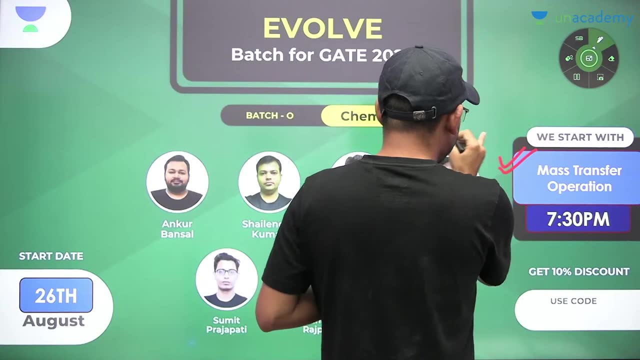 right, your distillation has started from tomorrow. so those who have to move with distillation and mass transfer and with us: okay, so you can definitely go with mass transfer. your distillation has started from tomorrow. okay, yesterday I covered your very basic part. 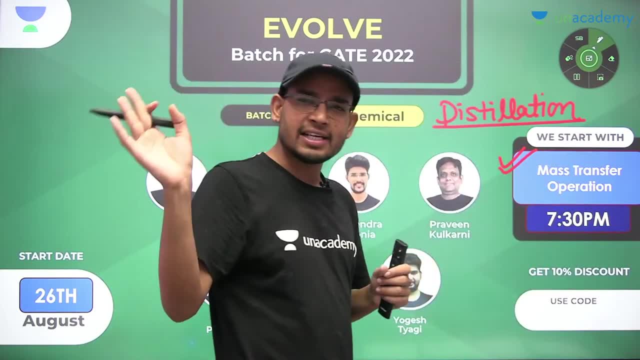 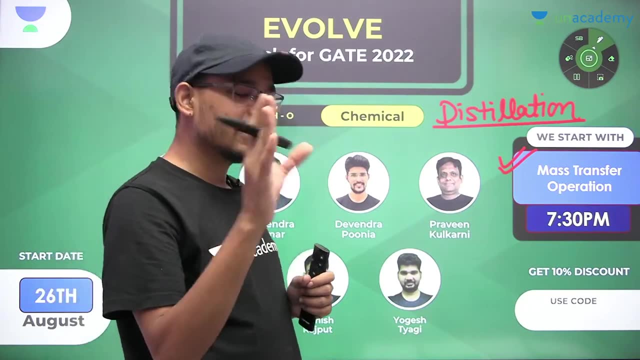 how distillation is done in refinery. okay, what is sensible heat? what is latent heat? we discussed this very well. okay, very latent heat, although this was not a small part in YouTube, okay. so these things, I went there. 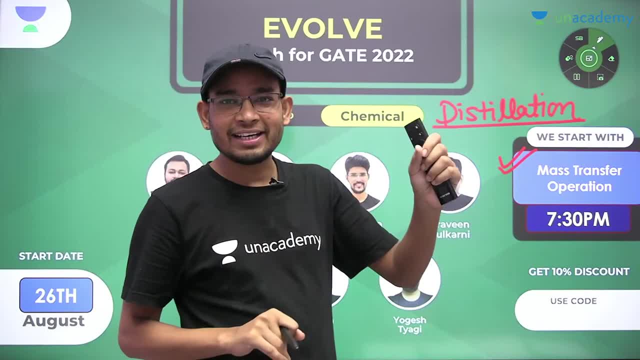 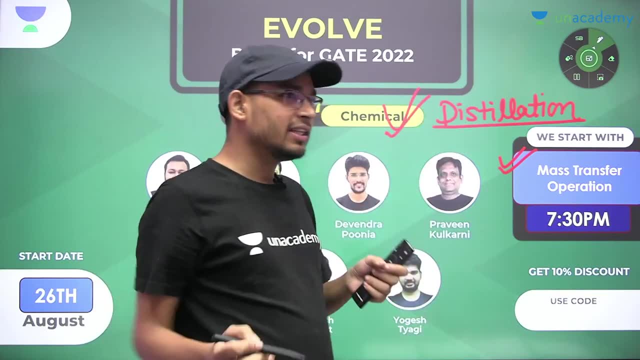 there was so much discussion that whenever the children were saying that this is latent heat and the sensible heat will never be forgotten in life. okay, so this was your session yesterday, so we talked about this very basic term. we talked a little about your refinery. 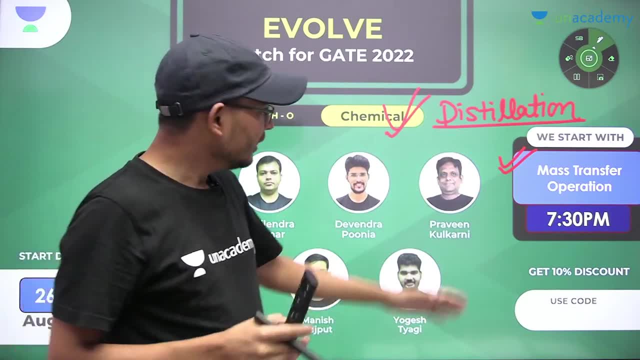 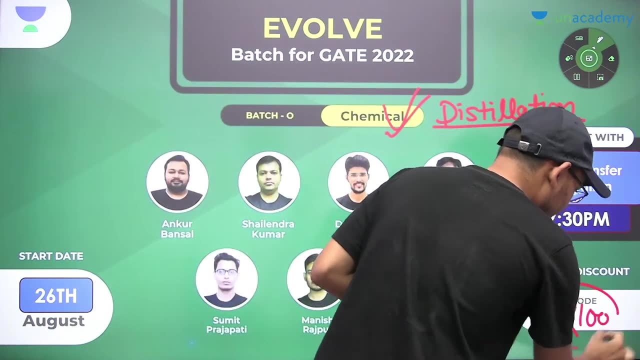 how to use distillation in refinery. we talked about all that, so you have to see once. in case there is a friend, then you can see from him. if you want to take, then you can take. you can use my code MR100,. 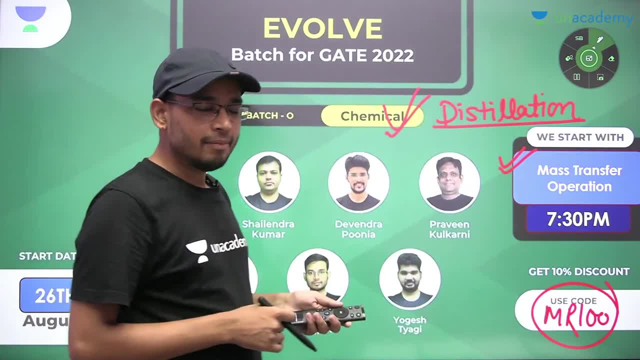 right, distillation is going on. now it will work, because it is a big topic. okay, so I will teach you this properly. okay, so this will work. now your 8 to 10 lectures will work at least, come on. 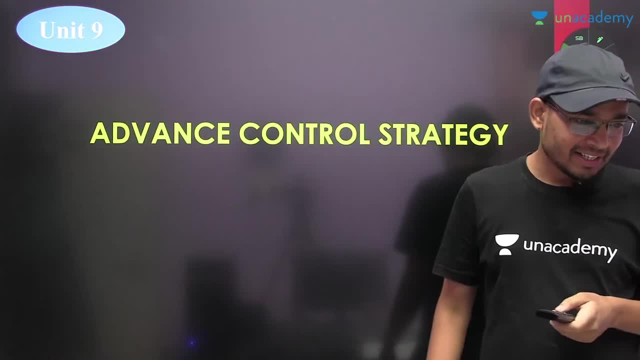 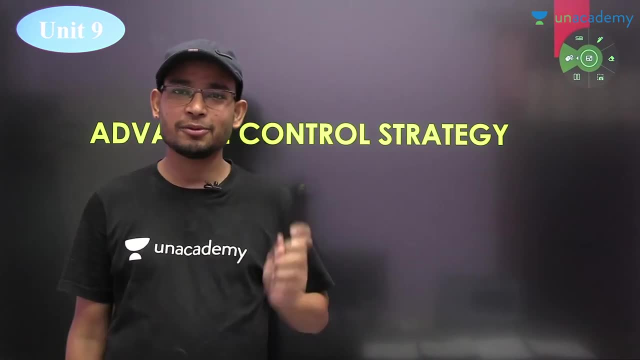 let's talk about the advanced control strategy further, sir. good food is available in the hostel of IIT. all this is from far away. yes, if you go to IIT, then understand that when you reach there, a different world will start. 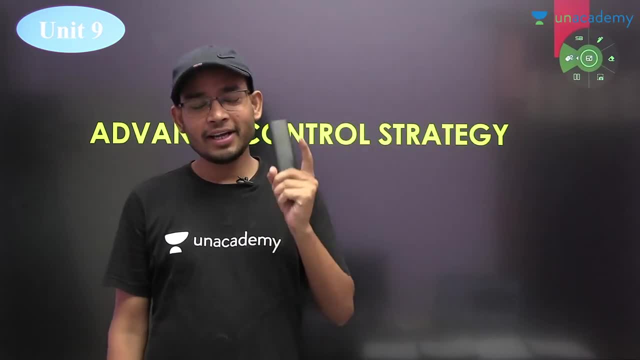 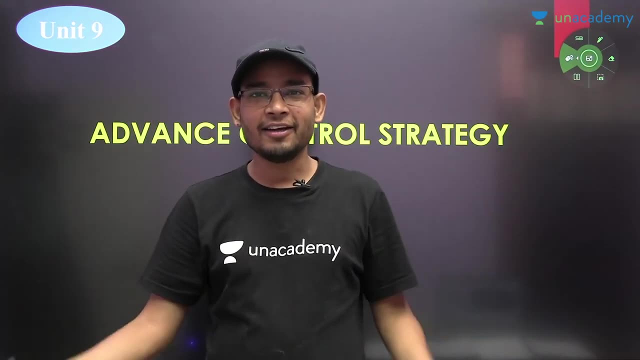 as you come out of IIT, you will see a different world. okay, yes, you will feel this only by staying inside IIT. if you stay inside IIT, then you will feel that, brother, what is life okay? 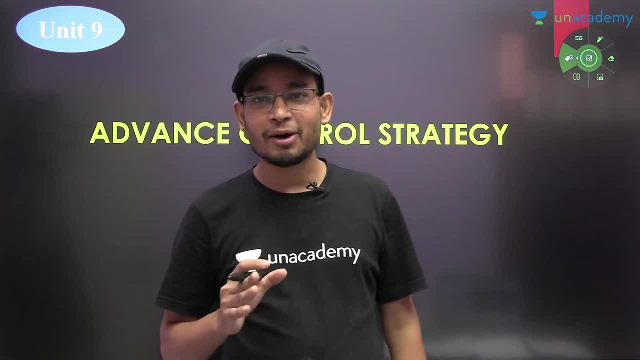 all the intellectual people. good, okay, the one who will be the master. he must be talking in English, yes, and your guard must also know English. so, and the student and the faculty, you will go. you will go to the department. 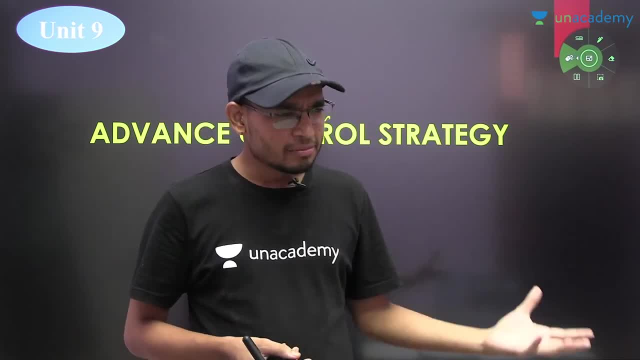 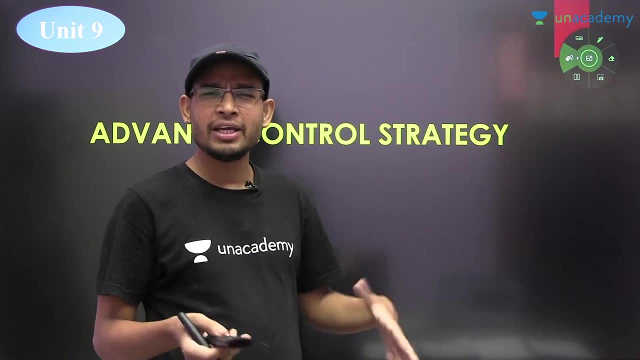 suddenly a different world comes out. okay, suddenly people will be going cycle. this cycle is used in IIT. okay, you will see, you will also buy a cycle. there is no bike in the whole environment. there is no noise. 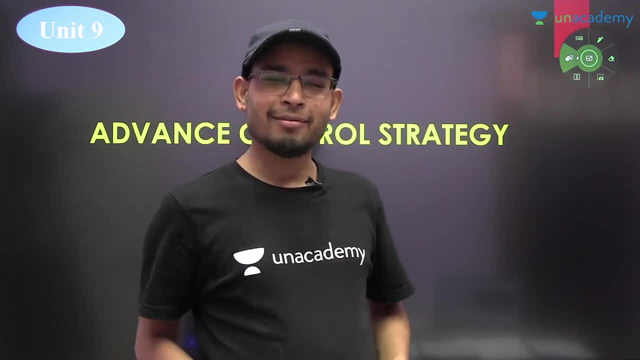 there is no noise. everyone is a professor. they are also coming from the cycle, our professor. he is coming with his daughter. he used to come with his cycle. one day we asked, we said, sir, from the cycle today. 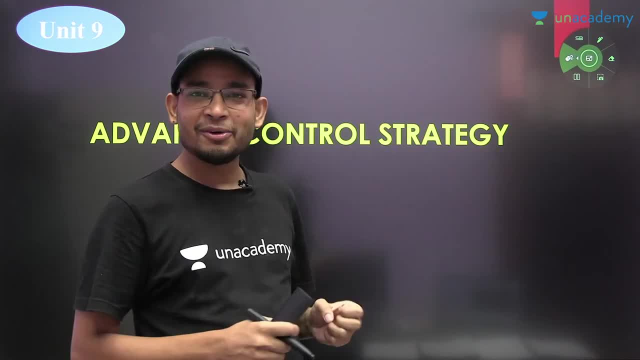 he said: actually, my daughter is going to journey, okay, so the cycle was kept at home. so I am just thinking about something. joking will also happen, and all this will happen. so we came to know there is a basket. 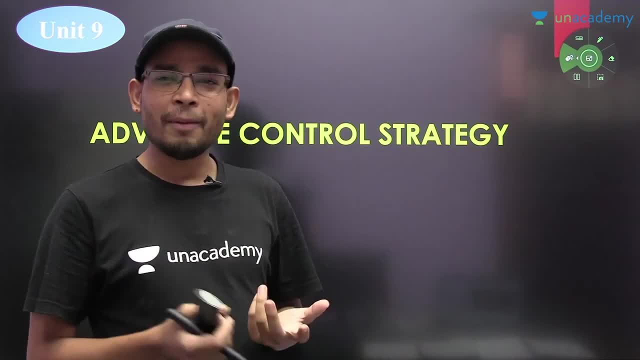 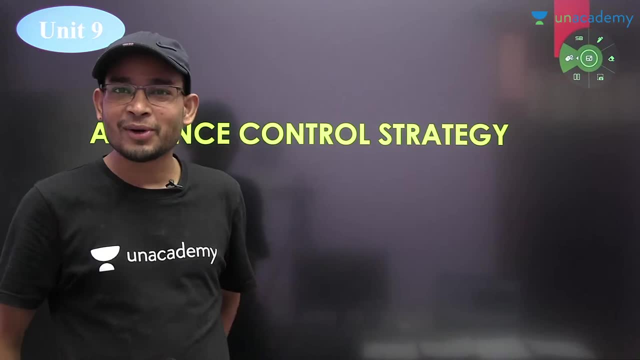 in which flowers etc are kept. they are coming with that cycle. so there is no difference there up and down, and in our college, in the BTech college brother, there should be a bike. okay, there should be a rank. 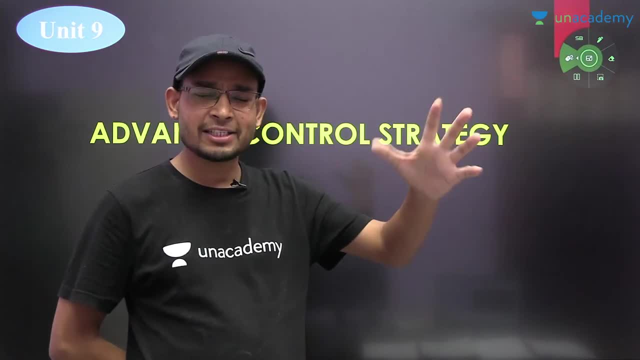 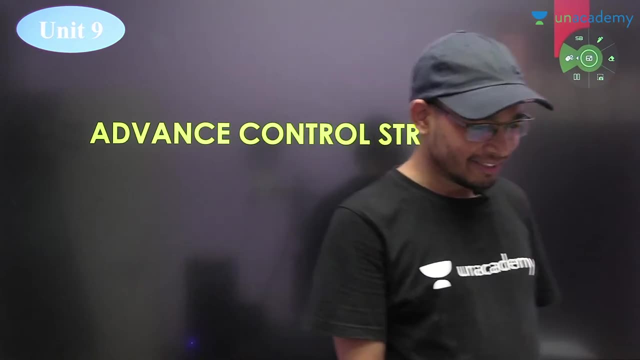 okay. so in our BTech college, in the state-wide college, who has a bike? understand that it is cool. its environment is different, so those things happen. so just these things you will get to see in IIT. 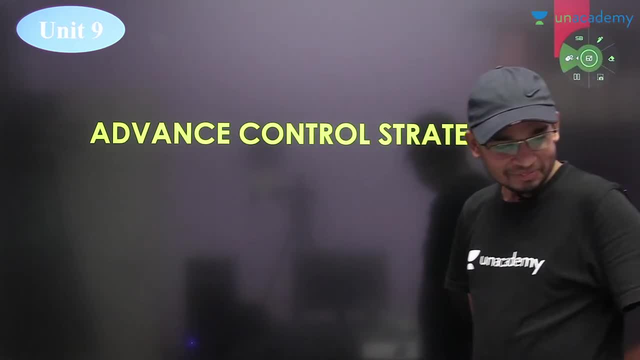 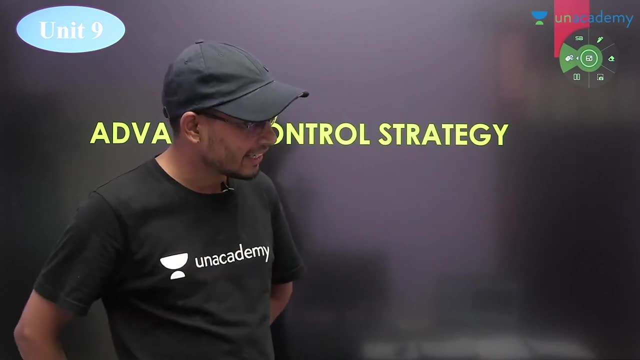 you will get to see there. yes, in your state college, in our state college. when it was there then it was found that there is no bike. you went by cycle. people are looking at you. hey, Manish, have you come by cycle? 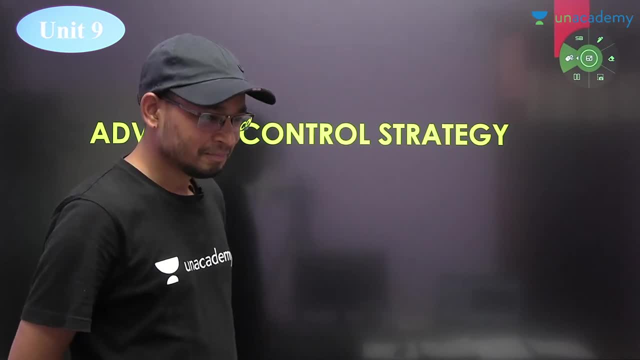 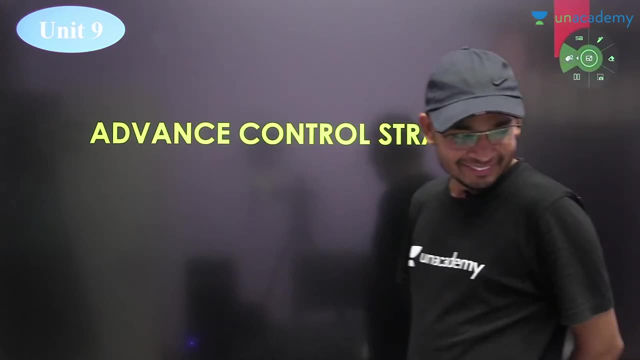 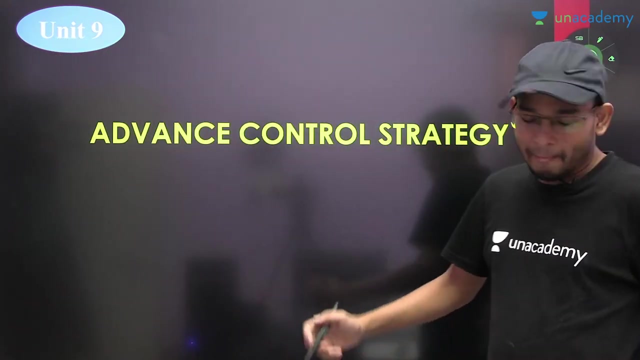 okay, and in IIT, if you will go by cycle, then you have more respect. if you will go by cycle in IIT, then you have more respect. yes, okay, then let me just start this session from here. I will talk about advanced control strategy. 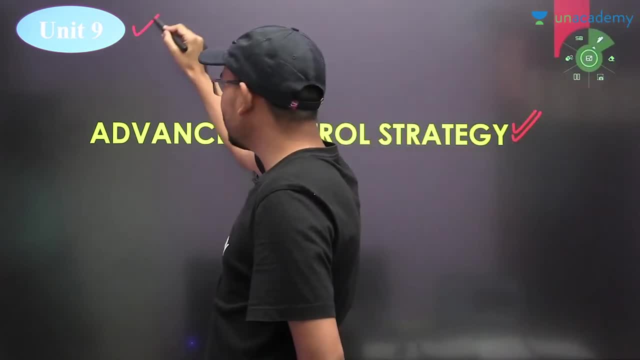 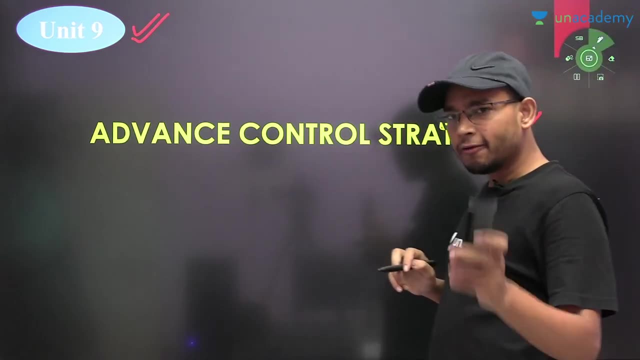 which will be your unit number 9, right unit number 9 will be Advanced control strategy. okay, we will talk about the advanced control strategy. there will be 2 strategies in it. one is feedforward and second you will read. 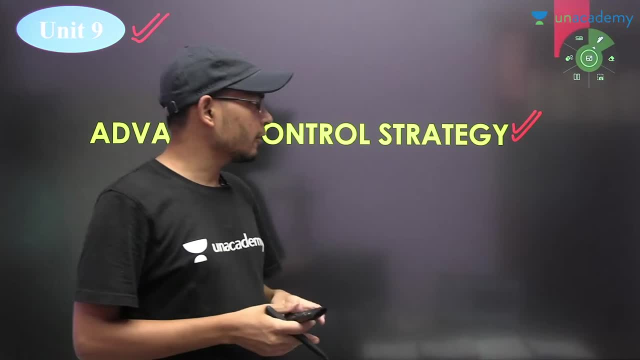 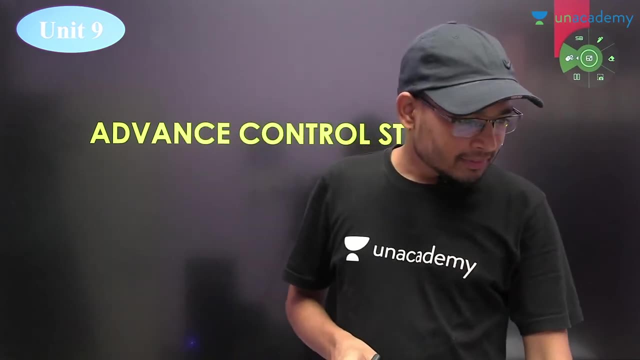 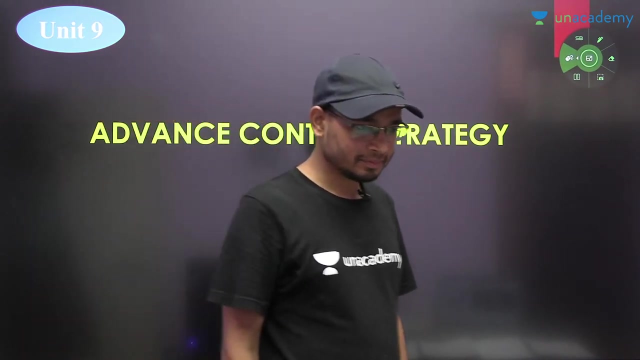 cascading. okay, then we will start with feedforward. Let's start with feet forward Once everyone will tell that they are ready to start. Are you ready? Let's start. Yes, Let's start, brother. Let's start beautifully. yes, everyone is ready. 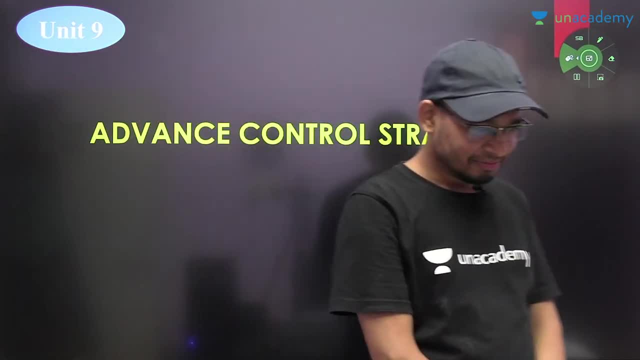 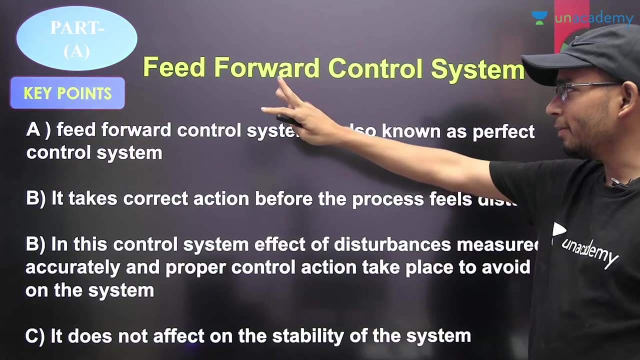 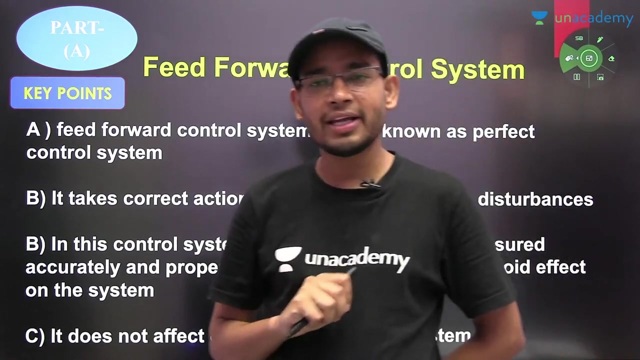 Let's start. Ready, Very good, Let's start. Let's start. We will read the first advanced control, part number A. In part number A we will read Feet forward control system. We will read another strategy- Advanced control strategy- We will do that later- In which we will talk about cascading. 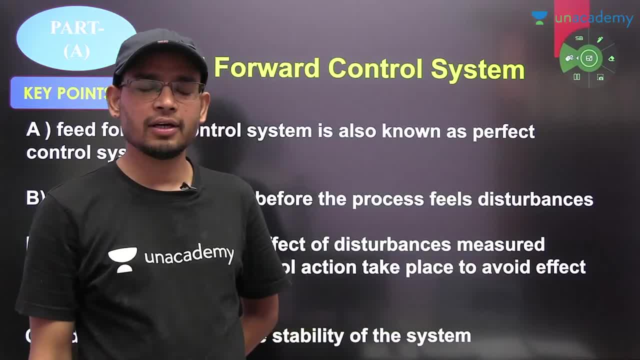 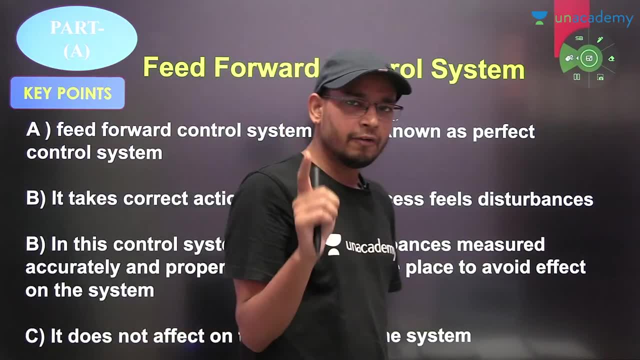 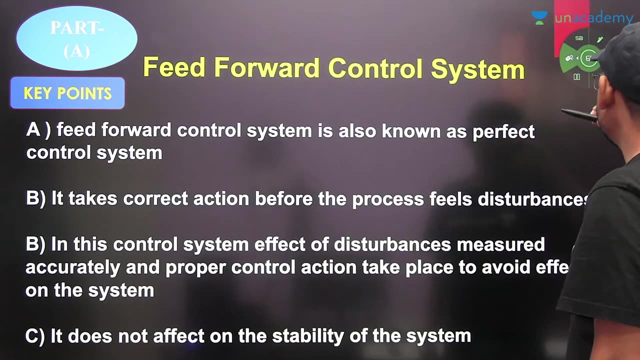 Multiple cascades, How you can handle and control it. We will talk about it tomorrow. This time there was a question, So first of all, we will add Part A- Feet forward control system, Part A- Feed forward control system. Everyone will add heading Feed forward control system. Feed forward control system. 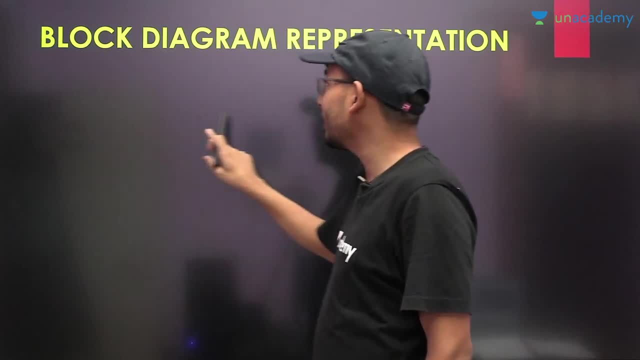 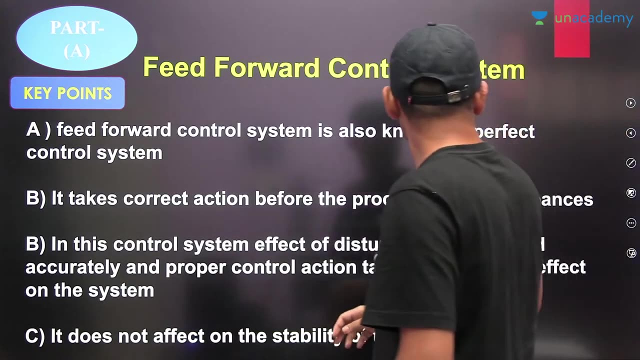 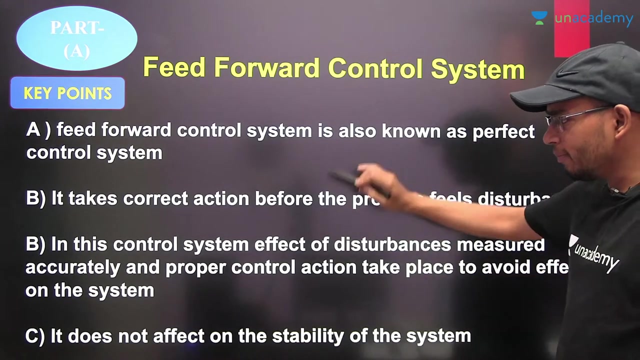 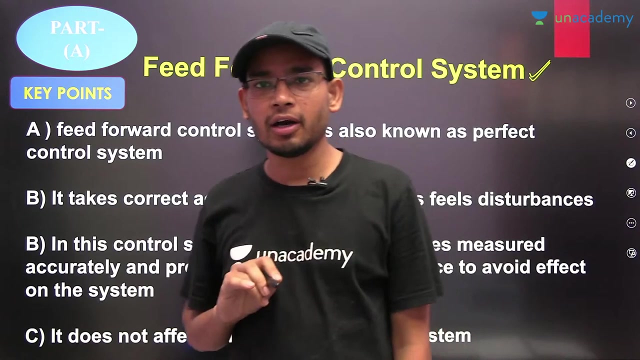 Before adding heading, I have brought key Points First. all will write their pin point And try to understand What is key Point. Everyone will understand What is key Point. 首 était, The key point is very important. why do we use it? This feed forward control system is also called a perfect controller. 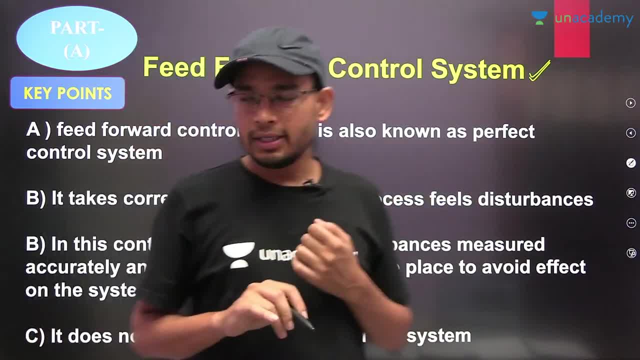 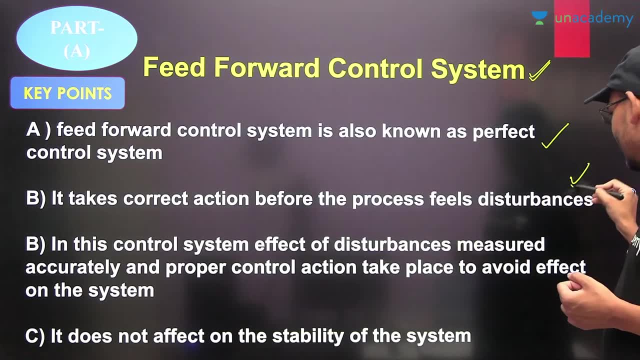 What is called a perfect controller? Why is it called a perfect controller? Understand the reason behind it. why is it called? Because this is feed forward this action of yours. first disturbance: the system could not feel the disturbance before that. it will take action. 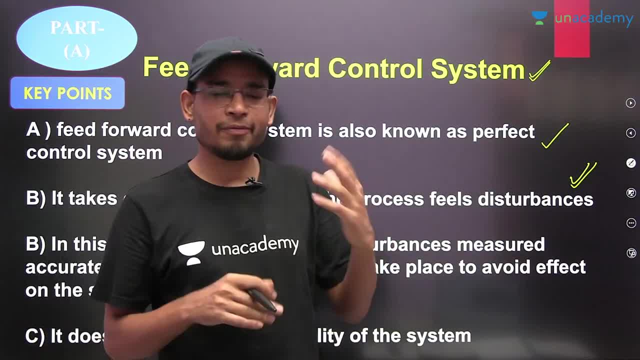 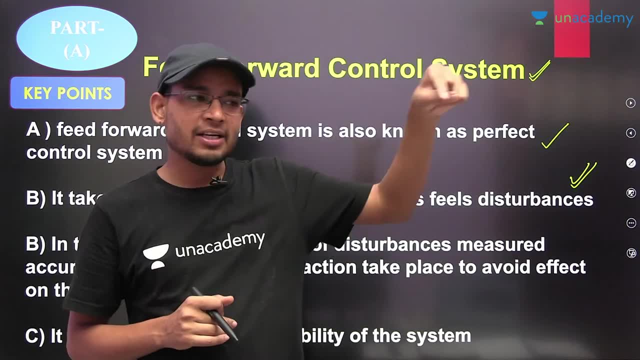 It will not happen that the disturbance first happens in your system. what used to happen in feedback? what you were reading till now, it was all feedback closed loop system. all of them were feedback means disturbance used to happen. then you used to check it that so much disturbance happened. 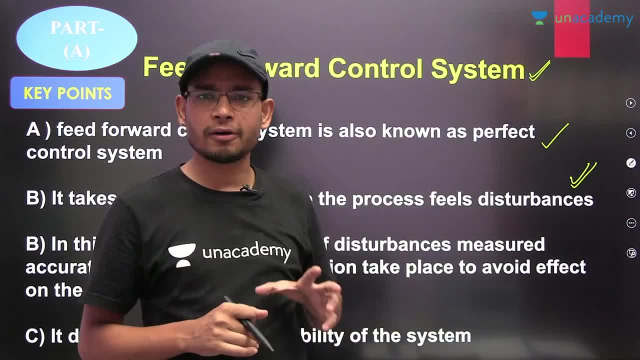 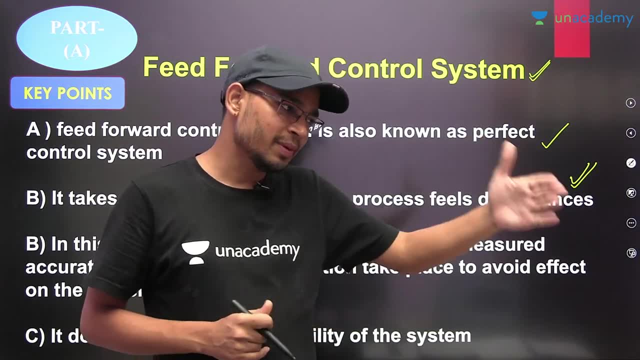 then you used to go and install the controller. then you used to control it easily. But it is not like this here. you will keep all the manipulation already. you will feel that this problem can happen in this process. then you will keep the manual ready from the beginning. 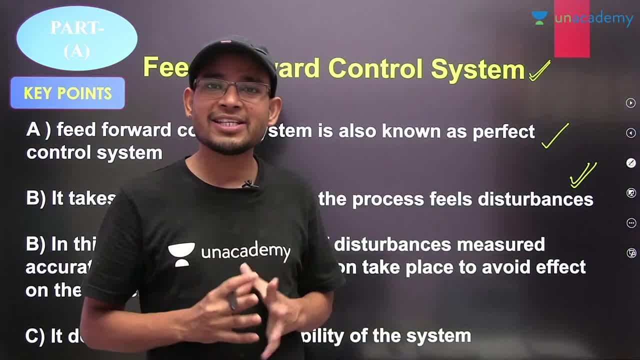 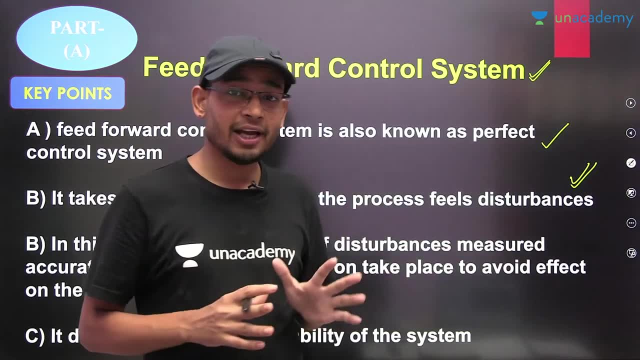 there is a little problem in making a manual in this. ok, Then you have to work well on the manual and paper. its designing has to be kept very well ready, because then you can't do anything in the middle. whatever you have to do, do it first, ok. 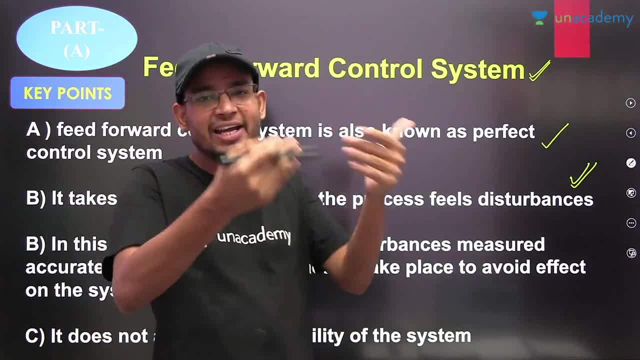 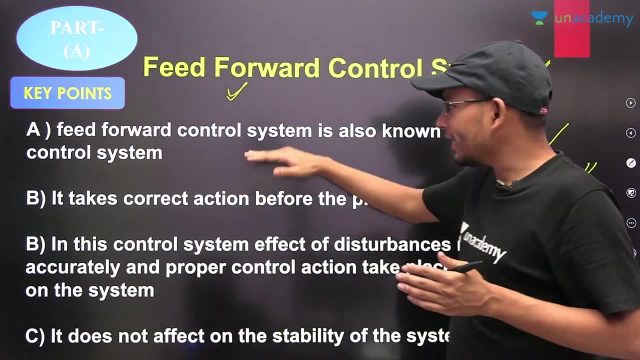 So what is in this? That what it does before the disturbance, it takes action. ok, So your feed forward controller is so amazing, yes, ok. So what does it do? Why do we call it a perfect controller? Because as soon as the system felt the disturbance, 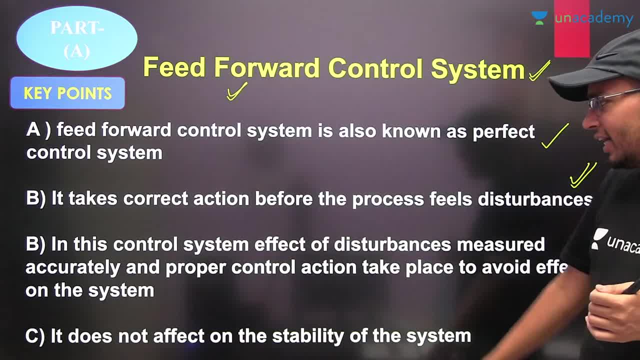 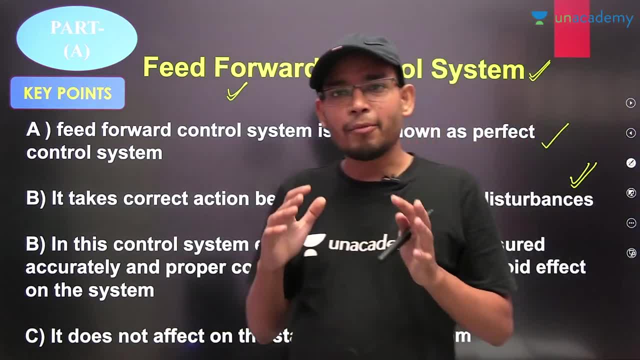 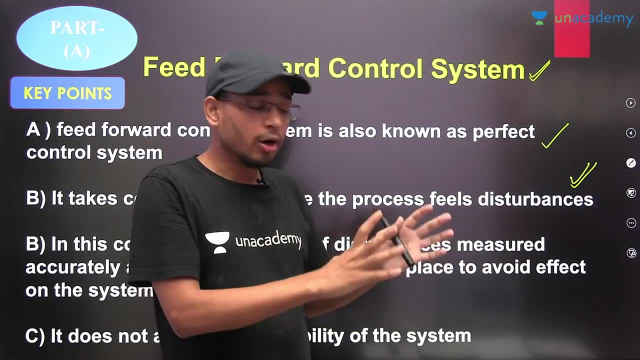 it took action and kept it ok. Second important thing in this control system: the effect of the disturbance measured accurately. what is in this? Whenever you do modeling of this, of whose feed forward, then the measurement of your disturbances should be very accurate. 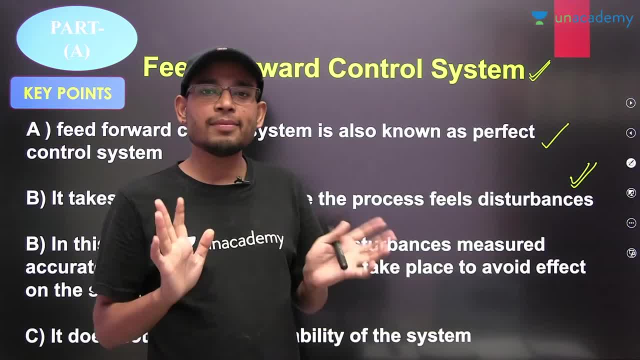 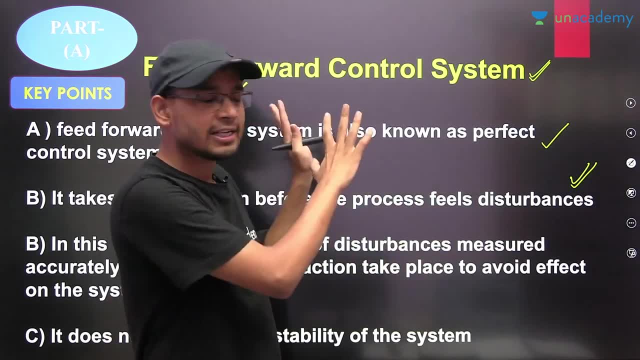 in case it is not accurate, then it will produce a lot of error. ok, You will not be able to control it later, so you have to have the knowledge of all the errors, problems and disturbances that are coming in it, in whose case in the feed forward control system. ok, 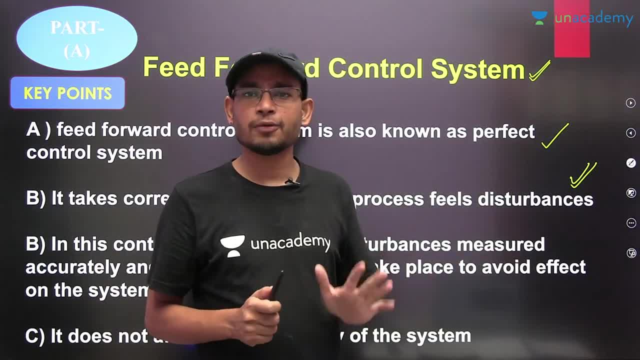 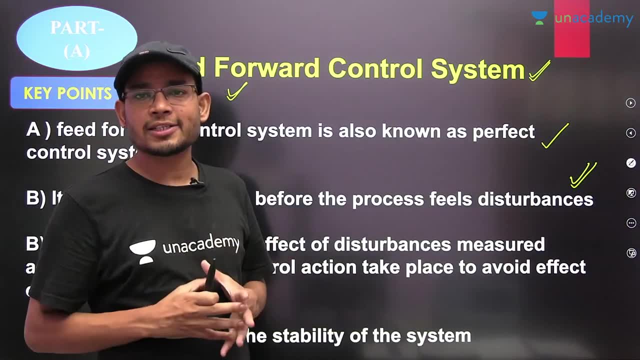 All the errors that are happening to you. it is very important for you to have pre-knowledge of all of them. ok, And what does it do? Proper control action. what should happen in this? There should be a proper control action, otherwise the system will produce an error. ok. 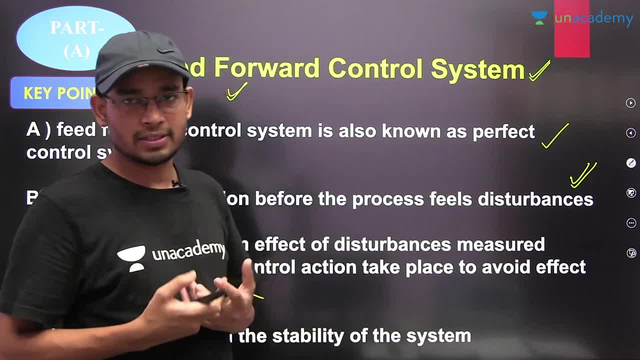 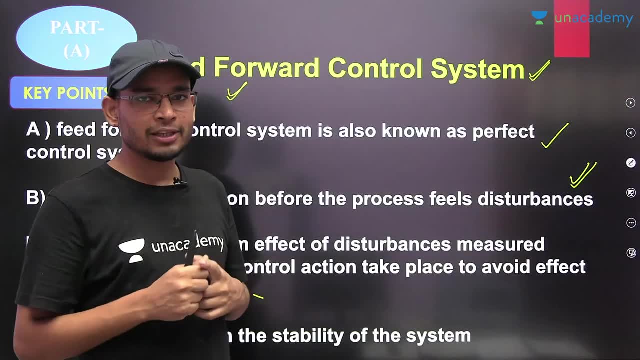 To avoid the effect of the errors or disturbances. ok, So you understood one thing: that the feed forward control system. we also call it a perfect controller. Why do we call it a perfect controller? Because what happens is this controller in case there is any disturbance. 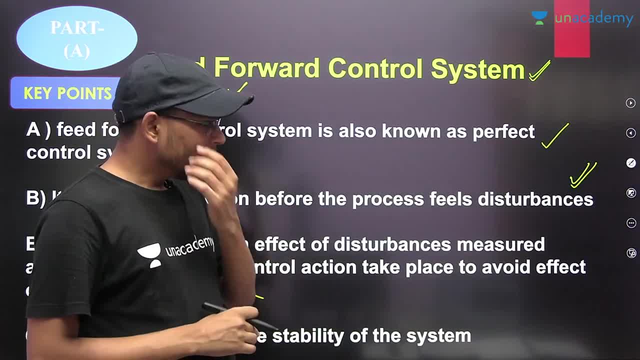 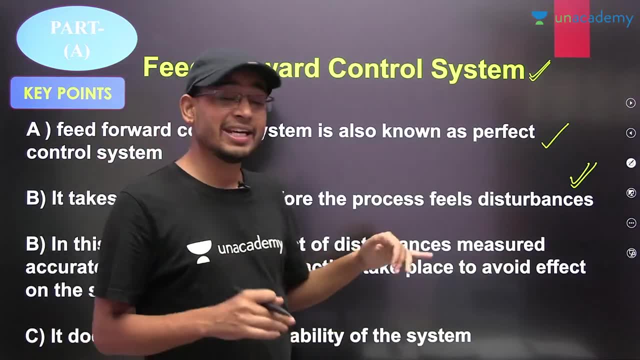 it takes action before that one. Secondly, for this there is a requirement of some things. What will be the requirement for this? That your disturbance measuring elements should be very accurate. Thirdly, your modeling should be very good. Your model should be very well prepared. 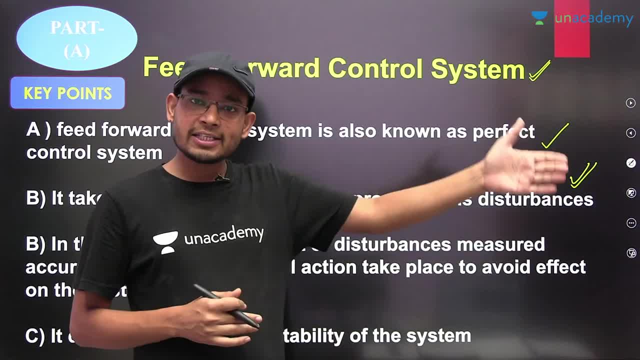 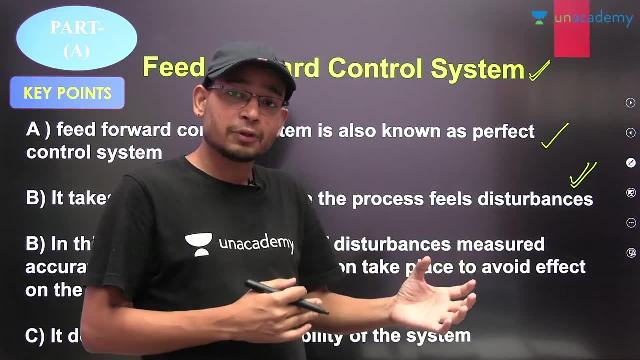 If you come to know that there is an error later, then you will not be able to control it later. This means that everything has to be done first in the feed forward. Feed forward means that you are not backward. This happens in your backward. yes. 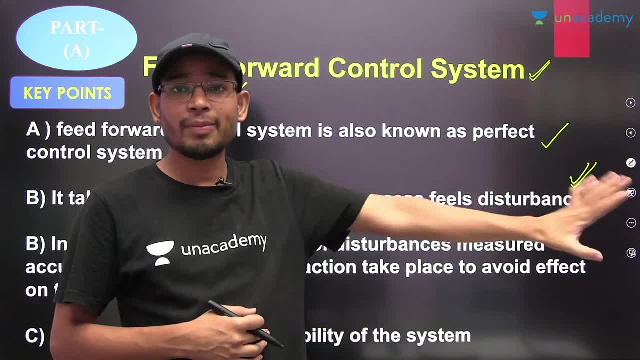 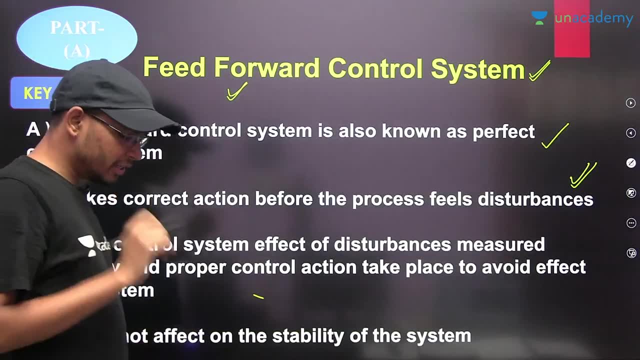 Your error came later in the backward. you will be able to manipulate it later. But in this you have to manipulate it later. In this everything is done without any manipulation. The third important thing: it does not affect on the stability of the system. 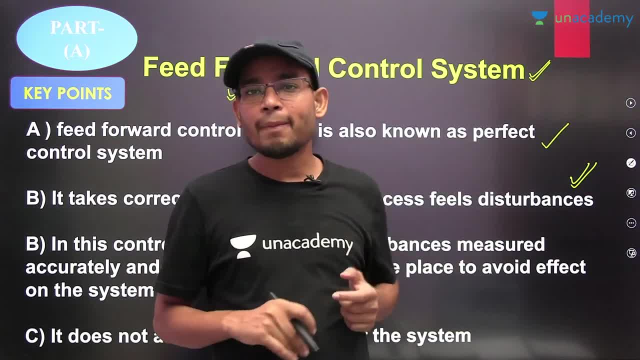 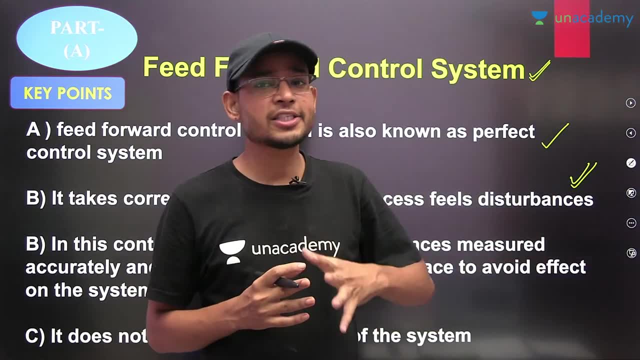 Yes, When you used to use the feed back system, then what could have happened in that? In that you will get to see that your order of the system could have increased, But your order will not increase in this. Ok, There will be no effect on its stability. 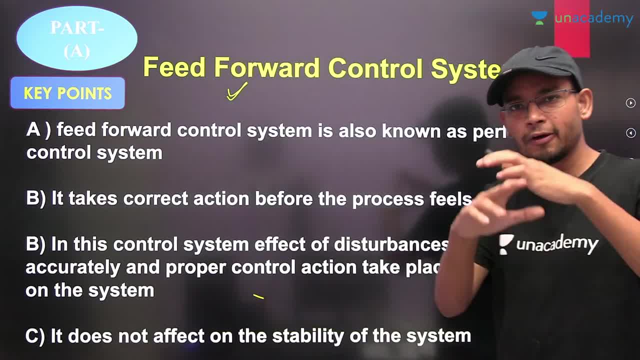 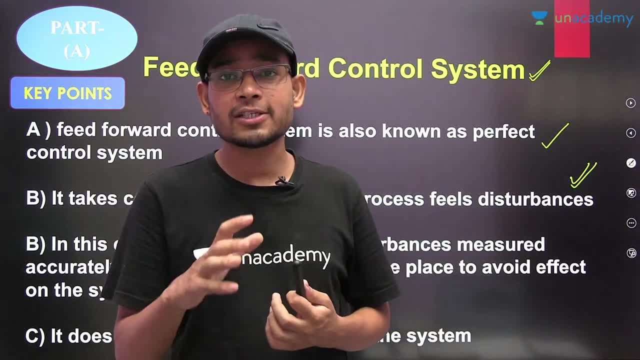 Ok, It does not affect on the stability of the system. Sometimes, when we control the feed back, then what happens is that the system becomes more sensitive. Ok, So the more the system becomes more sensitive, then what happens to your system? 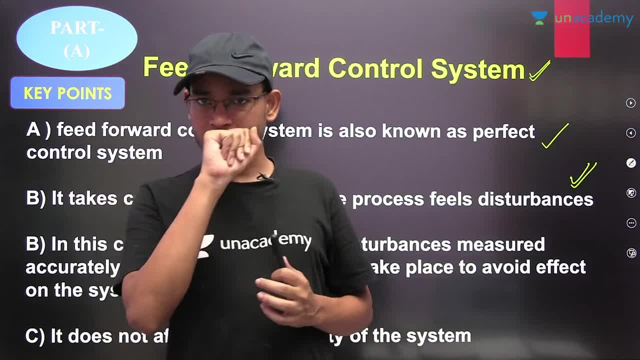 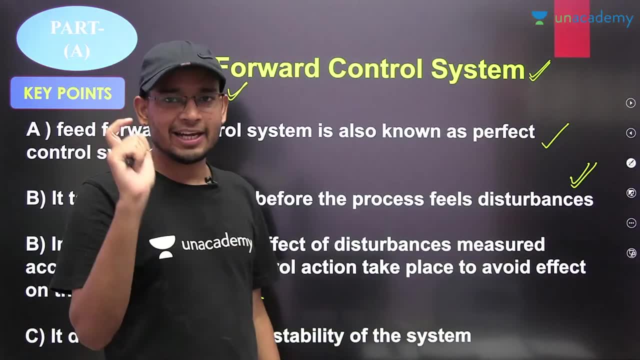 There are chances of it going to be unstable, But this is not the case in feed forward. Ok, It will always remain stable. There is no effect on its stability. But, yes, your feedback is more accurate in compared to feed forward. It is more accurate in compared to this. 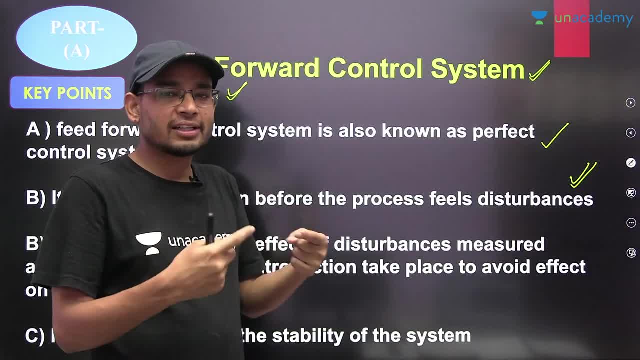 Ok, Because the error comes again and again. So what does it do? again and again, It manipulates it. But once this error comes, then it does not repeat it. Whatever error comes, you have to go with everything first. You have to go with the first term condition. 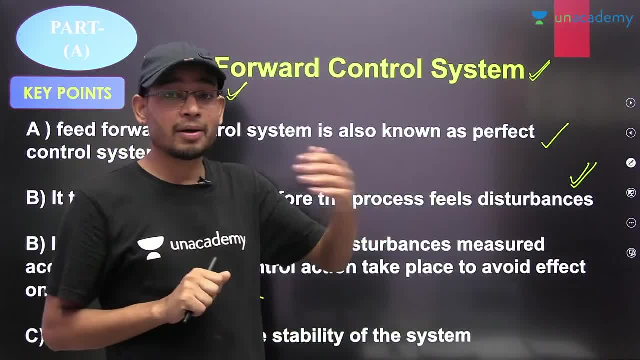 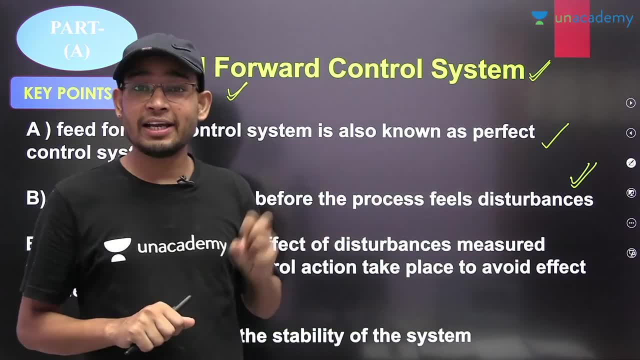 You have to go with the second term condition Here on the way. whenever you go ok with food, then you keep in mind that I will be so hungry by evening, so I will go with this much food. Ok, Yes. 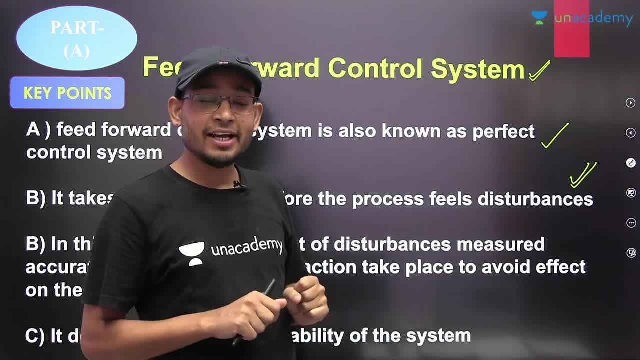 And what is the feedback? Yes, if I will be hungry, then it will buy in between, Ok. So what will it do to the system? It will make it stable, But feed forward is not like this. It will take everything from the beginning. 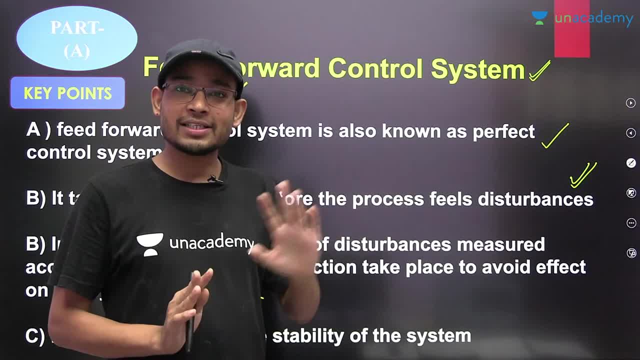 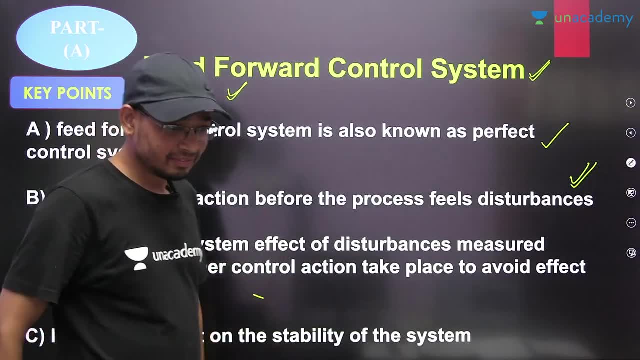 It will make arrangements That. yes, brother, if this happened, then we will do this. Ok, But yes, if something happened later, then it will not be able to do anything on the way. So that is the account here. Yes, 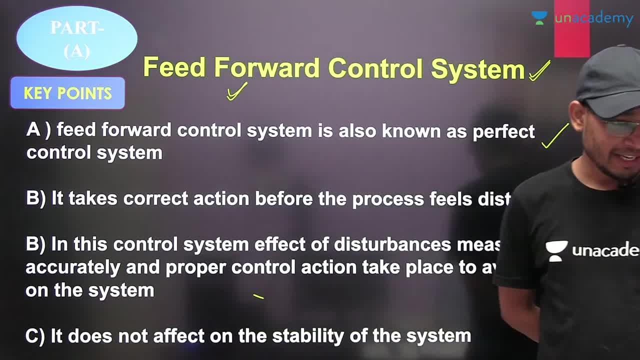 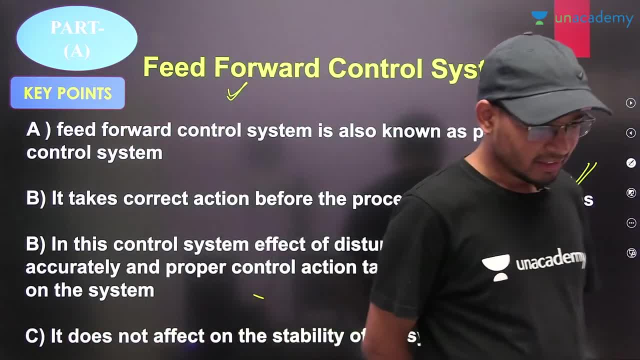 Let's take action in it first. Whatever action you have to take, we will take it first. Yes, Unit 9.. This is your last unit. This unit is last, Ok, So first of all, write all the points properly. 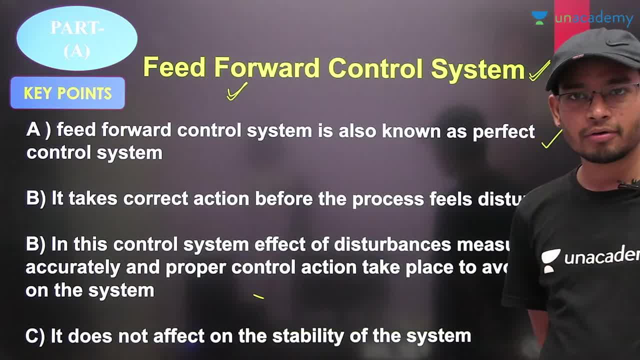 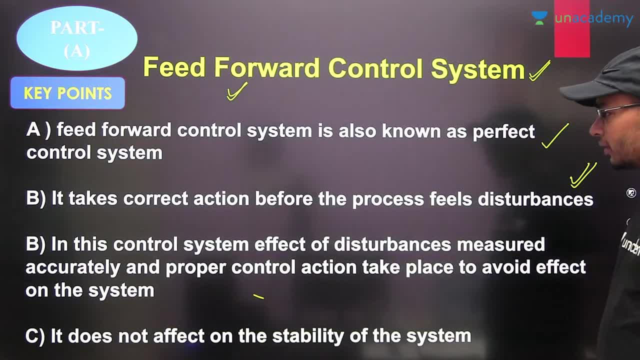 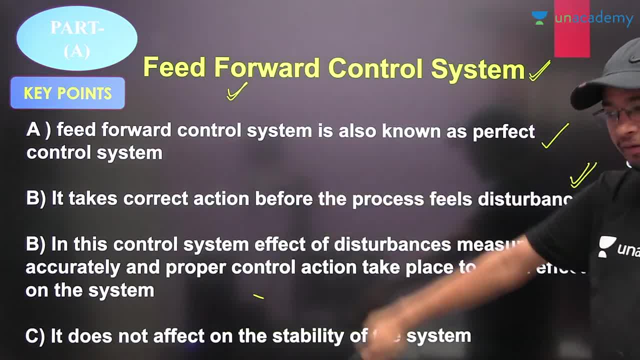 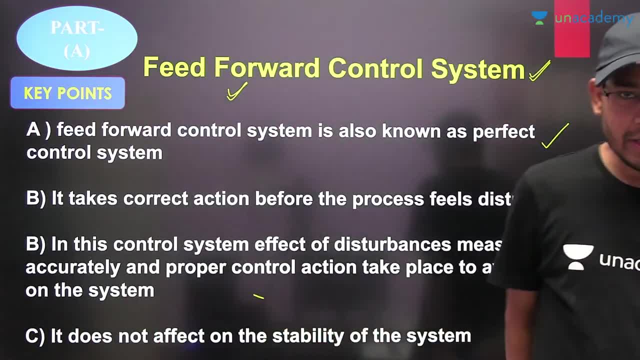 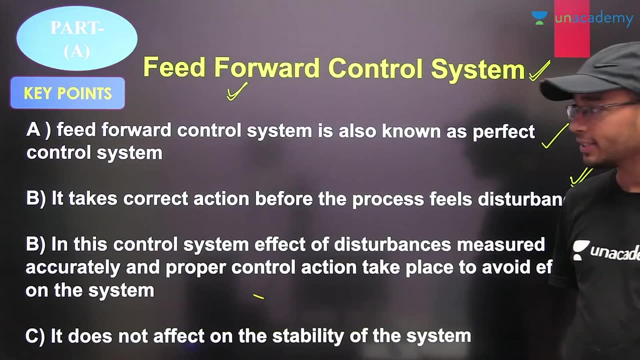 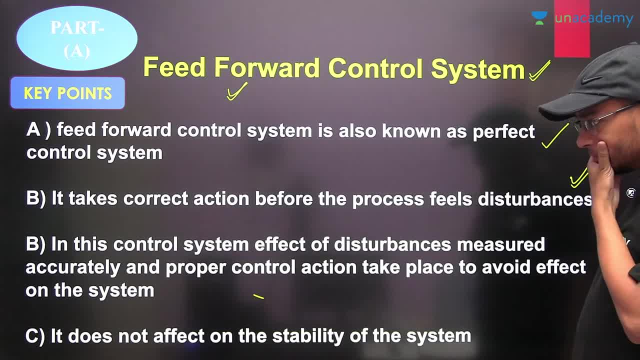 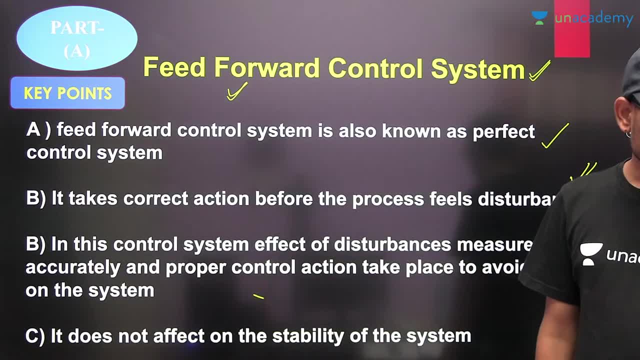 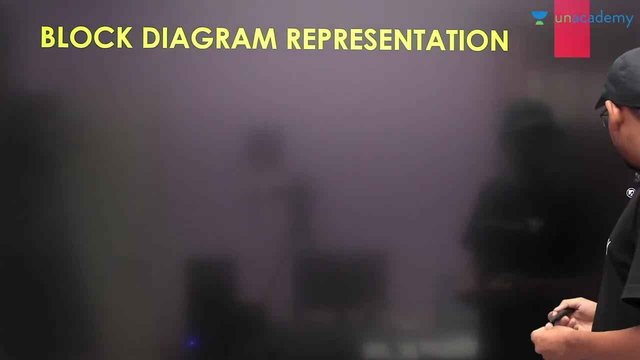 This is a little cheaper And this proteges your disturbance in the case of any disturbance rejection. It does And it manipulates the disturbance very well. Now I will talk about this next Block diagram representation. Everyone will add heading. Block diagram representation. 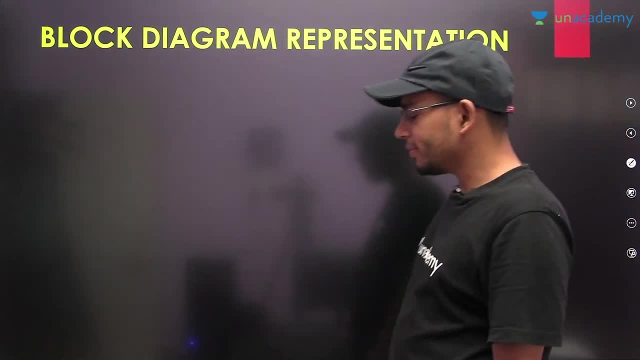 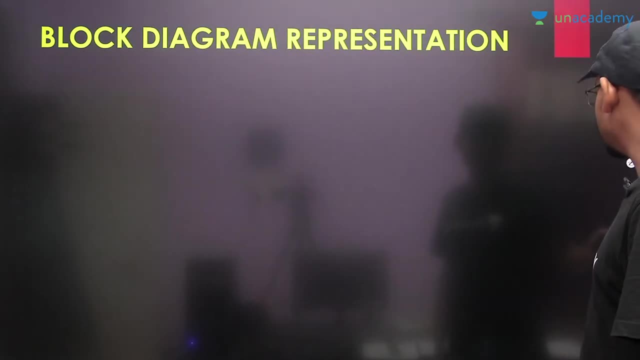 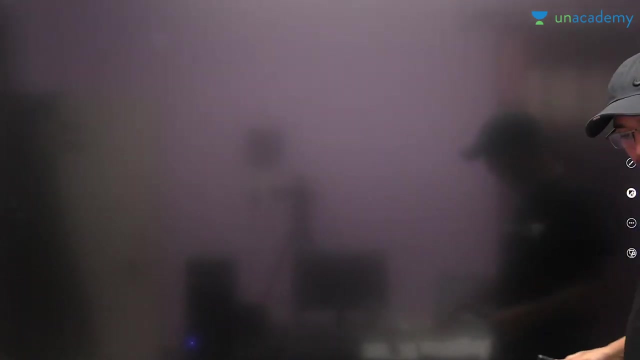 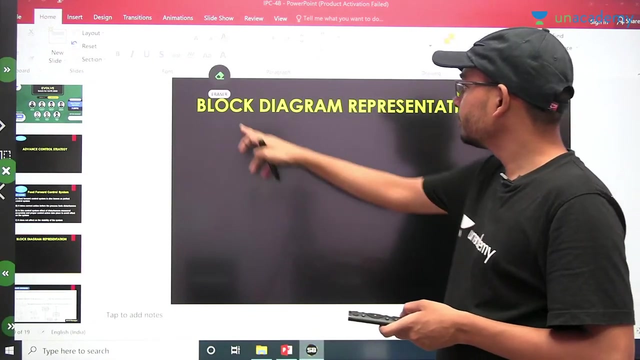 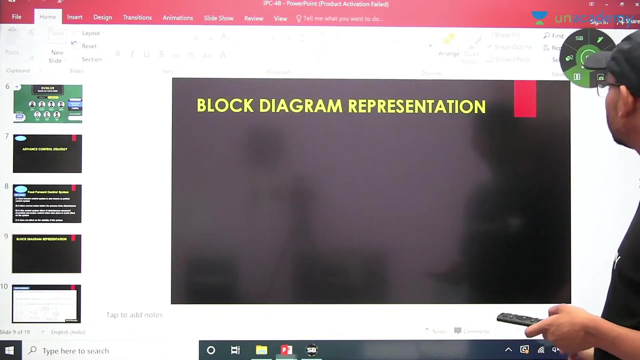 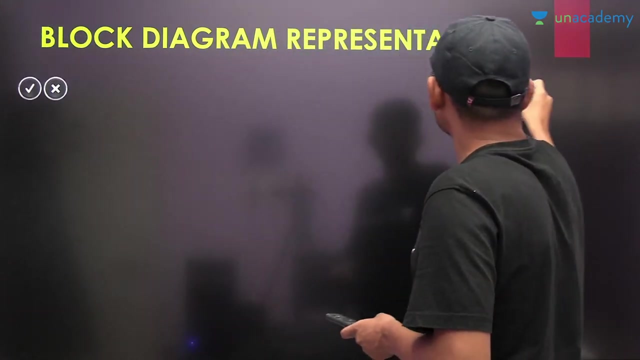 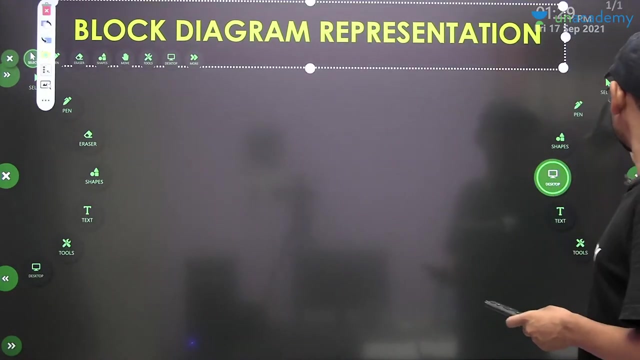 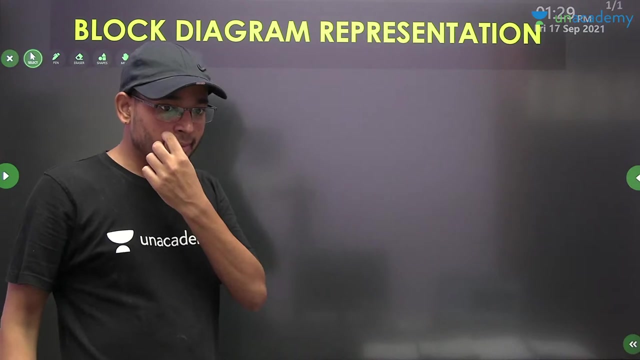 Everyone will add heading nicely. Block diagram representation. Block diagram representation. Everyone will add heading. Block diagram representation. Block diagram representation. Block diagram representation. Ok, Everyone will add heading. block diagram representation- Done, Ok. First we can learn about the block diagram properly. 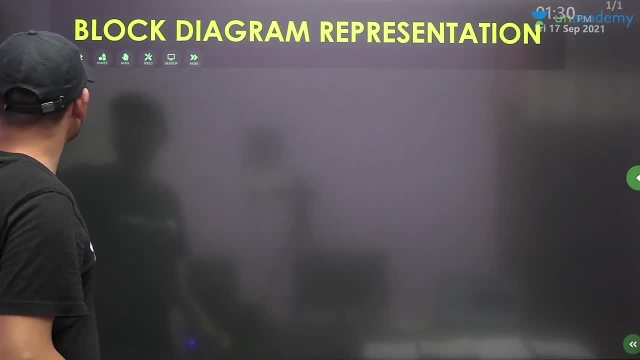 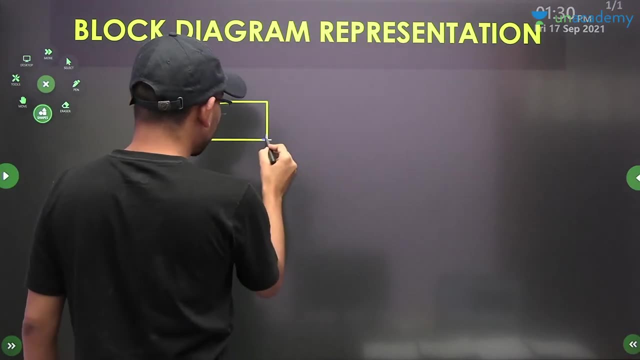 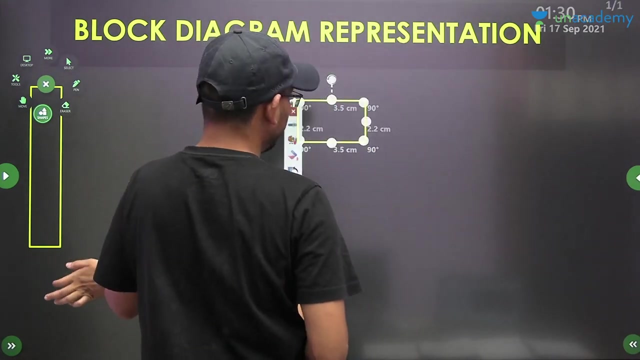 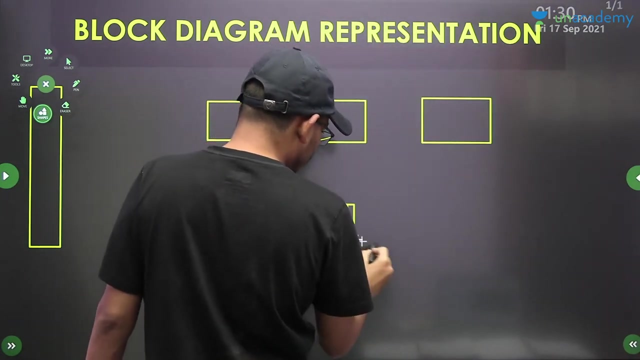 Let's understand its block diagram properly. So how did you make a closed loop system before? One was your controller, One was your final control element. This was your final control element, And one was your gp. One was your gp And one was your gm. I will write load. 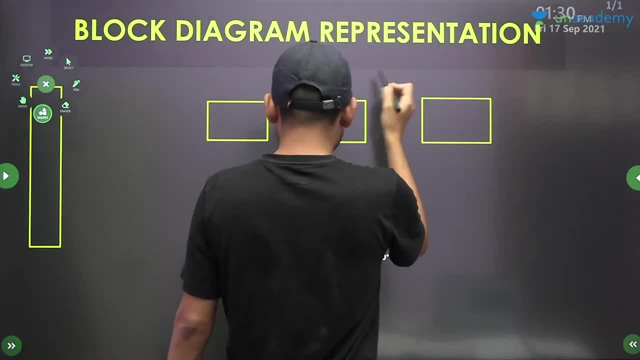 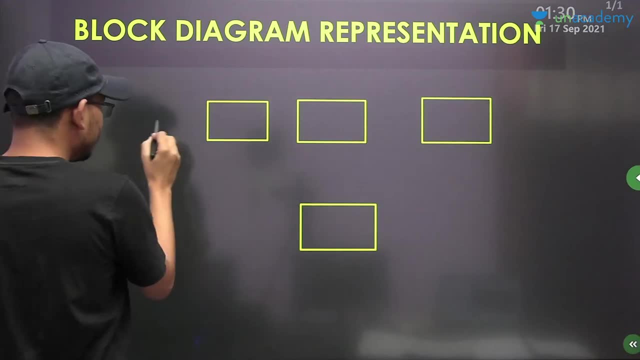 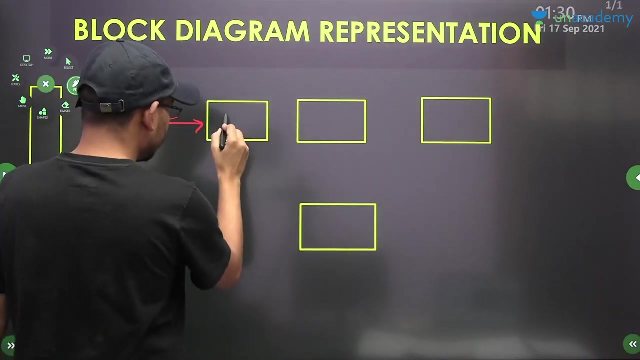 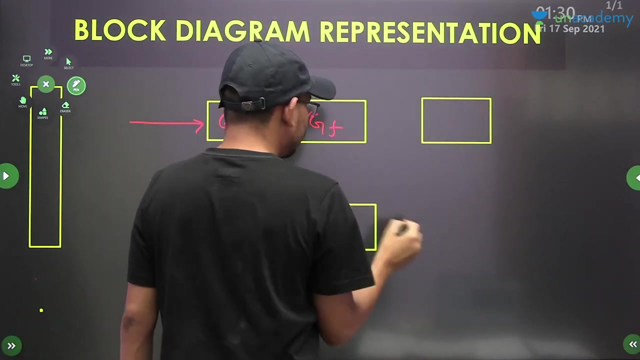 One load. I will write load, I will take pen. So what will be our eap? This controller was normal controller. Now which one you are using feed forward controller? I will write gff- feed forward controller. Where will this feed forward controller go? gf will go to gp process. 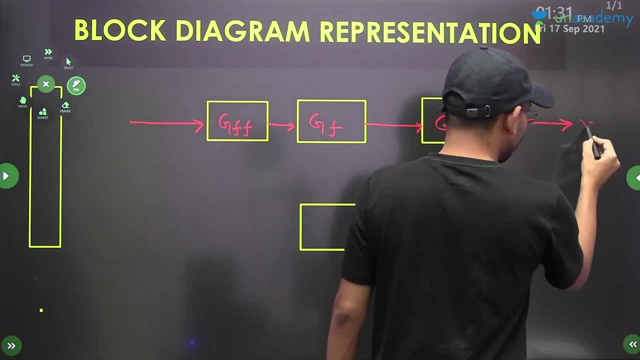 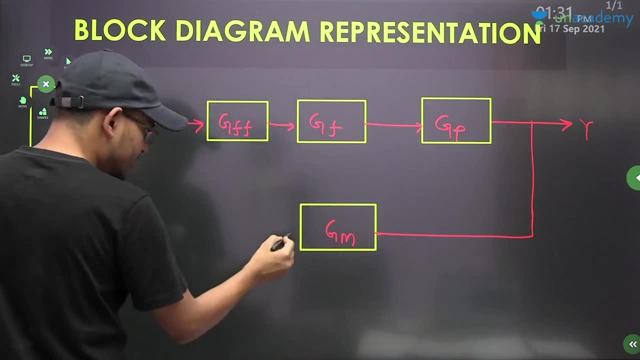 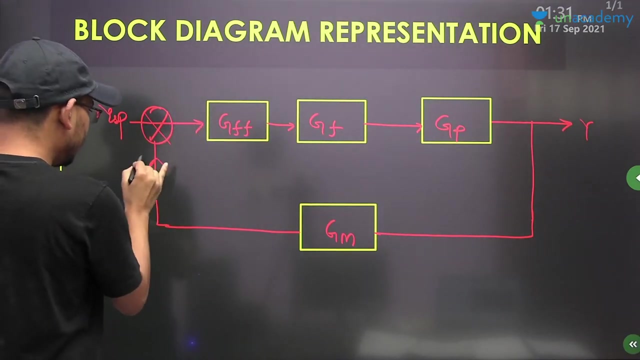 gf will go to gp process And output will come out Which we used to represent with y. This is gm. This was our measuring device. This measuring device used to match at set point. This was ysp. above this error would getaminommen in controller. This was minus and 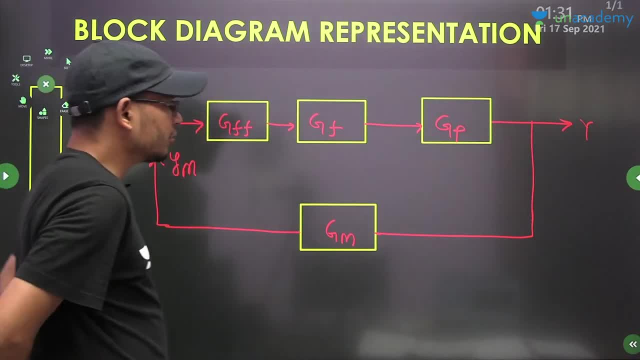 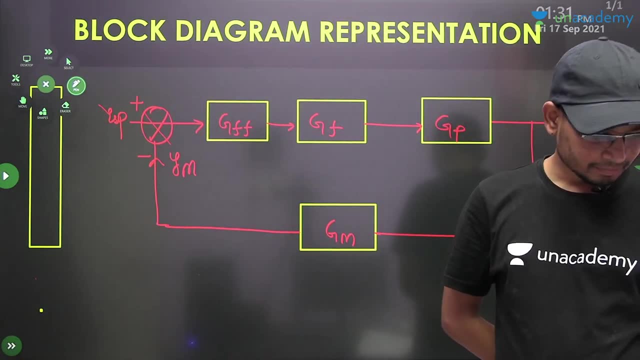 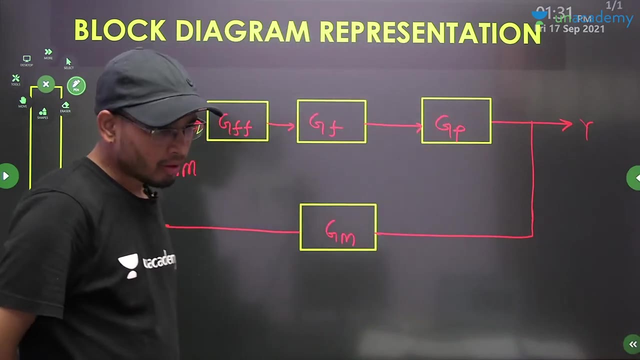 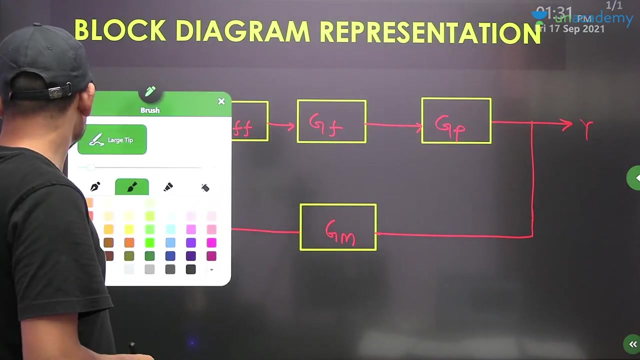 yúng for plus, And all you used to write general diagram. You guys make a diagram first. all of you will first make a general diagram properly. Now I want to load it, so load it too. I want to load it, so load it too. 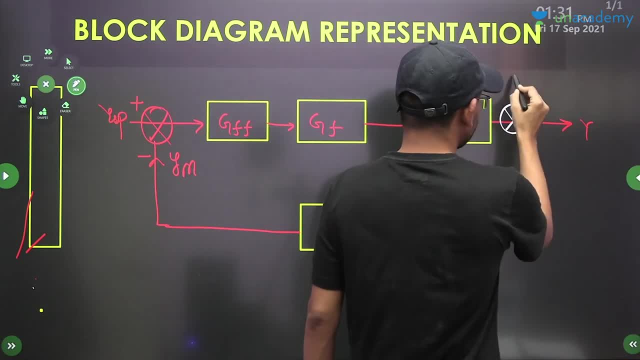 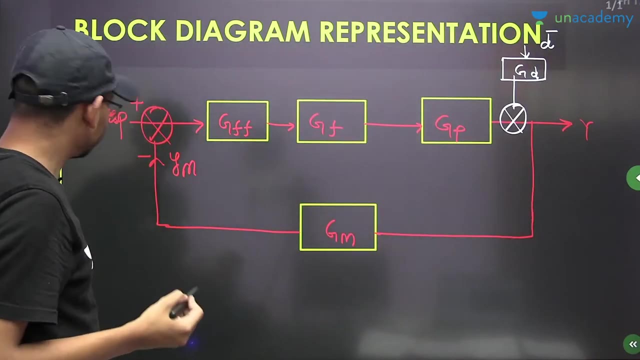 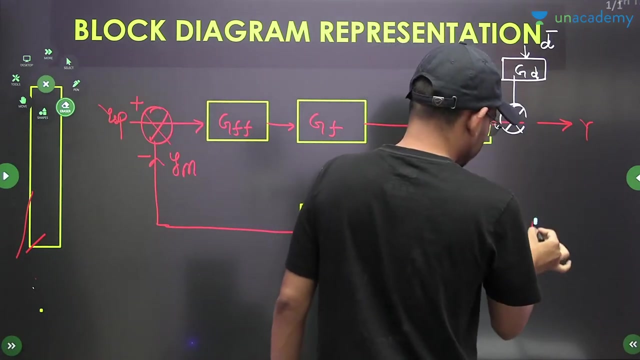 Put it here. put it here, brother gd, and here will come our small d bar. small d bar. ok, Erase it a little from here, make a little space for it And make it something like this: This is your y going, ok. 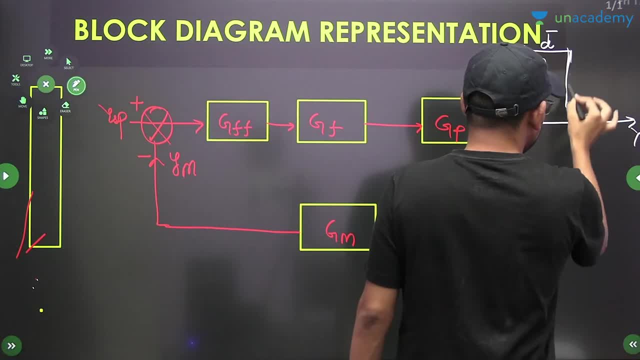 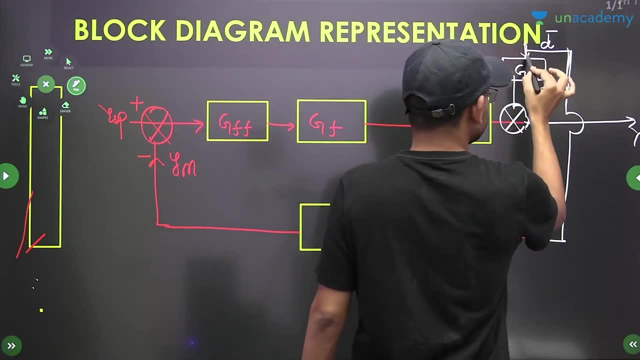 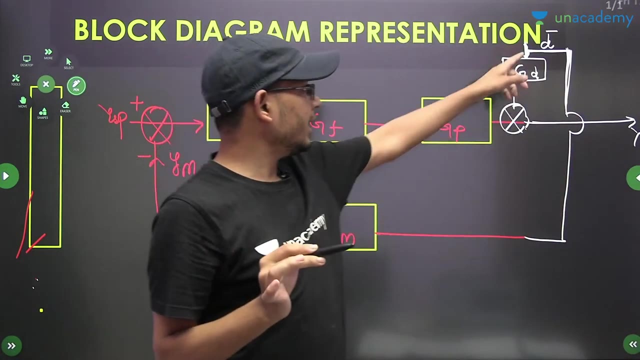 And transfer one more signal from here. One more signal. this is a pipeline. ok, it is a joint. What is this? It is a joint. What is this? Transfer function of the disturbance. What is this? Input of the disturbance, that is the d bar. 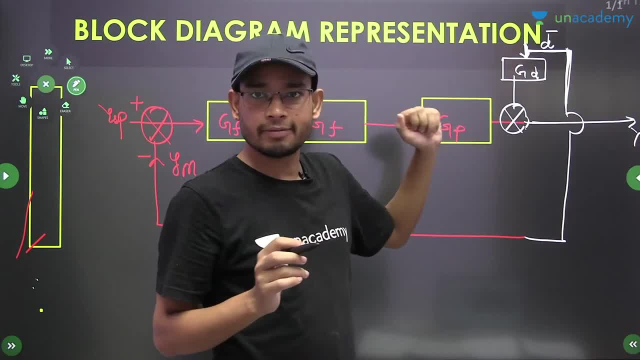 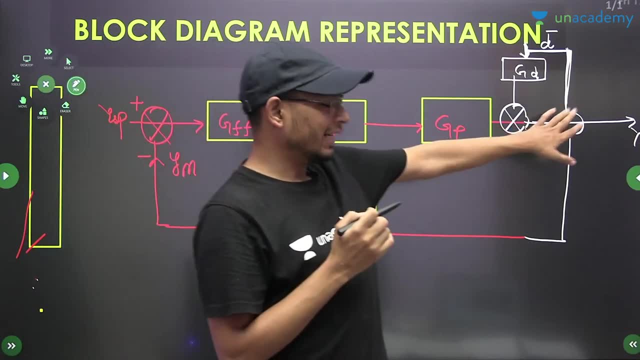 What is d bar Input of the disturbance? Ok, this is the transfer function of the disturbance. This is the comparator. This is the comparator. right, Make all of you more before this. This is a joint here. Ok, put both the signs plus. 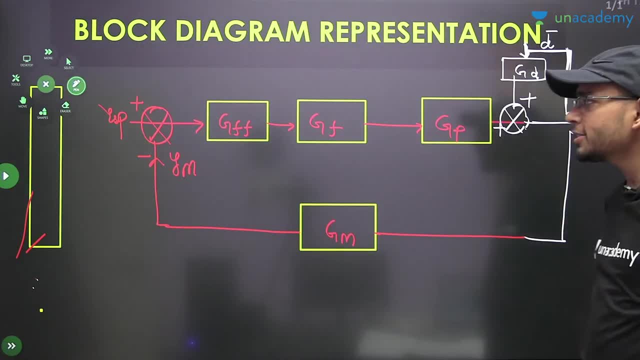 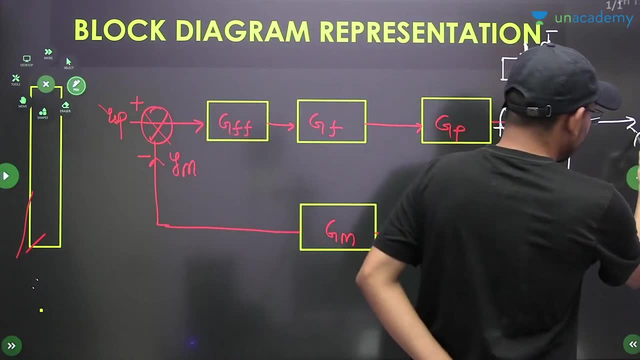 This is also plus, and this is also plus. Ok, now you guys solve this. All of you solve this a little. Yes, this is the output. This is the output By output. This is by output. see, This is your output. 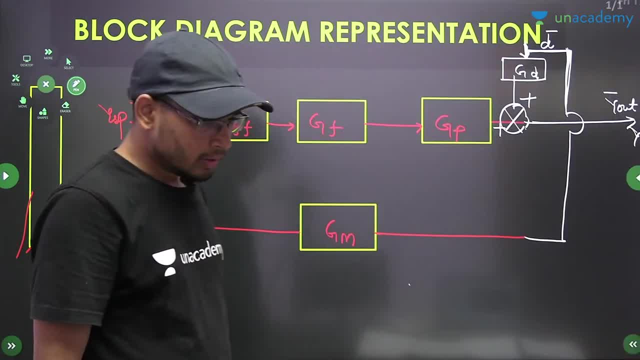 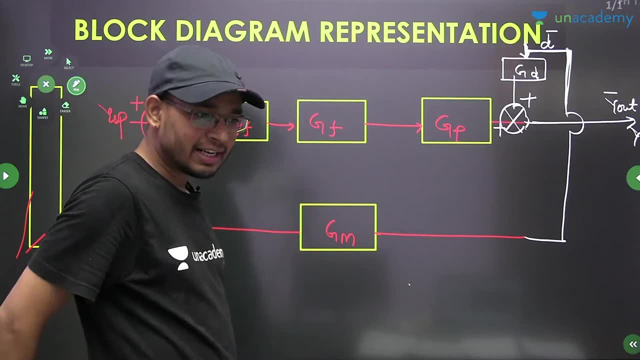 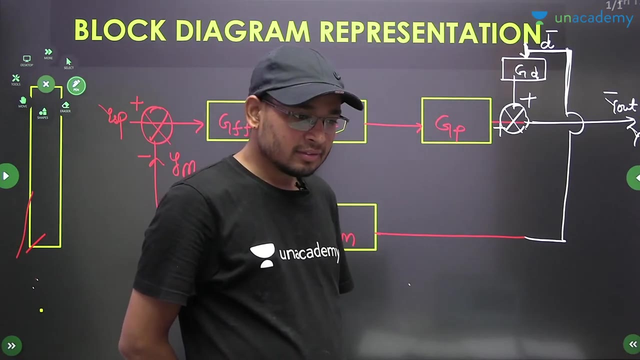 So Yes, GF, GM, This is the GF. What is GF? Are you doing the class for the first time? What is GF, What is GF, What is GF? All of you tell them by commenting: What is this? 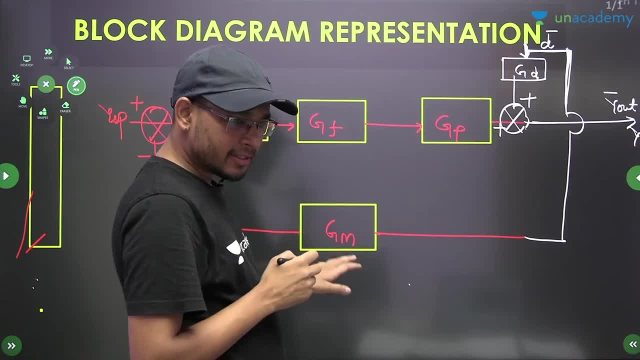 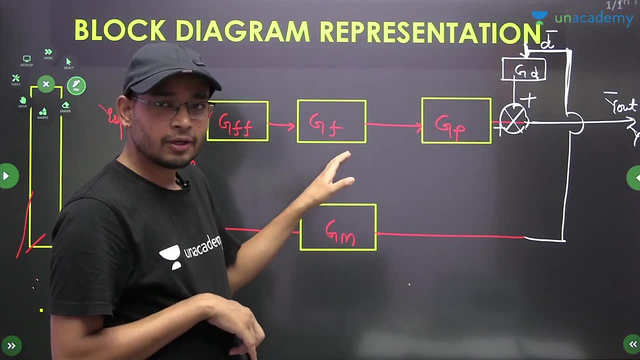 GF GM. This is the transfer function of the measuring device. This is the transfer function of the control valve. Ok, This is the transfer function of the control valve. Ok, You have not done the last class. Ok, Do the last class properly. 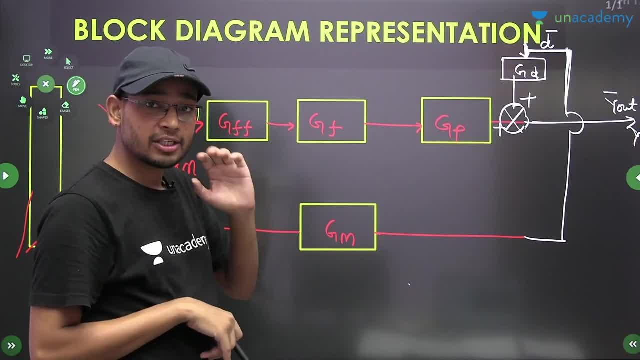 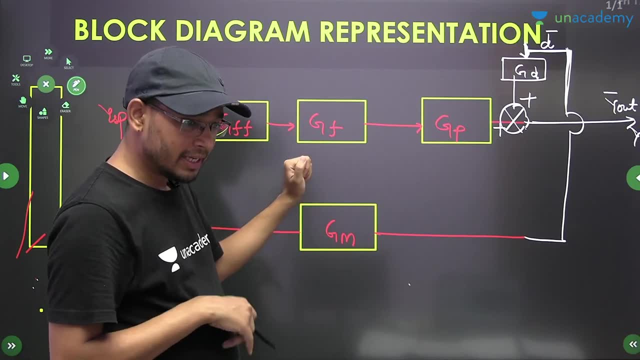 It is very important to solve all of this. I have explained very well how to solve these boxes. Ok, What is GF Transfer function of the control valve? Final control element: Yes, Ok, Final control element. What is this Measuring? 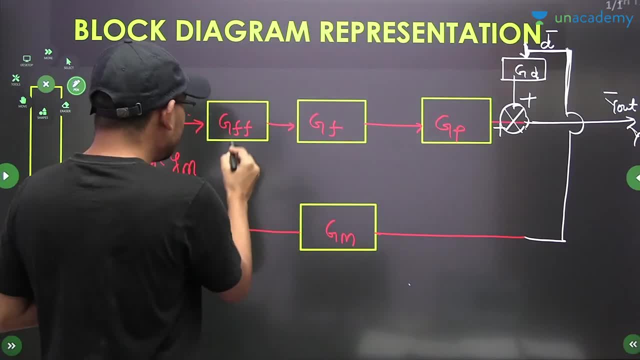 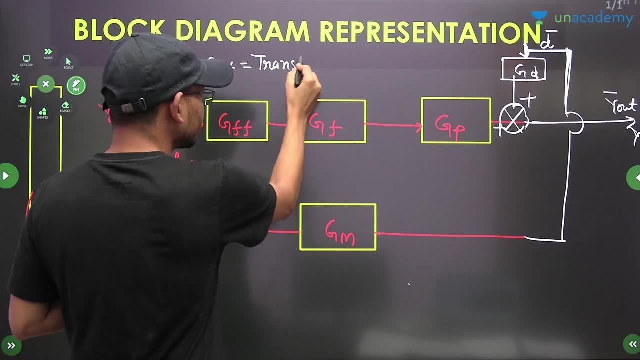 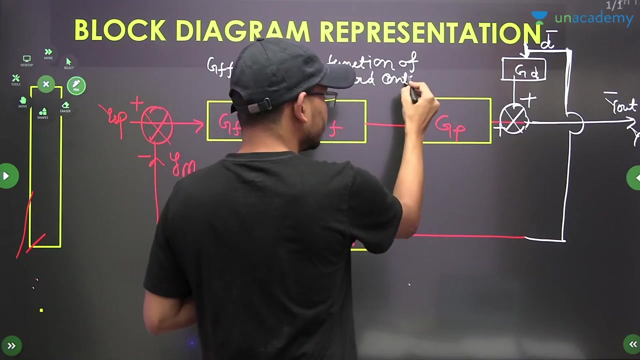 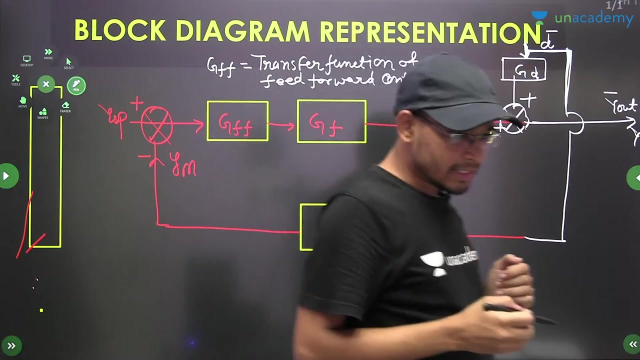 Yes, Measuring element. This is the block diagram. What is this Write? GF- Transfer function of feed forward controller. Ok. Transfer function of feed forward controller. Ok. Transfer function of feed forward controller GFF. Yes, We will solve it later. 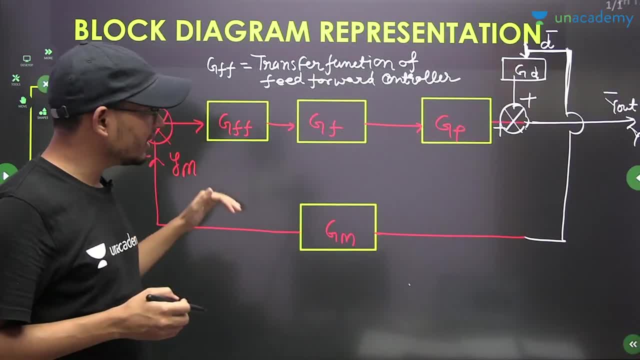 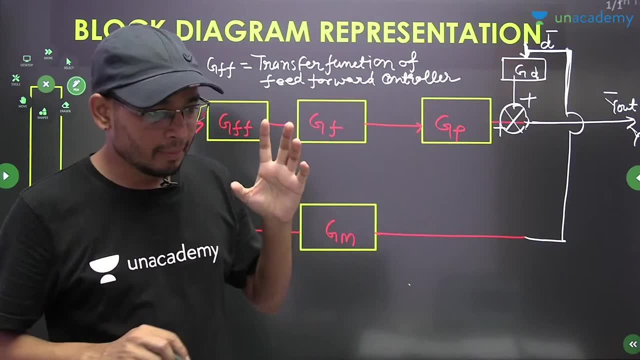 We will solve it later. First, design it properly, Then we will solve it. Look very carefully. I have told you very well how to solve the block diagram. Ok, I have told you very well And understand it properly, Because the last part of IPC. 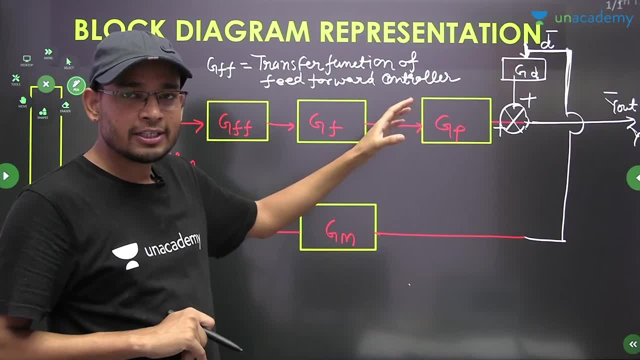 The better. I have told you, You have to understand it very well, Otherwise there will be confusion in it. Ok, So understand it very carefully. Everyone solves it properly. Come together, All of you come together, And we solve it very nicely. 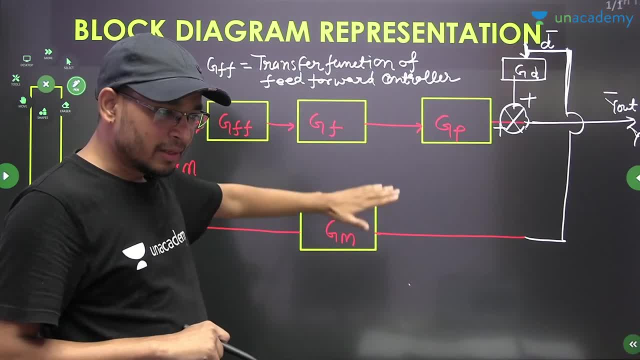 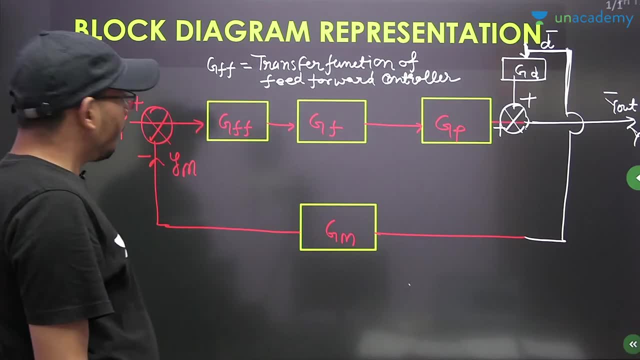 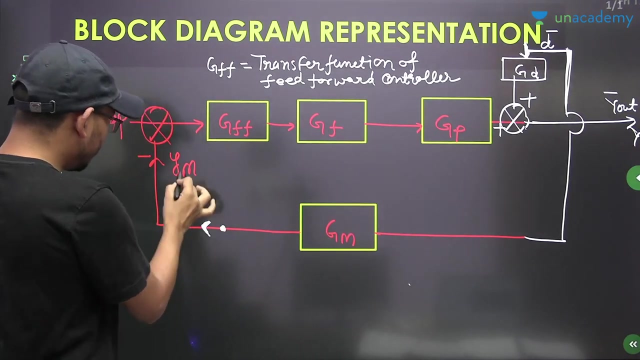 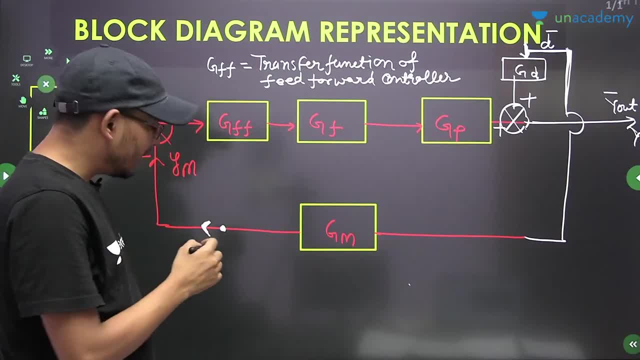 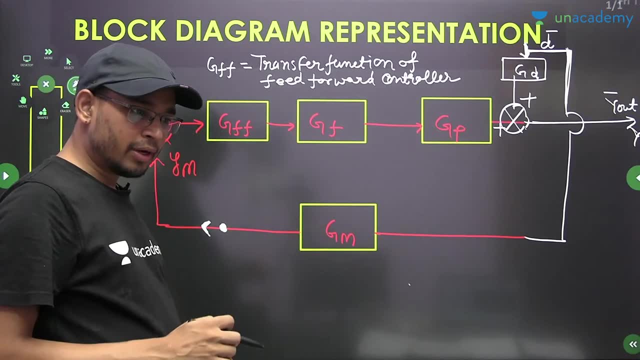 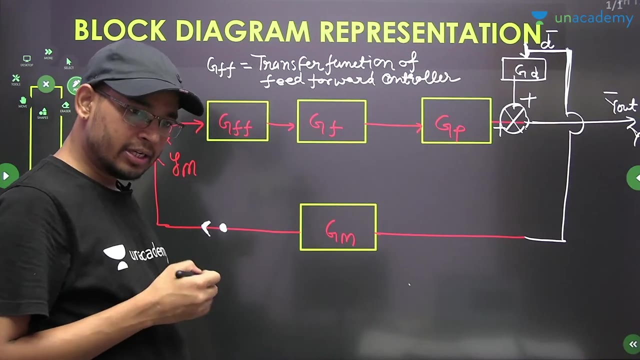 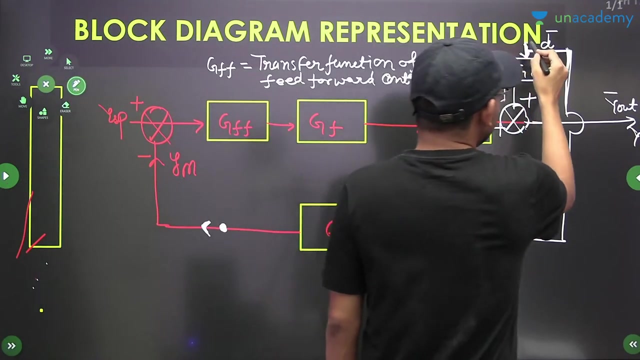 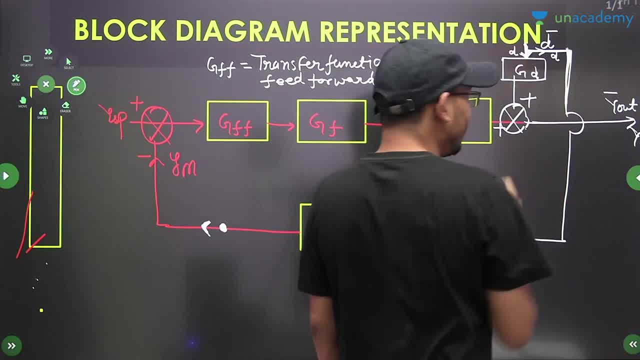 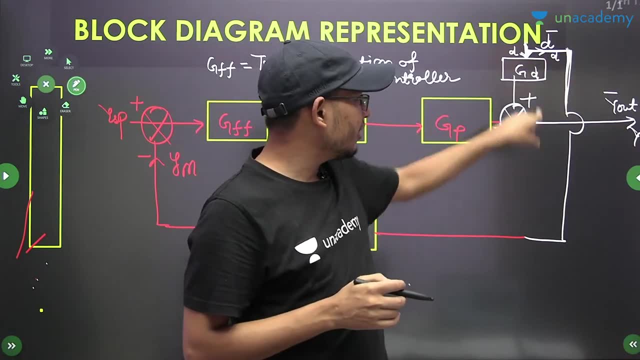 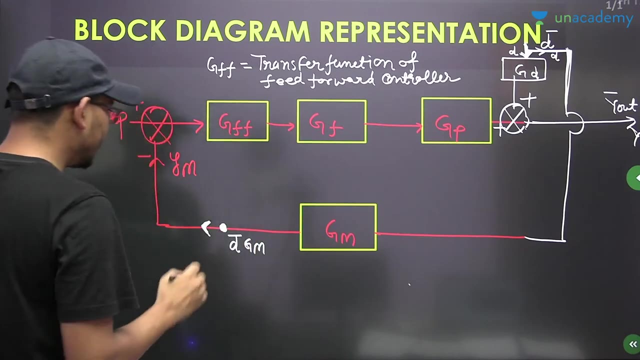 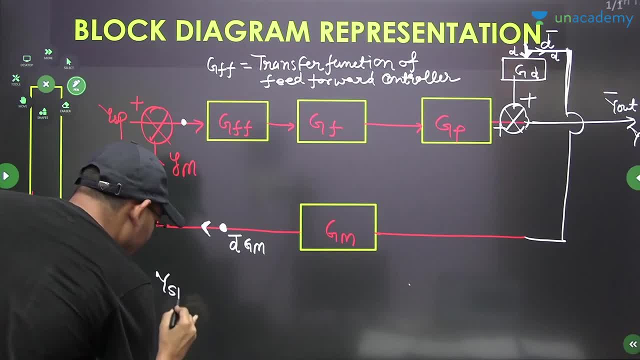 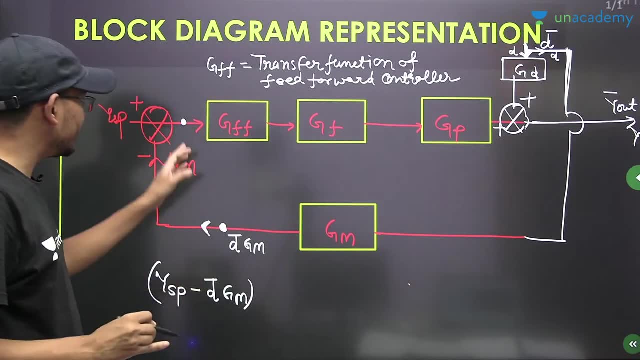 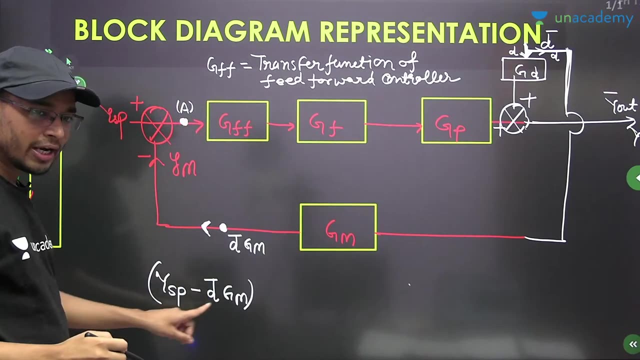 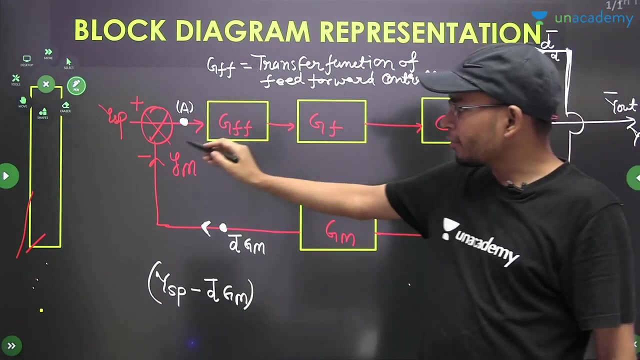 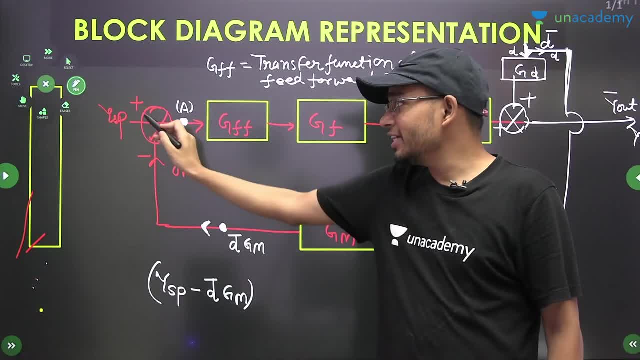 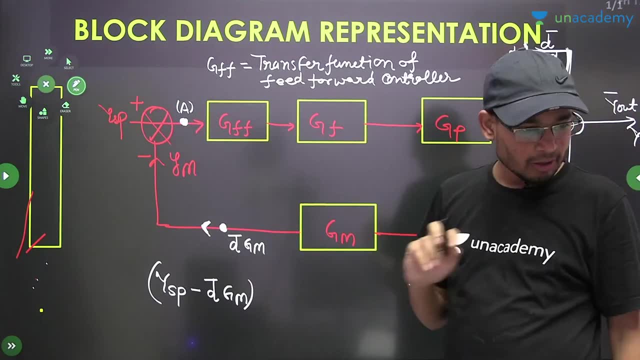 Because this is minus. so this much signal is coming from here. And what is this YSP? This must be coming with positive, So this must be minus with positive. This much error must be going in which. This much error must be going in which. 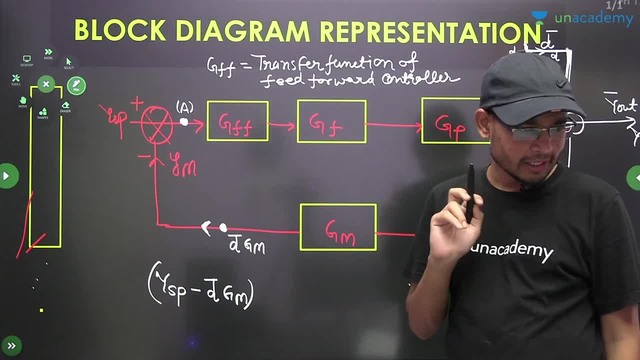 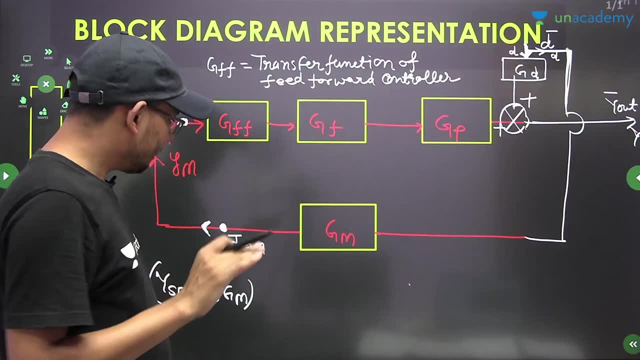 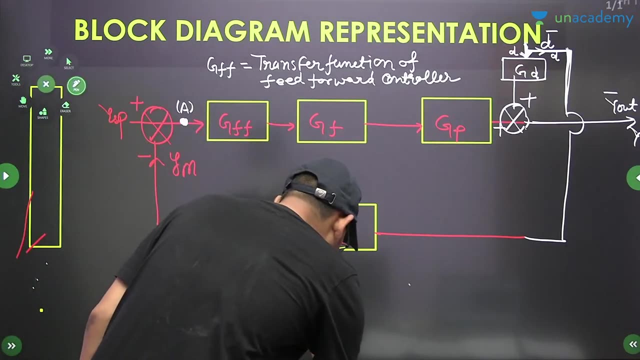 Yes, in our controller. This much error must be going in our controller. There is no problem in this. Look very carefully. This much error must be going in our controller. Right Now, hlm will multiply in GFF. Ok, This'll multiply in GF. This'll multiply in UP. 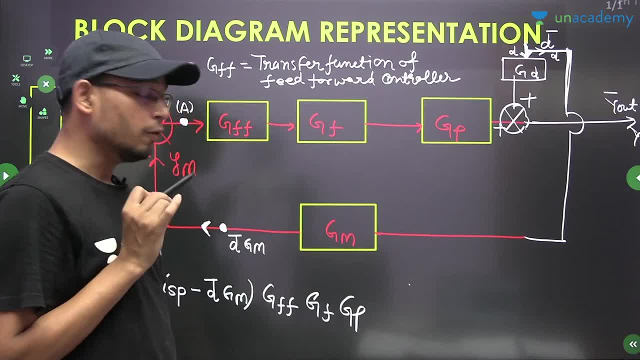 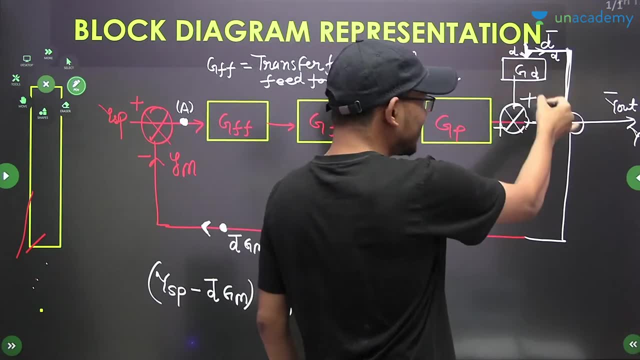 анst there Now what to do here? Wait for some time. Now tell me, this will add. And how much signal is there from above And how much signal is added from above? How much will be added from above? How much is added? 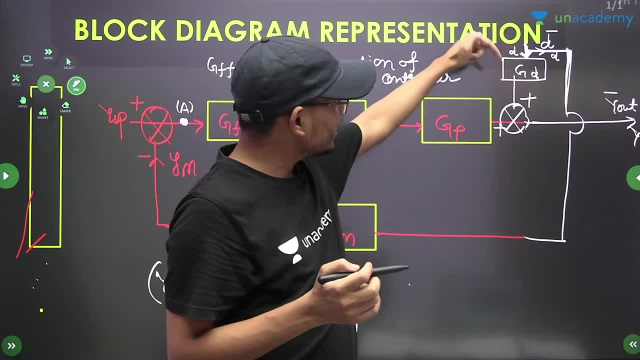 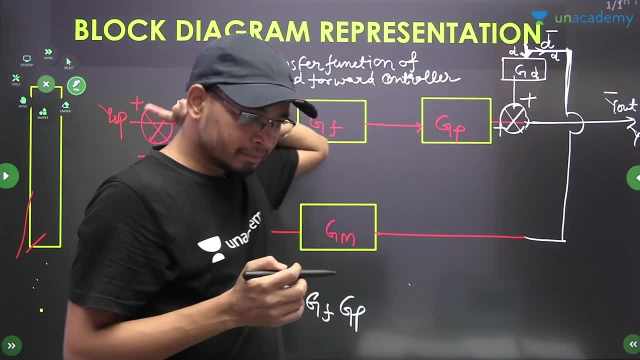 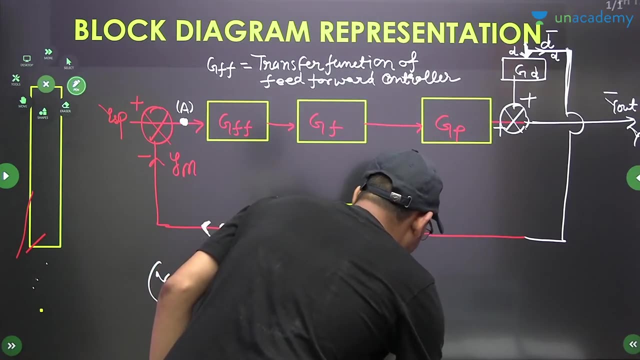 All of you tell me, How much do we add From above? how much signal is there? how much signal is coming from above? d-bar into gd, yes, d-bar into gd. how much is coming with plus? d-bar into gd, into gd, right, no problem. 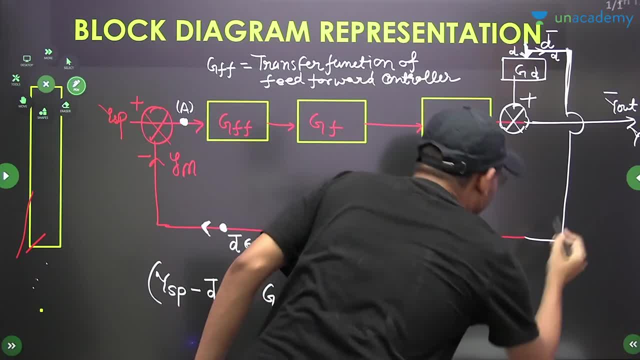 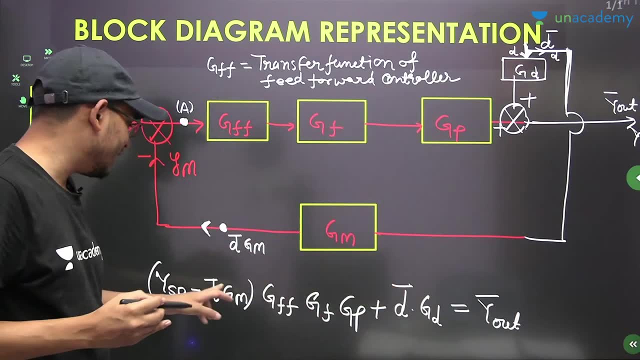 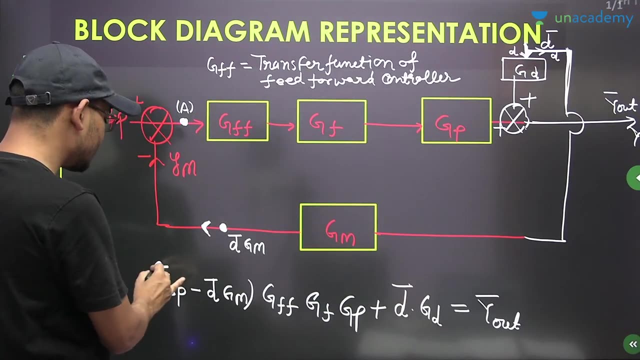 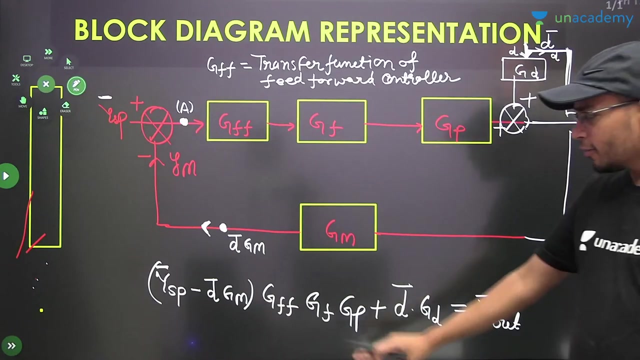 is equal to is equal to output signal. output signal is y-bar. y-bar means deviation. all the bars are deviation. you can put bar on this. you can put bar on this means transfer function is written in deviation form. that's why bar is written. why bar is written? because of deviation. 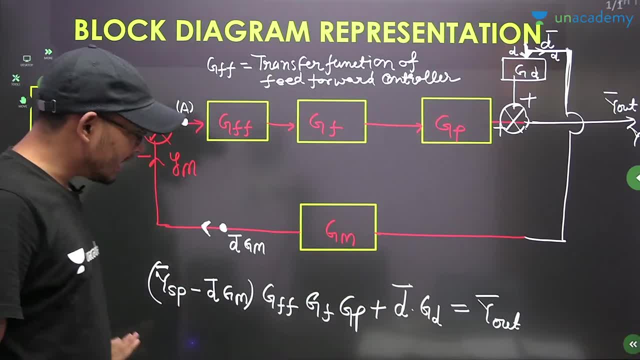 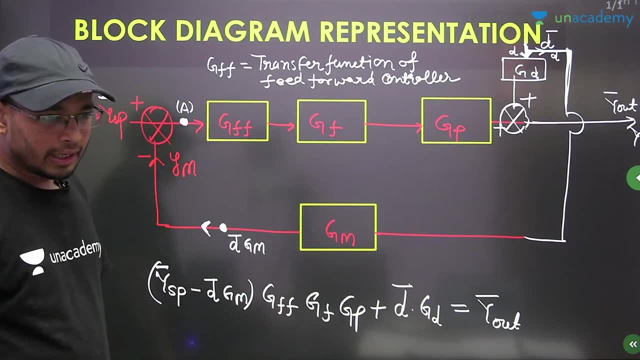 tell me everyone: are you able to reach this line? you have to write this line. ultimate story is in writing this line. are you ok with this line? crystal clear: are you ok with this line? everyone, everyone, is feeling comfortable in writing this line. everyone is feeling comfortable in writing this line. 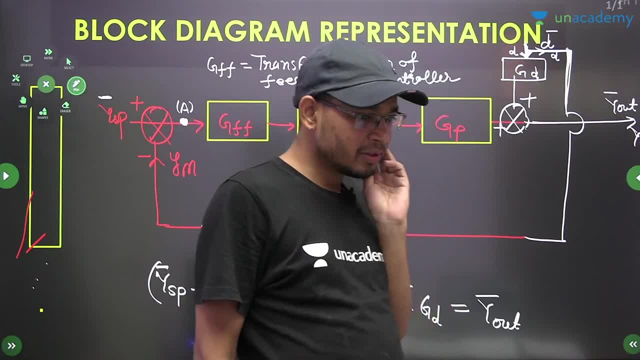 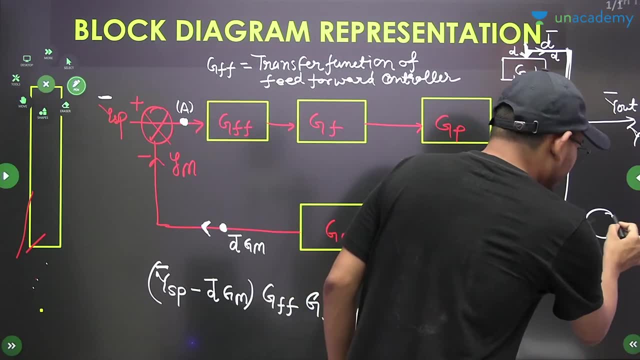 sir, i am confused about minus and plus multiplication. sir, i am confused about minus and plus multiplication. see, as minus goes, suppose your controller is on. see, i am telling you, as this controller is on, you have not done this first class. i have worked on summing junction a lot. 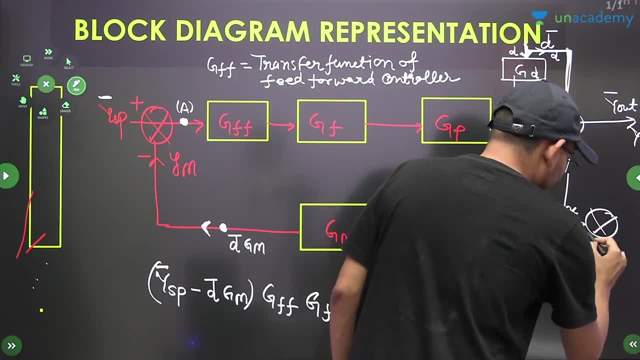 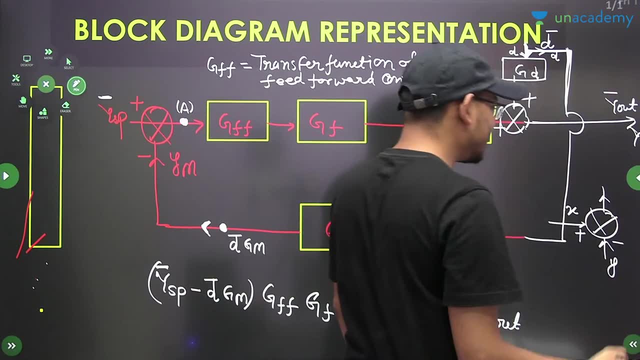 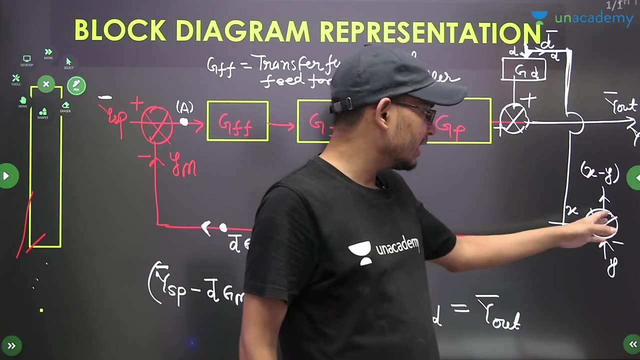 suppose your signal is coming: this is x and this is plus, and from here your signal is going y, this is minus. from here the output will be x minus y, x minus y. in case plus signal is going, minus signal is coming from here, the output will be: 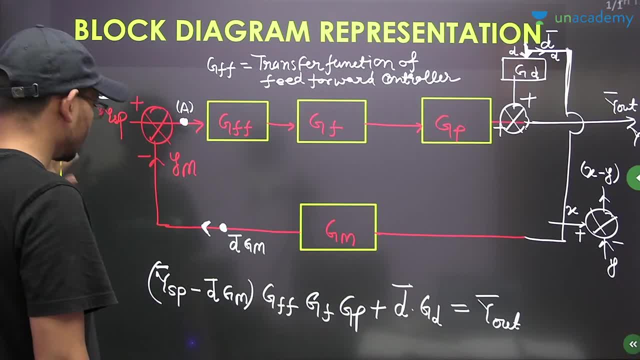 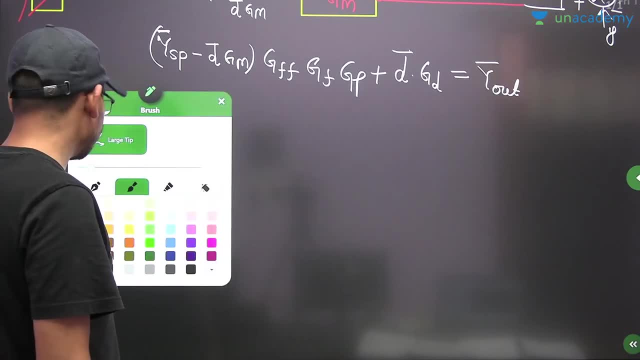 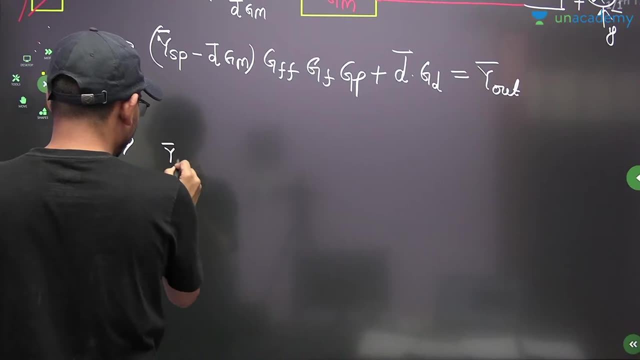 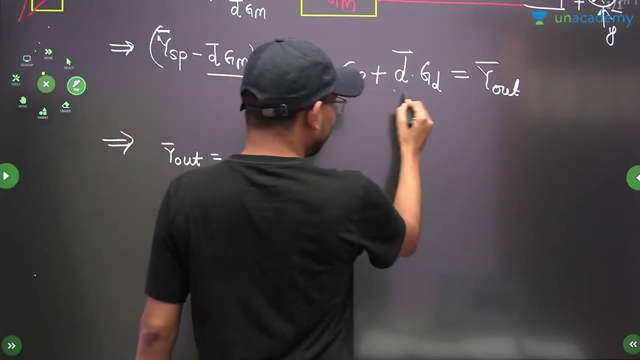 x minus y. this is the concept till here you have written. now solve this, do solve, solve carefully. so what will be? output equal to y bar? output equal to which one? equal to bring d bar together. d term is here and d term is here, bring them together. 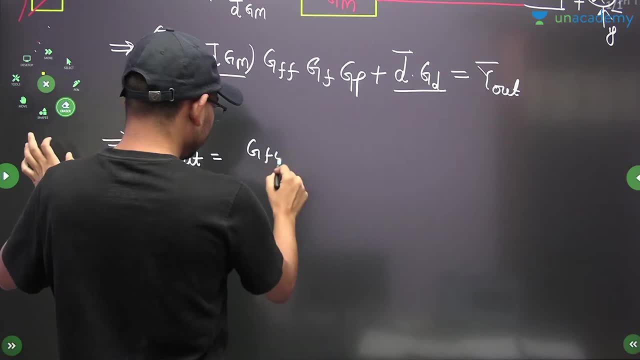 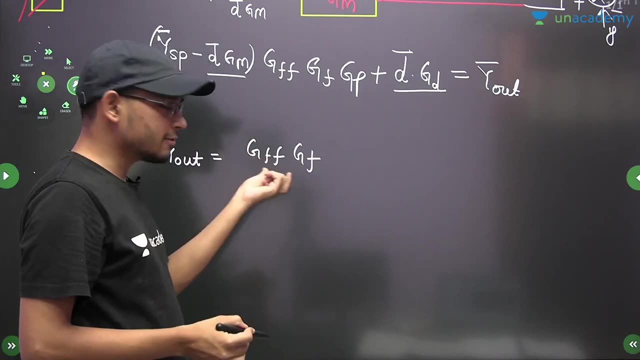 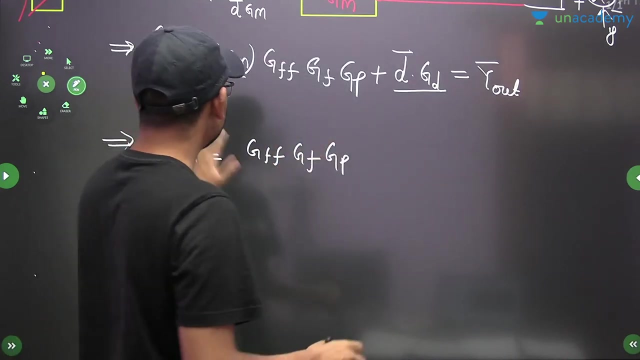 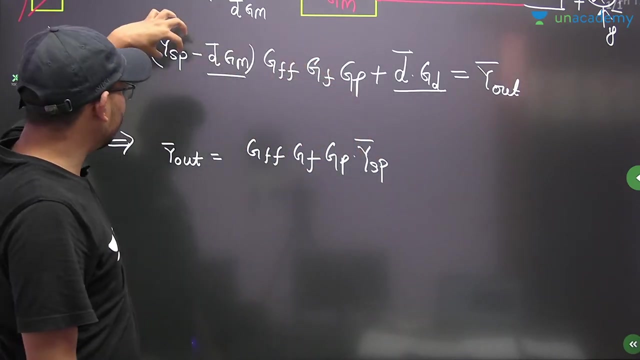 so this will be gff, gff, gff, x, gf. gff is the transfer function of the controller and f is the final control element and gp is the process. first order, second order, whatever the process is, and this will be multiplied by var sp. there is no problem. I have only multiplied these three parts with this part. 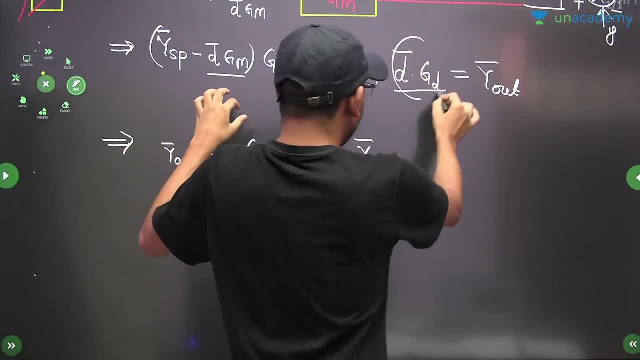 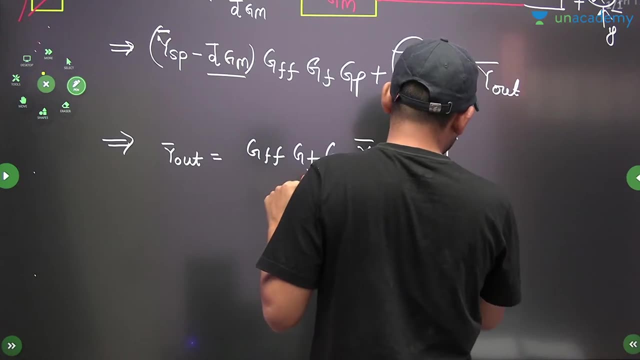 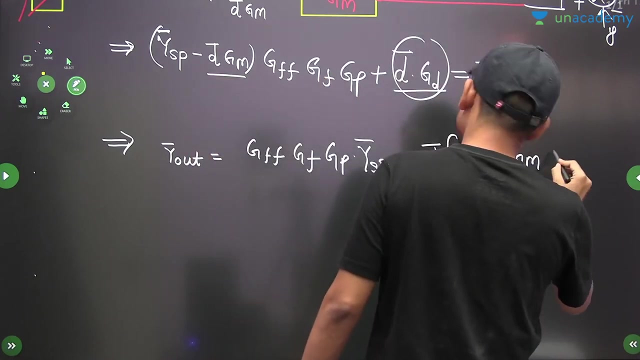 now I am taking them together and I am doing them together. I am writing them together with multiplying. so look carefully: plus d var, I am multiplying and taking the common too. I am doing everything. look carefully: gd minus, gm, gf, gp. tell everyone. can everyone reach here? this is the buyout. so I have written here. 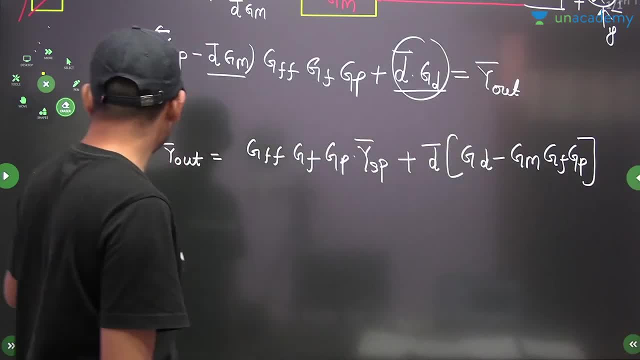 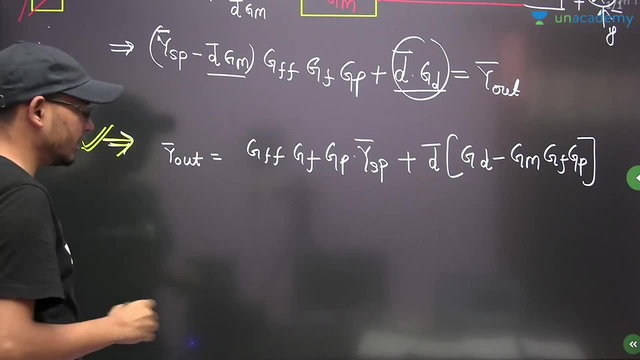 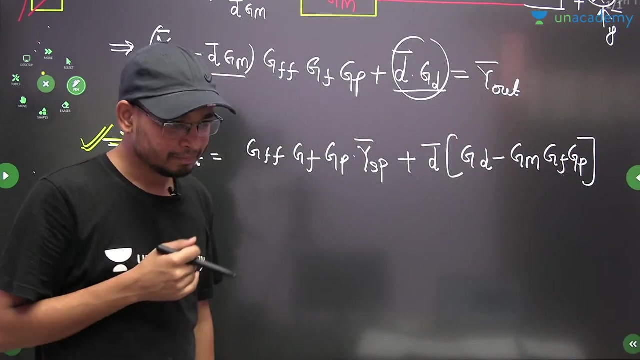 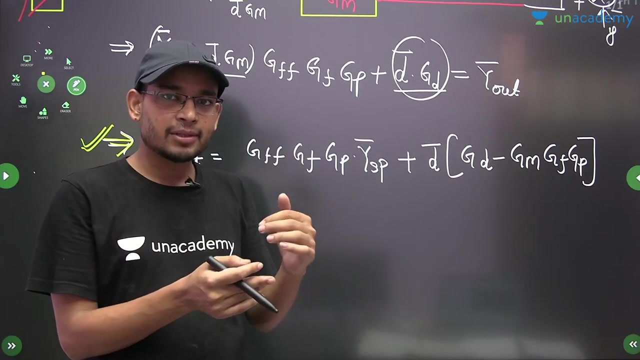 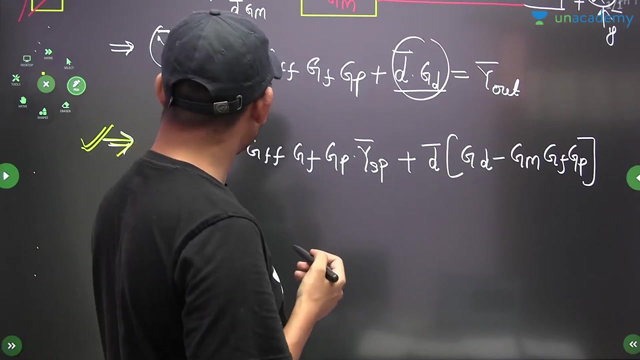 can everyone reach here? see once, can everyone reach here with a smile. everyone, everyone are ok with this line. can everyone reach here? yes, all the transfer functions are multiplied. comparator means summing junction. summing junction means addition and subtraction. gf is left. gff is left here. 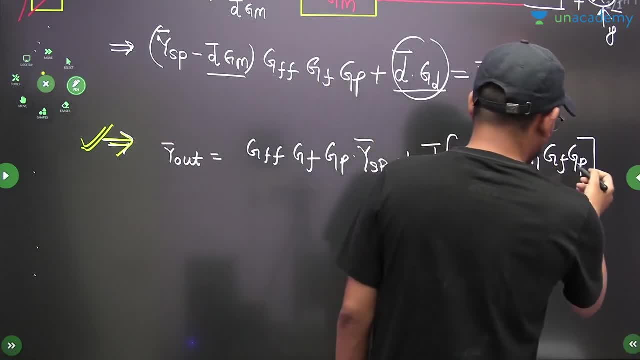 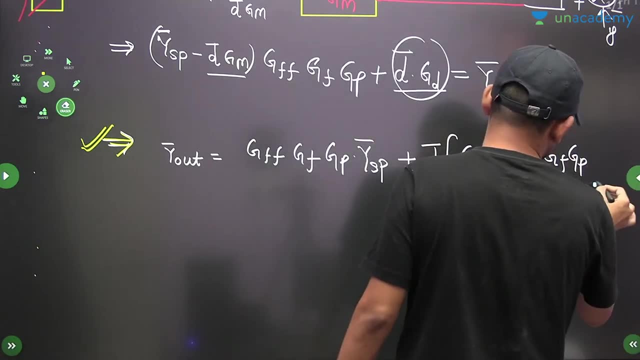 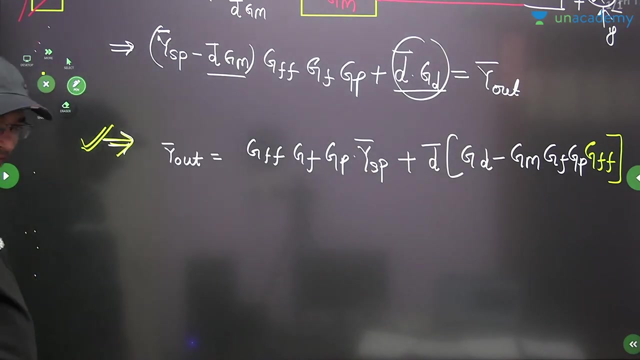 d var is left here, any one, c Razor, any another, any other, any one, any other, no one, any one. Put this in bracket. Put all of them in bracket. Put this in bracket Now. start from here with cases. Now start with cases 1 by 1. 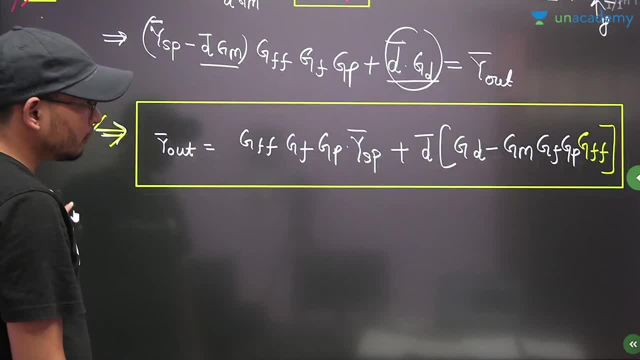 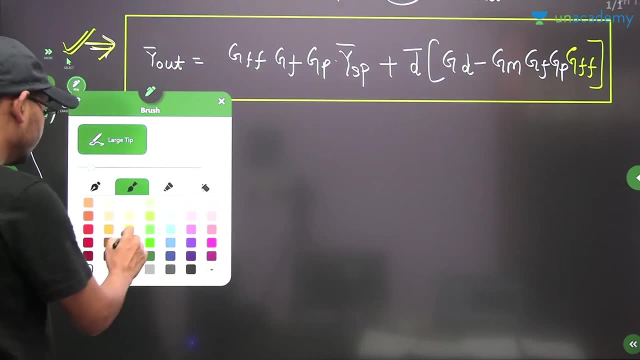 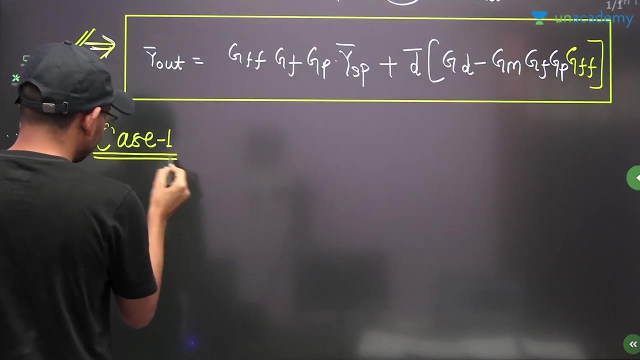 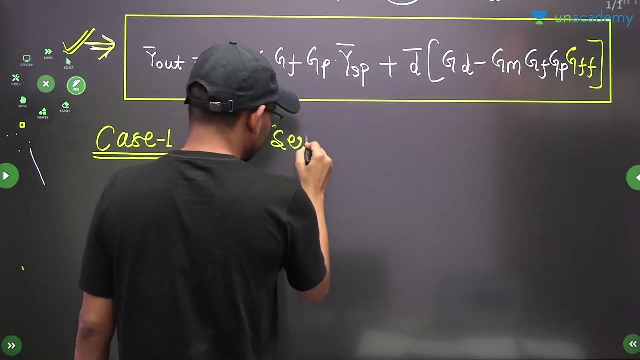 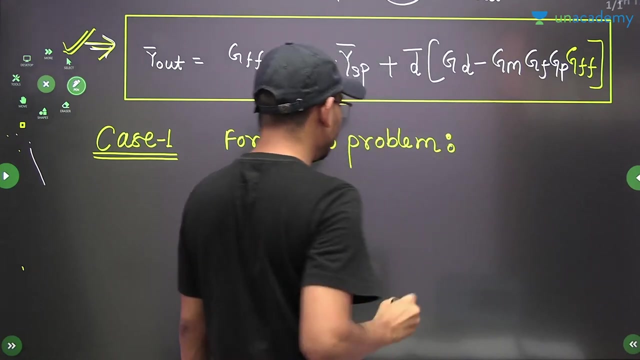 Now we will start with cases 1 by 1 properly. Put this in bracket. Now write case 1. Write very carefully case 1. Case 1: For servo problem. For servo problem, Servo problem. What was the servo problem? People will tell me What was the servo problem. 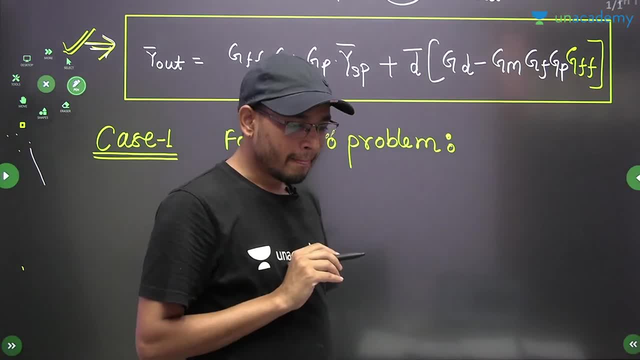 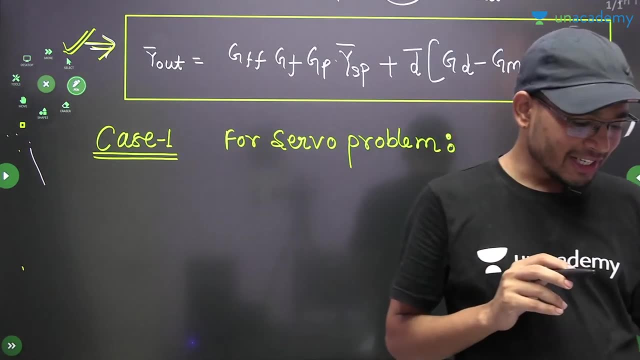 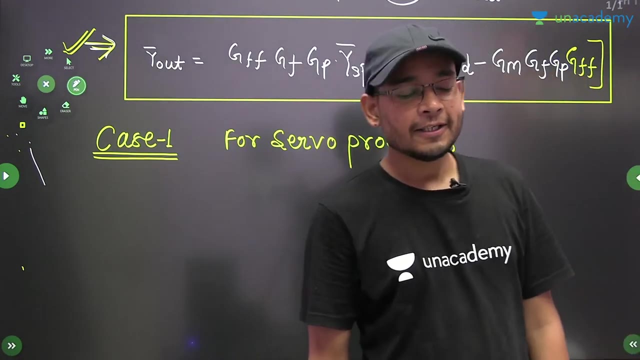 Everyone will tell you What was the servo problem. What was the servo problem? kisi ko yaad hai kya piche aap log padke aayo. what is the servo problem? hmm, there is no change in the disturbances tk. there is no change in the disturbances to servo problem. 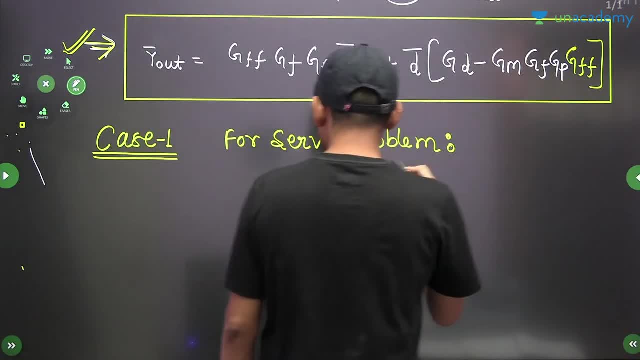 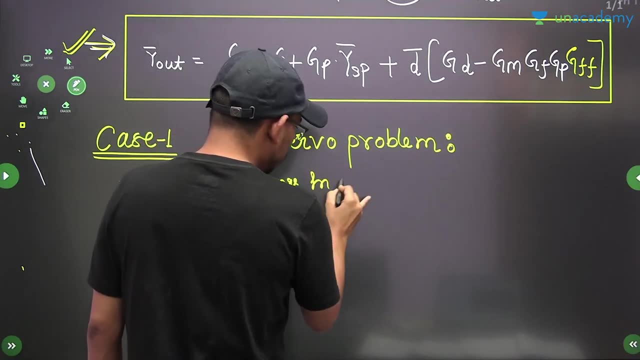 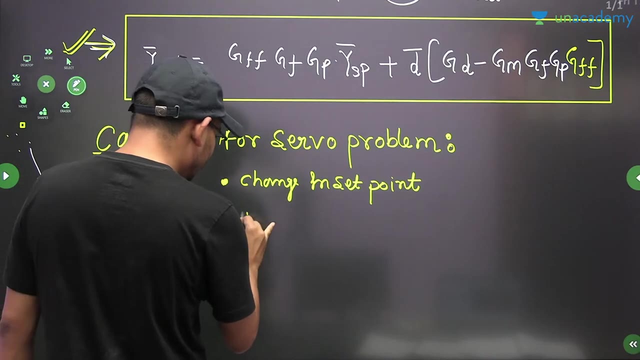 ya set point tracking isko. aur kya bolte the change in set point, iska matlab kya hua? iska meaning hua. change in change in set point, set point mein aap log change karte ho. change in set point tk. change in load mein: kya hota hai? change in change in load mein: kya hoga? 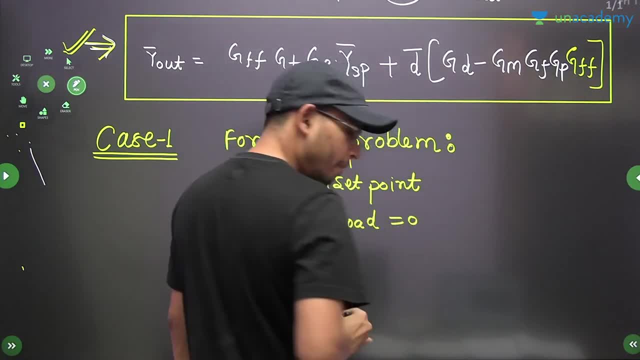 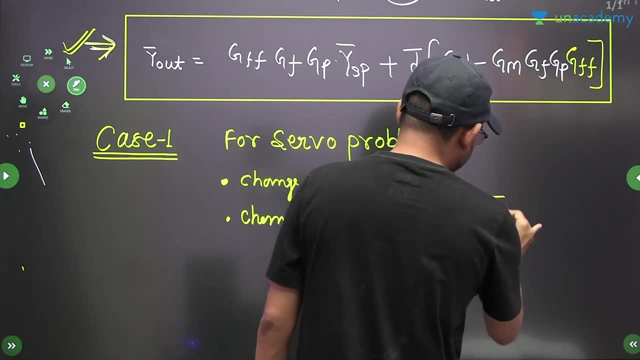 load mein kya hoga? sir, log jara batao change in load mein. kya hoga zero iska matlab d var ki value? kya ho jayegi d var ki value? kya ho jayegi zero d var ka matlab? ye change hi. 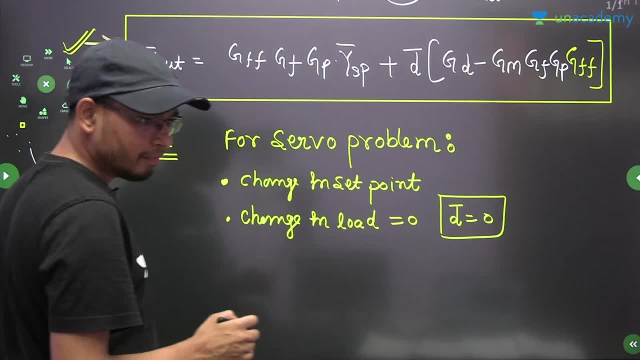 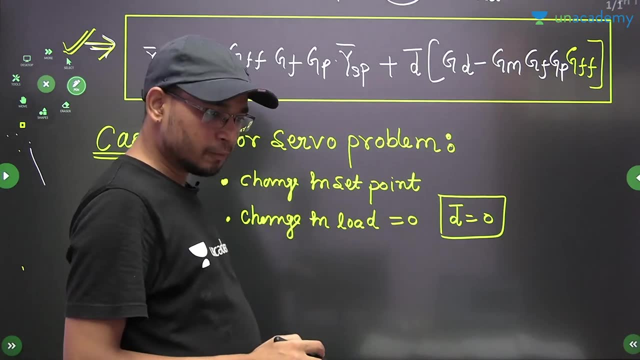 likha hua hai. ye change hi likha hua hai. tk. ye, kya ho jayega zero. change in servo: yes. set point mein aap change kar rahe hoge. change in servo: yes. change in servo: yes. change in delivery: yes. change in delivery蓁d var mein kya ho jayega. very goodjust put change in. 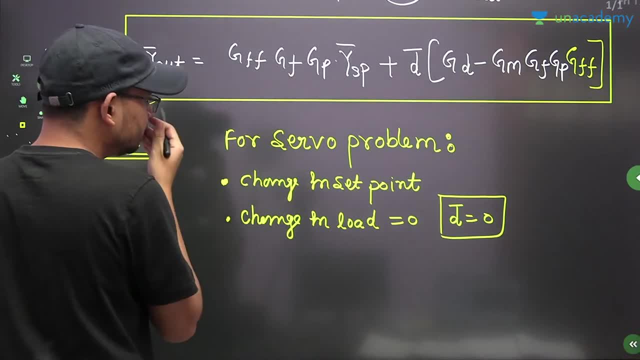 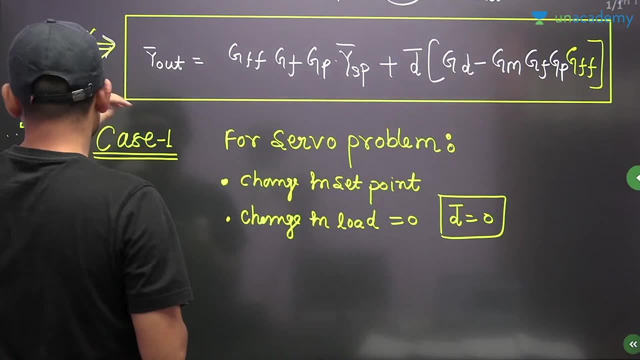 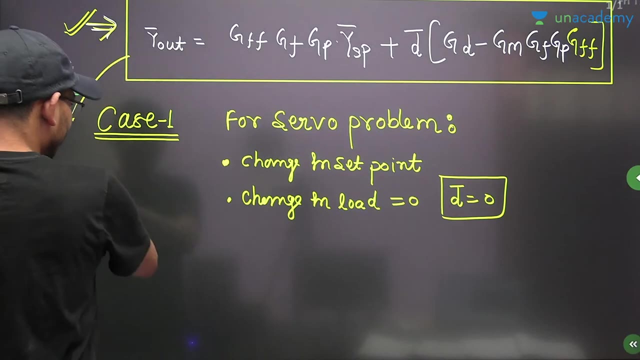 my d var. kya hoga ge ga zero protect ke check. kya hojayega d var produce in servo easily. so y apka y output別 f usfике, exchange f usfiek. don't do that when we receive it as gross stn. 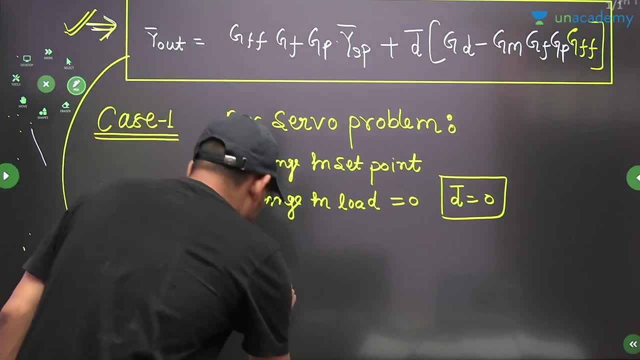 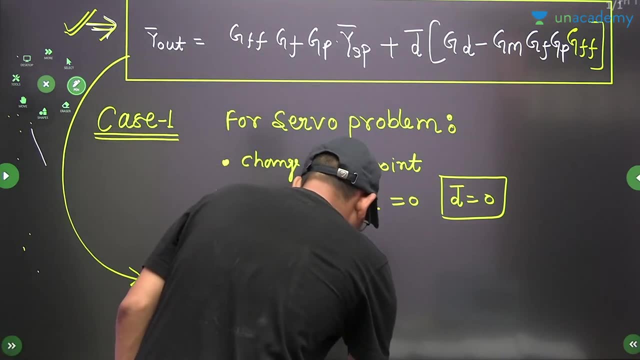 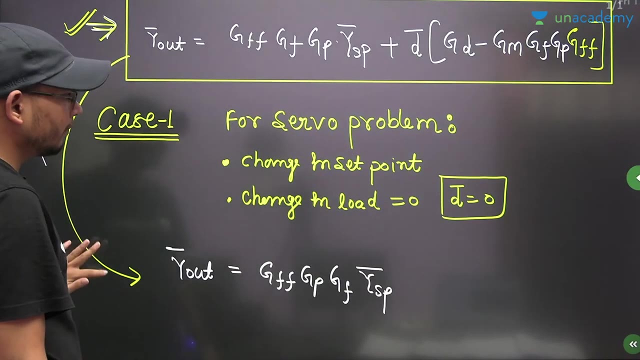 it's called to. kya jayega aapka gff gp tk hai aur gf aur ye kya jayega ysp tk. yaha tak sara log hope so poch rahe hoge. yaha tak sara log muskura ke poch rahe hoge koi samsaya. 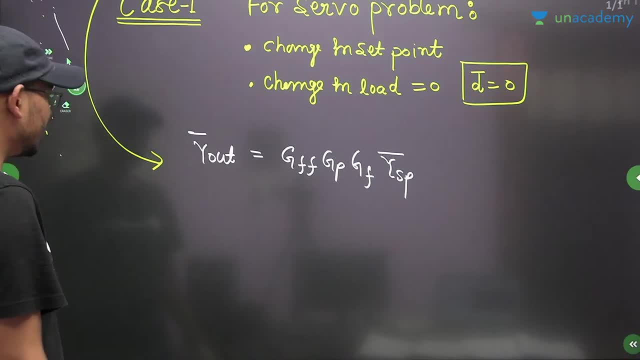 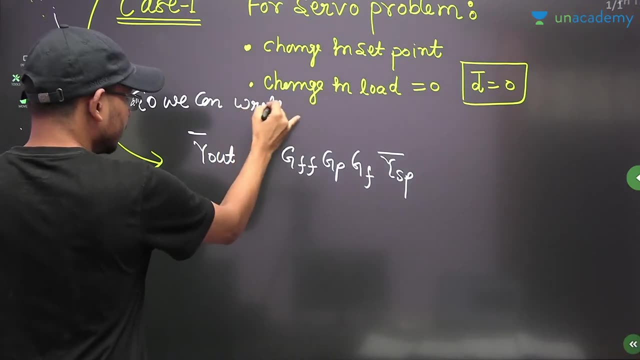 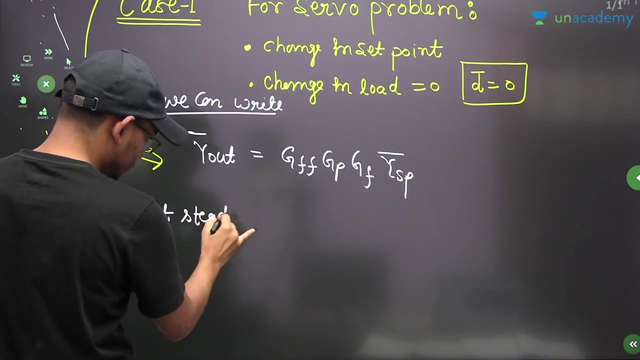 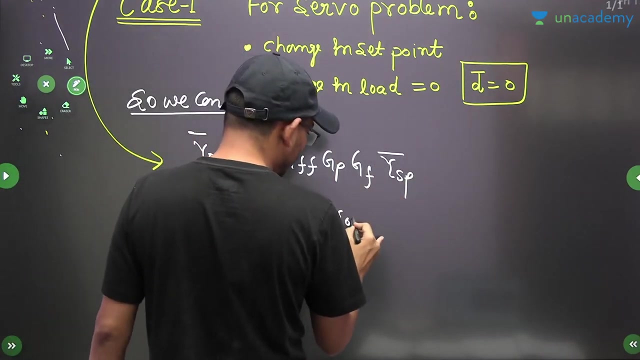 hi nahi, tk yaha tak, so that we can write like that: tk, apn log iss tarike se likh sakte hai at steady state. at steady state, steady state pe kya ho jayega input is equal to output to y. output is equal to kya jayega ysp tk. kya jayega y? output is equal to, output is equal. 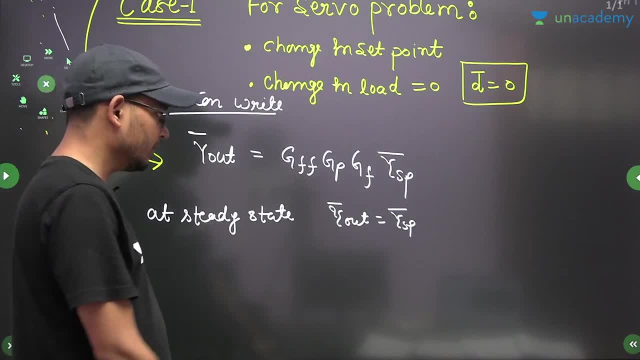 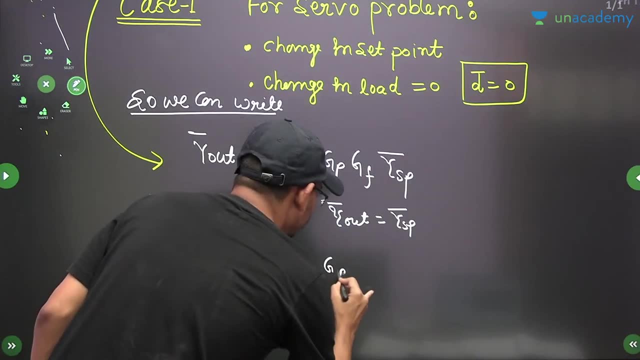 to ysp. input is equal to output. ho jayega kya at steady state to yaha se am log baat karege to kya jayega one is equal to gff. gp into gf right to yaha se ultimate apk objective. 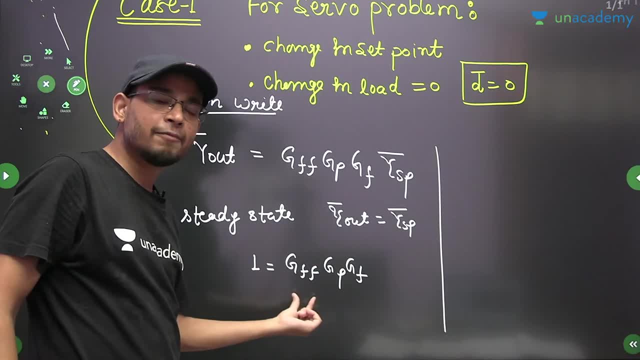 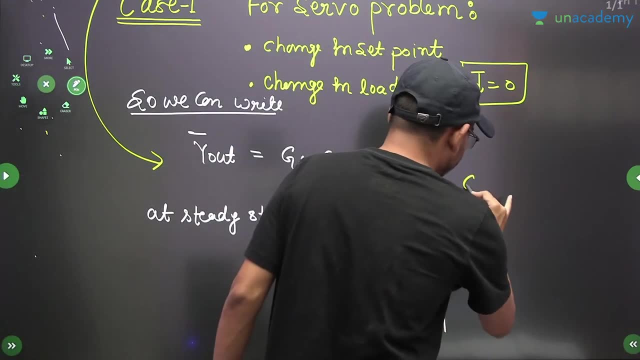 kya tha to calculate the transfer function of the feed forward controller? ok, objective. kya tha to calculate the transfer function of feed forward controller to yaha pe likh denge gff ki jo value hogi vo kitni hogi one upon one upon gp into gf, gp into gf, gp into. 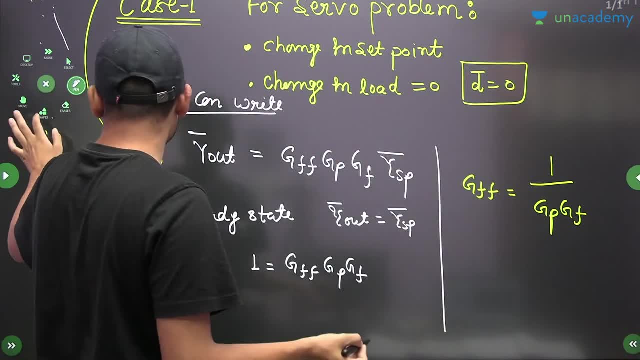 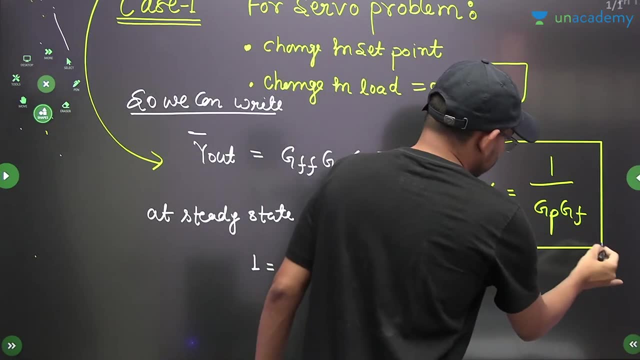 gp into gf. whatever the value is of this, you will keep it. sometimes the value of gf is 1, then its inversely becomes simply 1 upon gp. simply becomes 1 upon gp if your gff is equal to 1,. 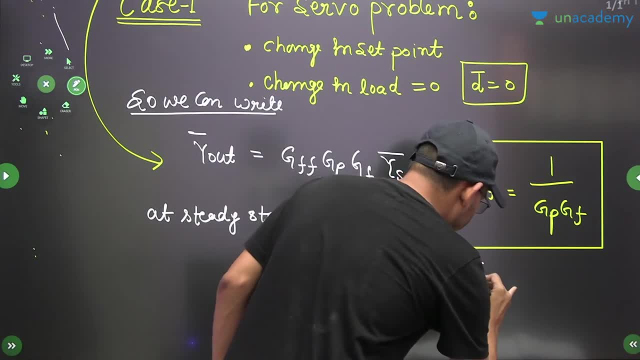 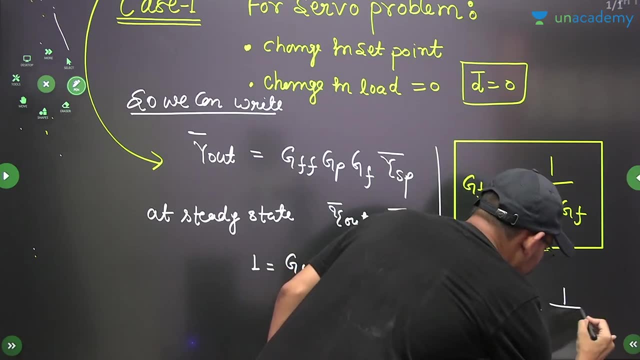 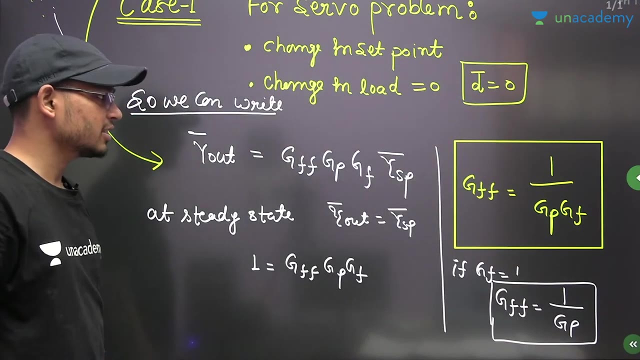 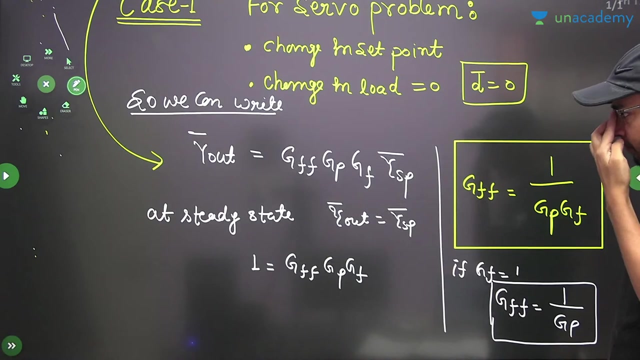 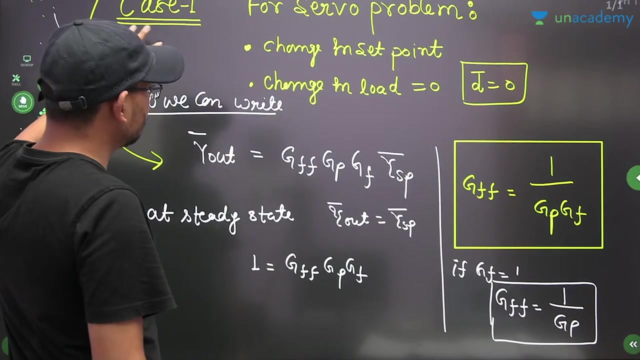 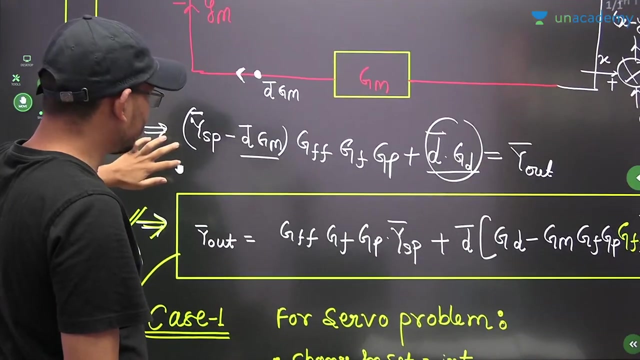 if gf is equal to 1, then the transfer function of your feed forward controller, gff, will be inversely proportional to gp. write these two points first: reach here in a proper way. has gm left here? has gm left here one minute? has gm left here? where was gm in this? where is gm in this? 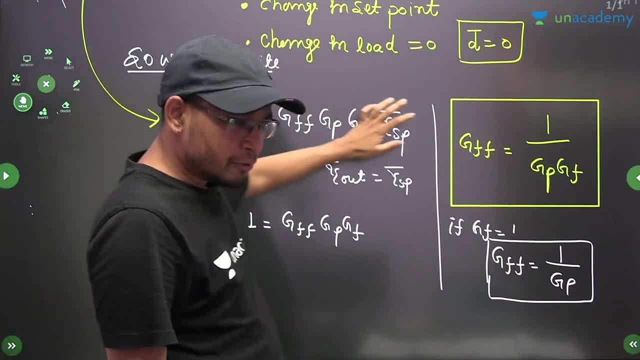 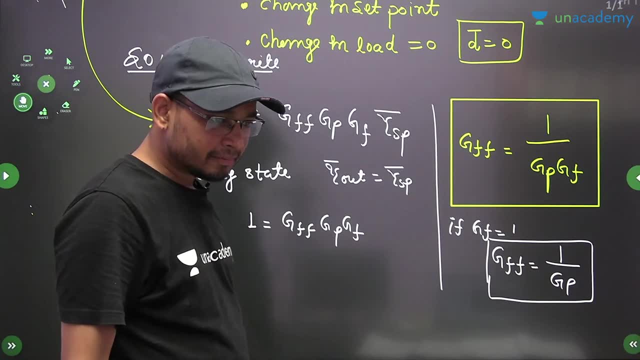 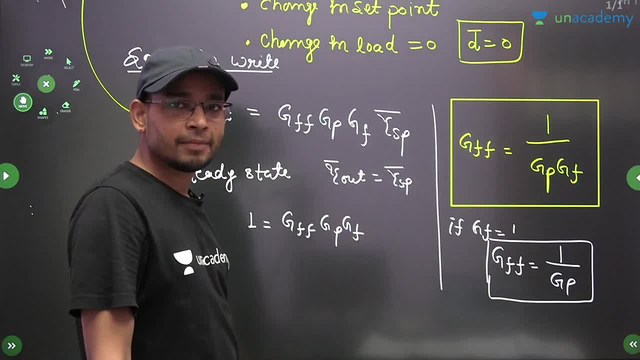 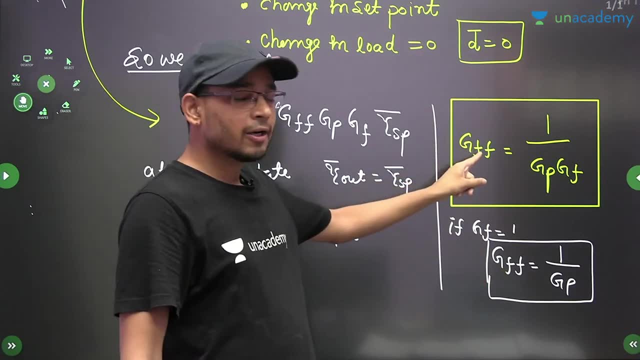 that only you will say: how is your controller? it is a perfect controller. Okay, We will not say�� input equals output, then you will not call the controller as a perfect controller to find out the value of a perfect controller. it means that your process should be operated at the. 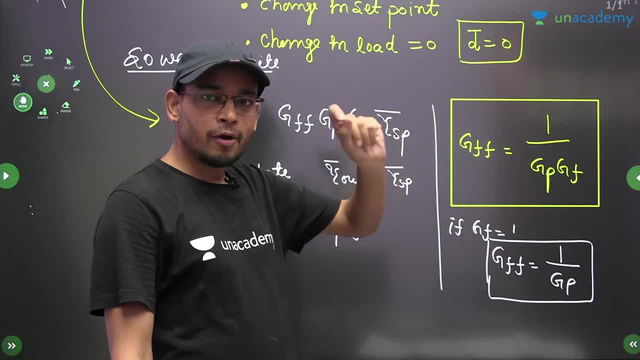 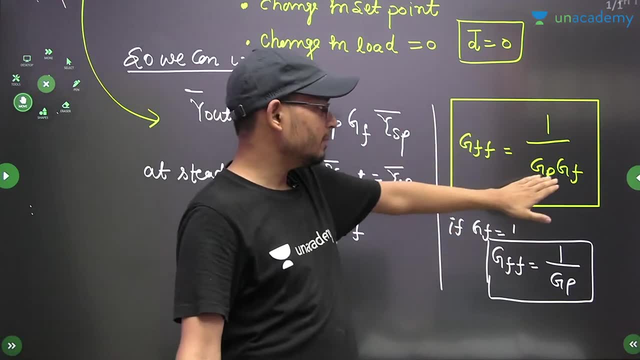 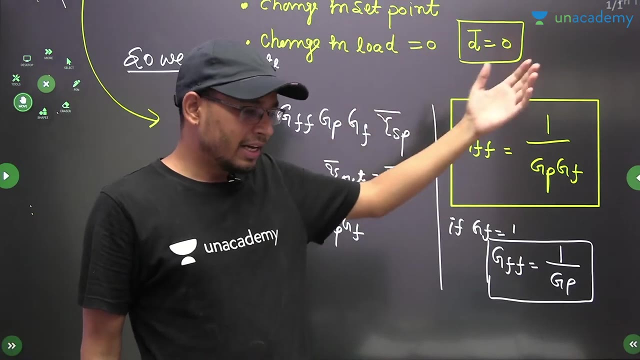 operate at the steady state condition. okay, so if it will operate at the steady state, then only your controller will be perfect controller. so when will you get the value of perfect controller at the steady state? so it will be 1 upon gpgf. yes, it will not come in this, it will come in gf. now, oh brother, you guys are not copying. 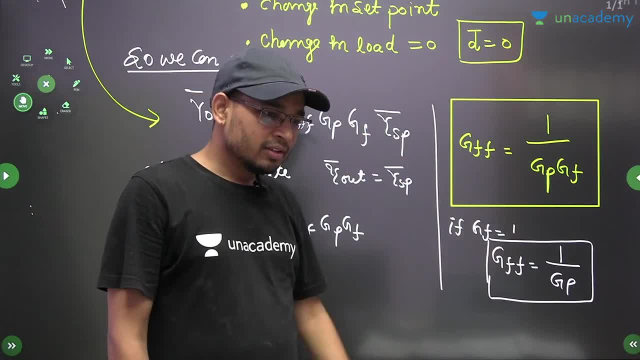 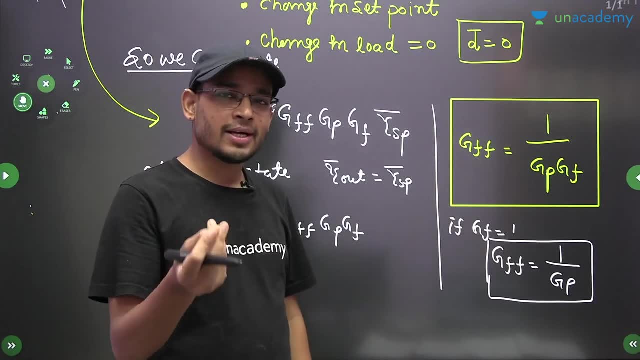 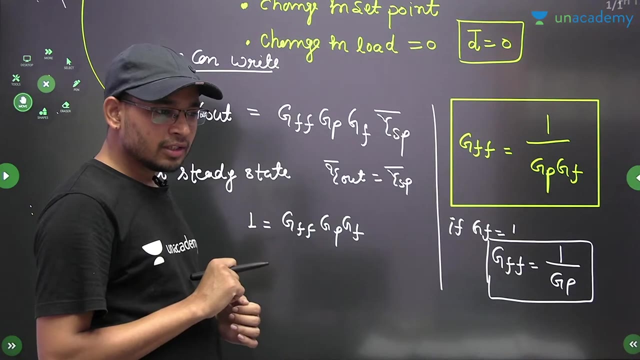 are you not doing end calculation in copying? this means you are not doing calculation in your own hands. in case you are saying that gm did not come in picture, so this means you are not doing calculation from there. this is written for servo. this is problem. 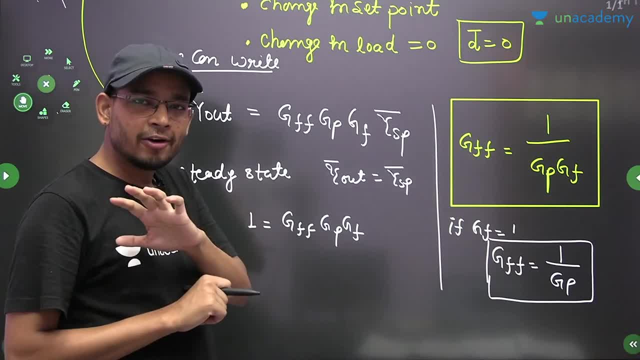 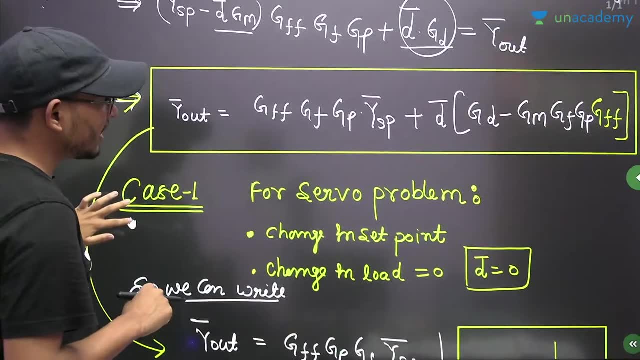 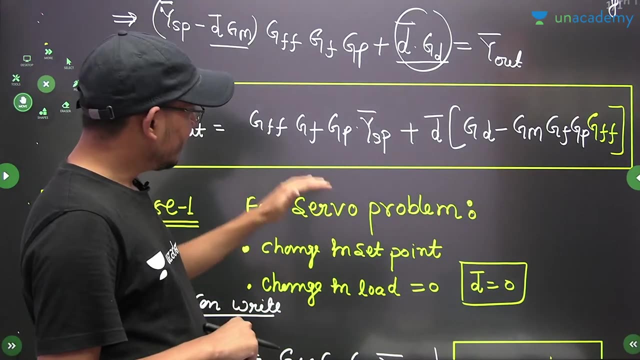 only for servo problem. okay, I have not talked about regulatory problem. when you talk about regulatory problem, then only it will come. see, listen carefully. this is written for servo problem. so in servo problem there is no term of the gm. okay here, if gm does not come, then will they forcefully bring gm from yogesh's house. 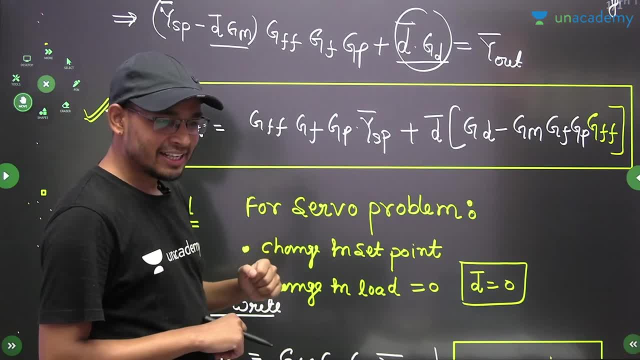 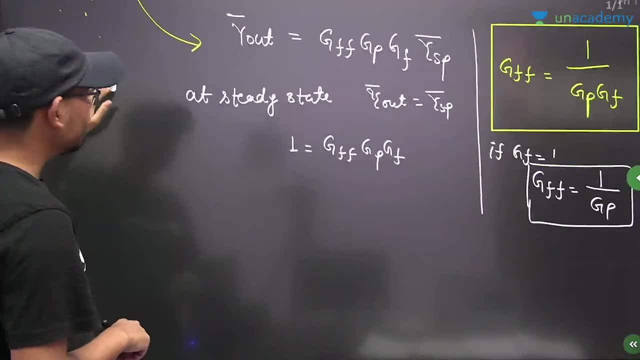 tell me, yogesh, will you give. they will not bring from yogesh's house. then only it will come in the picture, then it will not come here. okay, now case number 1 was this case number 2, let's talk about. 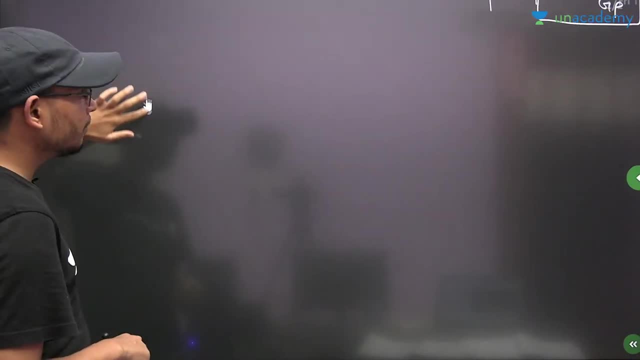 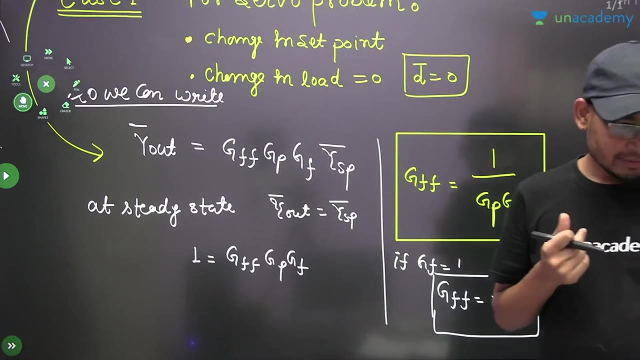 case 2, case 2, till here you guys have written. first tell me this: till here it is done. till here it is done. till here it is done. everyone can write it. till here it is done. yes, this transfer function will depend on loop. 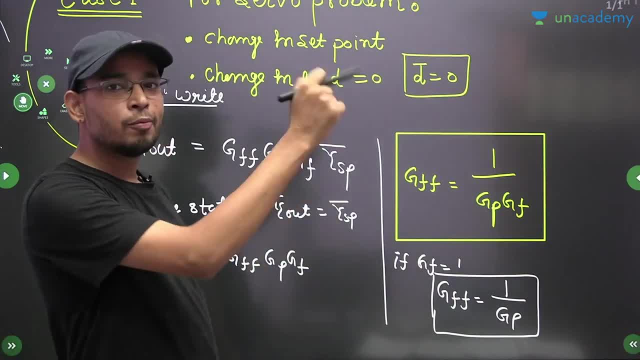 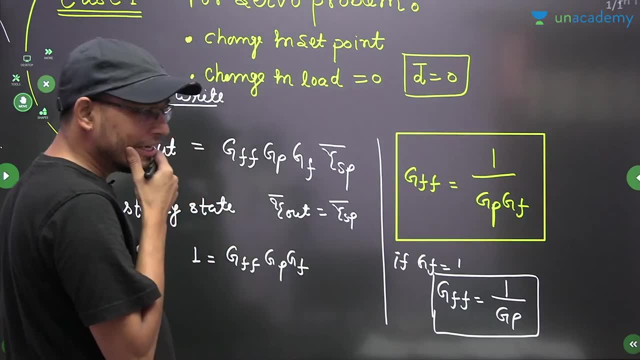 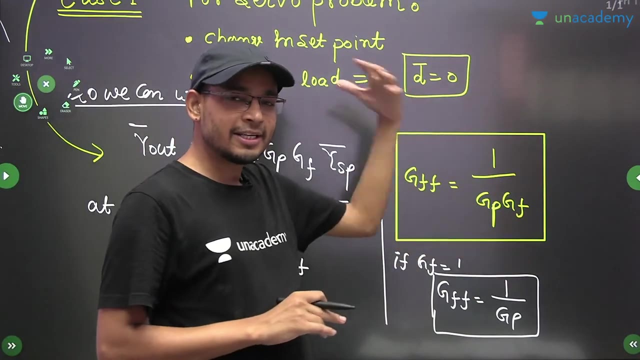 only on which. it will depend on the type of loop you have made. we will make the loop separately in gate. now we will do the question. we will make the loop separately done, okay. okay, we will make the loop and then come. it is not always valid, it depends the system. 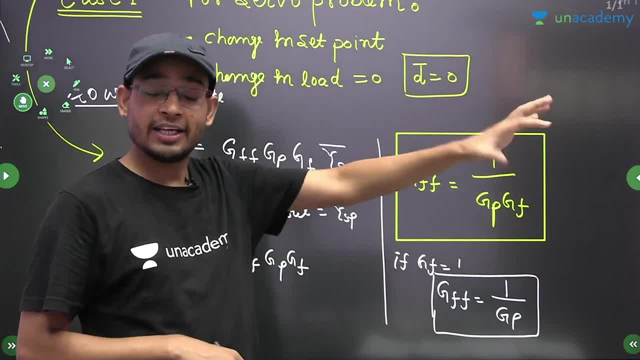 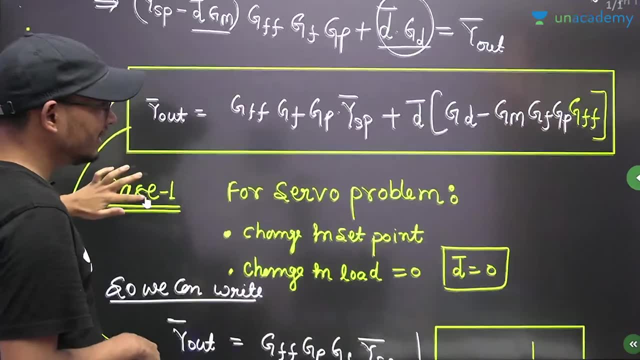 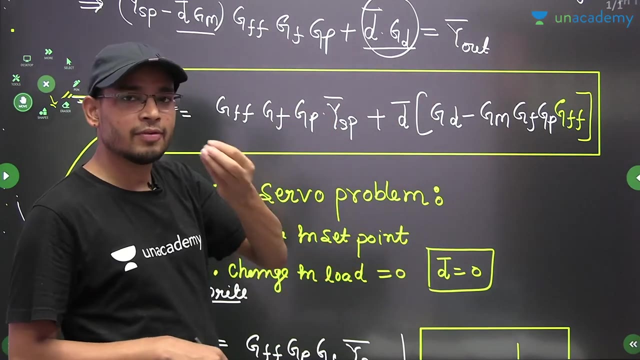 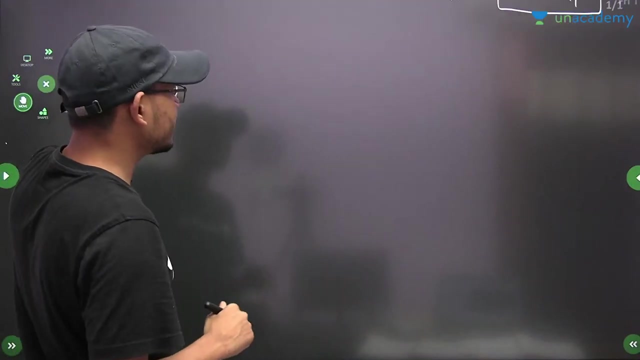 according to that, you have shown it is possible to make your own in the gate that now take it out. then what you have to do is simple: you should know how to write this line. you should know how to write this simple line. okay, you should know how to write the line and if you are asked for a regulatory problem, then you have to follow the procedure. in this way, whatever the value of GF will come, you will come out smiling and come out okay. now, if you will ask a question, then you will understand how things work. come on, so this is completely done. now case number 2 for regulatory problem. 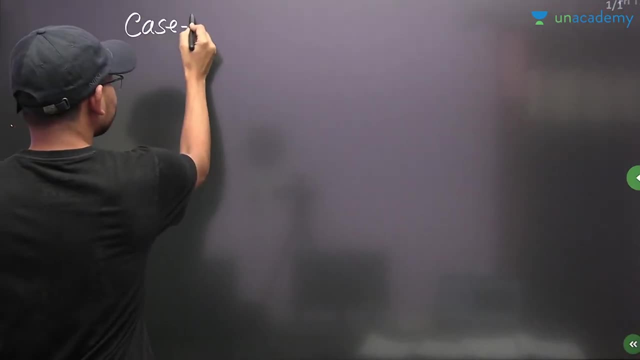 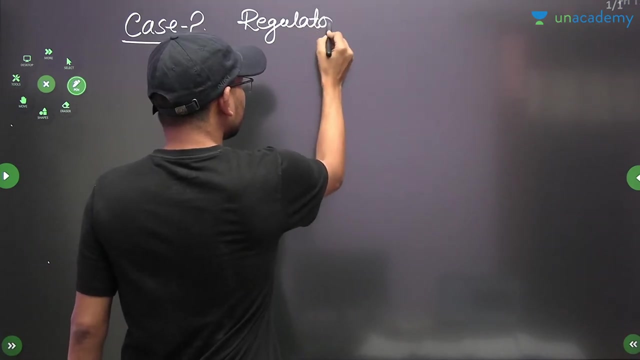 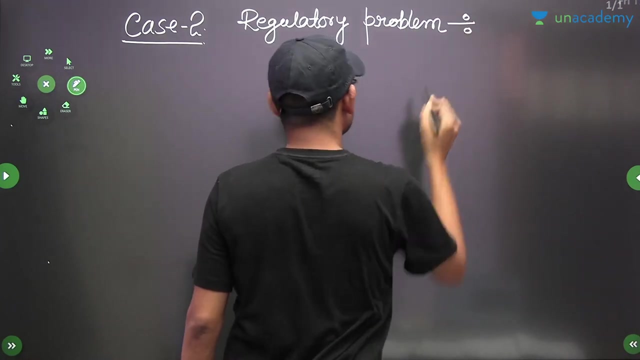 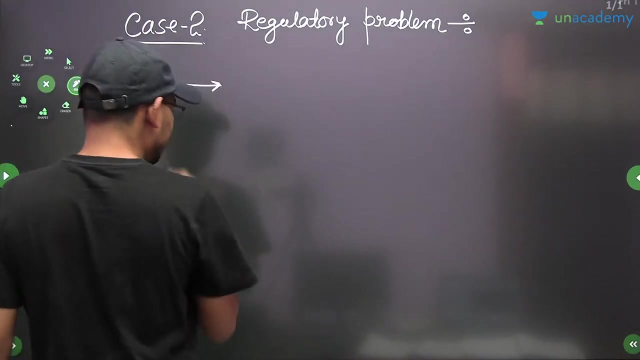 case 2, regulatory problem. problem, regulatory problem. okay, what is a regulatory problem? everyone just tell me by smiling what is a regulatory problem: change in the disturbances? change in the load or disturbances? change in the load or disturbances. 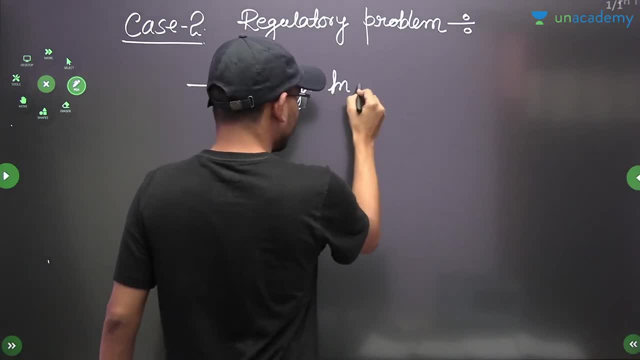 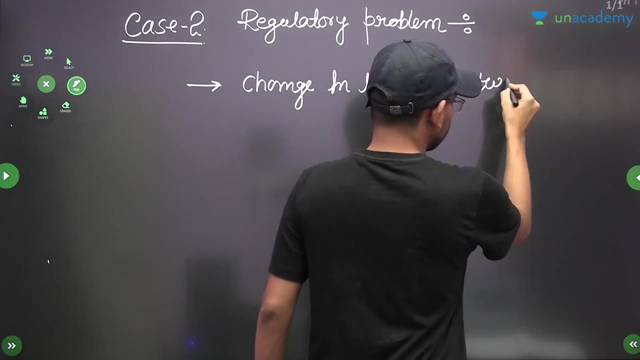 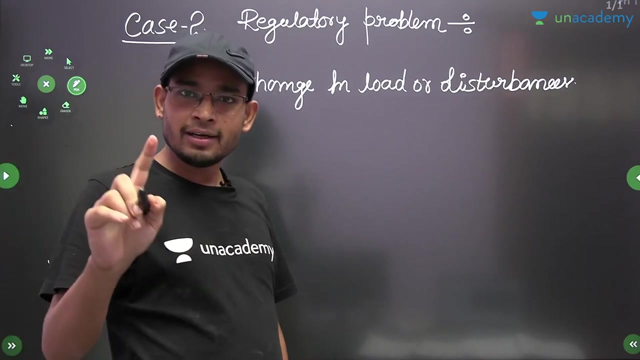 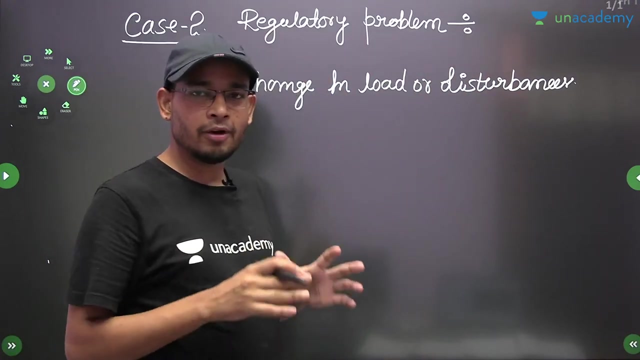 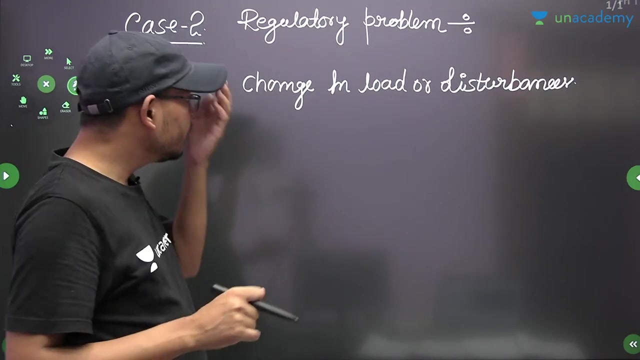 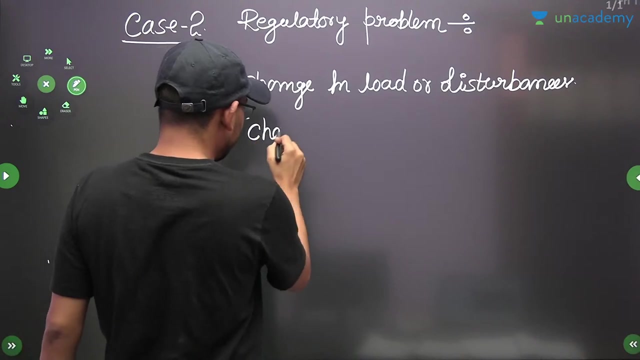 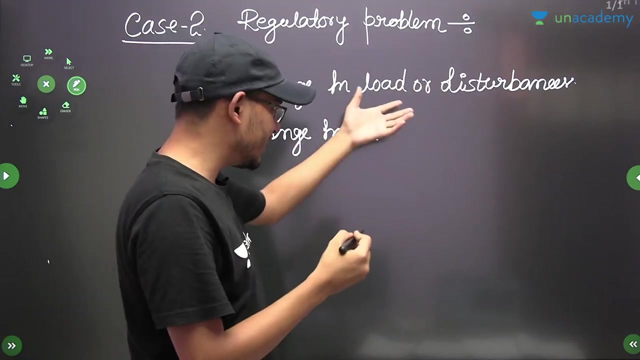 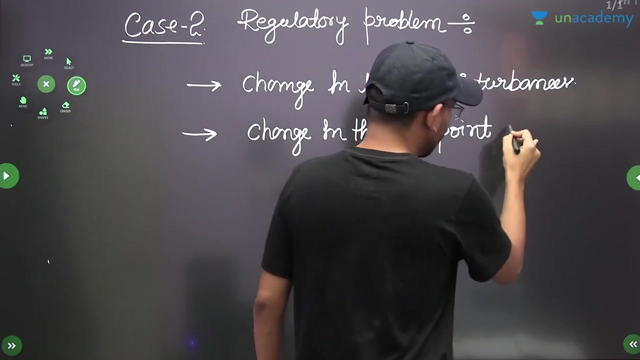 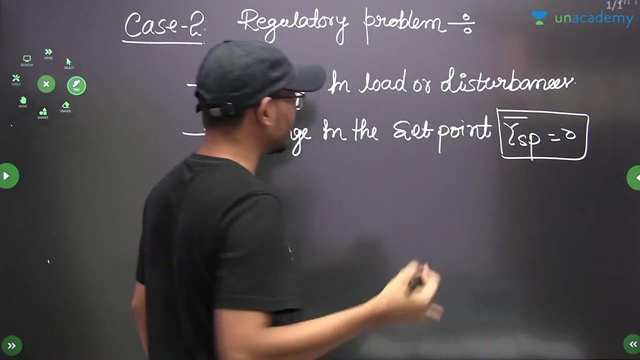 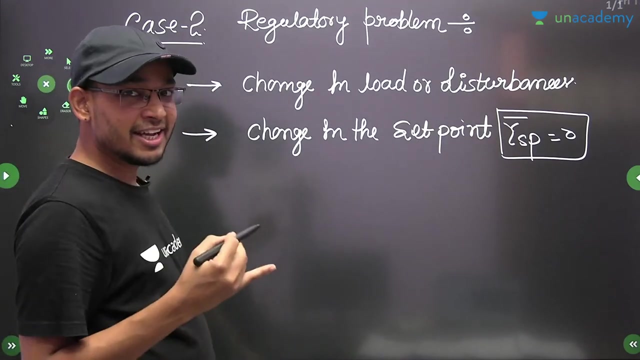 change in load or disturbances. change in the load or disturbances. change in the load or disturbances. change in the load or disturbances. I am getting it written properly because some people have caught the train in the middle. okay, from where the train is going, they are not giving it from there. the station is coming in the middle. 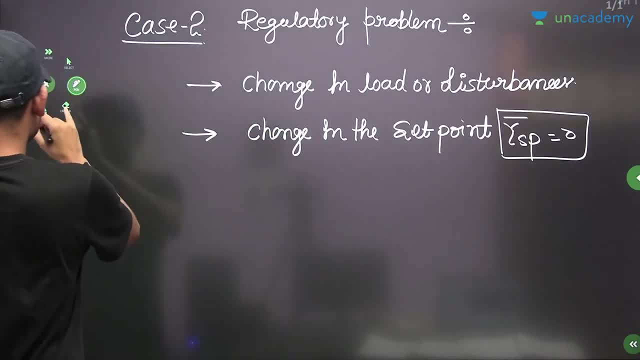 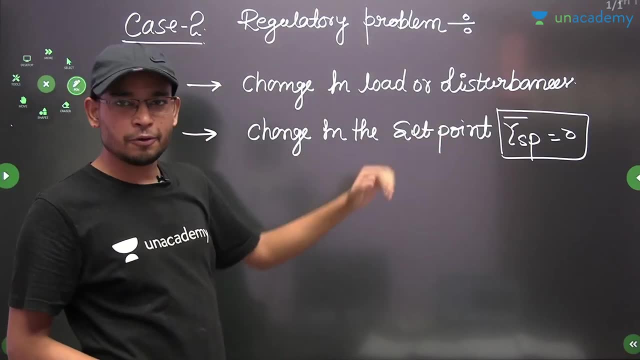 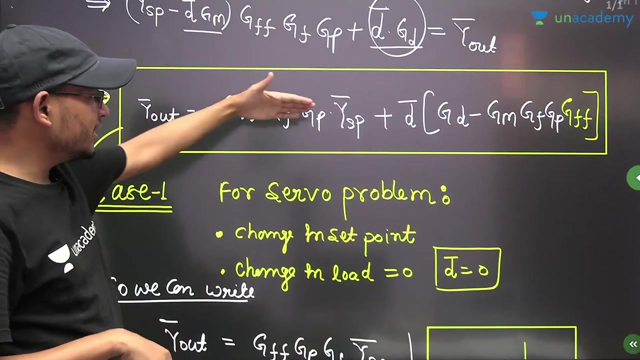 they are climbing there, then the problem is coming now. come on, brother, come again, come again. regulatory problem means you will do YSP zero, then you will do YSP zero. come back to the same equation. then, as soon as you do YSP zero, Guru, if you do YSP zero, then this part will end. 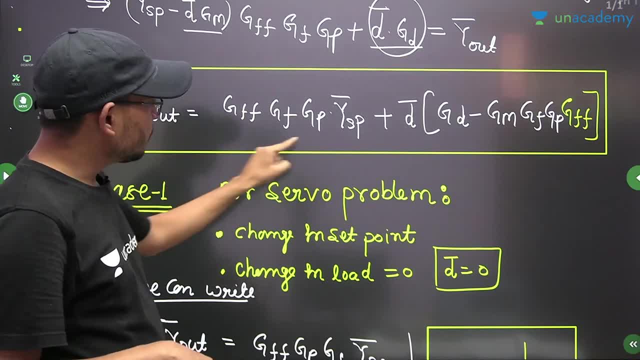 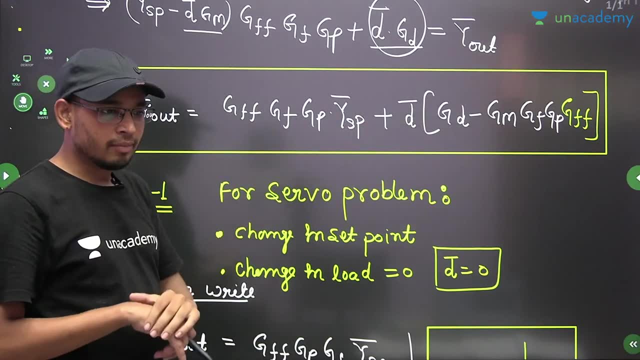 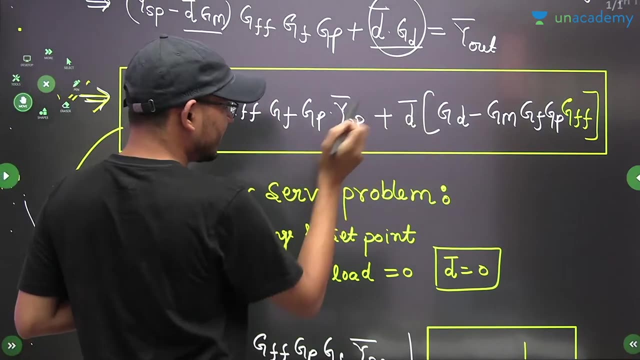 okay, this part will end. then Y output will be equal to all. of you tell us what will this part sustain? that part will end. so as soon as this part ends, that means sustain, that will deal, sustain this one. so it means whose Y output will be equal to this one. now watch very carefully. 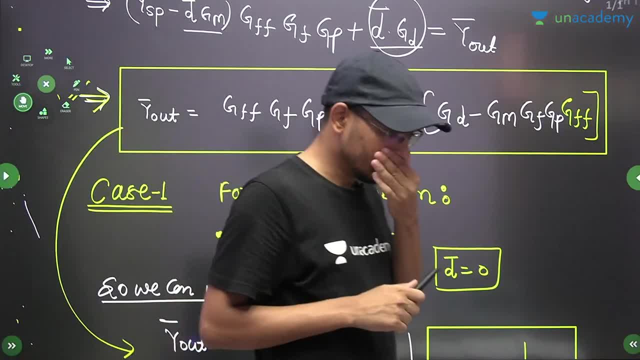 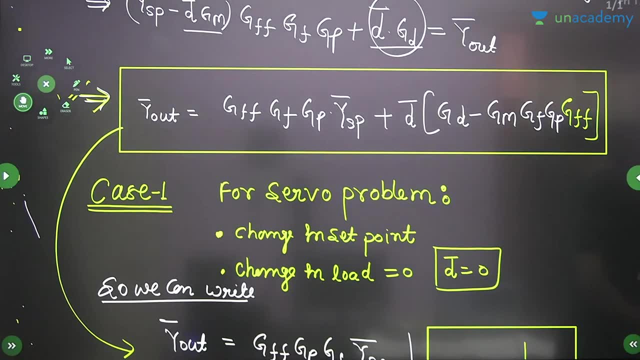 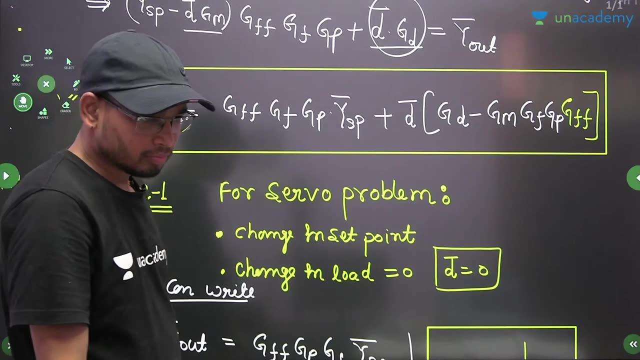 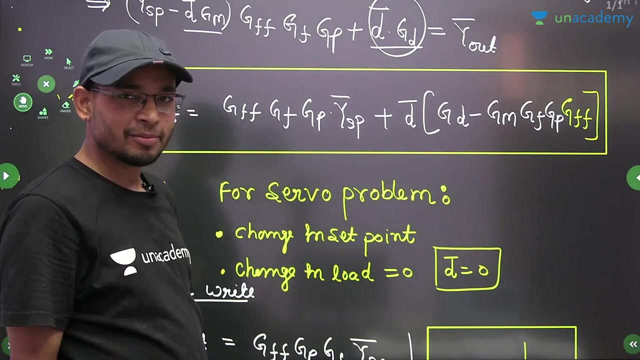 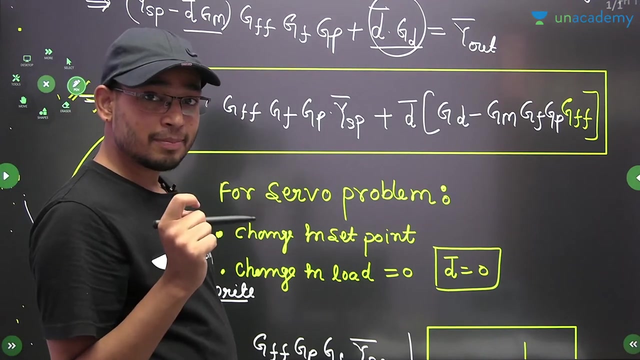 watch carefully here, very carefully. you will have to see another point very carefully Now. you have to understand the concept here. now. what do you have to do? what is your ultimate goal? listen to me very carefully. now. there is a concept here. then care what. 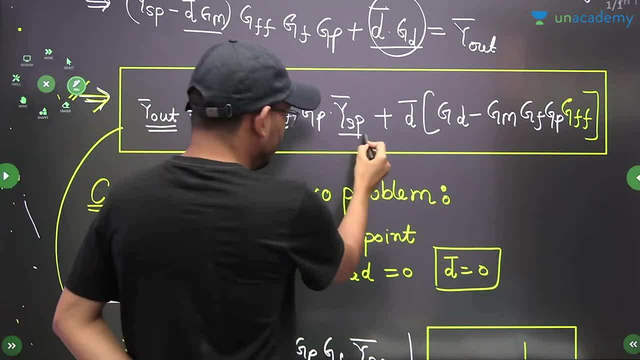 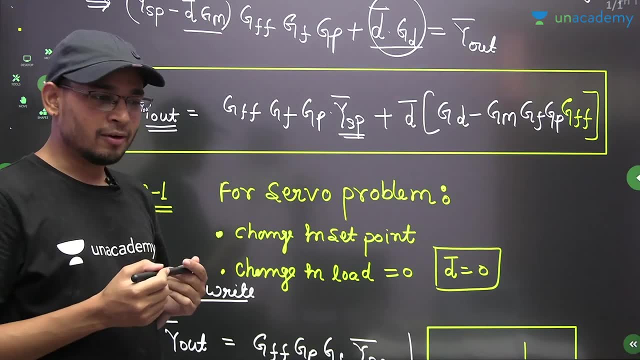 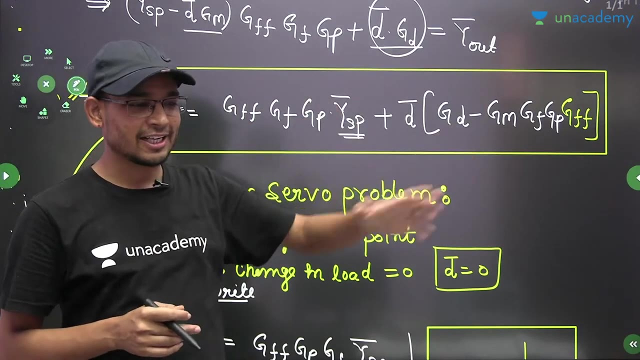 is your goal. if y output is equal to y set point at steady state. if you want y output is equal to y set point, then in what condition? what is the condition you will enjoy? tell me what condition should be there. if output is equal to input, then what condition should? 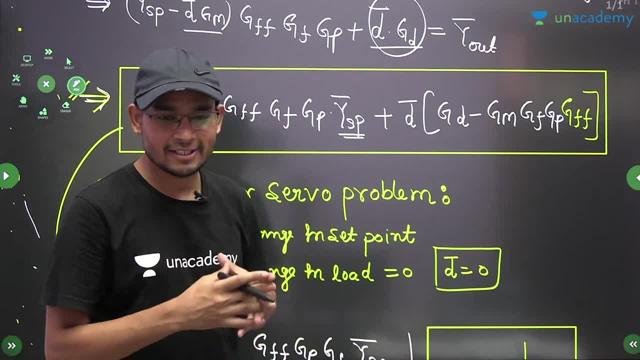 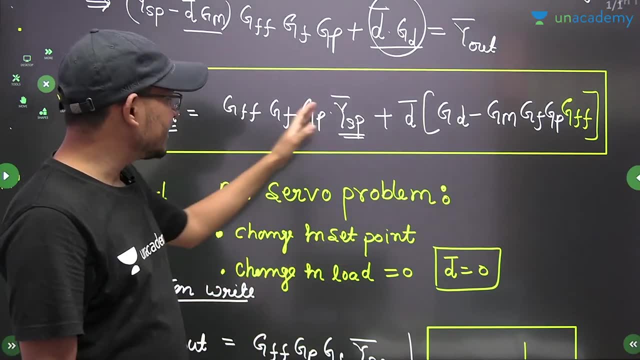 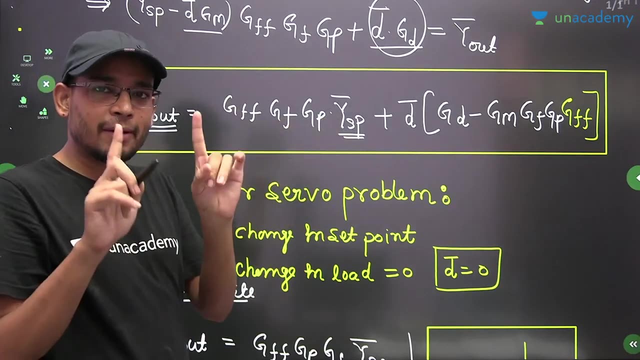 be applied in it for perfect disturbance rejection. tell me, are you able to think a little? I want that output is equal to input at steady state, then what condition should be there? okay, so I want it, bro, because your input is perfect. what is the disturbance rejection? 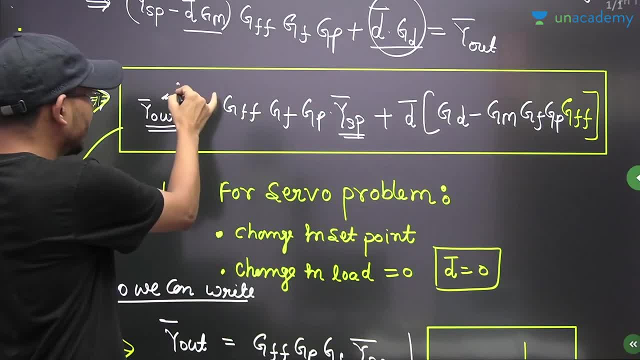 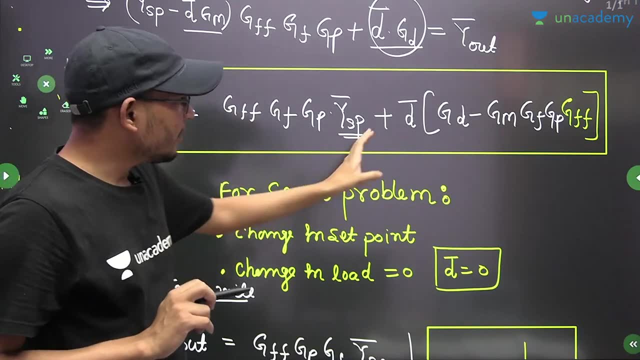 this means ysp is zero. that means you want to make this zero. understand very carefully: ysp is zero, which means you want to make this zero too. when will you be able to make it zero? then this whole term will be zero. then you will be able to make zero means this: 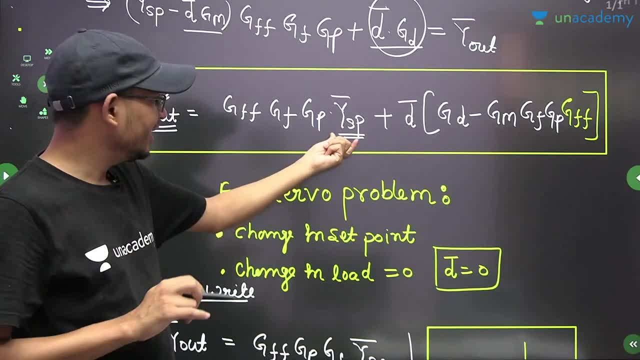 term is zero and you want to attack zero. only input is equal to output, then this term also should be zero. for this term to be zero, this term should be 0, but you have to be able to perform the same process in order to create this pattern. so what you have to do is you. 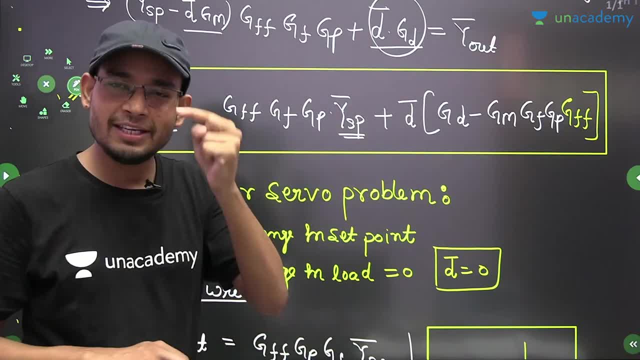 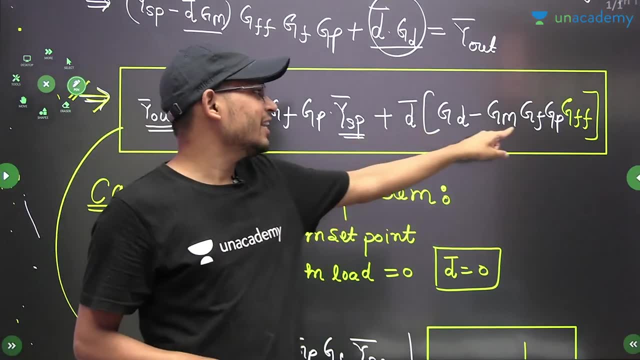 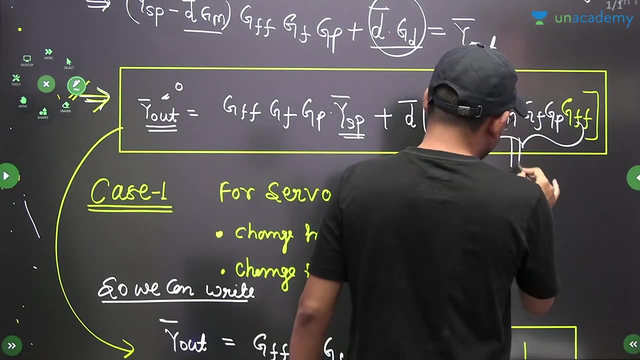 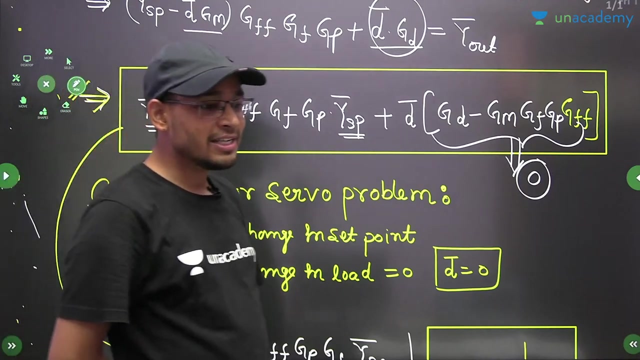 So this term is zero. this term should also be zero. now for this term to be zero, your d bar is not zero because there is a change in the load, so d bar will not be zero. it means whether the inner part will be zero or not, everyone are getting this point. it means this part must be zero. half the people do not understand this. they read it completely. this concept does not come in front. this part must be zero. understand how this happened and you will keep reading this book. you will not understand how this zero happened. 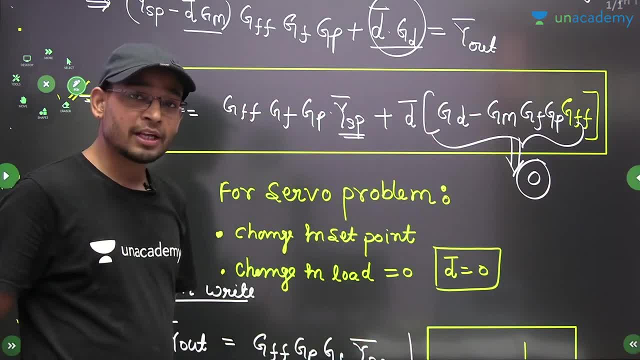 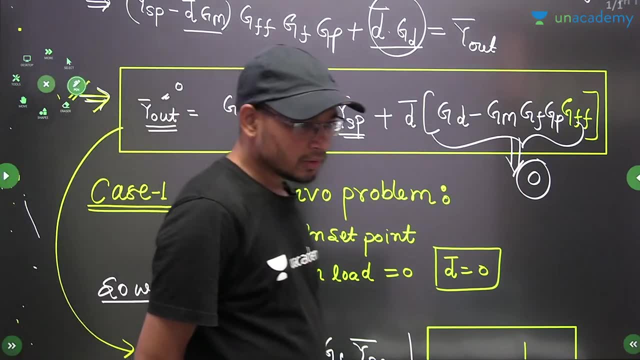 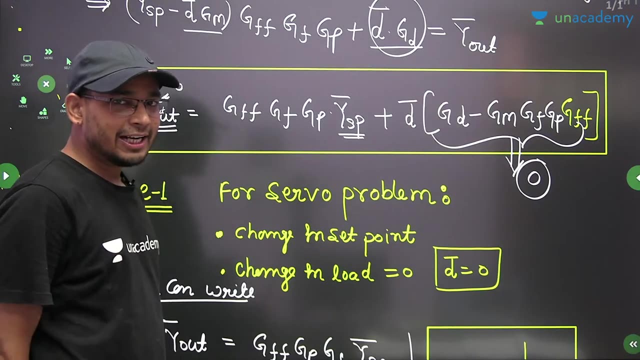 you will just read zero and remember it. I am telling you you will keep reading the book. you will not understand why this zero happened. okay again, please. okay. it means what we want at steady state, input is equal to output. okay, so it means you are not doing anything in the change input. 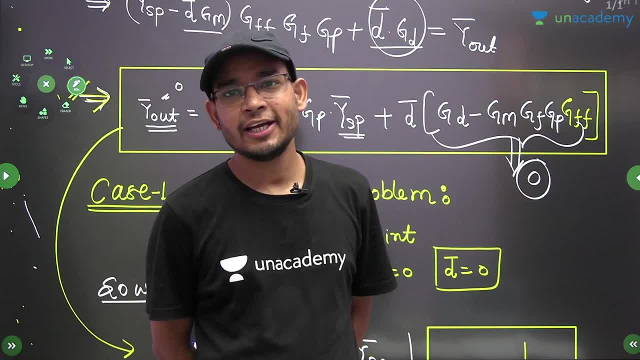 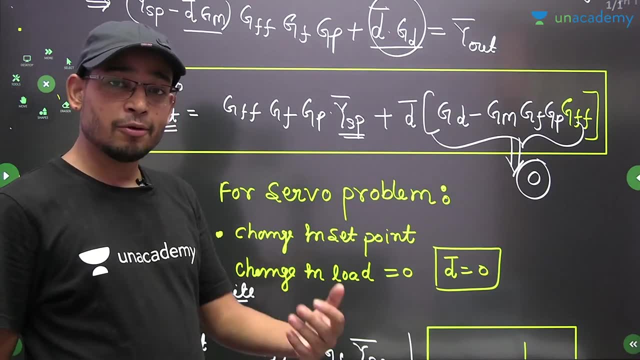 bias is also input. you are not doing anything in the input. it means there should not be any change in the output. okay, then there will be some change in the input, then only your change in the output. it does not happen that the process is running. you have changed something in the input. no, your output has changed. 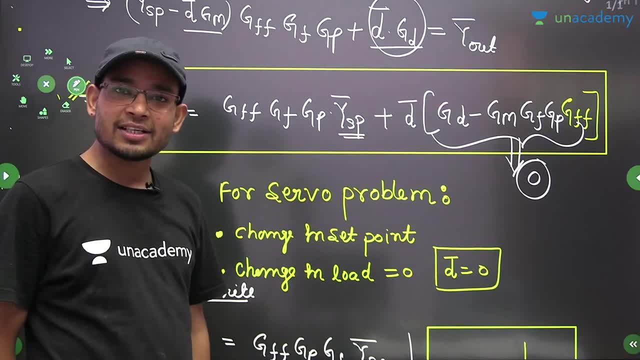 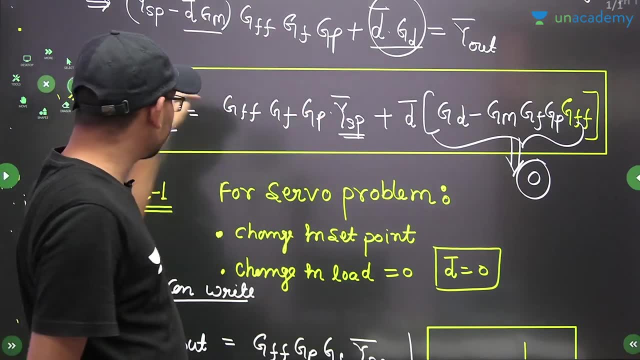 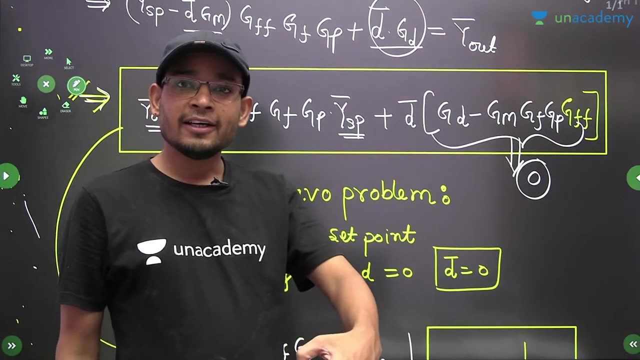 suppose you gave the input 45 degrees centigrade and the output is 50, you do not want this. okay, so you are not changing anything in the input. then there should not be any change in your output. it means ysp must be equal to the y output. it means ysp is zero. why? because you have kept the case perfect. whose perfect disturbances. 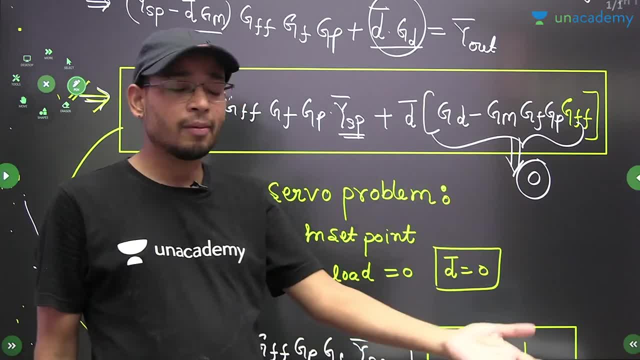 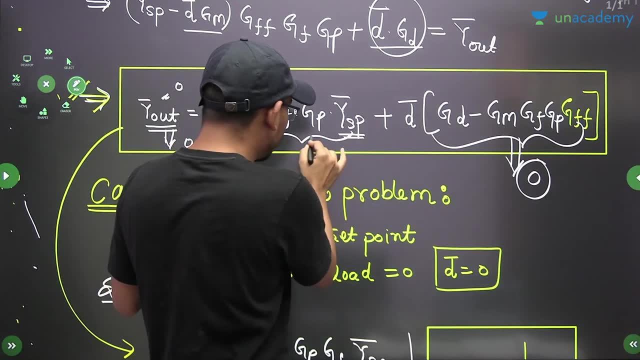 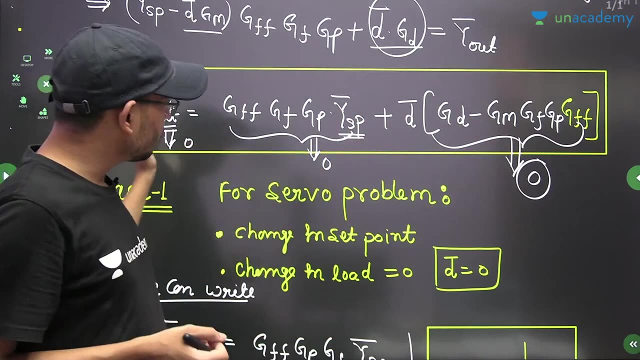 or what. you have regulatory problems. so if there is a regulatory problem, ysp is zero. this means to do this part zero. you should have this part zero and this part should be zero. okay, now, these two parts will be zero only when this part is fully zero. this part is completely zero. now come. 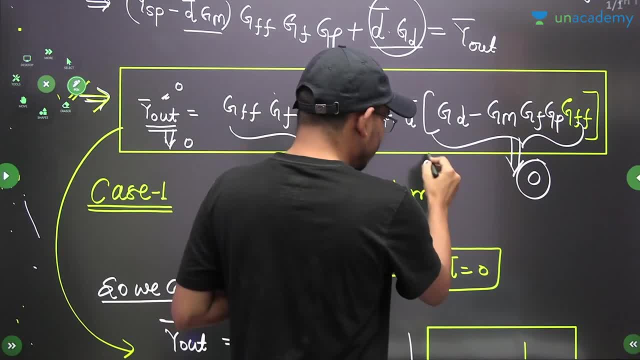 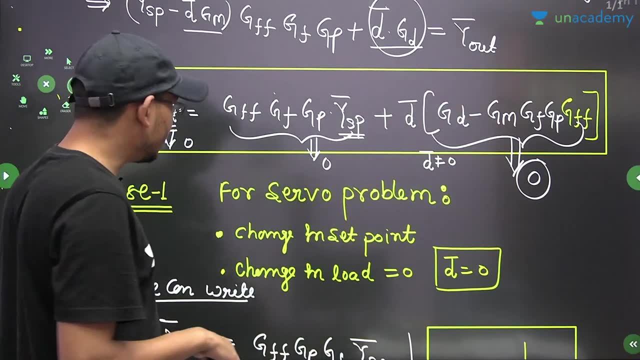 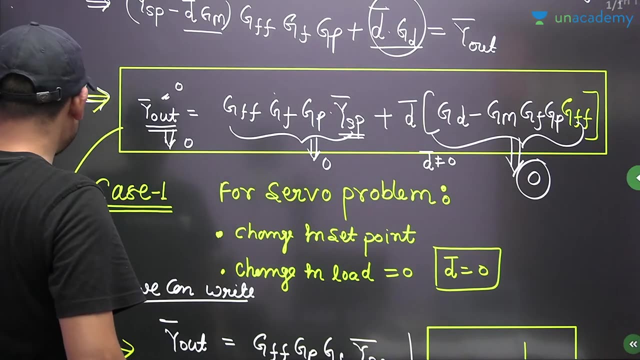 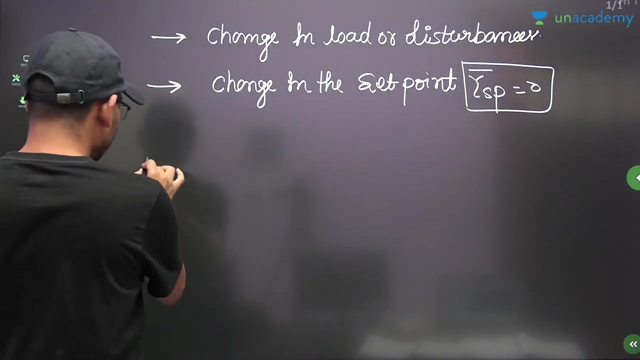 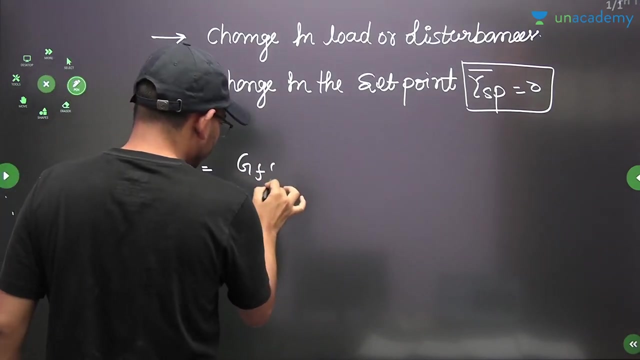 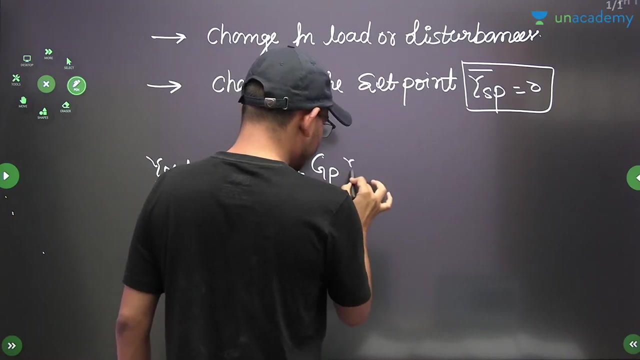 your dvar can never be zero. dvar cannot be equal to zero. this can not be zero. then what is zero? I will write it again here. I will write it properly once again. go down and write the line below. see here where you are writing. I will write it again: y output is equal to what was your y output is equal to what was gff- gf and what was your gp: gp into ysp. 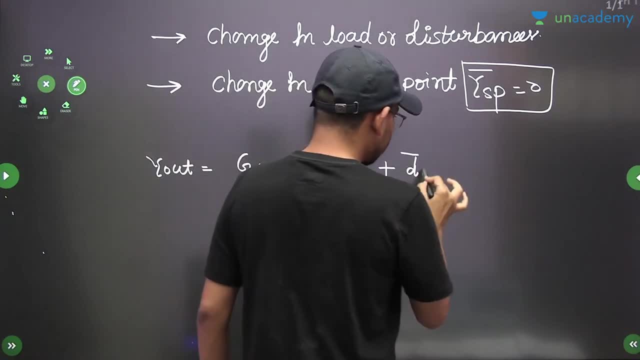 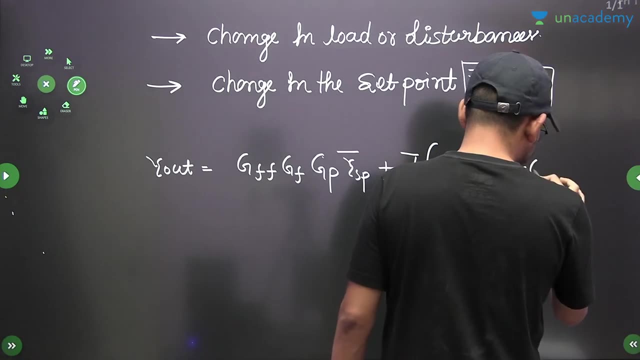 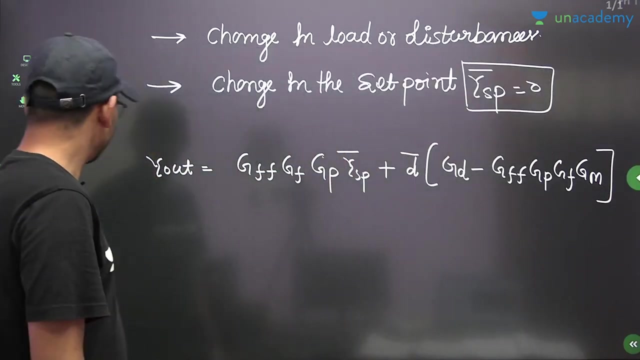 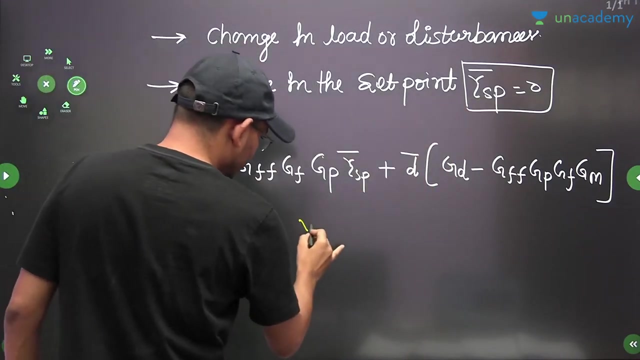 okay, plus d bar. plus d bar, what was your gd, gd minus minus gff, gp, gf and gm? this was it. see, once check everyone. this was it. this was it or not? yes or no, this was it. now. what do we want? that our set point is 0,. so what is your y set point? 0,. 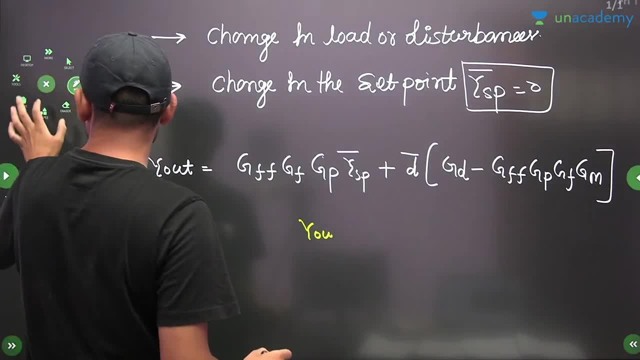 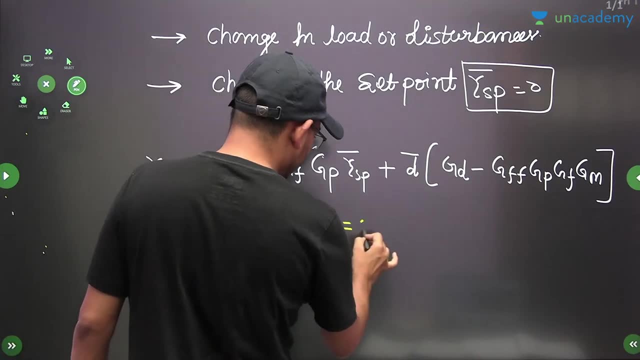 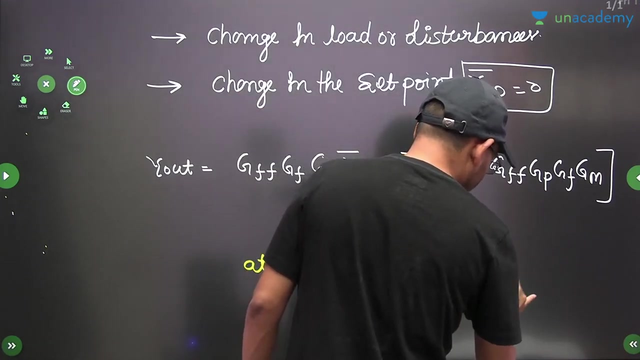 so your output must be at the condition condition of 0,. okay, so what should your output be? it should be 0, so what is your ysp, bro? 0, then then, at steady state, at steady state, at steady state, what will happen? y output, output is equal to ysp. and what should this be? it should be 0, both. so to make this 0, to make this 0, understand very carefully. 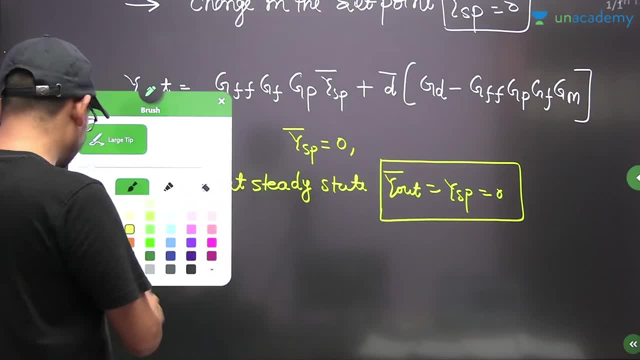 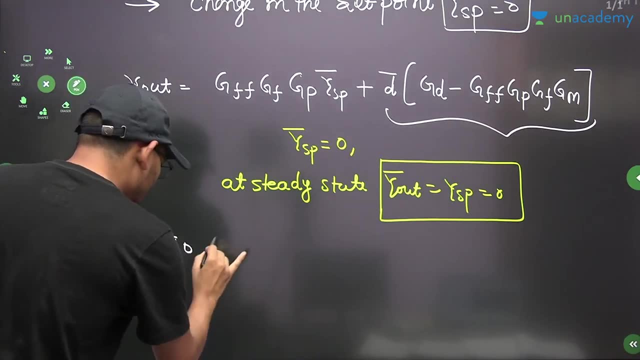 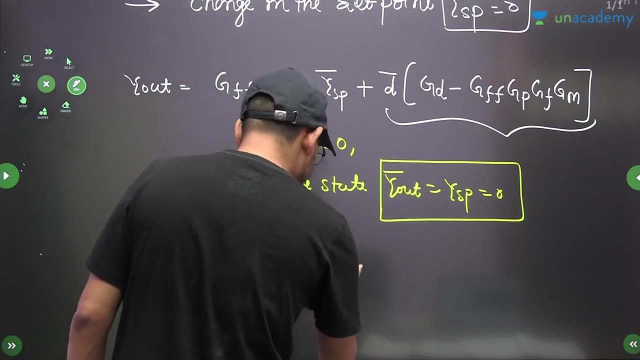 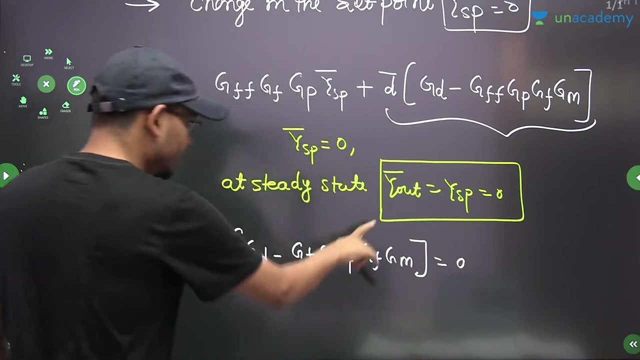 this term should be 0,. you are taking the guarantee of this term, that this one must be 0, this term must be 0, so so d bar, d bar, gd minus minus gff, gff, gp into gf, into gm, must be 0, this should be 0, because of this condition, hold it okay to hold this condition okay. 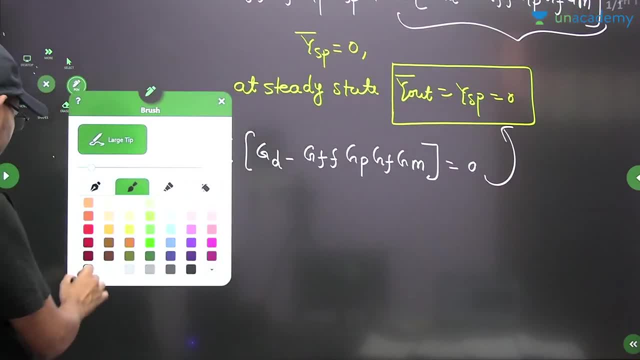 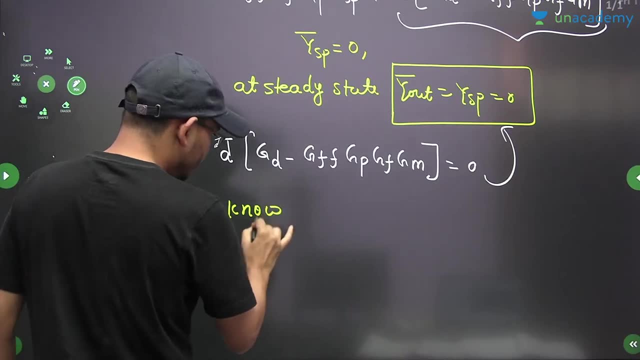 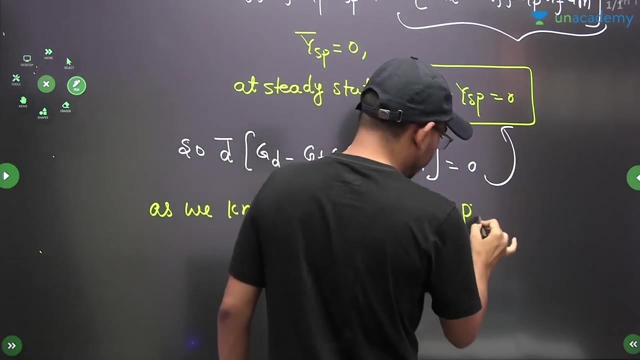 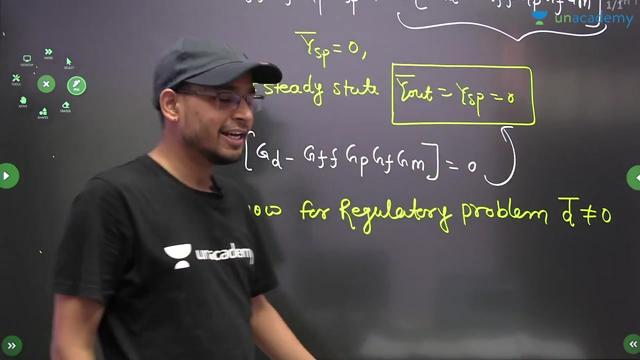 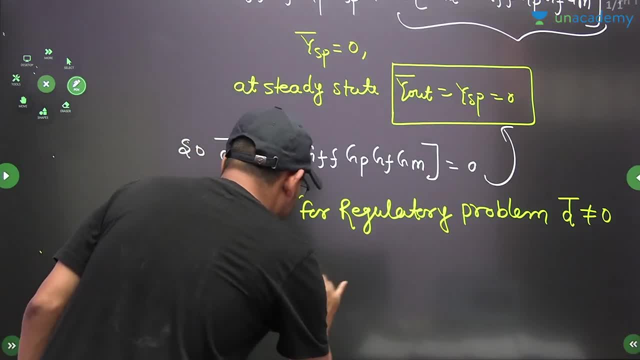 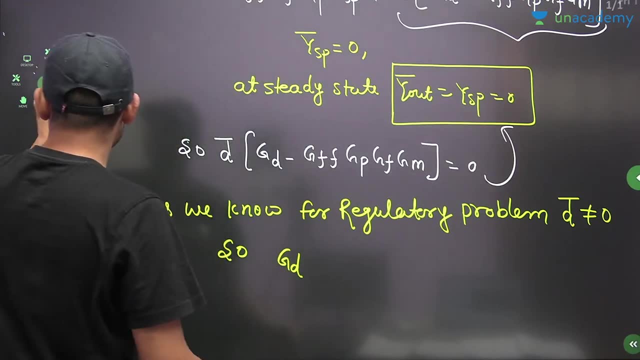 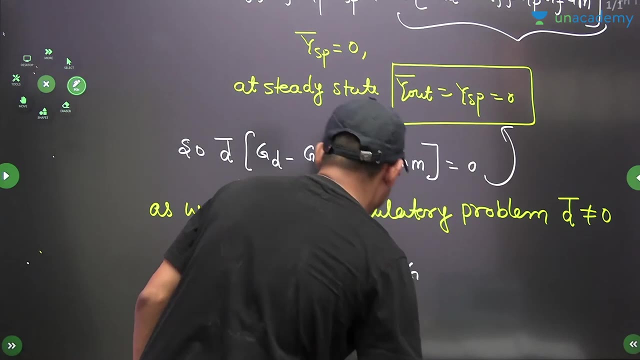 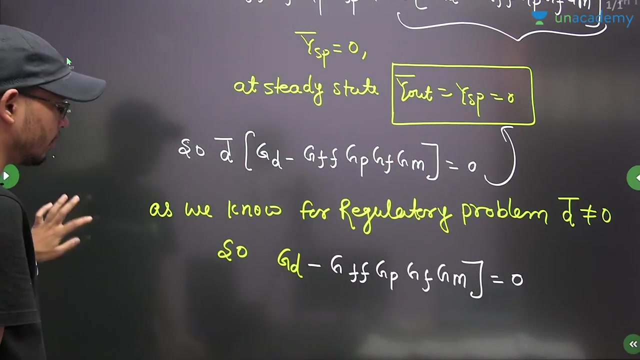 So gd is equal to gf. write it like this: write one more step because people have joined in the middle. if you have written one more step, then it can be wrong. gd minus gf is gp minus gf and gm. keep writing. I am not looking at your comments. I will process the whole process and then I will see your comments. 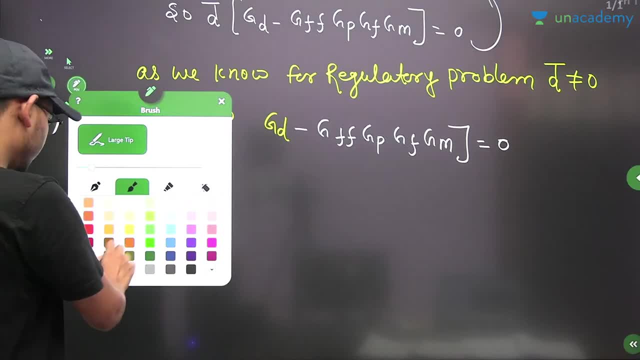 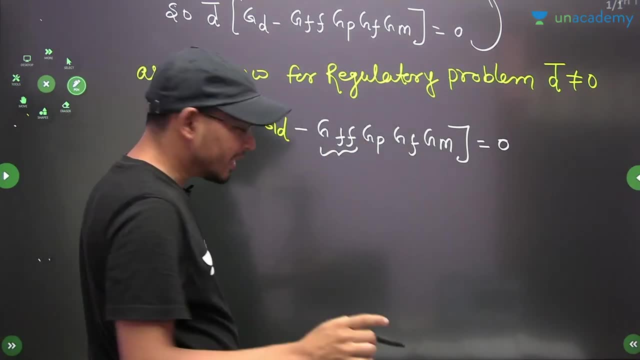 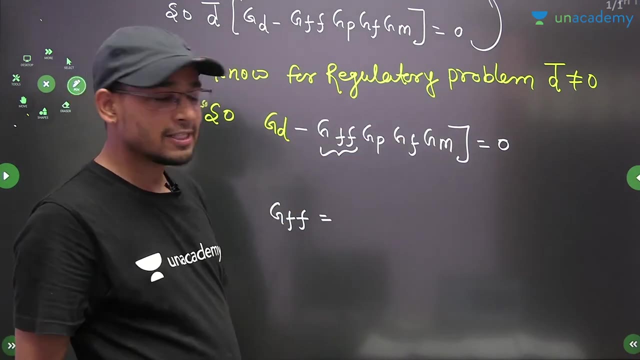 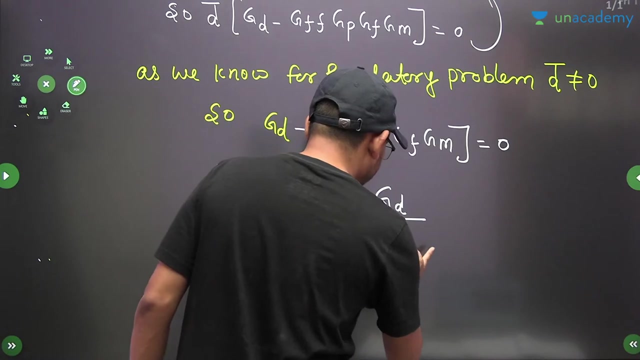 Okay, I will process the whole process and then I will see your comments. I will take you to the final destination first, so this will be our feed forward controller, where the voice should go. so how much gff will come? how much gff will come? tell everyone now, how will we get the value of gff from perfect disturbance, rejection, gd upon gd upon what will come: gp, gf and gm. okay, so this has come. for which your comment. 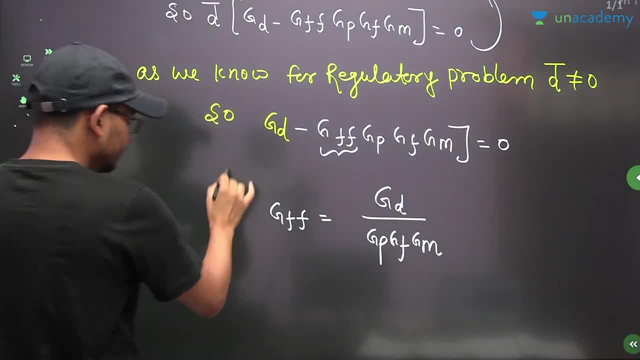 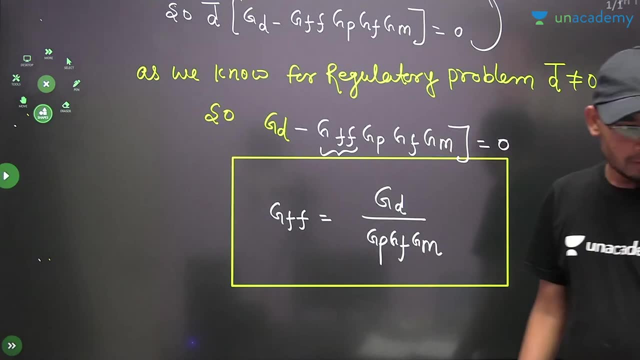 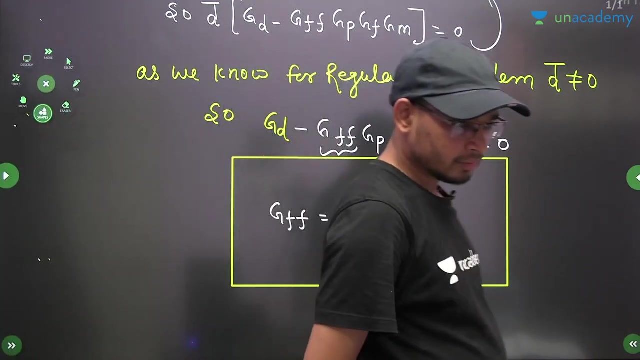 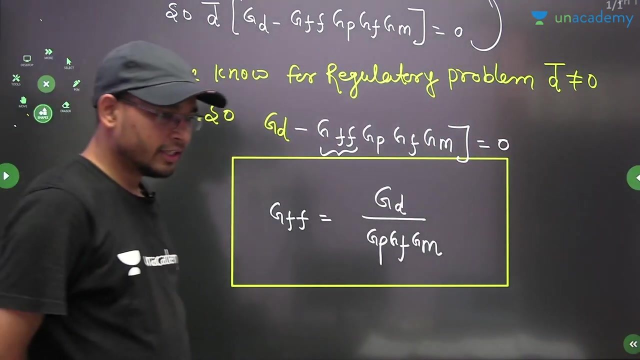 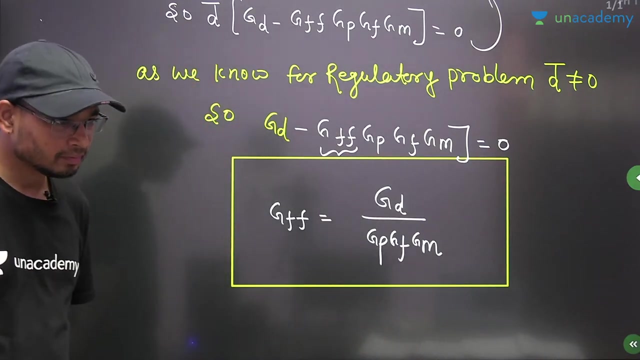 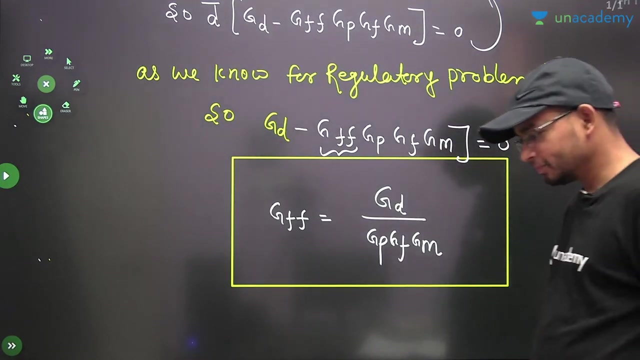 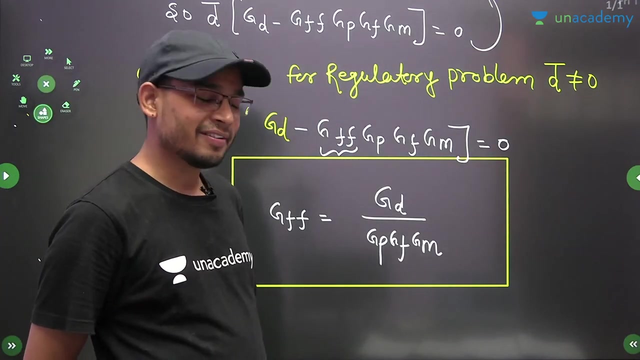 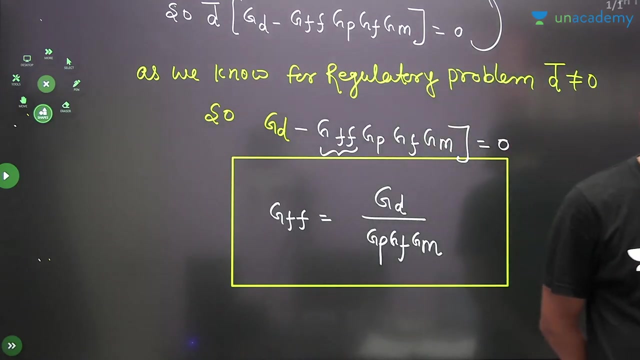 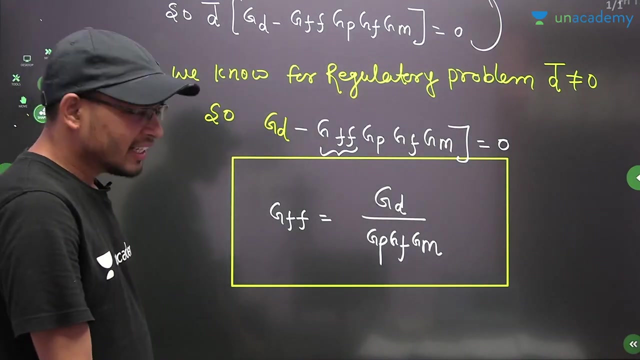 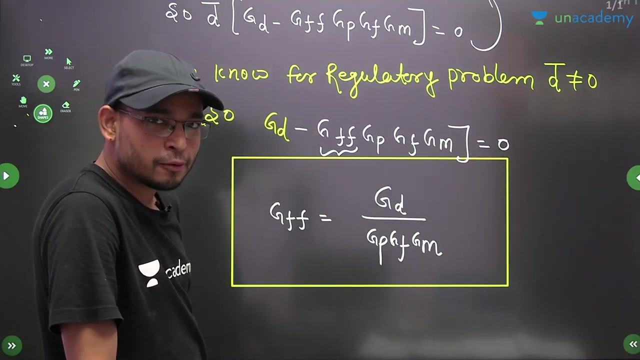 for regulatory problem, sir, yes, for regulatory problem. this is the for regulatory problem till here everyone is able to reach, not in a proper way. yes, Mohit, great explanation, great explanation done. yes, Does anybody else want to comment? 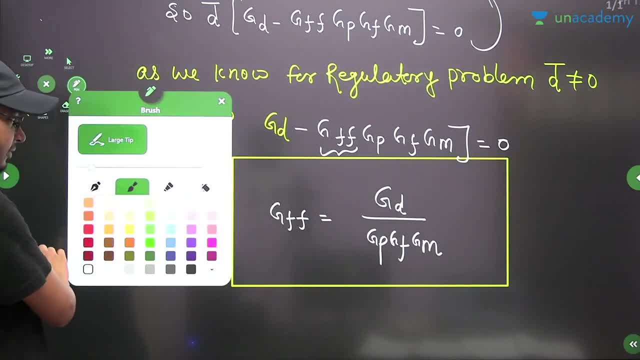 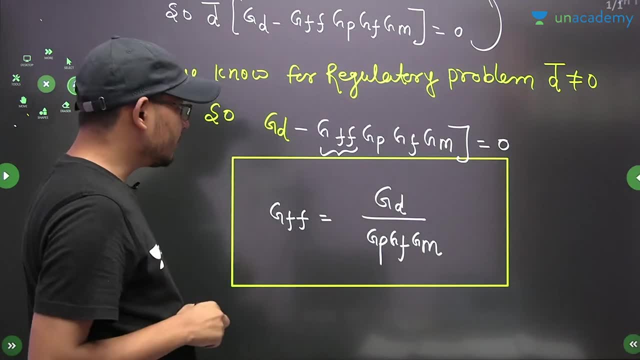 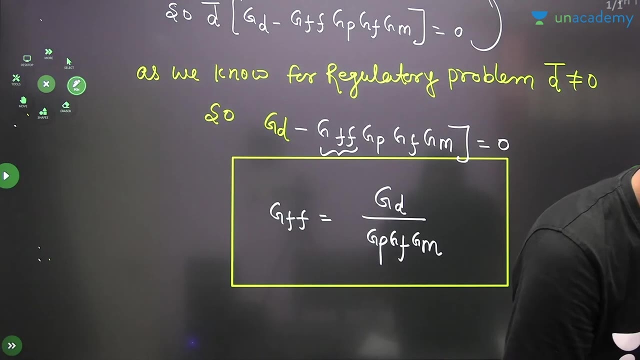 I don't need anymore comment. Should we get the final track again first? Maybe we will get a result that I am honest with you, doctor, because in fact don't give an answer. but be it, you should house the card, take the card or ask him, so it doesn't happen. 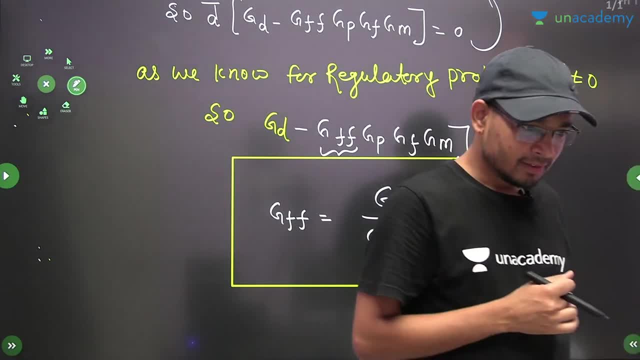 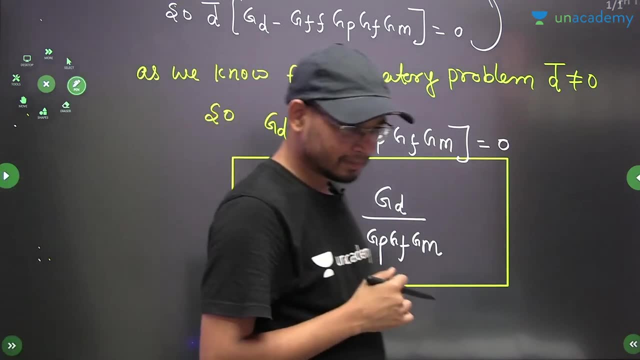 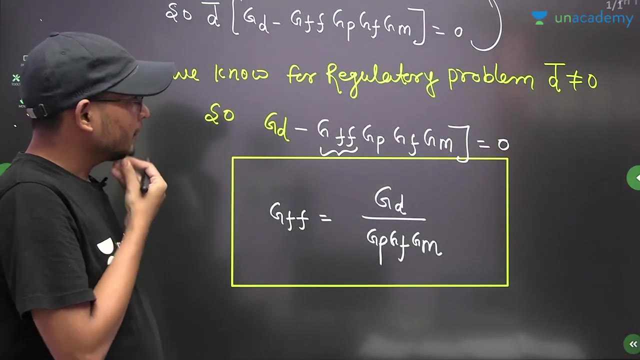 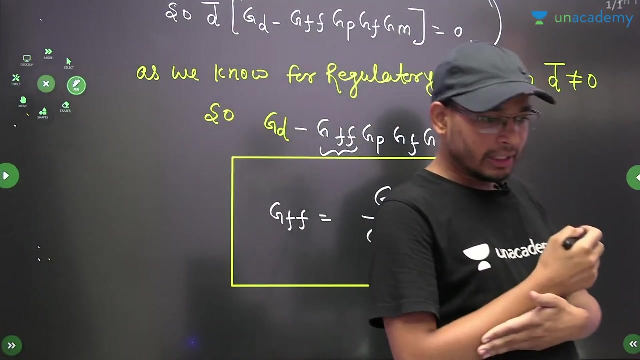 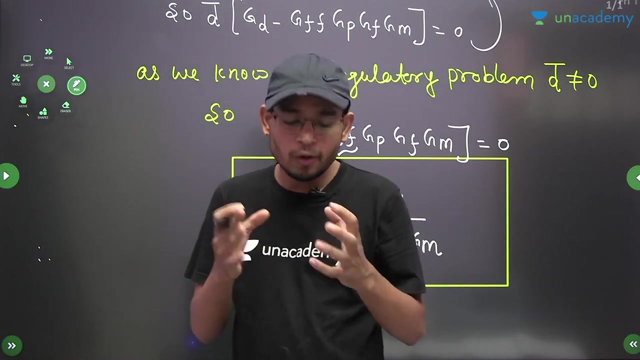 then from now on also, He will recognize you. So this was our EA and you can think about it in one way. in case you have to think a little, in case someone says: see what they call it: whenever there is a change in the load, we call it perfect rejection. 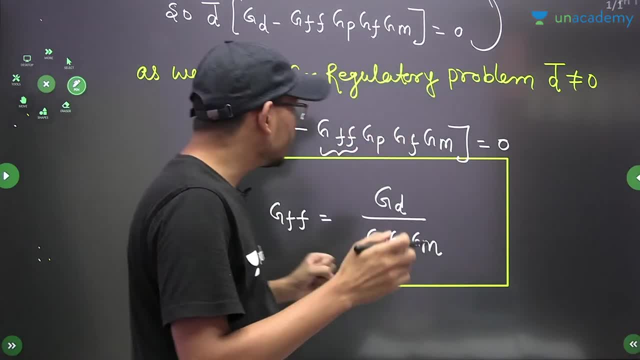 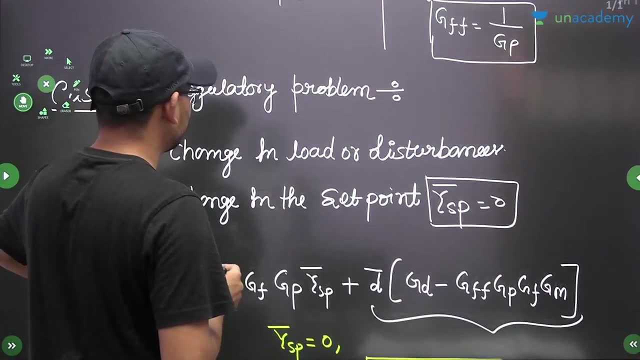 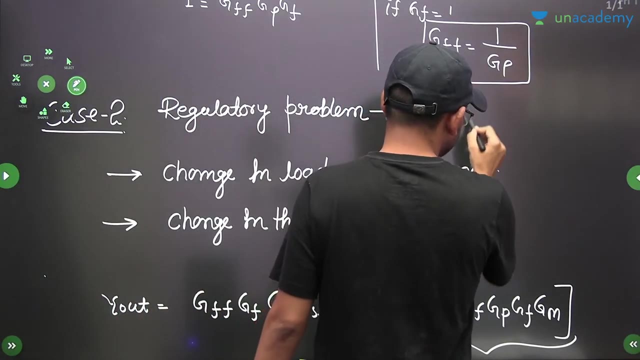 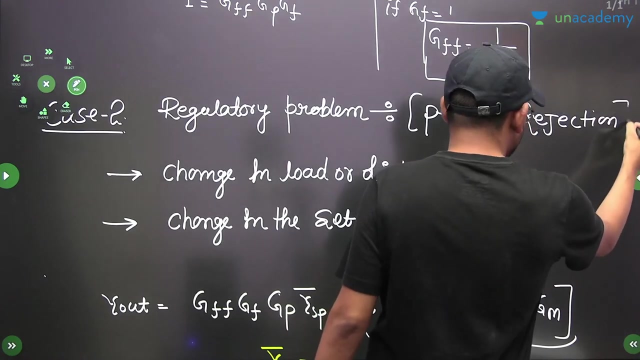 What does this mean? what does perfect rejection mean? See, we call it with another name: perfect rejection. Whenever you talk about regulatory problems, we call it perfect rejection. We also call it perfect rejection, Perfect rejection, Perfect rejection. If you look at the book, there will be a term written there. what will be written? perfect rejection. 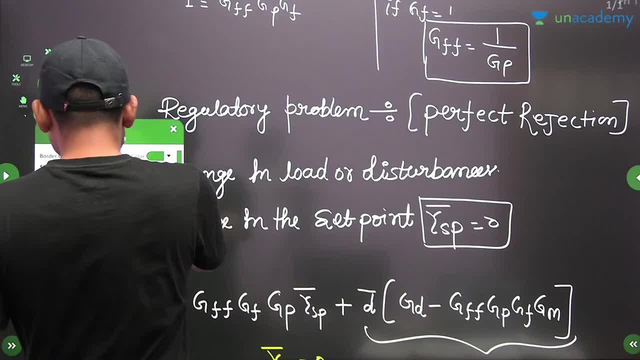 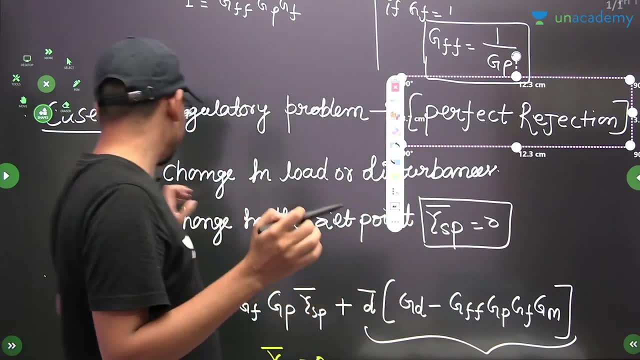 Okay, one more term is written. what is written? perfect rejection. Let me change the color a little and write this: This is called perfect rejection, And if there is any disturbance in the perfect, when will it be able to reject the perfect? 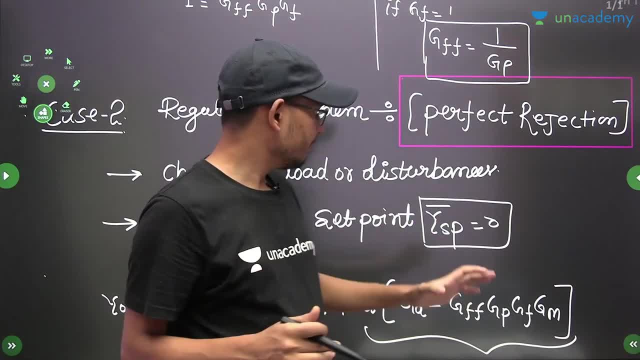 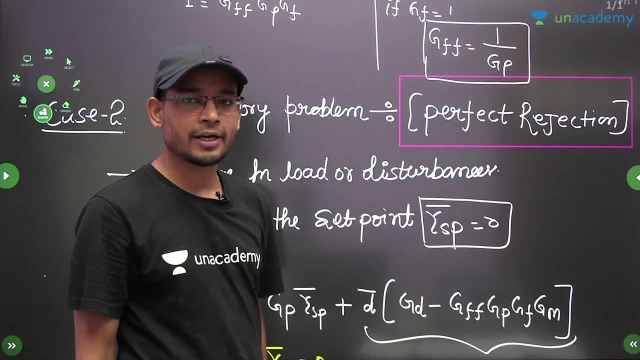 When whatever disturbance is happening in it, zero it. This means: whatever disturbance is happening in it, you can directly zero this part too. In case like this, If you are able to think a little. Okay, perfect, rejection means whatever changes are happening to you through the load. 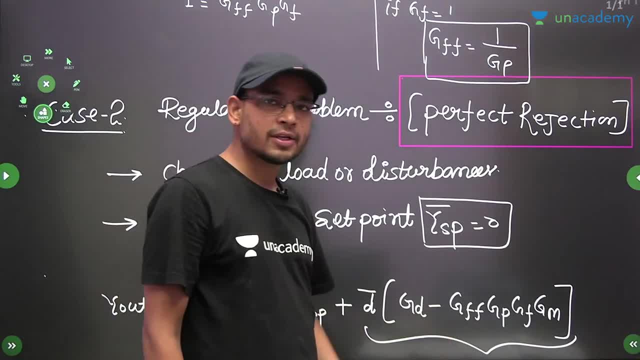 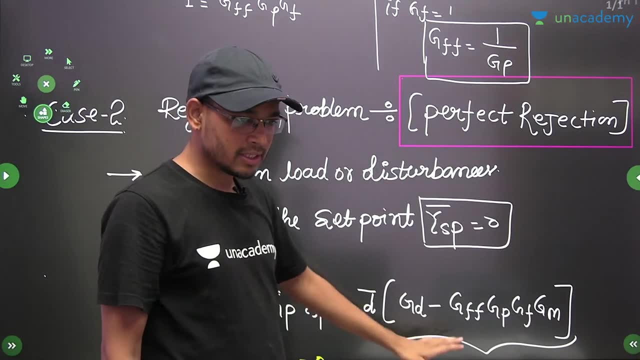 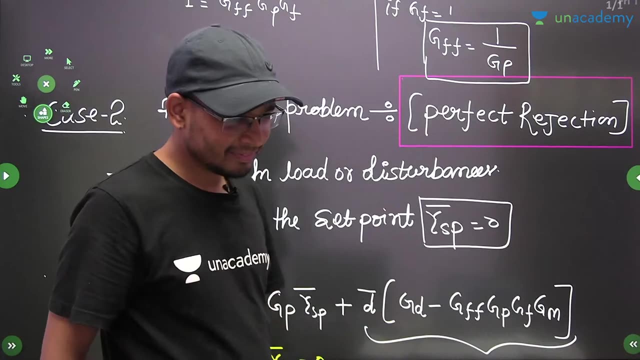 Whatever your disturbances are happening through, the load should also be zero. Only then you will be able to call this controller perfect rejection, And perfect rejection in that case is called regulatory problem. So you can see it in this way too. Yes, they make it very complex. 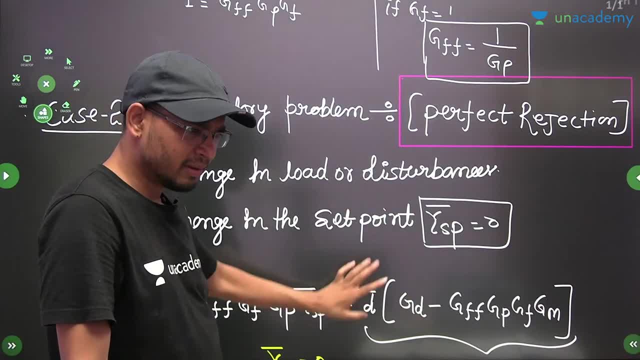 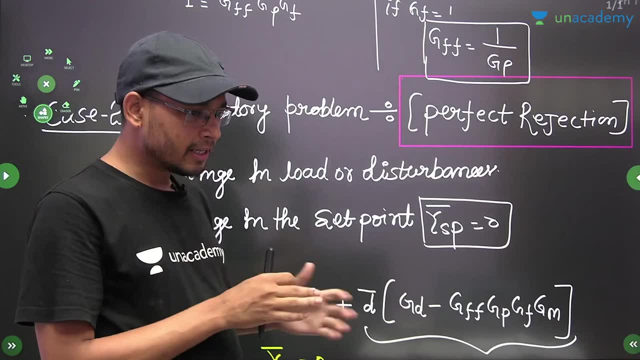 It is very simple. They make this part very complex. Okay, it is very simple. You will follow it step by step. You will learn the concept of this by smiling, Otherwise this thing becomes a big deal. It seems that what is going on, something is very next level. 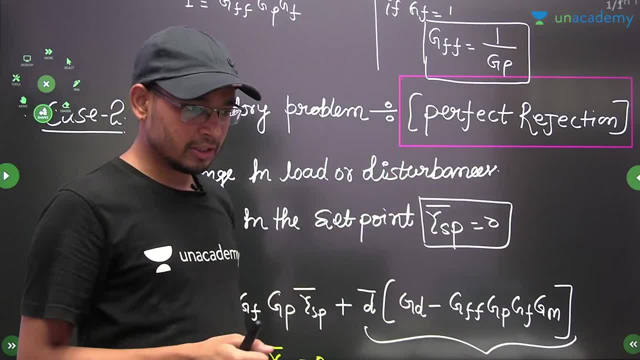 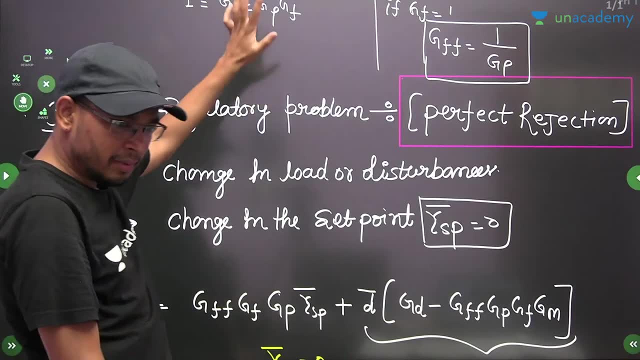 It is nothing. If you follow the process very easily, then you will understand things. Come on Now. let's talk about the question from here. Are all of you ready? Will the question be given? Everyone is ready. This has come completely. 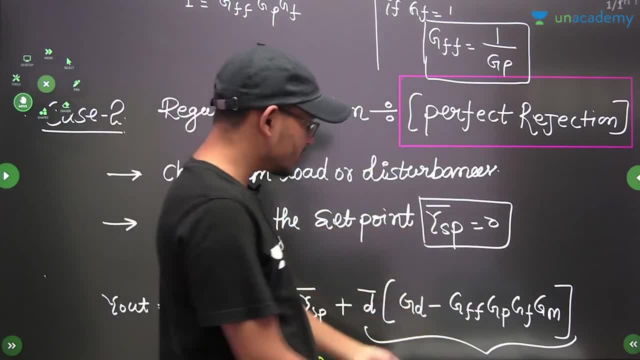 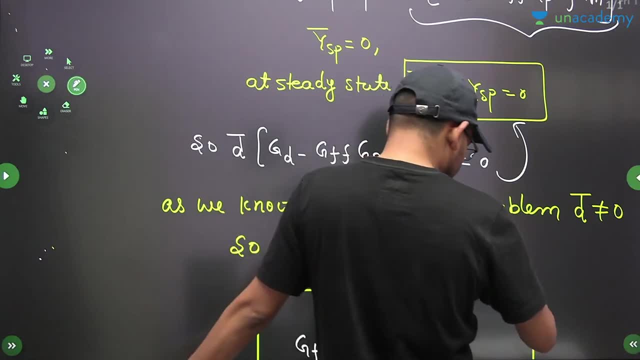 Tell me this first: This has come completely Perfect. rejection means this term will be zero. Okay, You guys are completely ready up to here, right, Properly, Come on. It has come completely Once in a great way. Yes. 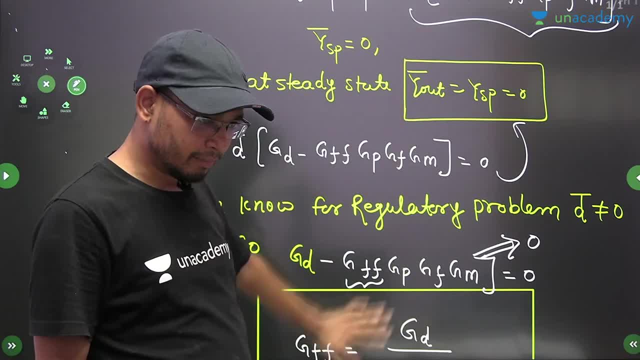 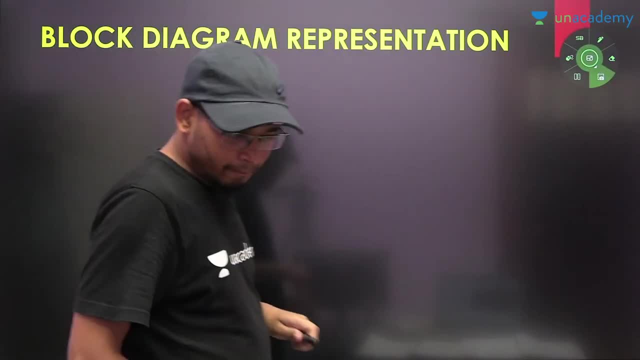 Right, It has come completely with love, There is no problem. Okay, Come on Now. I will give you a question. I will give you a question. Are all of you ready? Come on Now, don't do anything wrong, Okay. 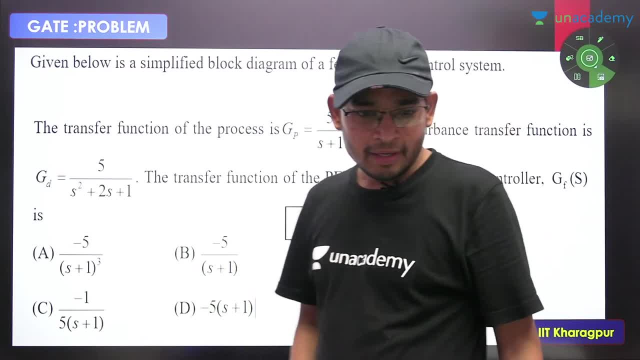 Now, don't do anything wrong. The question has been asked in 2014.. Now, don't do this question wrong. Okay, You have learned. You do it. and see, Some people were asking that. sir, this will always be in the case. 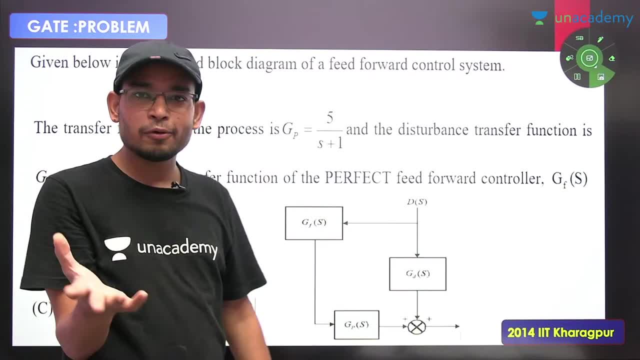 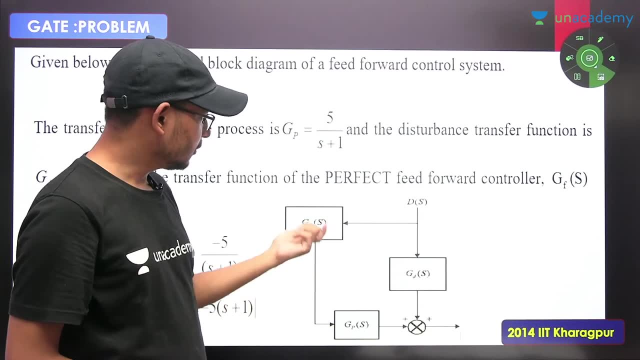 See, I told you that they will make a transfer function and give it to you. Okay, What will they give you? They will make a block diagram and give it to you. You have to find the value of GF here. Okay, So find the value of GF for perfect. 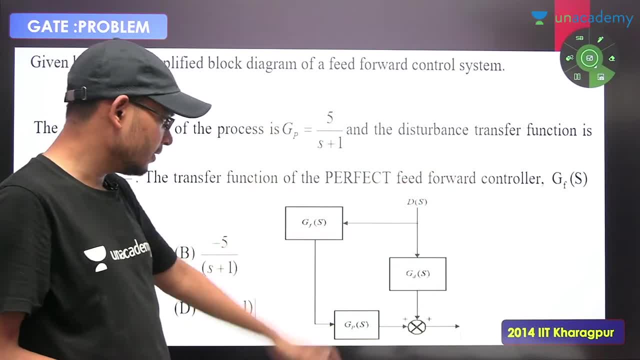 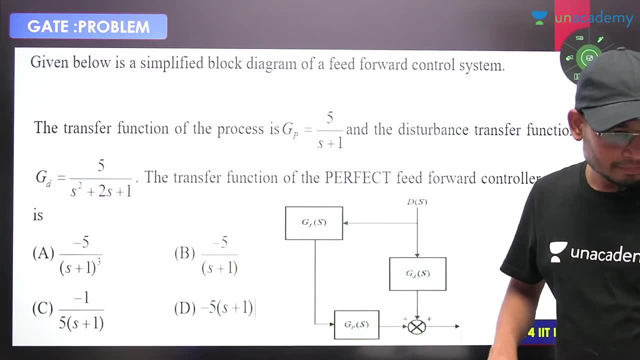 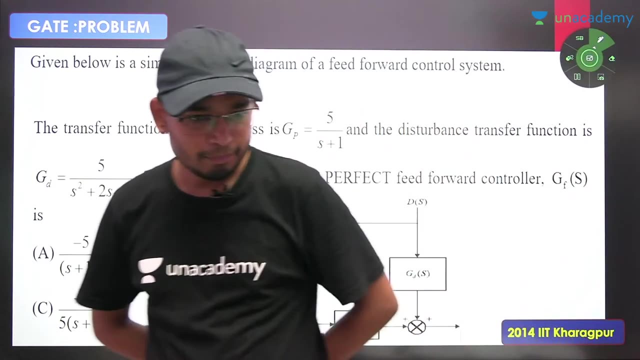 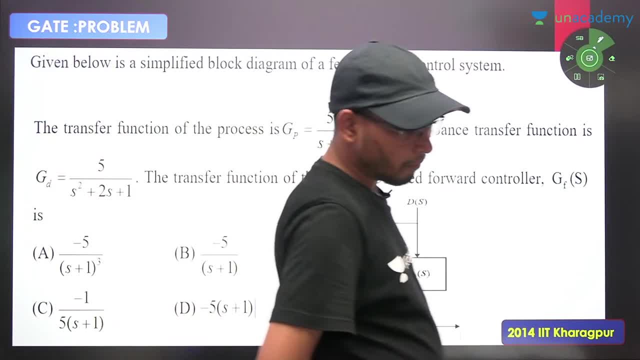 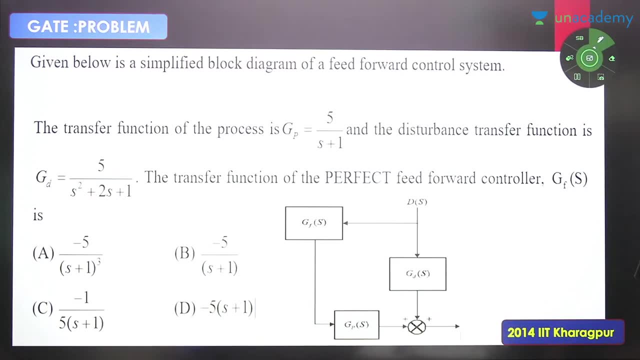 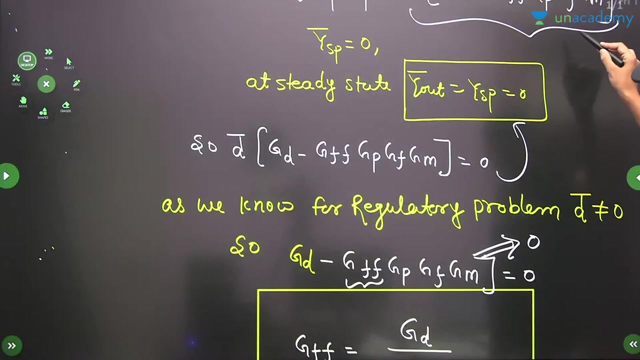 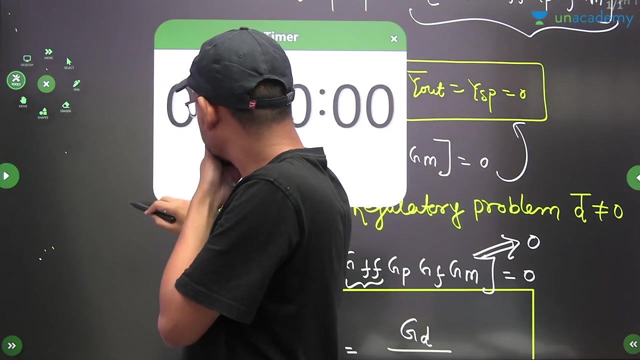 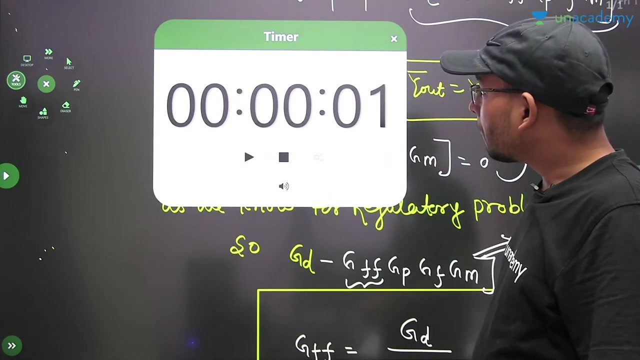 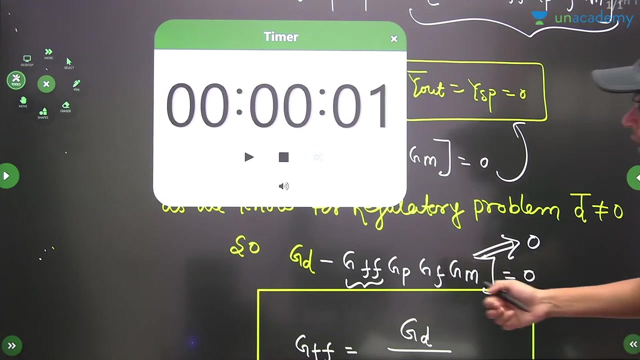 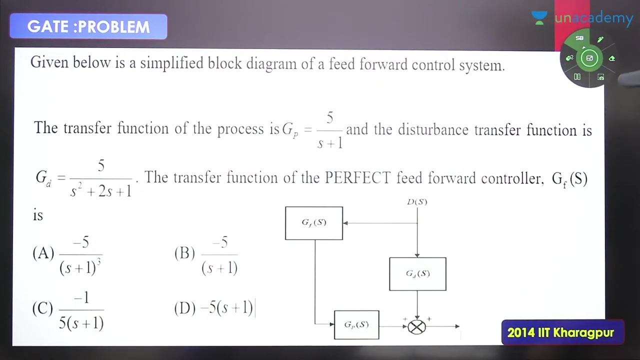 Properly. Yes, We will do it a little fast, Okay, But it won't go there. you won't be able to see anything. you won't be able to see anything. take it there or I'll drop it. Do it quickly. 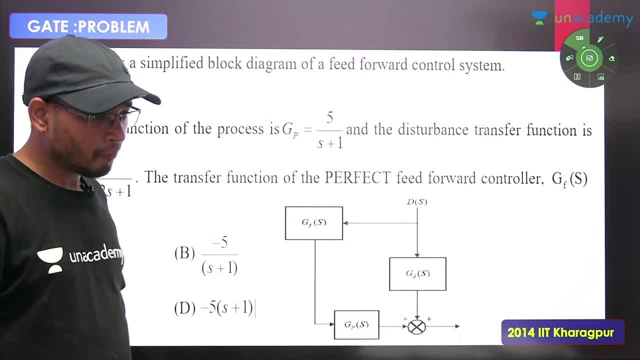 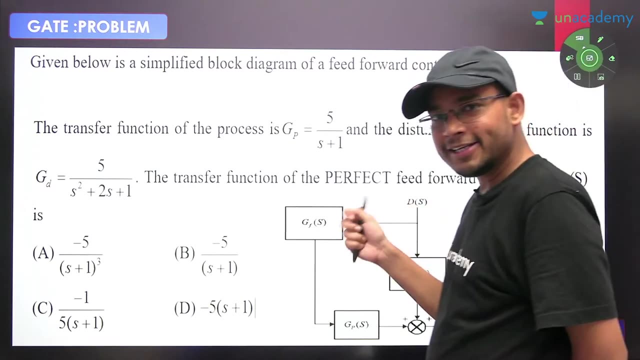 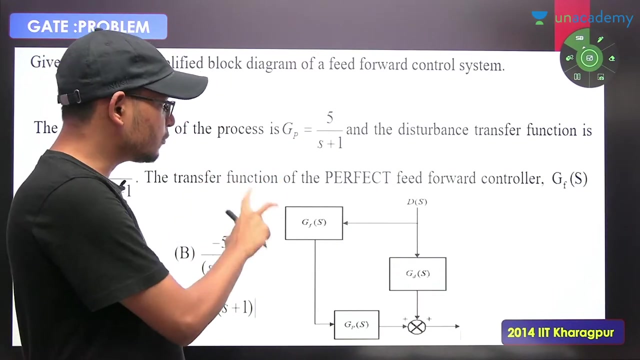 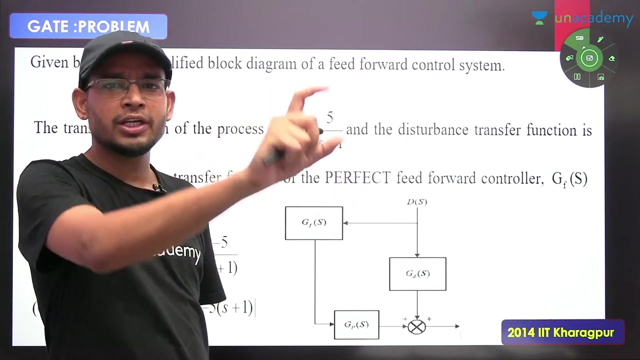 Will everyone try it on themselves. I am telling you that these questions are left in the IPC. they do everything- first order, second order, controller- but such questions are left. so these questions sustain you, the questions related to the problem that in one subject I am having a problem here, or in this subject everything is fine. I am only missing in this part. so I am talking about that part. 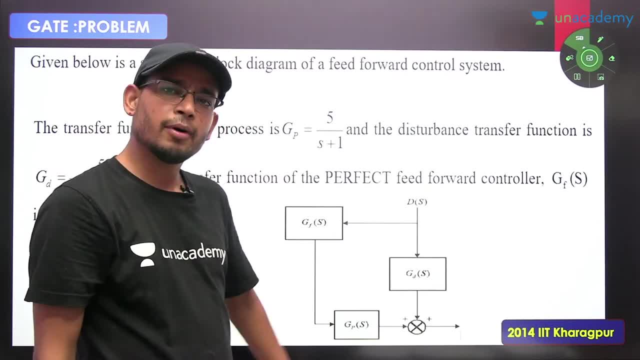 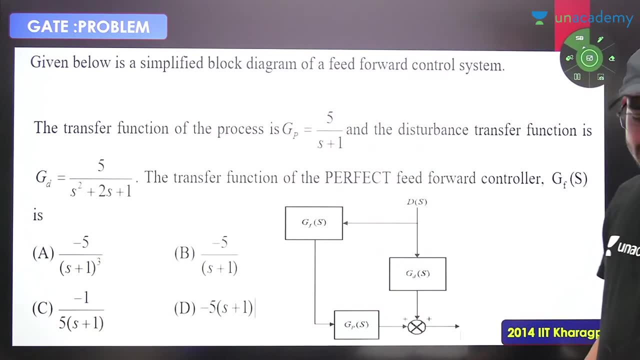 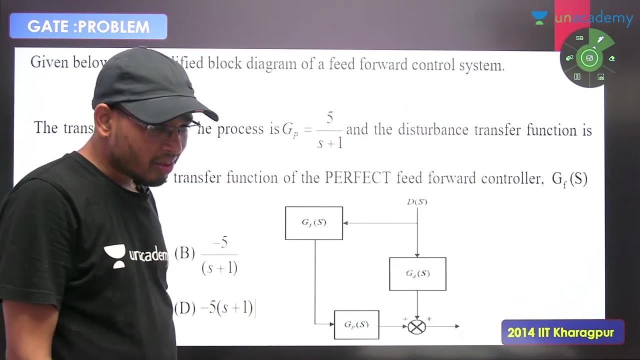 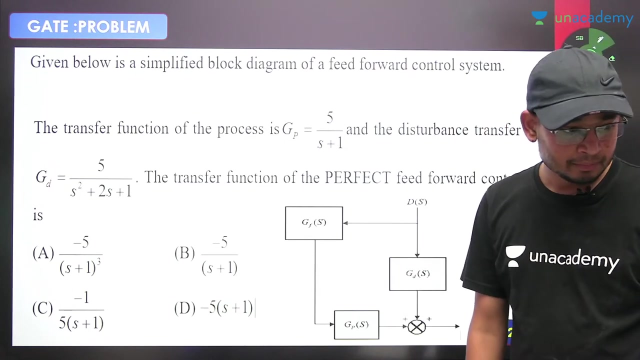 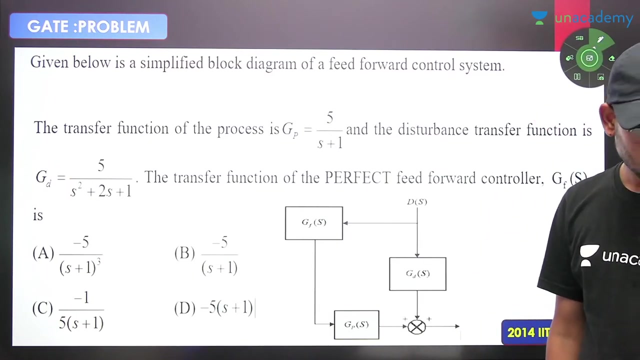 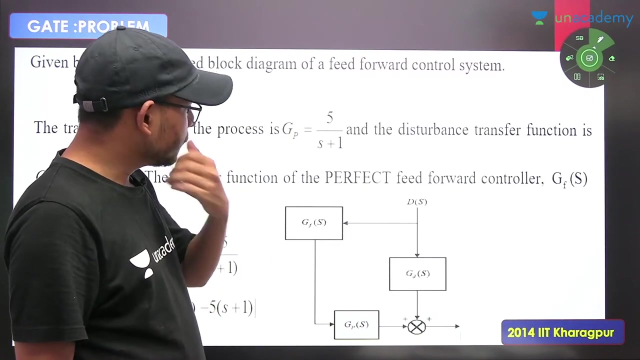 In this part. there is a lot of query of the students. there is a lot of query that these type of questions are not made, so make it like this: this is the zone of the whole IPC Done. it is possible that there is a little misprint in the option. let's see. there is no problem, it is not matching. it is possible that it is not matching because it is of 2014,. you will have the option then once you will tell me what correction to do in the offer. now we are seeing. whatever answer is coming, we will see. 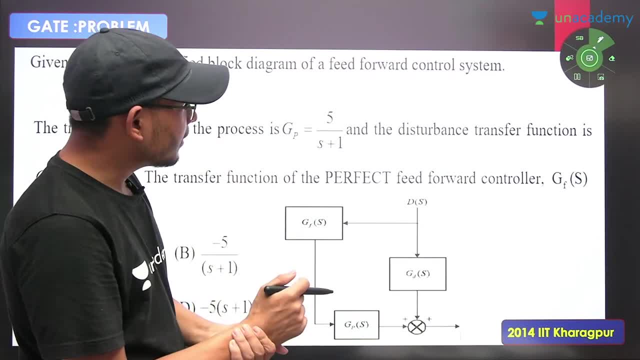 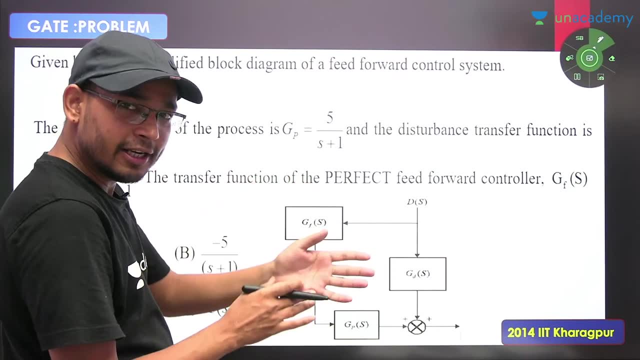 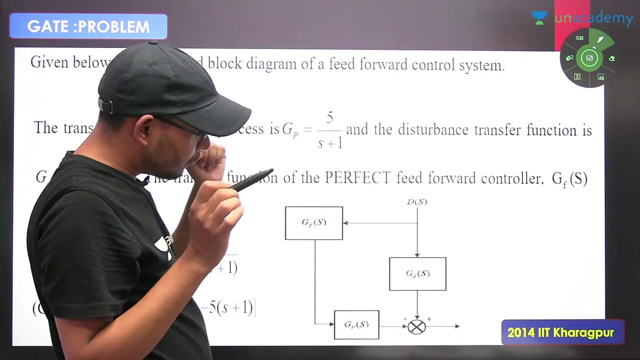 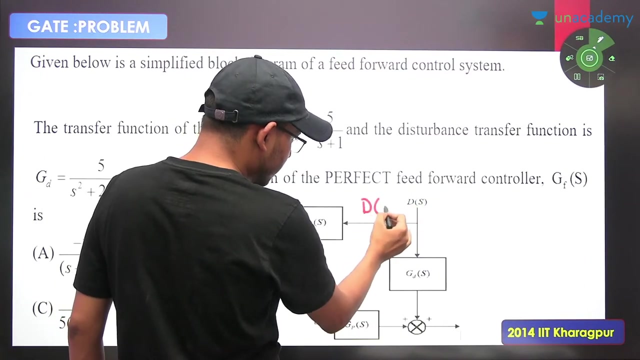 So let's start solving. start solving. it will be solved here in the middle. everyone will support we are solving here. pay attention, everyone, take care a little and I will try to solve it in the middle. So first of all, we should know how to solve the loop. so I have taught you how to solve the loop. brother, will the DS come here with a smile or not? everyone first tell me your DS will go here and your DS will go here. 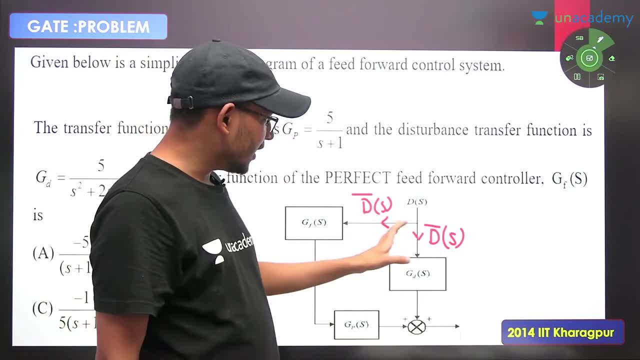 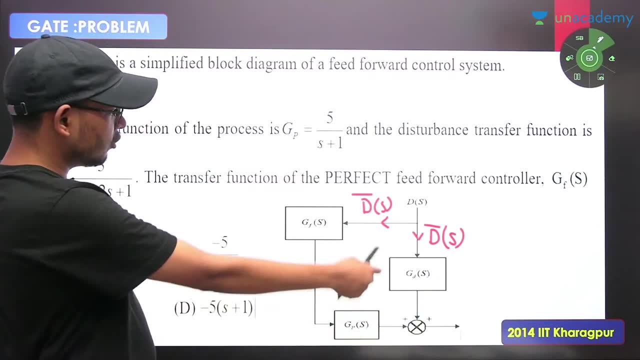 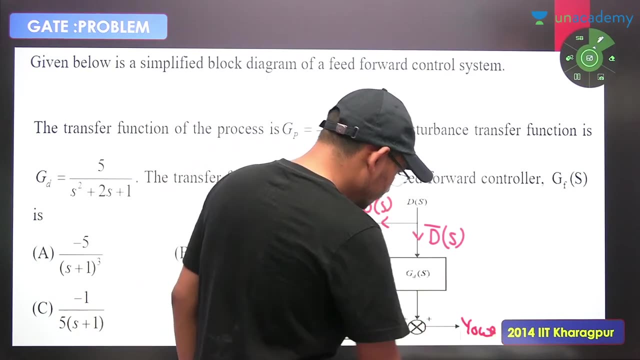 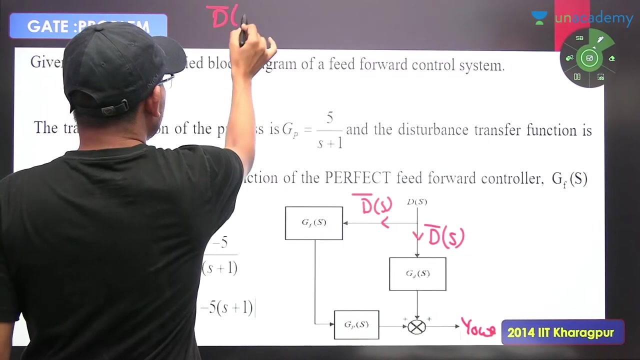 The signal never transfers. I would have said this line at least 50 times: come on, keep writing, keep writing. and this is your output. ok, this is your output. take the output, keep writing. so what will happen? your D bar will be going here. so I will write D bar of S into GF, into GF. take out GF. only what is this? 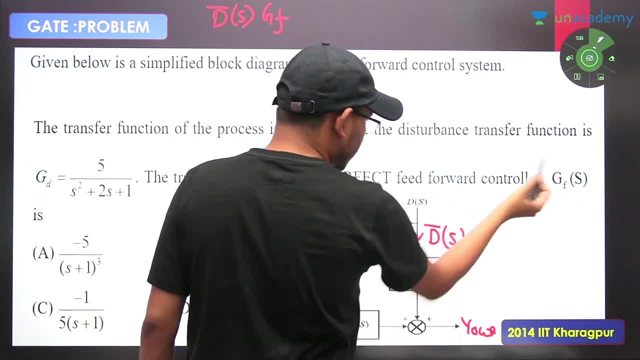 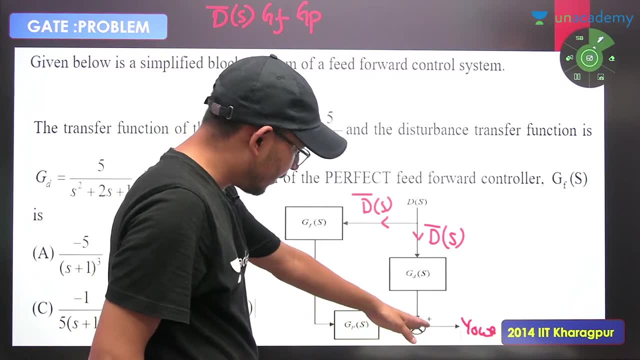 This is the transfer function of the feed forward controller. see perfect feed forward controller. GF is written into GP, into GP. ok, into GP. plus sign is put here. plus sign is also put here. how much will be coming from above? 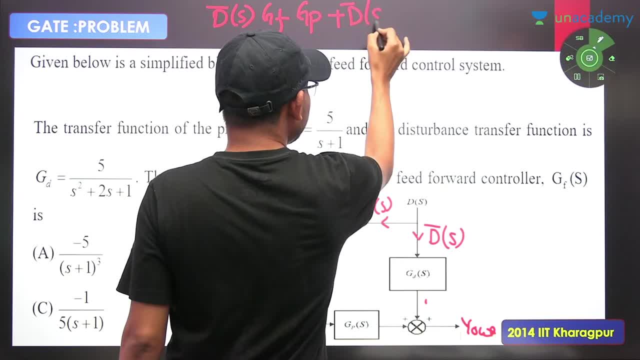 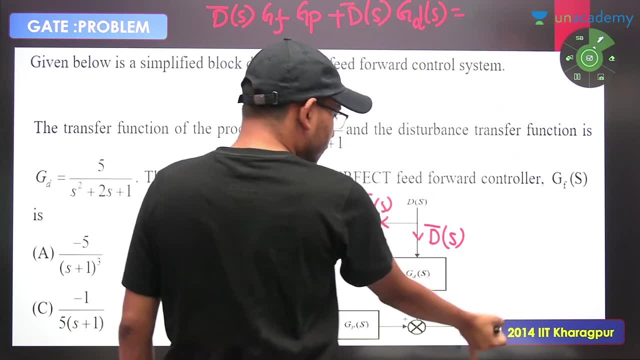 How much will be coming from above? D bar of S? D bar of S. the multiplier will be with this. with GD- GD of S is equal to the output- will not work. come on, I am taking it as the output. ok, I am taking it as the output. right, come on. 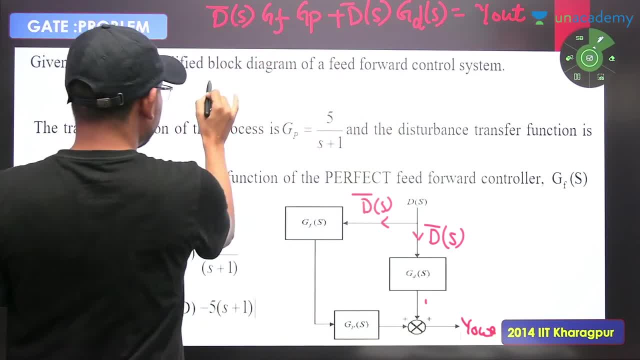 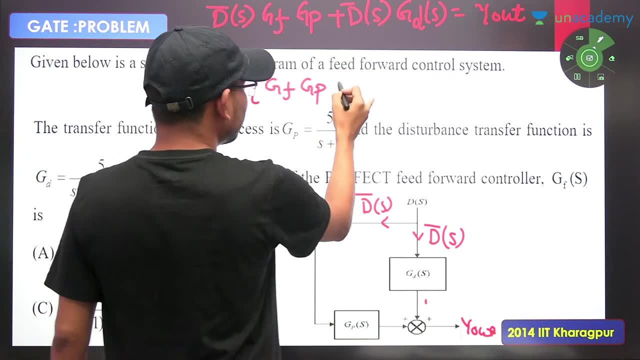 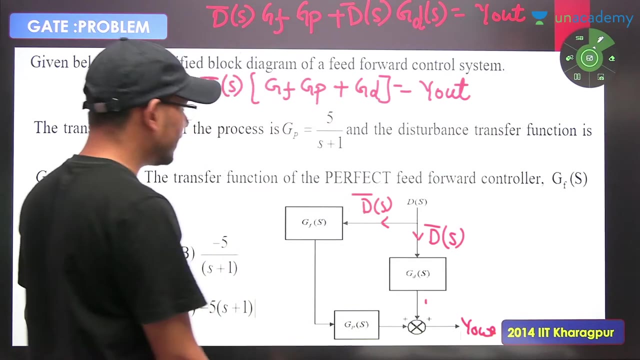 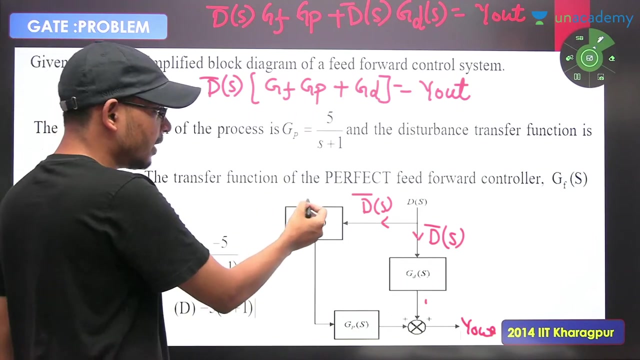 And take this common. if we take D bar common, then we will see very carefully. if we take D bar of S common, then what will be here, GF, GP, ok, and what will be left of plus GD will be left right and what will be this Y output: ok, ok, perfect, your yes, GD is this and GP is this. ok, transfer function of the perfect feed forward controller. whenever you have to take out, then always whose problem will you take out? 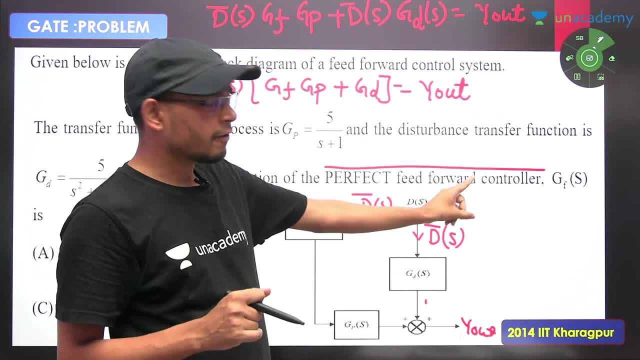 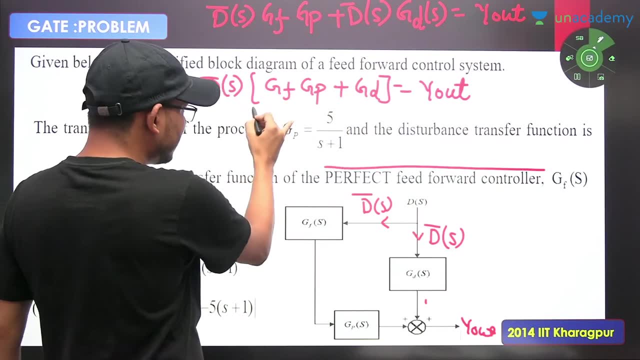 Regulatory. now I had written: whenever you have to solve the problem of perfect feed forward controller, then always, whose problem will you take out? Regulatory problem: ok, so what do you do for the regulatory problem? What did you do to this inner part Zero? what did you do to the inner part Zero? why did you do zero? 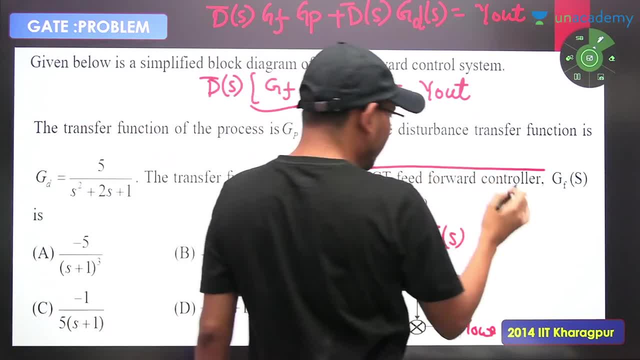 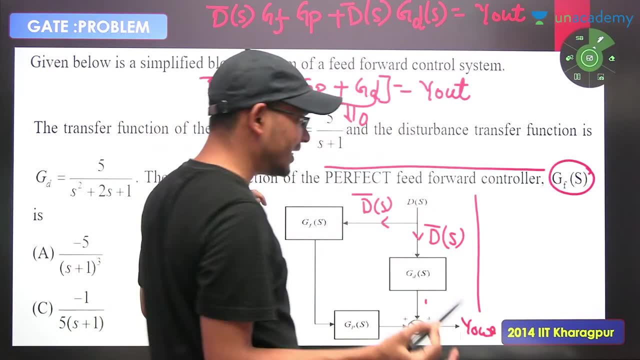 I have told you in the back: why did you do zero? ok, come on, so this will come to my mind, so I will write it here. so from here, we need GF. ok, what value do we need GF? because the question is asked: GF, so we need the value of GF. 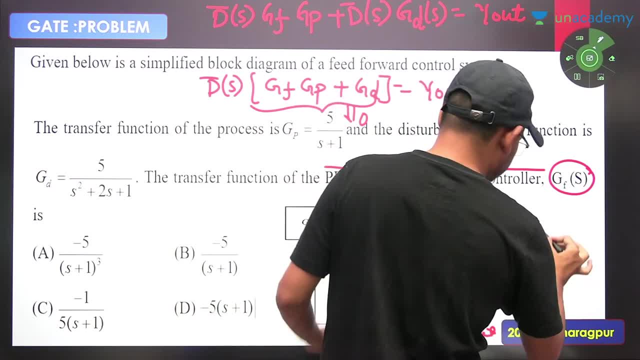 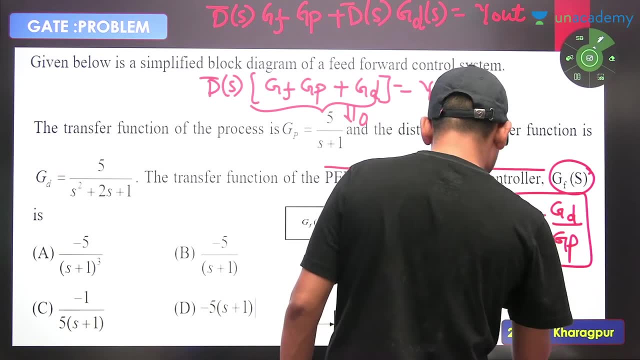 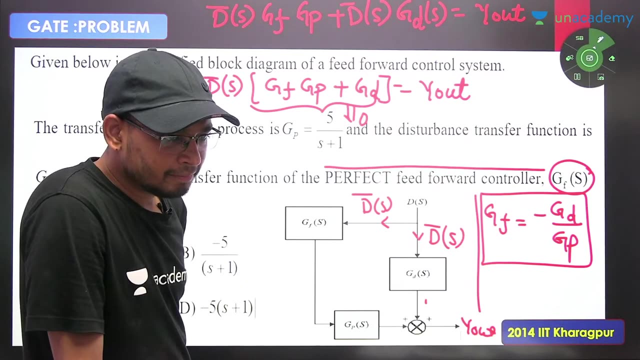 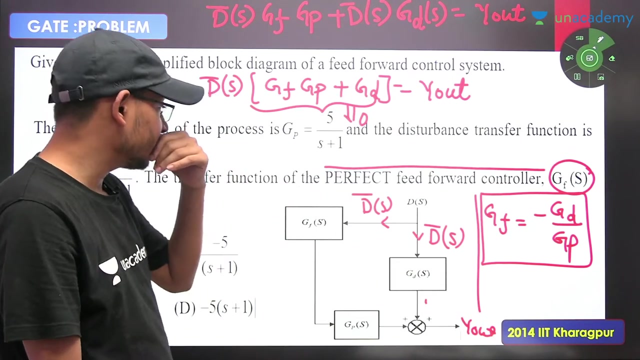 GF is equal to how much? GF is equal to minus GD upon GP, minus GD upon GP. can everyone reach here or not? Now keep the value given first. tell me: can everyone reach here, yes or no? Can everyone reach here first or not? Tell me, can everyone reach here? If everyone reaches here, then the work will be done. it is very important to reach here first. so if you have reached here, then keep the value of GD and GP. 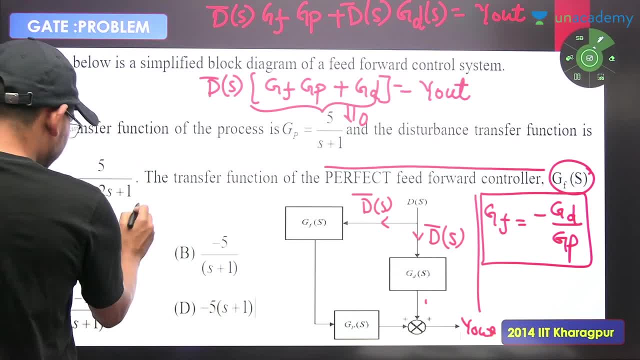 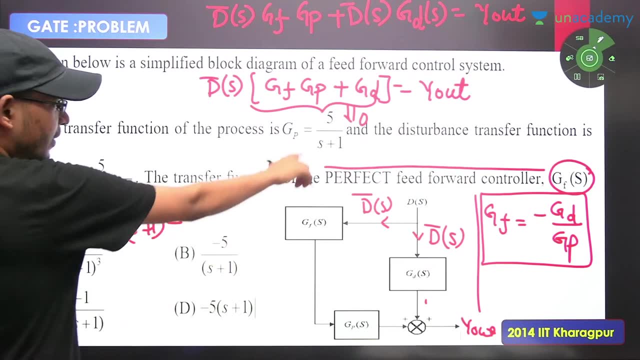 So this is GD. So this is GD. If you solve it for a while, then what is written here? The whole square of 5 upon S plus 1, is it written here? The whole square of 5 upon S plus 1 is written here. this is written: 5 upon S plus 1.. 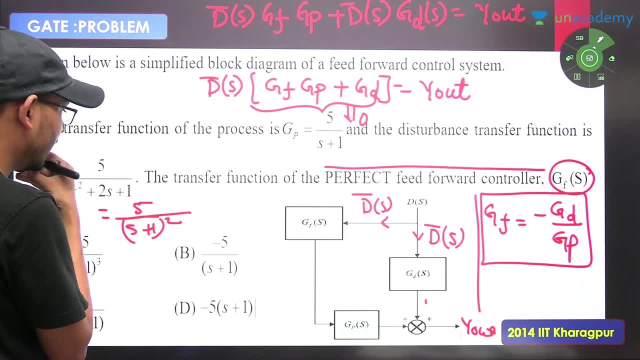 So if we do GD upon GP, then 5 and 5 will be cancelled out and S plus 1 and S plus 1 will also be cancelled out. Minus 1 upon S plus 1 will be left. This means that there shouldn't be 5 here. there shouldn't be 5 here, so it means that the one which is simply remaining, GF, is equal to minus 1 upon S plus 1.. 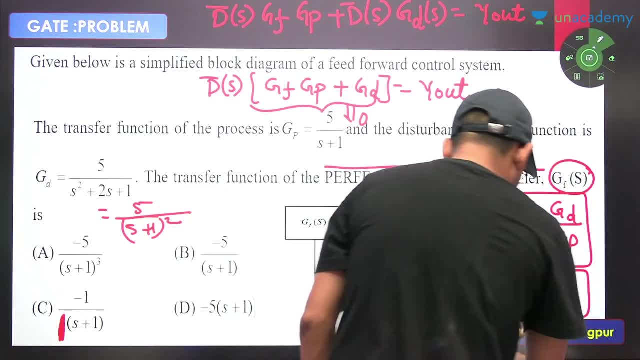 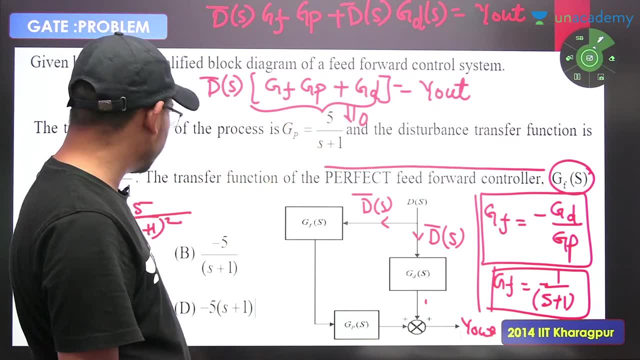 Everyone. just see how much is it remaining? minus 1 upon s plus 1 will be left, because if you divide gd by gp, so 5 upon s plus 1 is here and 5 upon s plus 1 is whole square. so by cutting everything, 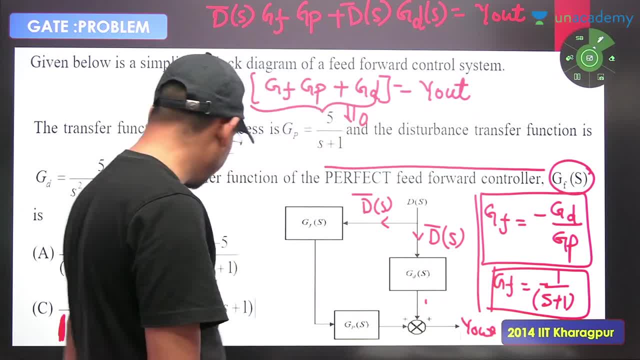 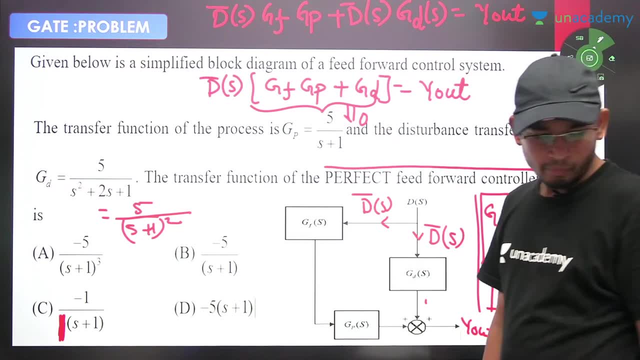 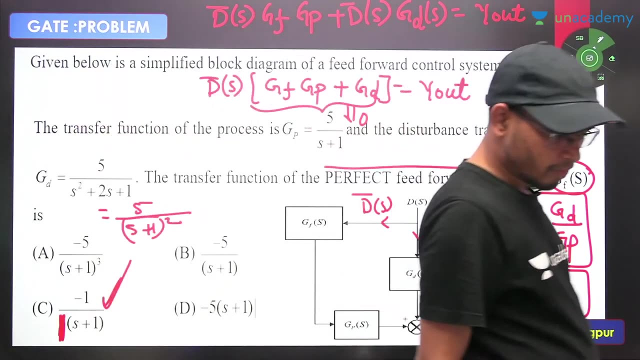 the minus sign which was placed in front, the same minus will come and s plus 1. so here it means that 5 will not be there. ok, so all of you are able to reach here. so the answer will be c part. answer will be c part. 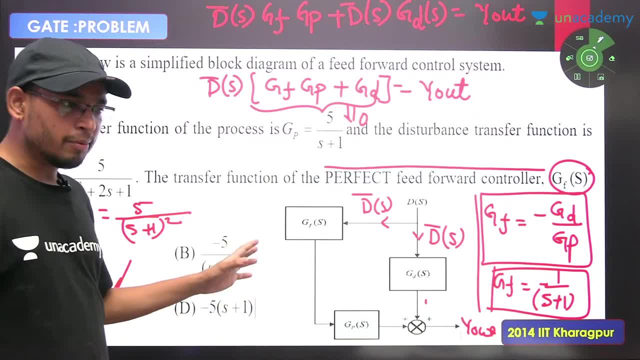 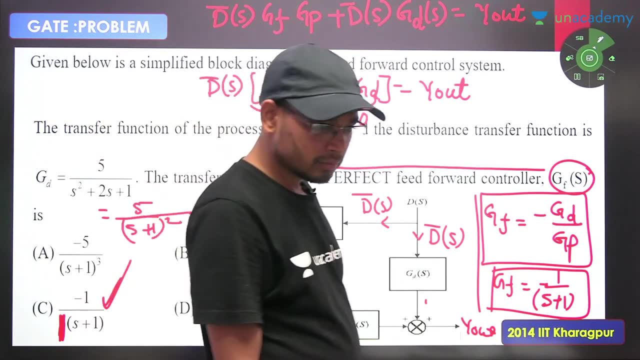 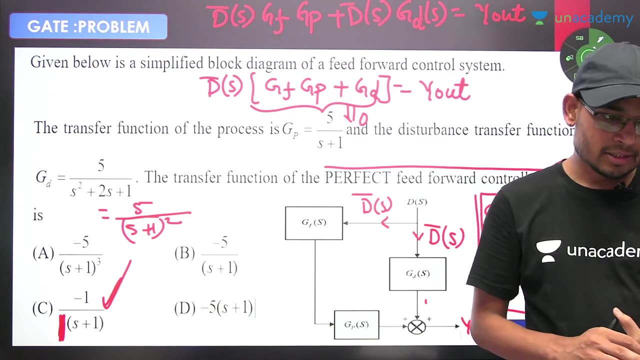 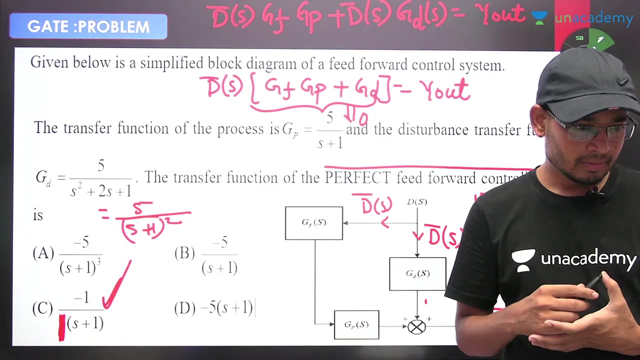 ok, did you get the answer from all of you properly? any student who didn't get the answer you can ask: ok, did you get the answer from all of you properly? yes, most of the questions will be about this. yes, yes, yes, yes, you can assume. 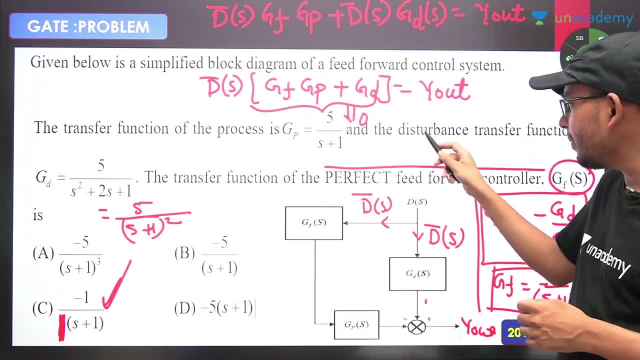 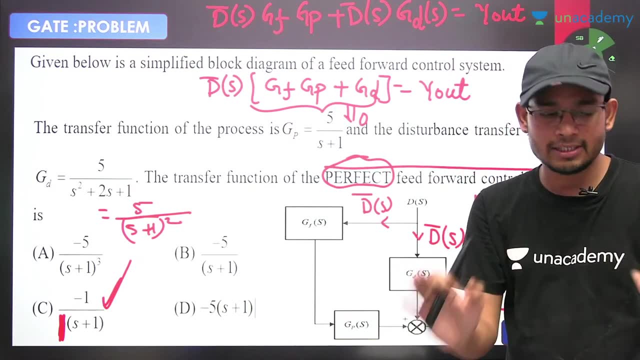 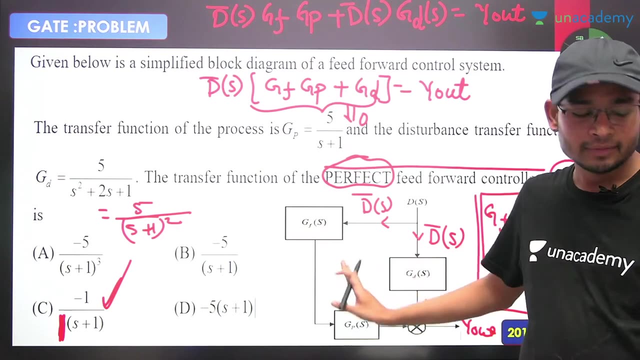 if ysp is not given, you can assume ok. and if there is a perfect word written anywhere, then perfect word is said, then it means regulatory problem. ok, your change will not come in disturbance. sir, if that problem is said, then it changes the setup. sir, if that problem is said, then it changes the setup. 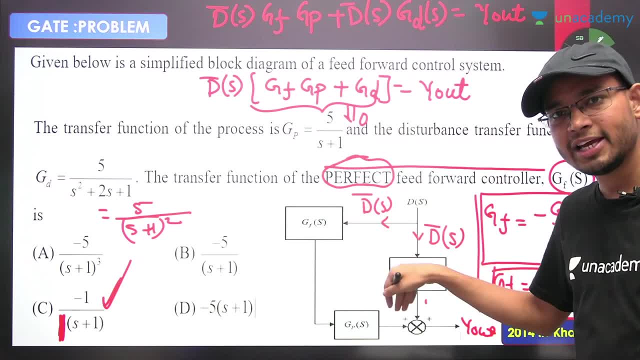 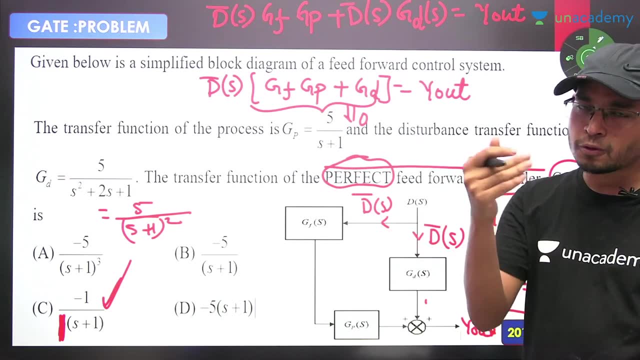 ok, it means it has talked for load only and actually the feed forward controller: you read that. you read for load only. that you read for load only and you don't have any disturbance due to load, that you control it. basically, ok, we don't read for servos. 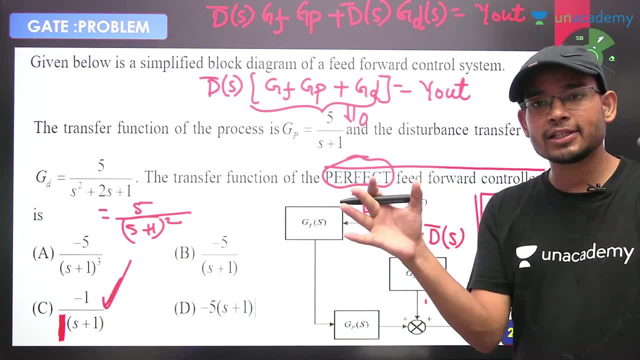 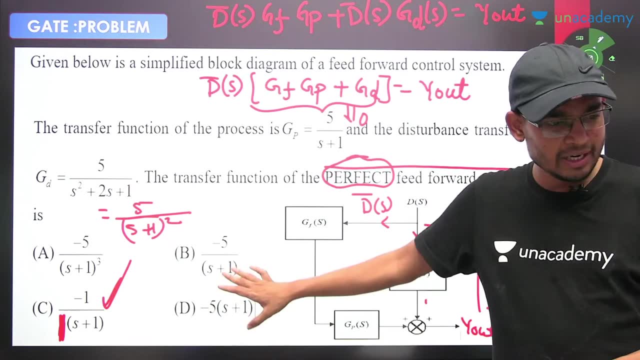 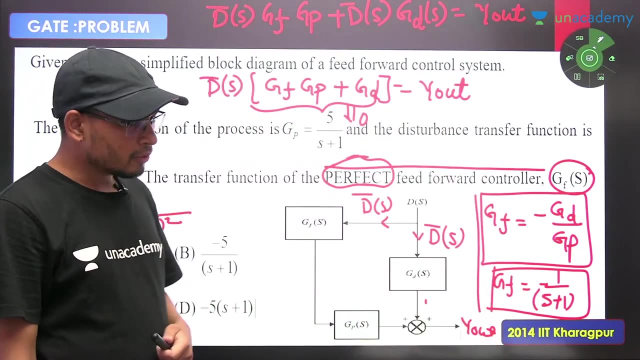 for servos. you can control it in the beginning, all the disturbance coming from the surrounding. you control them. you have to design this controller. so basically, you are talking about it. this theory is for load only. actually, sir, if you were there, what else I would not have given in the question? 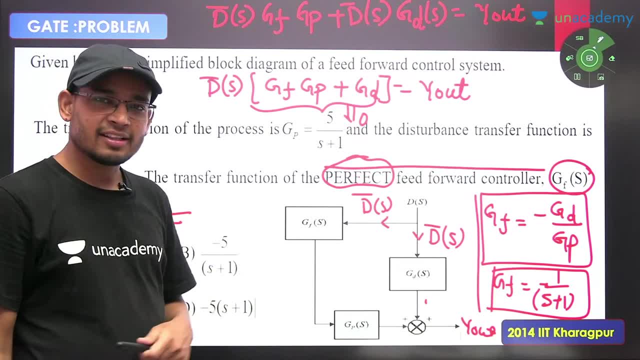 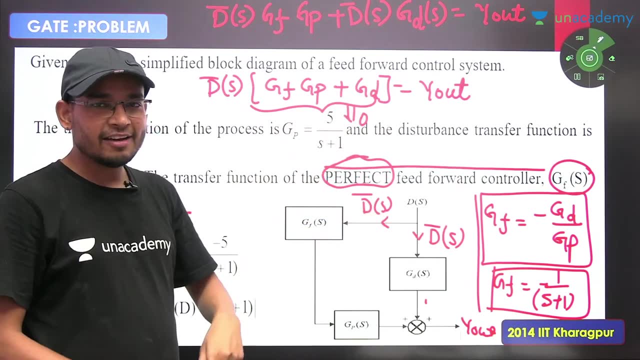 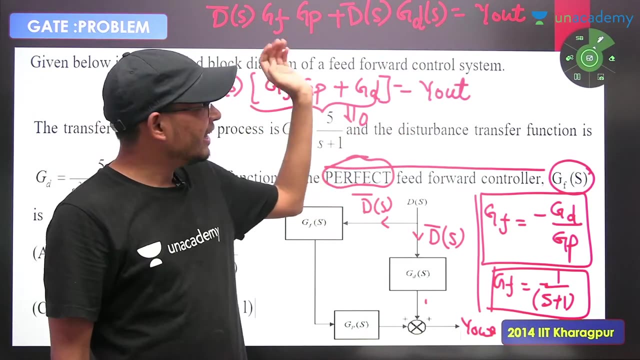 I would have made this complex. ok, I would have made this complex. that it is not so easy to use this control because you can't change the concept. but you can't write this line so easily because you wrote this line very easily. you wrote this line with a smile on your face, you didn't have to do any hard work. 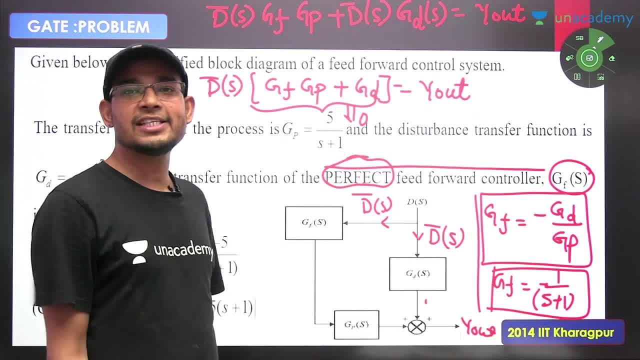 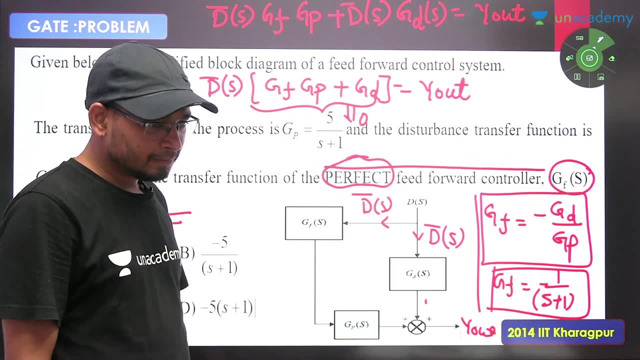 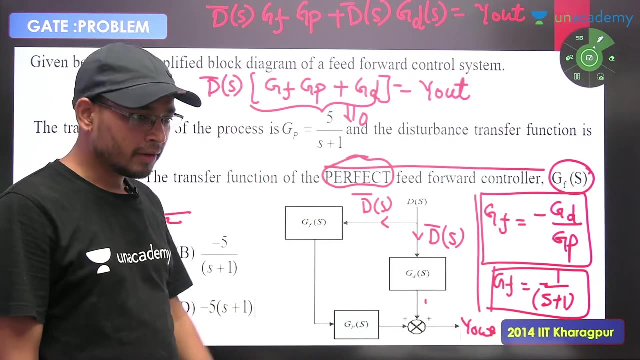 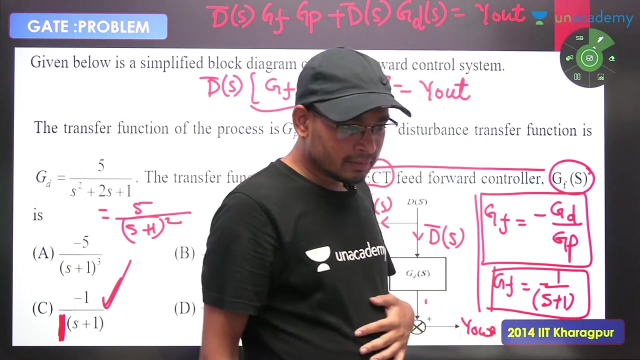 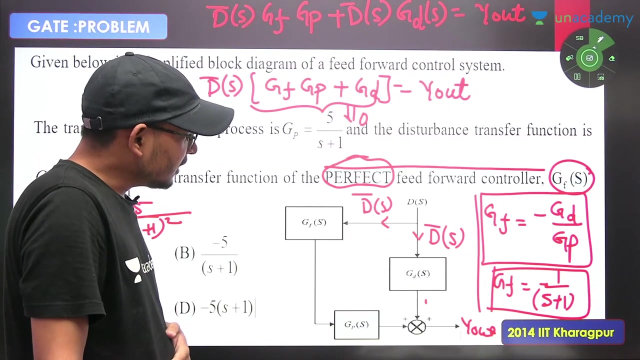 we would have made this system complex. then I would have checked from here whether you know how to solve the loop or not. right? so make this part strong and move forward with strength. ok, this part, yes, sir, you make it, I will make it. you will have to solve the loop. 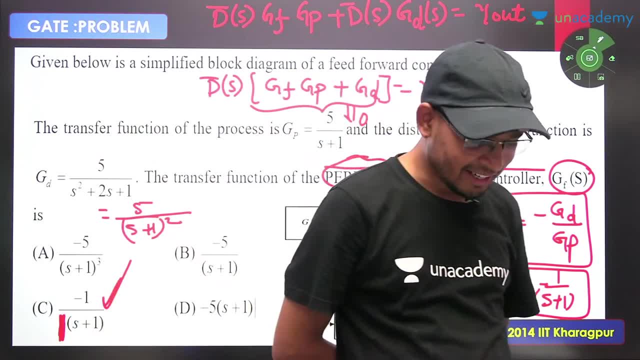 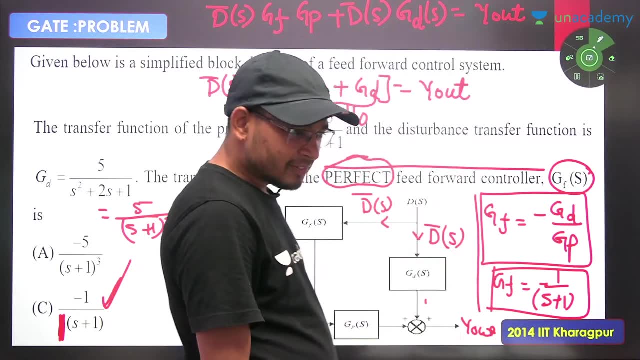 is it a demand? it will be made. is it a demand? tell me, you will have to think. it will take time. come on, we will see it sometime. give me the new. we will see it sometime. there is no problem now. the time is over. 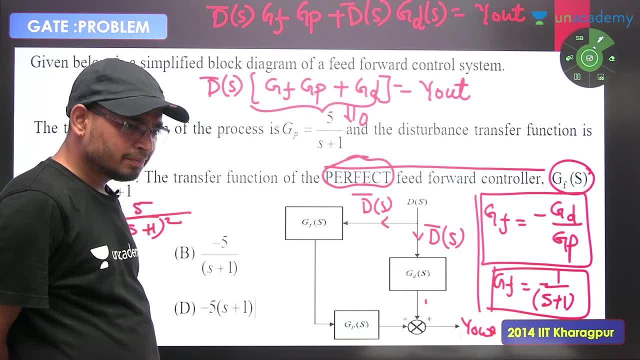 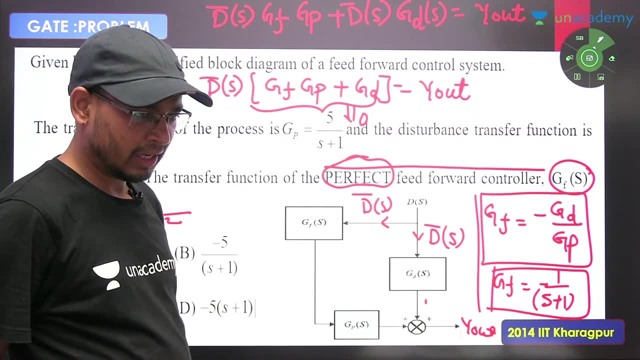 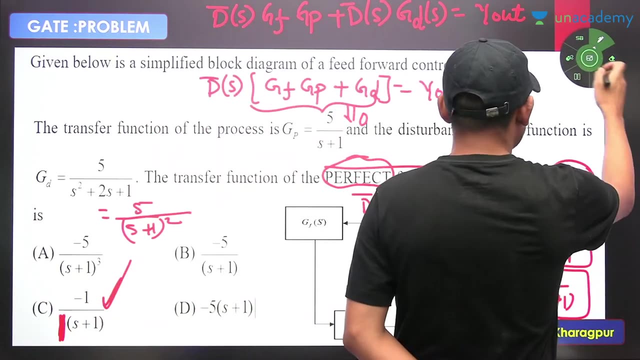 ok, then the time will be too much. we will make it a little. ok, it will take time, otherwise that is the problem. you should know how to solve the loop. ultimately, you should know how to solve the loop. one strong thing will happen. come on, let's do it. 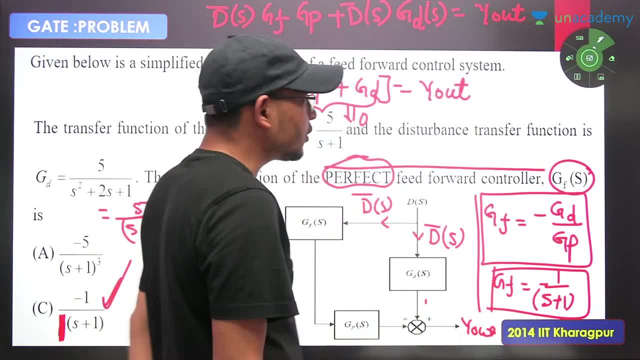 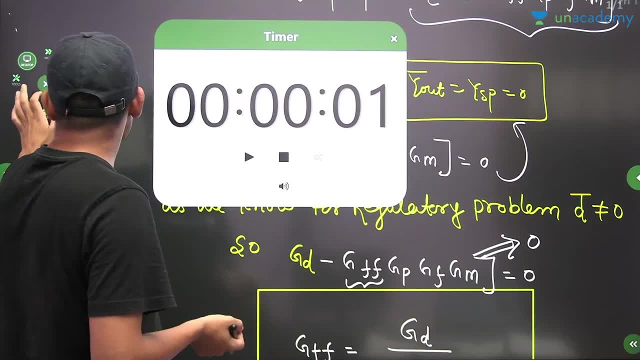 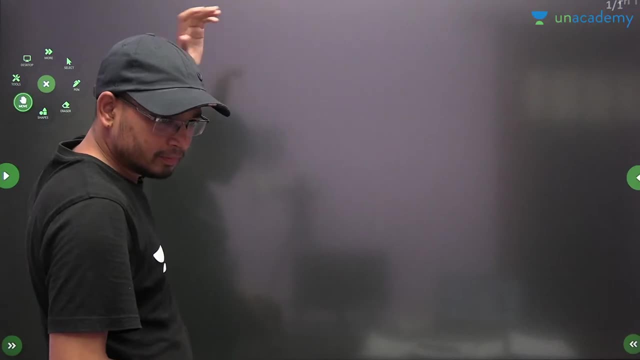 what is this? ok, then you will have to solve the loop, nothing else. you will have to solve the loop. ok, cancel this. first, you will have to solve the loop, nothing else. one more. come on, it will be done, but do it fast, ok. 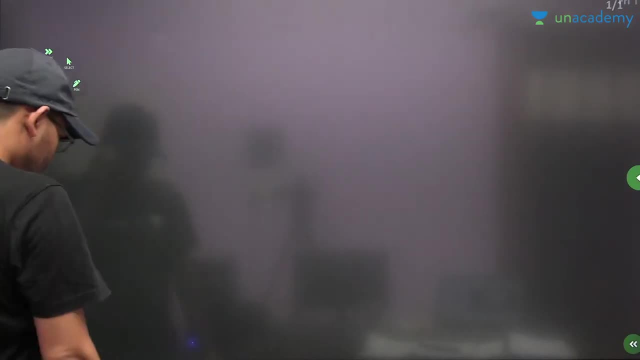 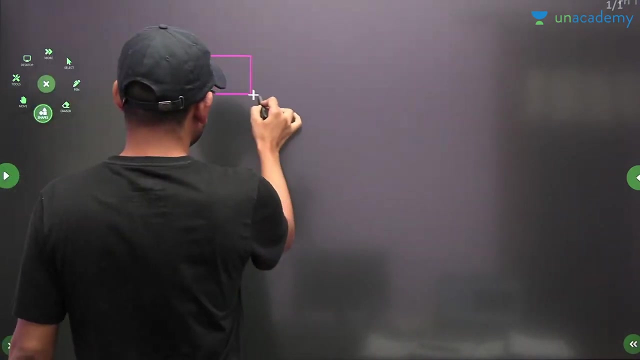 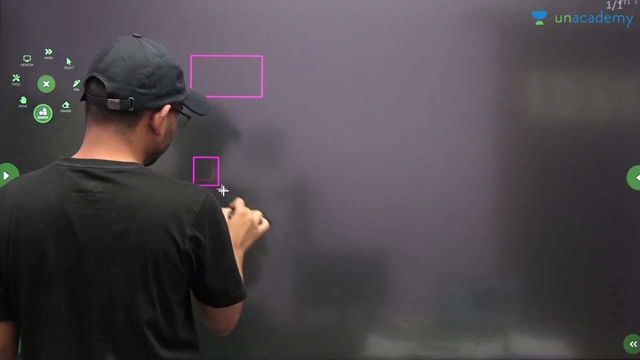 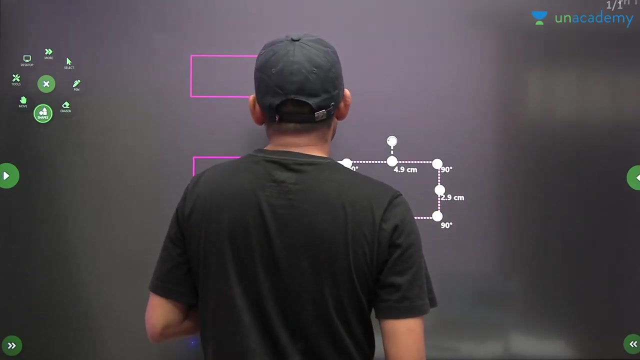 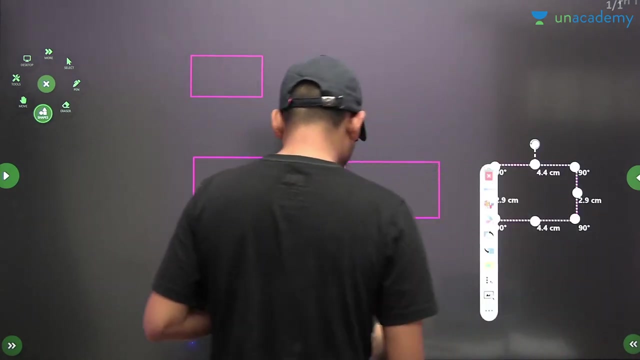 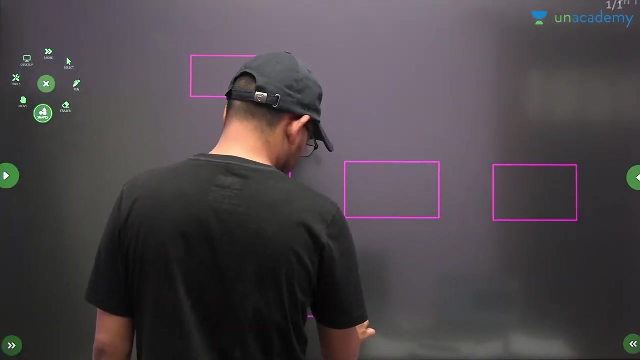 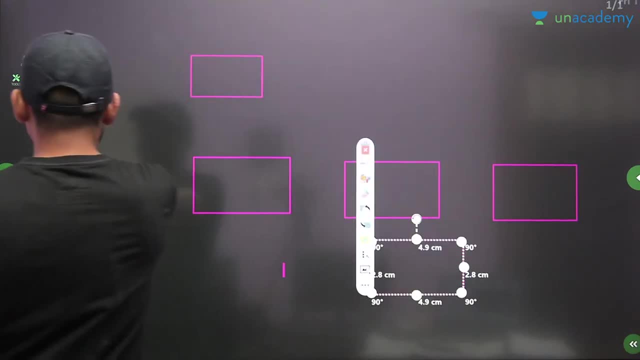 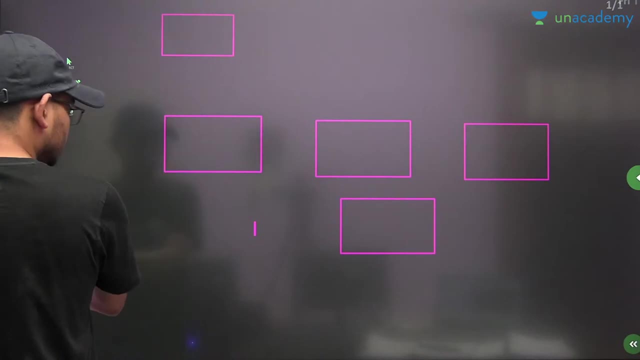 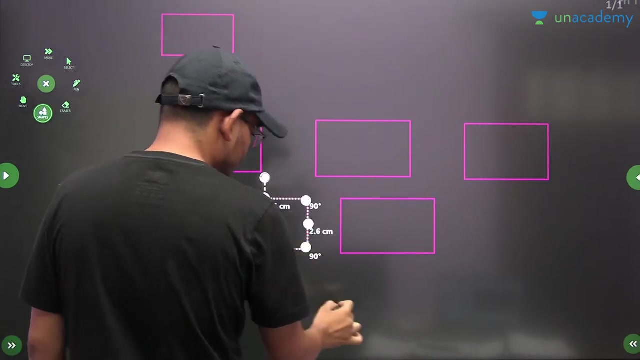 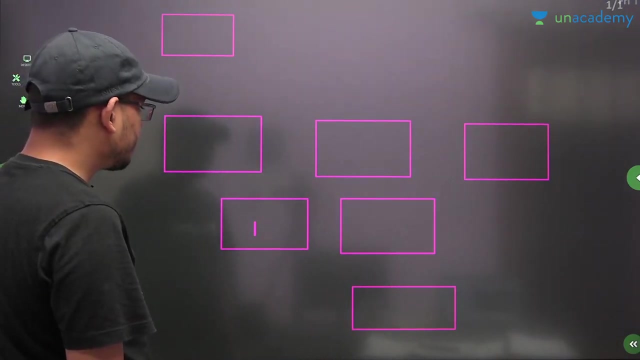 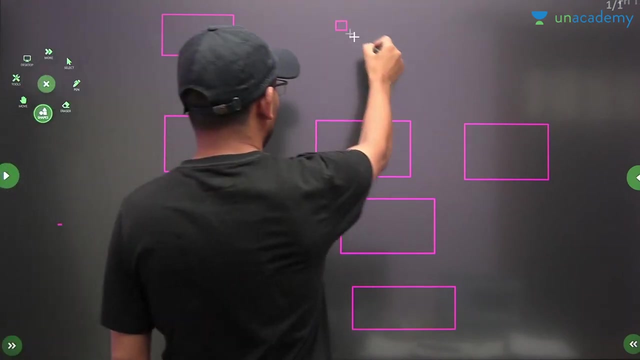 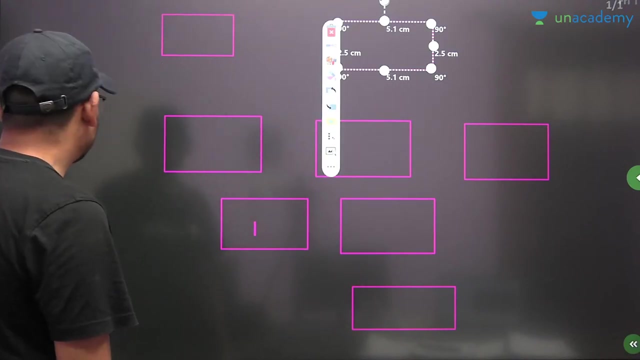 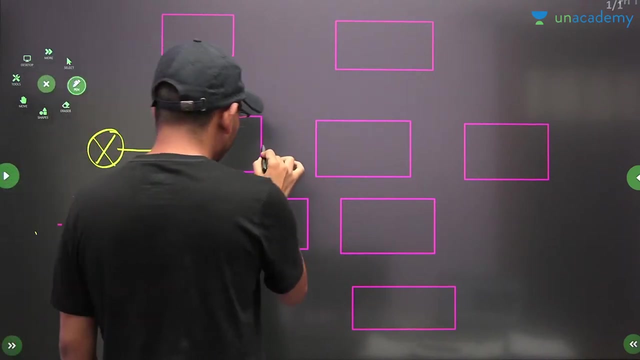 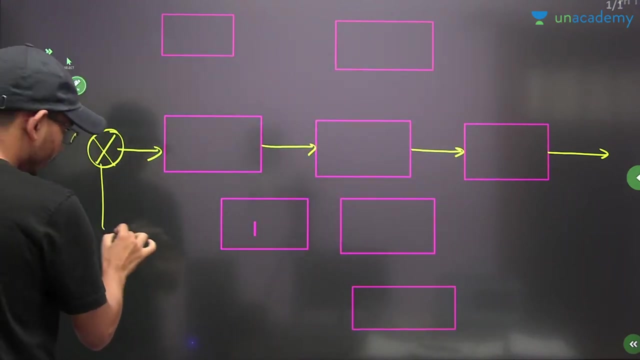 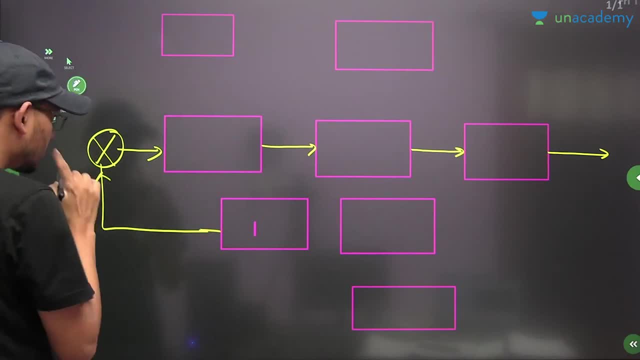 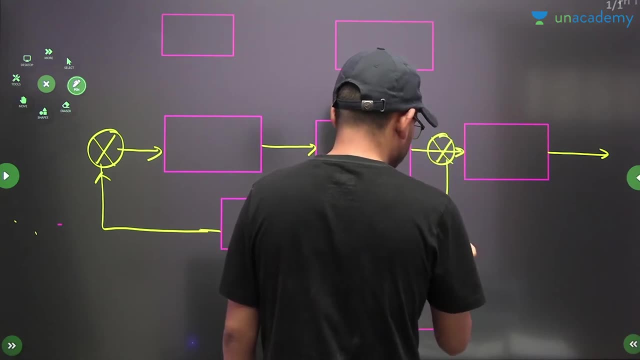 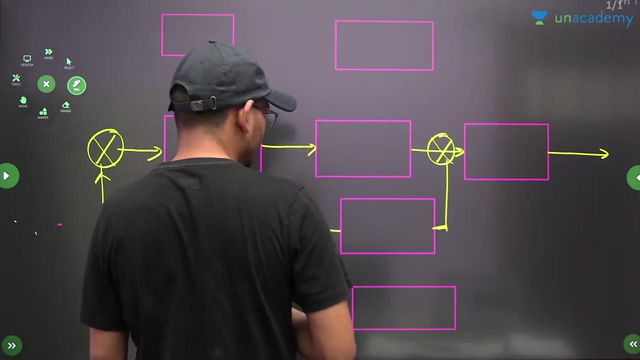 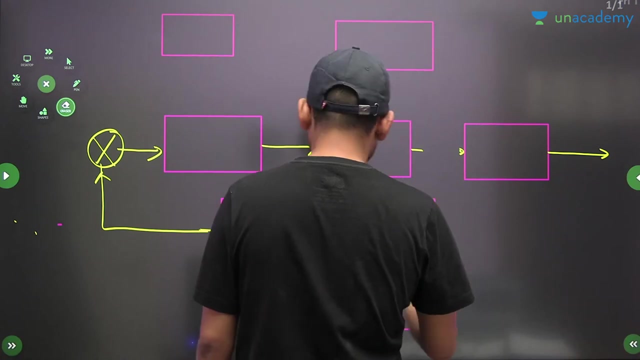 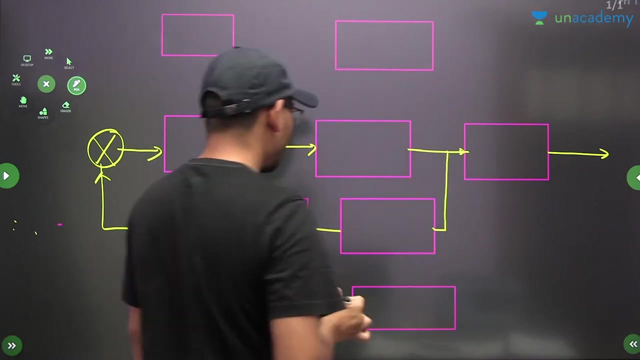 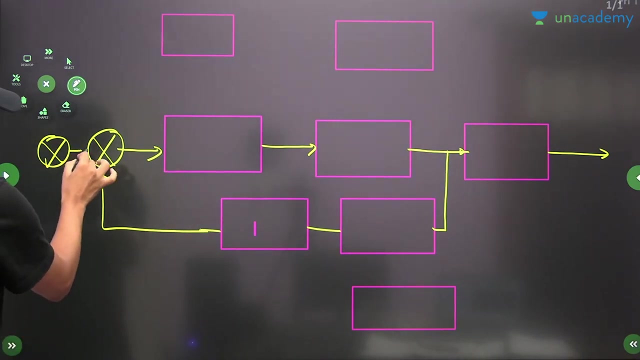 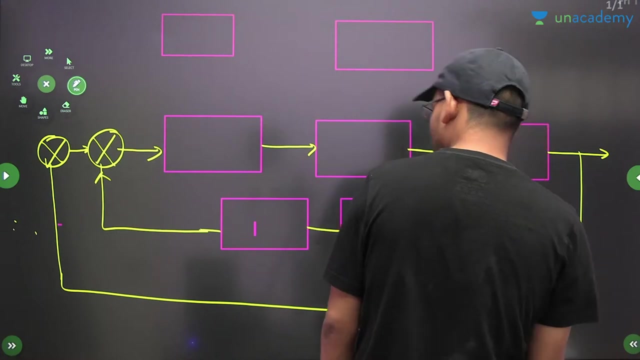 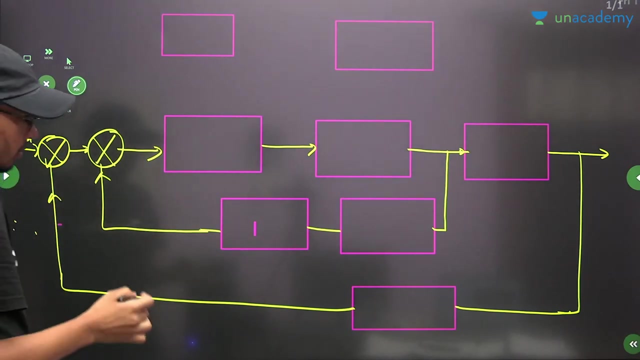 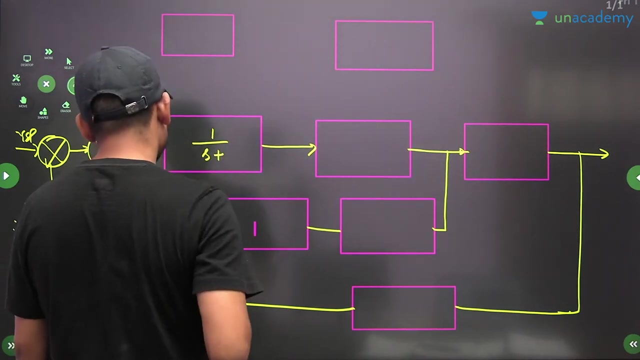 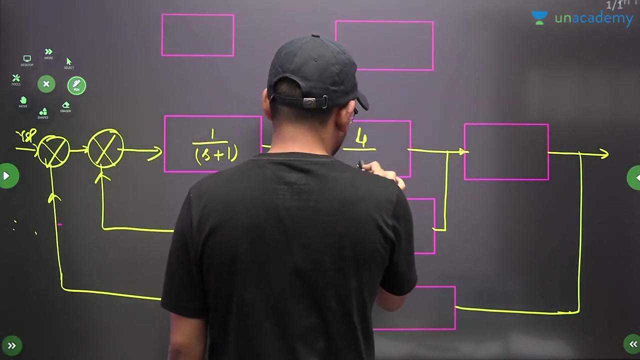 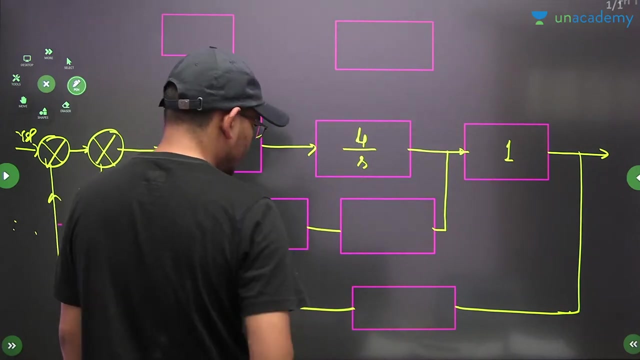 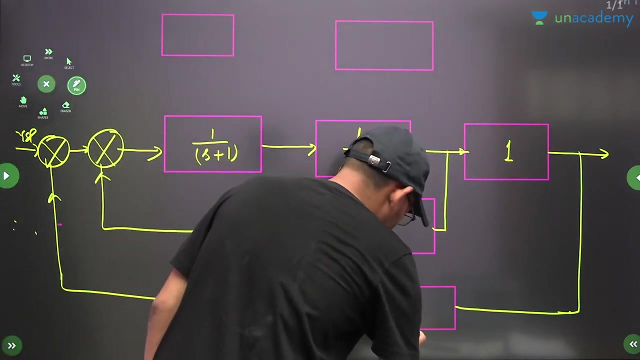 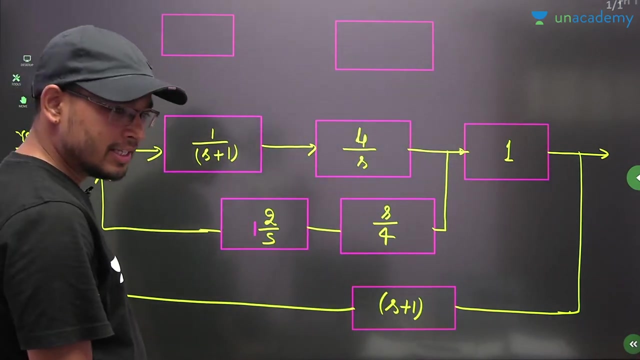 ok, ok, Just give me a minute's time. it will take a little bit of time, that's it, Okay. Okay, it will be solved easily, don't worry, it's easy. it's easy, it will be solved easily. 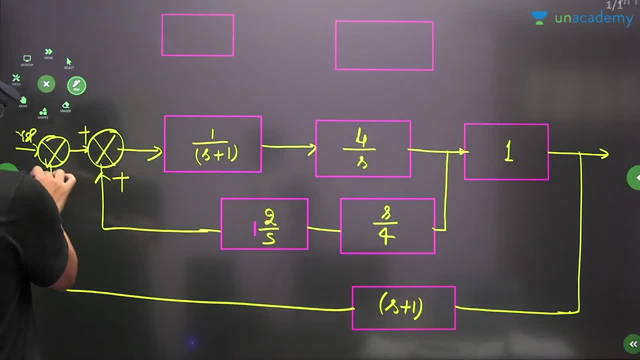 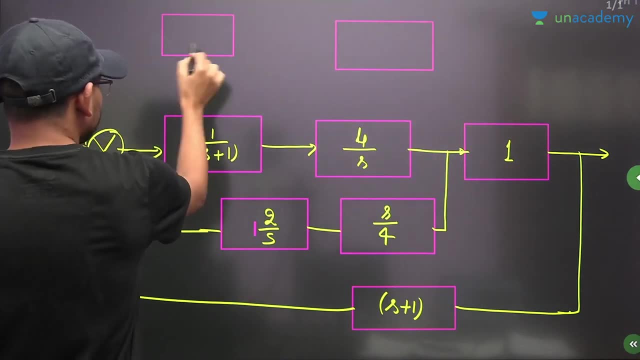 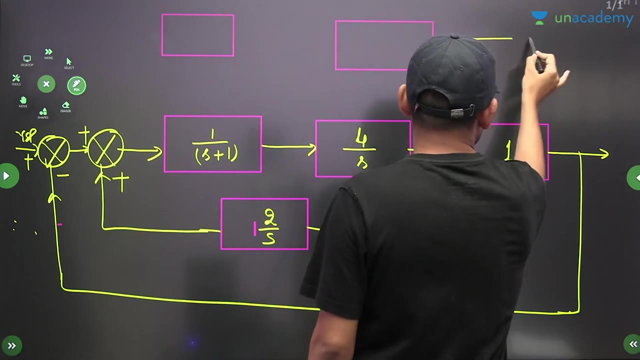 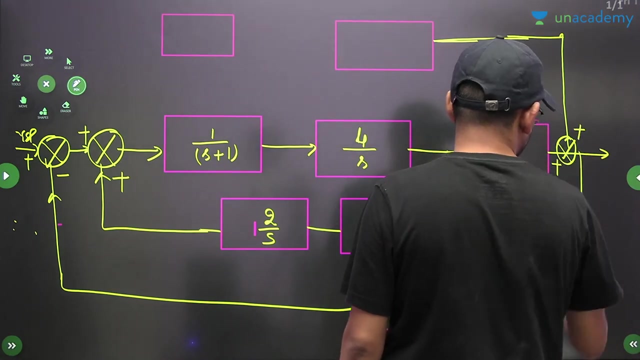 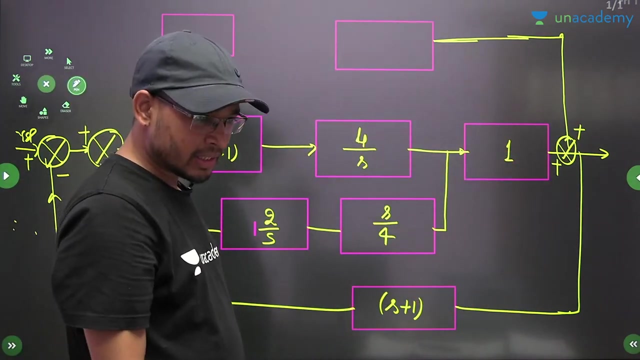 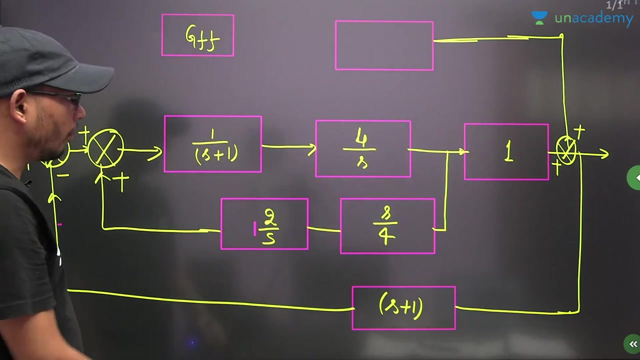 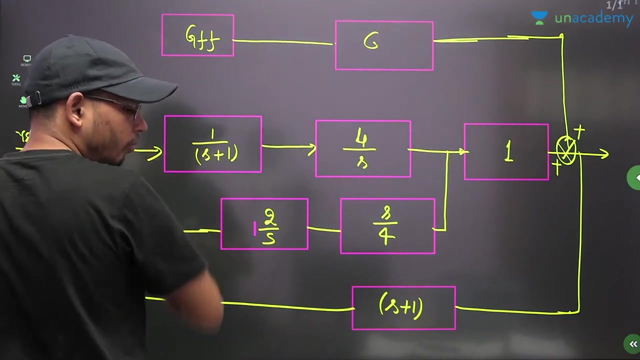 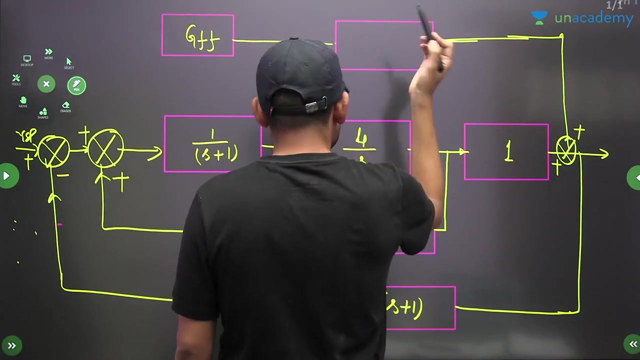 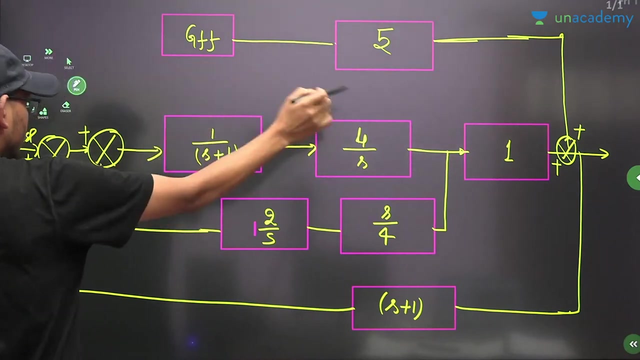 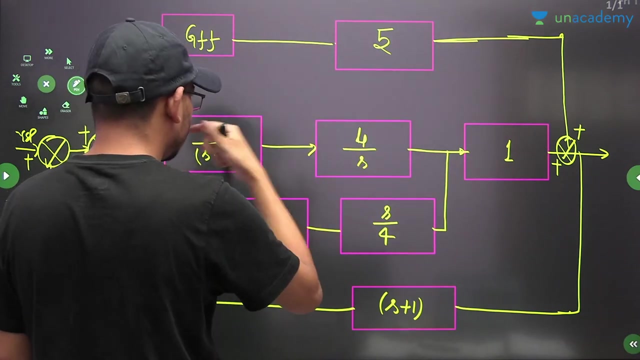 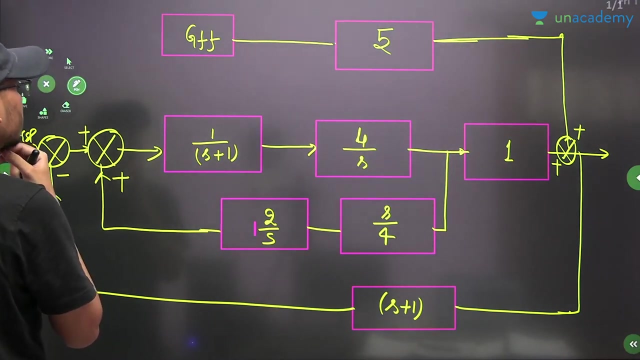 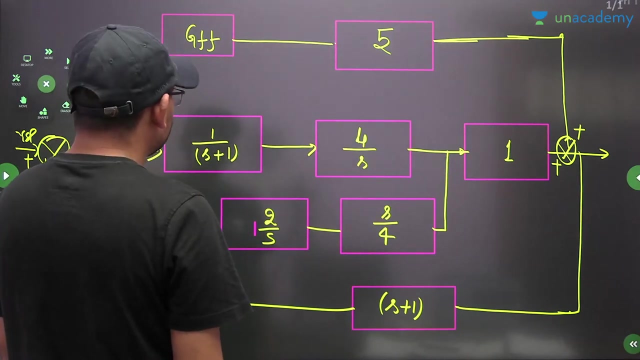 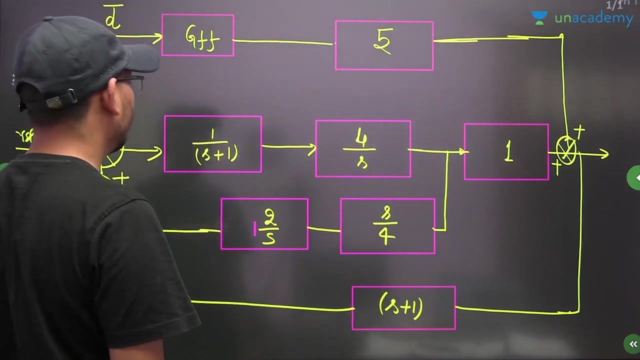 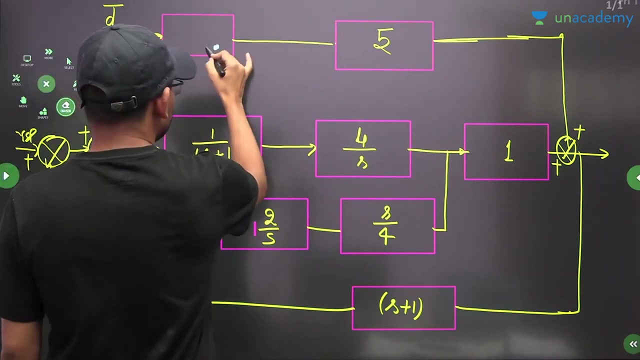 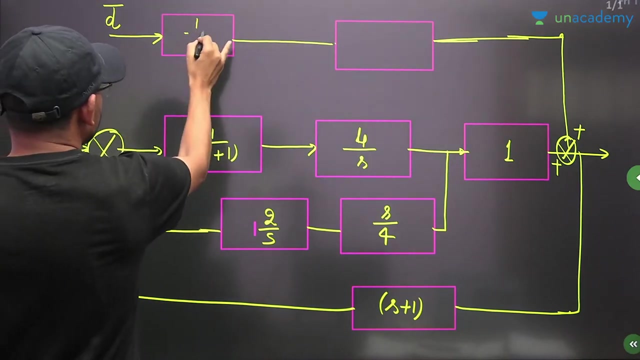 Okay, it will be solved easily. don't worry, it's easy, it will be solved easily, Okay. Okay, don't worry, it will be solved easily. don't worry, Give me a minute's time. Okay, it will be solved easily. don't worry, it will be solved easily. 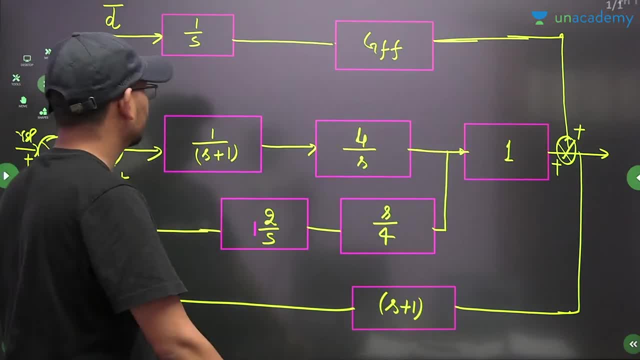 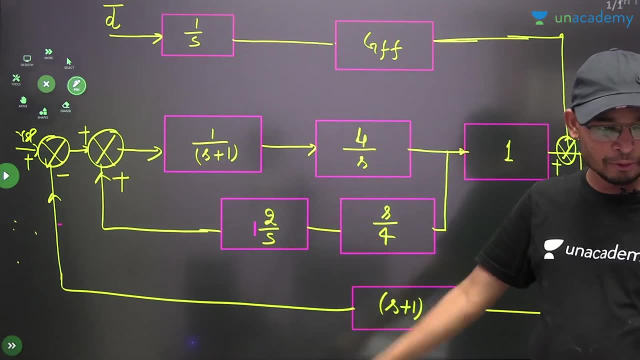 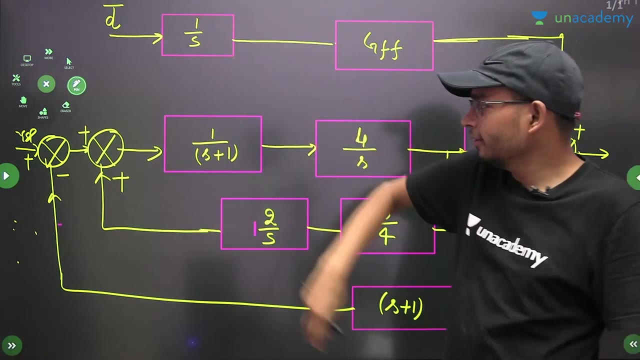 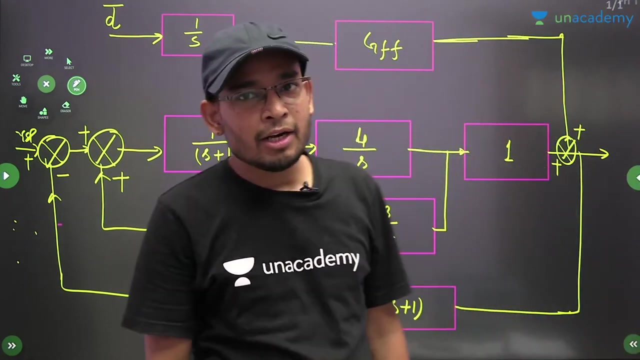 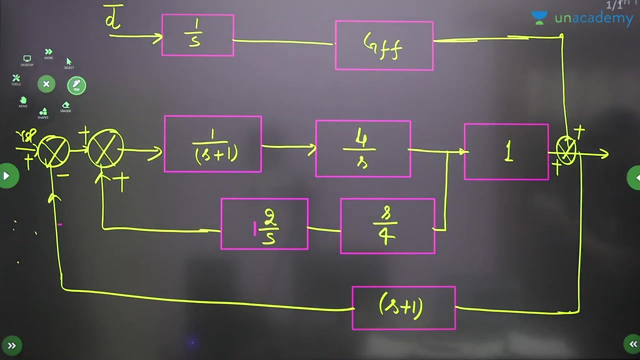 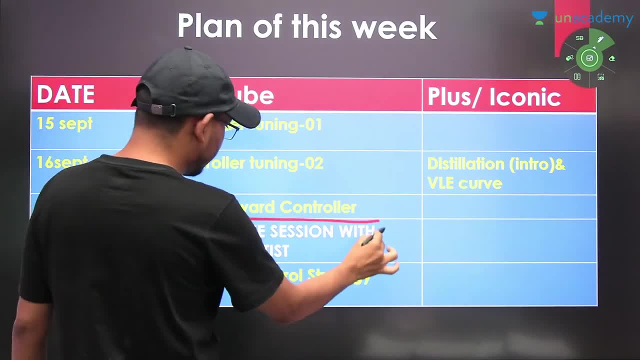 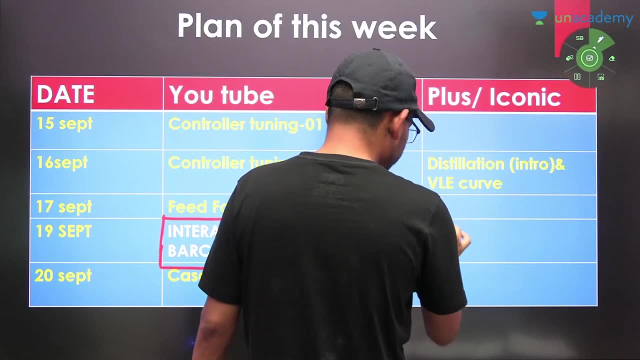 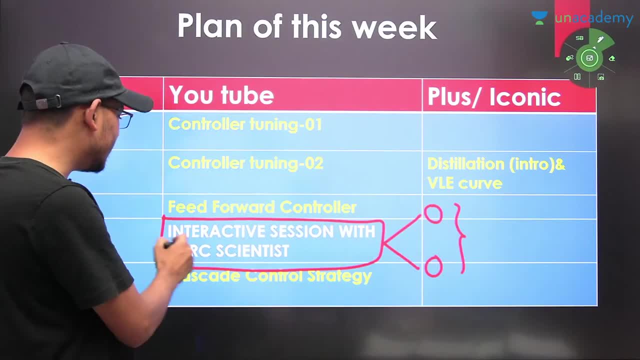 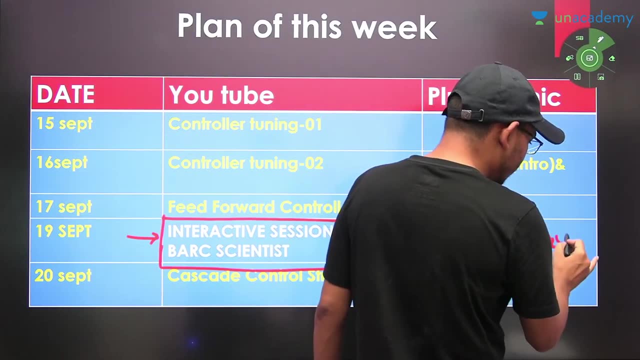 Okay, it will be solved easily. don't worry, it will be solved easy. Okay, we got. either we heard about this or we have seen this. Good, thank you very much, sir. There's something wrong in our worry: so power we forget right. 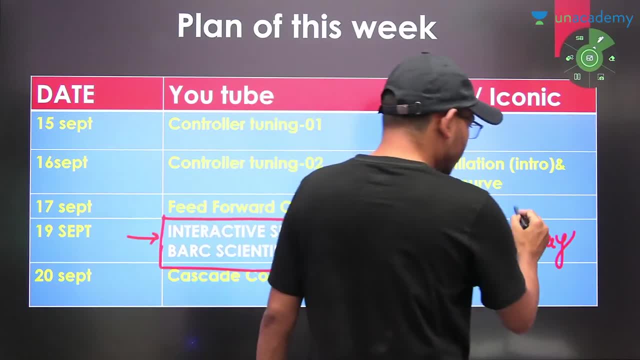 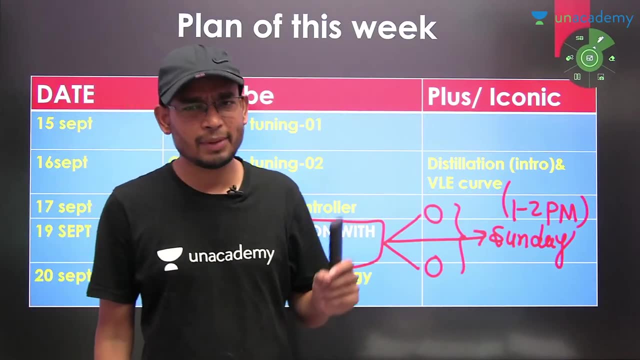 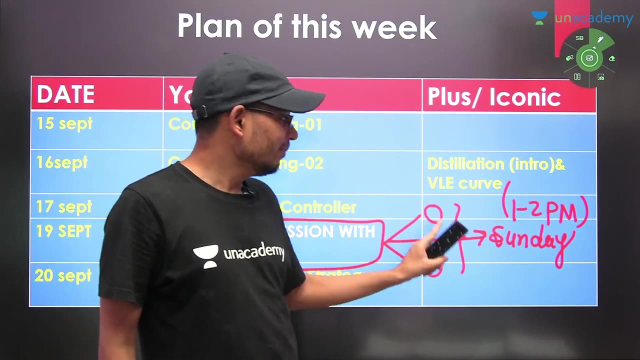 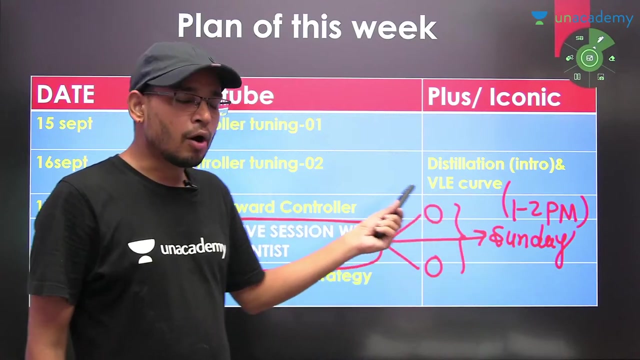 You will have a session on Sunday, the timing of which will be 1 to 2 pm. so you will set an alarm once and I will provide you a link. everyone should be on Saturday before Sunday. everyone's status should be set. I should see everyone's status definitely set this session on Sunday because this is going to be a very informative session for you guys. and now your bark will come after 3 to 4 days, so how do you have to follow the process properly which is present in the current bark? 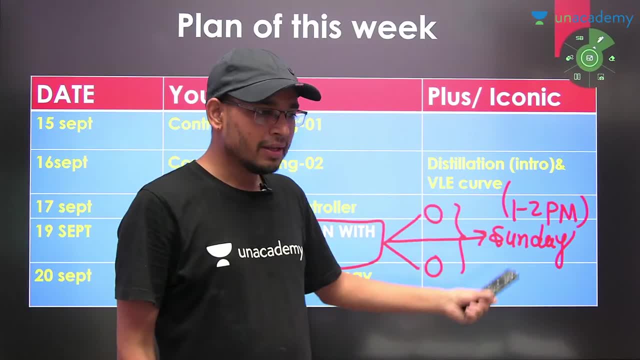 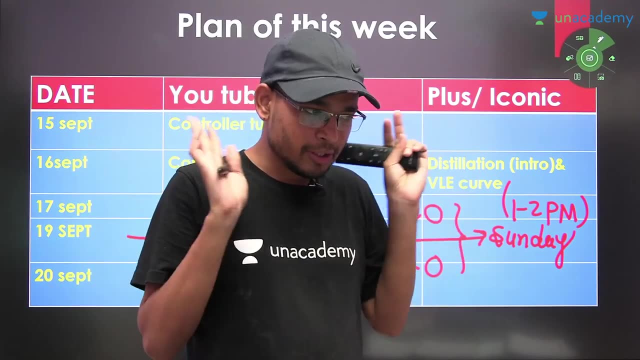 and my experience is that I will share with you guys. this will be your timing brother. yes, timing will be 1 to 2 pm on Sunday. I have kept this class running at the same time and this session will be on September 20,. the last lecture will be of cascading. 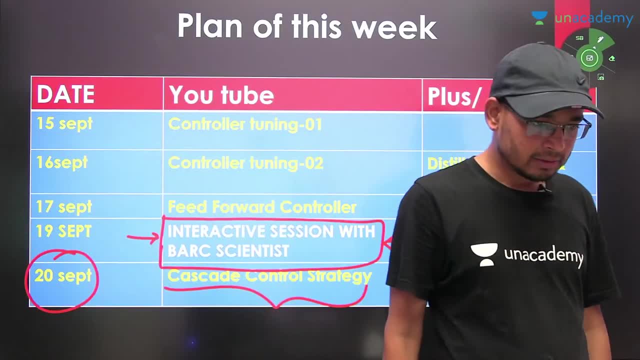 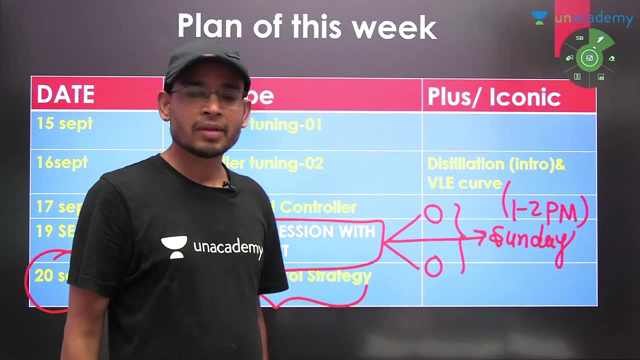 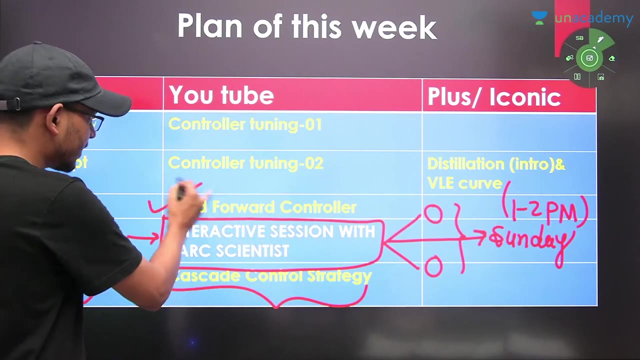 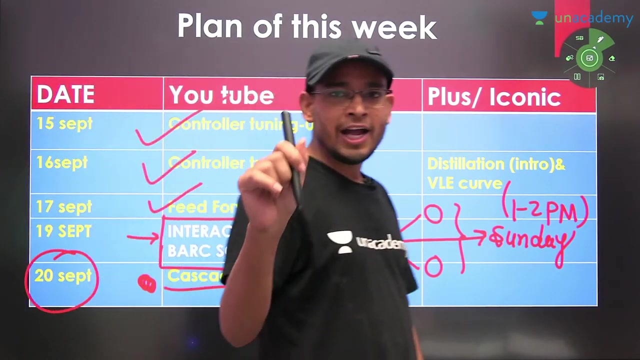 this will be the last lecture of cascading. yes, yes, I will give you a link. the link is in our telegram group. you will get a link by evening. so this will be an interactive session, properly between 1 to 2 pm. right now your feed forward is over. the controller tuning is over. ok, only one part is left- cascade control strategy. one part is left- cascade control strategy. ok, we will cover this on Monday. 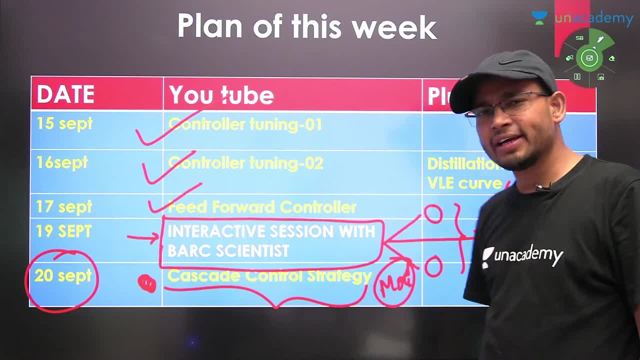 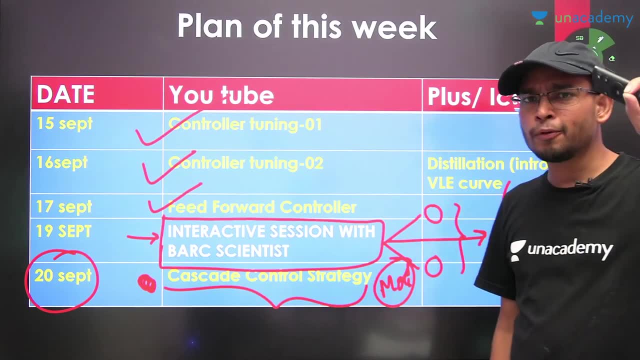 your class will not happen on Sunday, in case you want to see. then you will get a session on an app. you will get a session between 1 to 2 pm on the app. if you get it, then you will get a link. you will get a link properly. 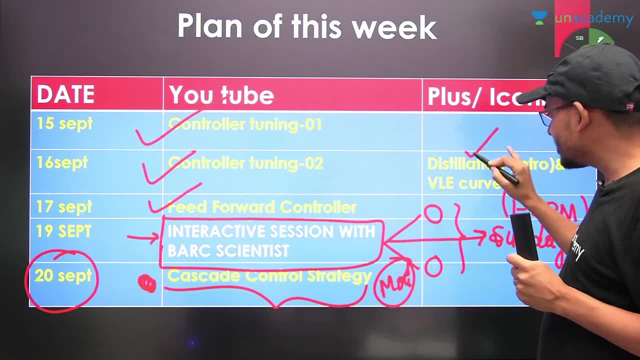 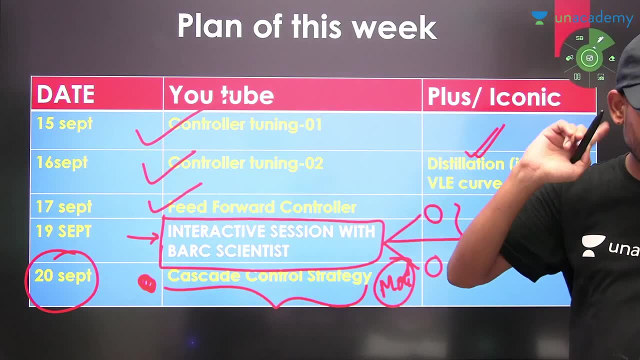 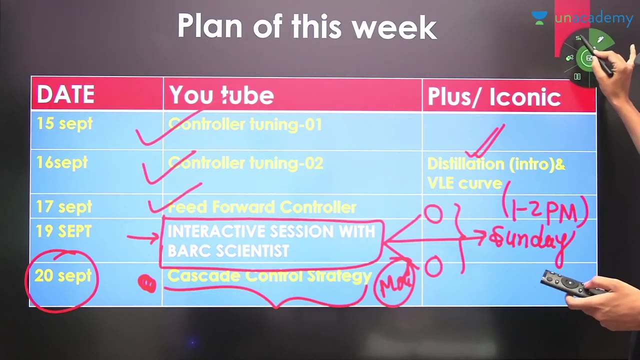 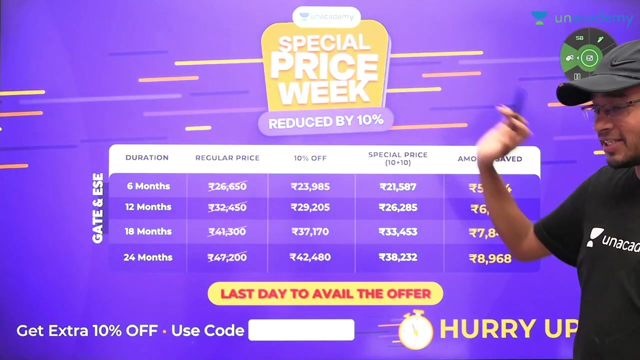 and the second important thing, brother, there is a distillation going on for the students of the plus. then whoever wants to move with the plus, they can move with me with the distillation. you will enjoy properly from here. ok, yes, so note this thing now. I will tell from here. look carefully. one more information now. see, those people who think that this special has been reduced by around 19 percent, ok, 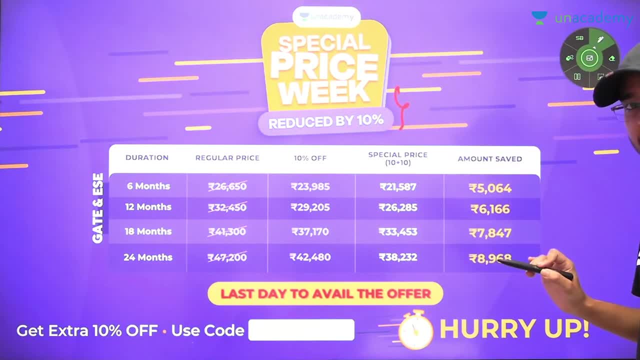 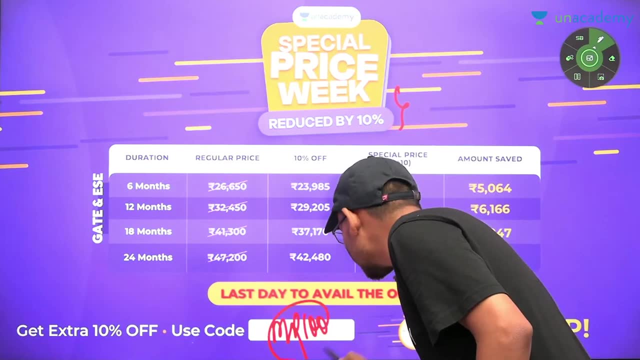 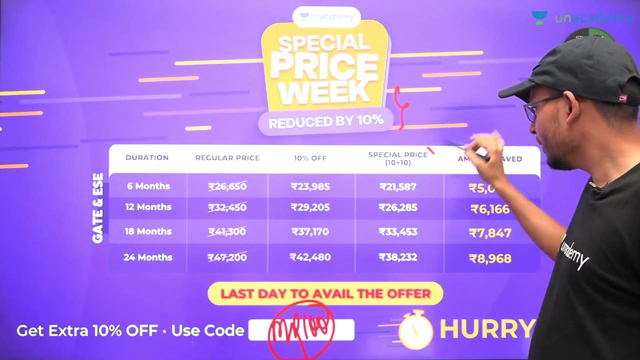 right. 10% is being provided by Unacademy and 10% you will use my code MR100. So you have to use the code MR100 and you can move from here properly. And in case you join for 6 months, then there is also an offer of 10% plus 10% available. 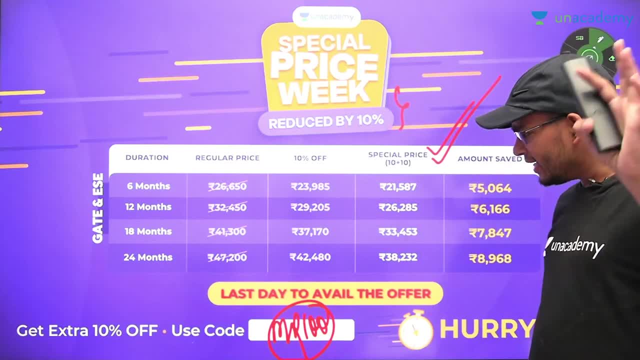 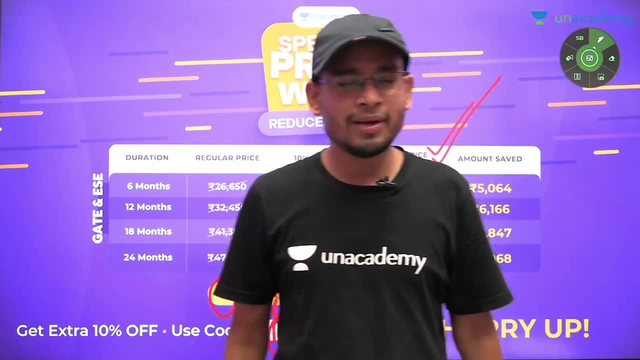 So with this you can move if you want properly, This is the last day, then you will not get to see such an offer again soon. You will not get it soon. the time will go on and on until you know that the mass transfer distillation is over. 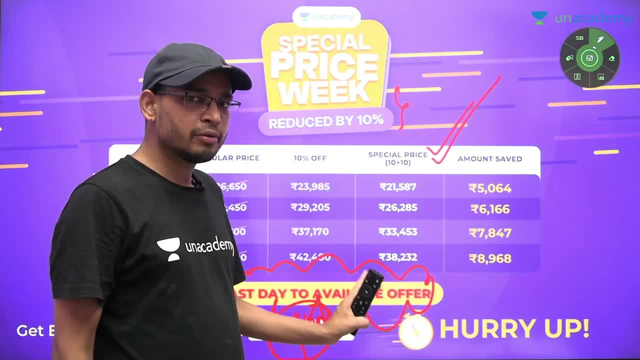 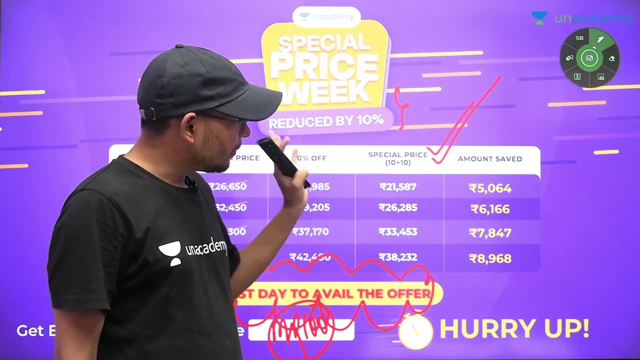 So, in case the distillation is going on, then take advantage of this offer and join atleast And take it for 6 months. you will get it in a very low way, So you can take it and you can utilize it in a very good way. 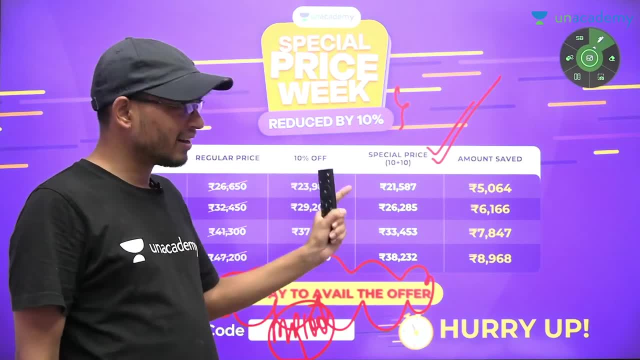 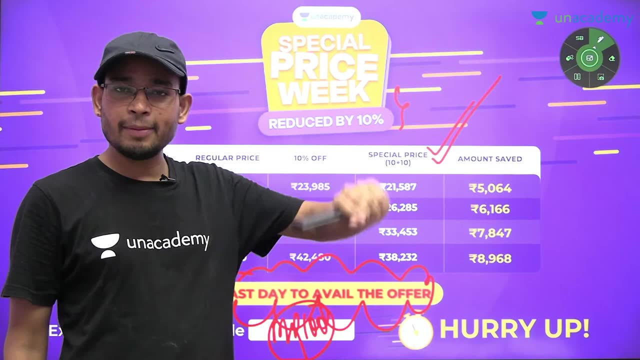 So this is the offer for today, and you have to study distillation. So now, distillation has been one lecture in which I have only told you the basics. Your boiling point curve will run today too. Your distillation will start from tomorrow. Even today, I will tell you the whole boiling point diagram. 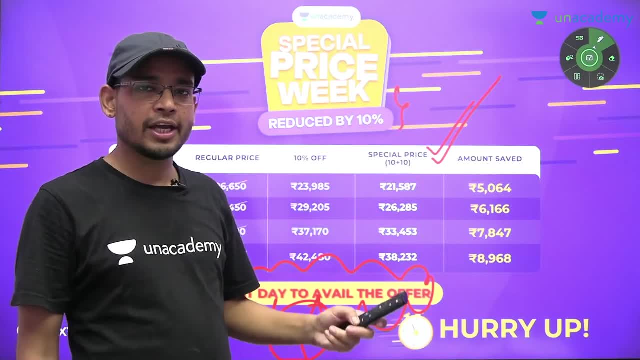 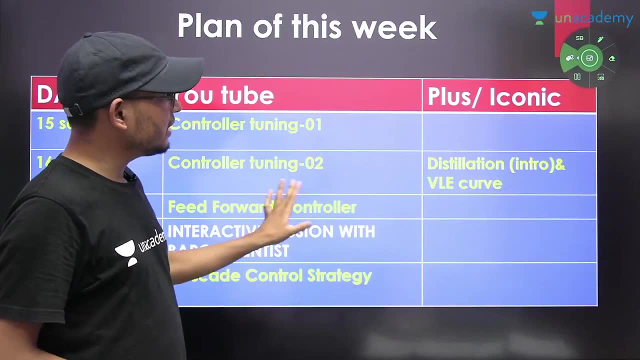 I will tell you the effect of the presser. There are many more things you will see in it in the evening, So the timing is 7.30 pm. After this I will just talk. this is done. this is done. This is my information. 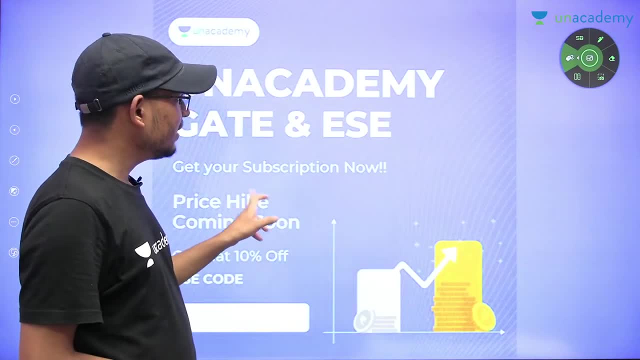 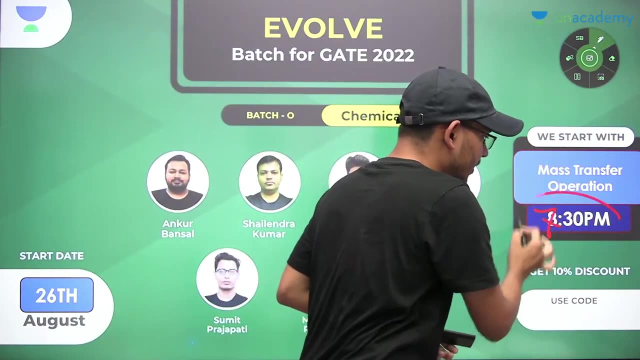 Now. the price will increase in the coming time, so you can save yourself from it And the mass transfer that is going on in the evening, whose timing is 7.30 pm. How much is your timing? 7.30 pm, So meet properly. 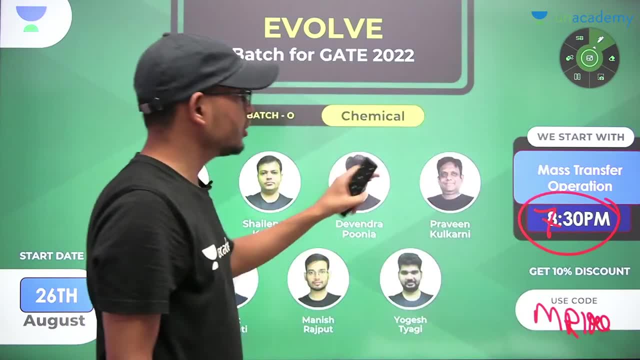 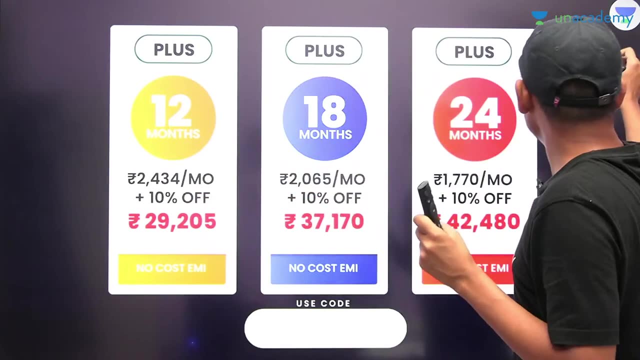 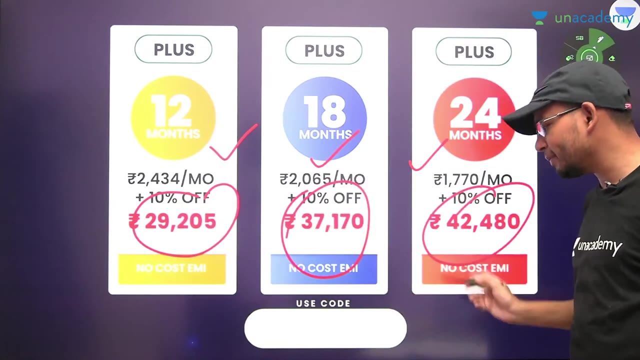 And you guys Use the code MR100. After this I will tell you about the fee structure: 12 months, 18 months, 24 months- See here the fee structure has been given to you, So every place you have 10%, 10%. this is 10% off.